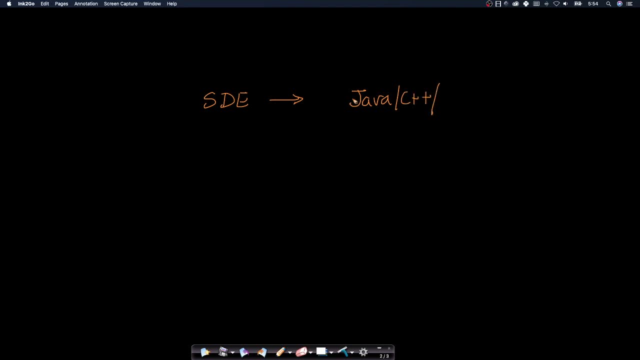 languages. It can be Java, C++, any object in which you're looking at. So, if you're looking at virtual programming, Python, again. Python is a very, very popular language now, But I see a lot of people doing Java. also fewer people doing C++, Again, data structures and 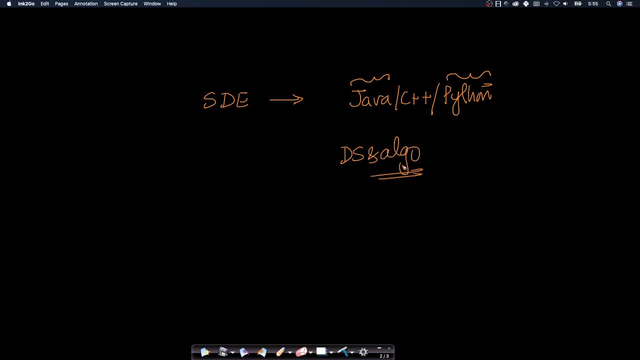 algorithms. We have discussed a few of the basics in the previous live sessions, but you should be able to solve, given a problem involving dynamic programming, or as or or or or, a good, interesting problem. The expectation at a top product based company is that from 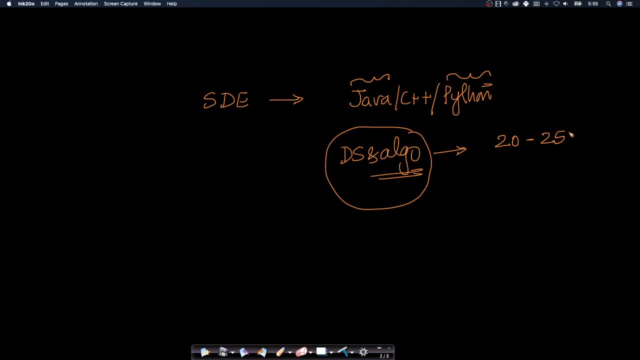 the time the problem is explained to you, you solve, you come up with a decent solution and you can solve the problem. So if you need to solve a problem, you can solve it with a simple method. write code in any major programming language in 20 to 25 minutes- okay, that's the expectation. so 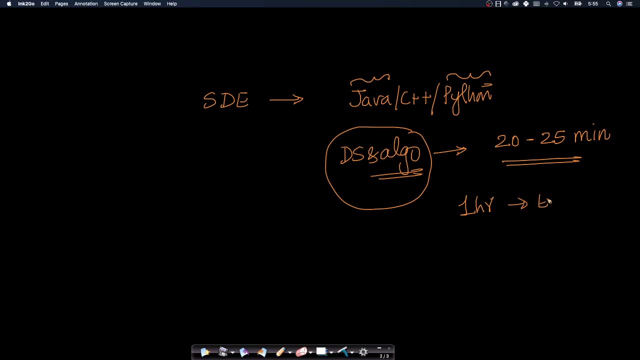 in a typical one hour interview, you will be given one easy one, medium, again. depending on the performance, you might be asked a medium or a slightly, slightly harder question. that's it, okay. so this is the. this is what is expected in a one hour interview. again for a fresher, you will: 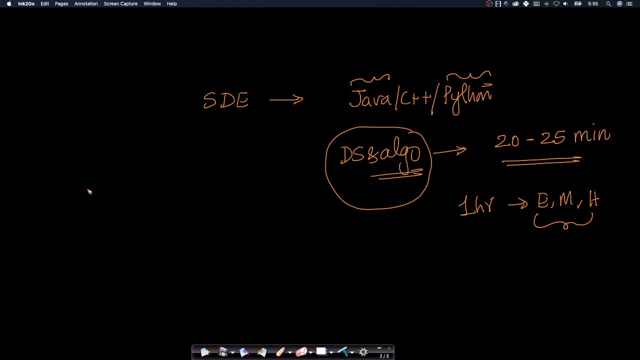 not be asked lot of lot of design. so if you are an experienced software engineer, you will be asked software design like low-level design, high-level design. as you become senior and senior, there is more focus on architecture design or high-level design. if you are a youngster, not so much focus. 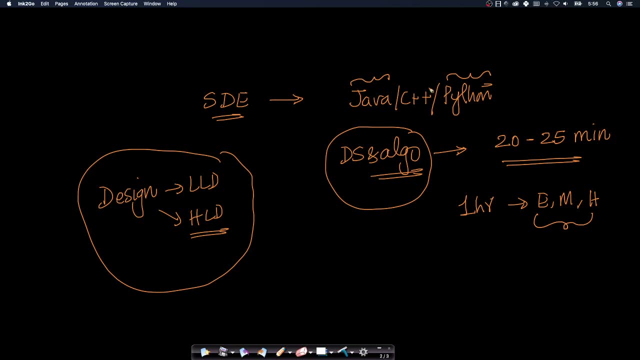 on design for entry-level software development engineers. it is simple: programming data structures, algorithms. in some roles they might ask SQL also. okay, some questions on data, especially for a computer science student. they might ask questions on databases, operating systems etc. But only 5% of the time they ask in databases and OS. Most of the time 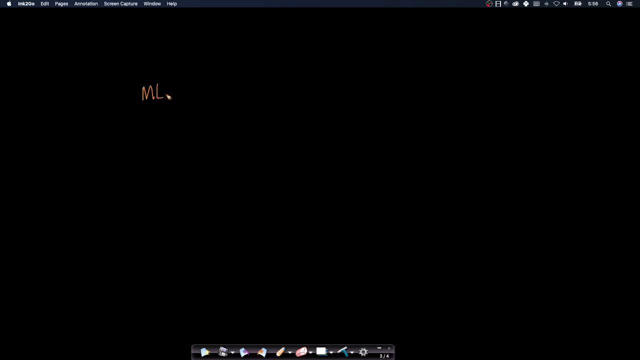 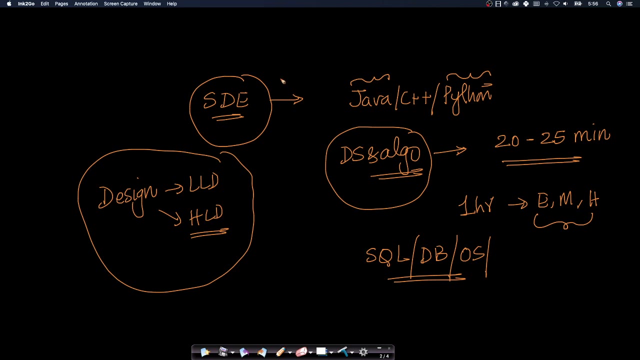 they'll ask on data structures, algorithms. For a machine learning engineer or a data scientist, the bar is lower, So the complexity of questions asked are certainly not at the software development engineer level, unless you're a CSC student or you come with prior software development experience. 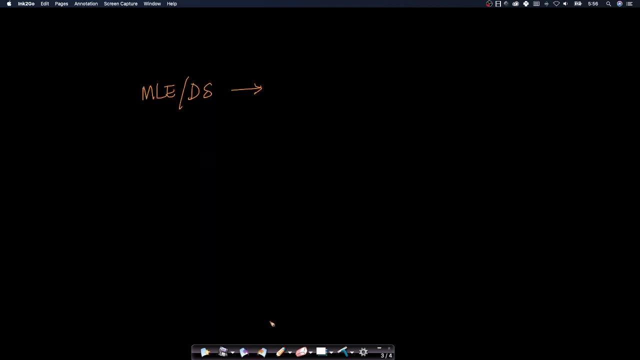 So the bar is typically one level less than software development engineers. Typically you will have one round or maximum two rounds of SDE-like interviews. Again, in these rounds also, there will be focus on the problems that are typically asked are simpler than a typical. 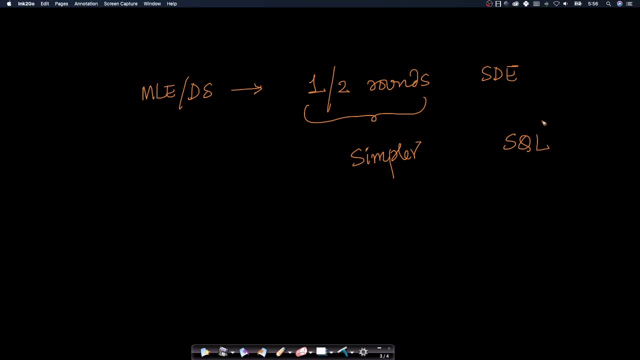 software development engineer. There is, of course, some focus on SQL for most data science roles because they expect you to be able to write SQL queries. The complexity of problems is certainly lower than software development engineers, Like most companies, typically have one round. 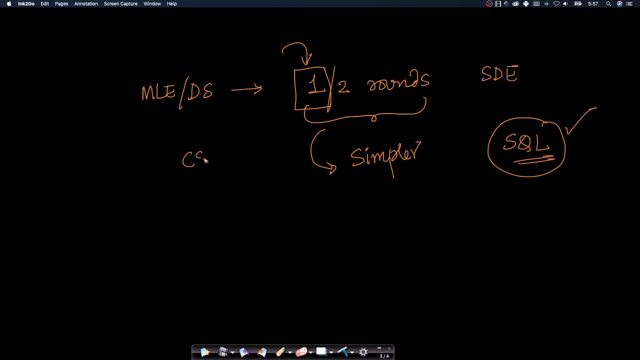 Again this round. also, the complexity of this round depends whether you come from computer science background or you come from non-CS backgrounds. If you have worked in software, if you worked as a software development engineer, certainly the bar is going to be like a CS student Right. So again, there will be most. 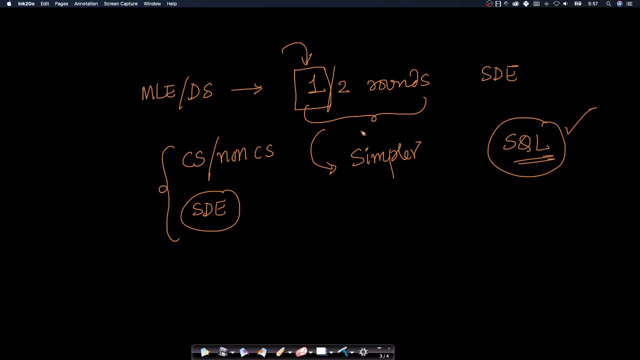 of these questions are not hard to be honest with you, Right? So we have shown, we have seen we have solved some problems in the previous public live sessions. They are a good benchmark Again. I've picked up a few problems from my own interview experiences. interview experiences of: 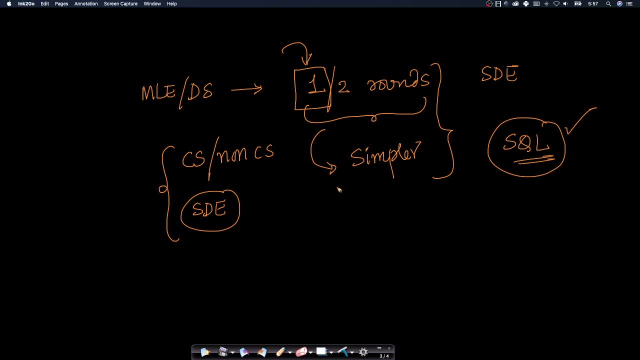 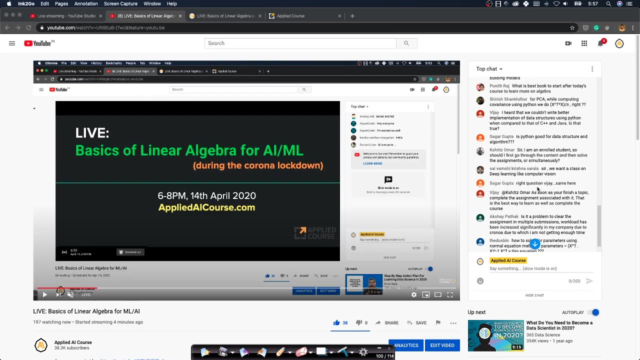 others in top product based companies and showed them in the previous live sessions. Right, So you can check those out. Cool, Okay. so okay, somebody has another question. Sagar has a. says right question Vijay. Okay, which question is this? I heard we couldn't write better implementation of 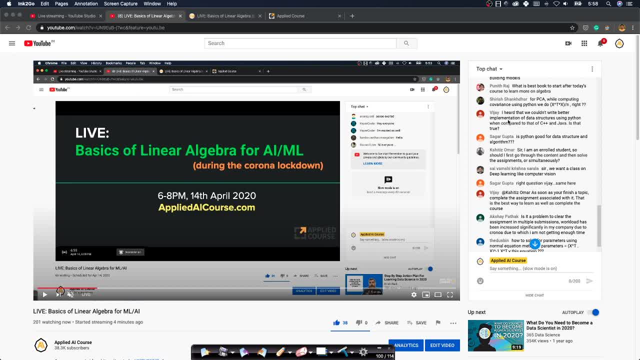 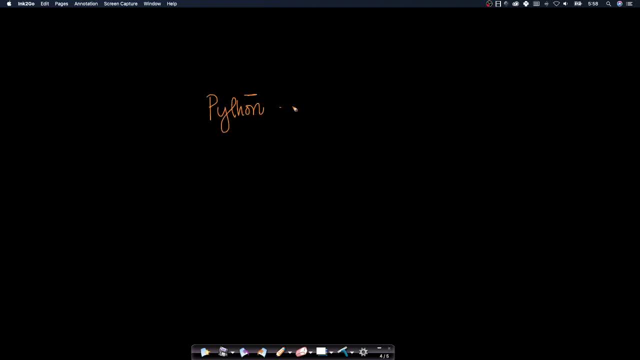 data structures using Python when compared to C++ and Java. Is that true? That's a good question. The biggest problem with Python is it is slow. Okay, this is one of the biggest problems with Python. So what happens is a lot of data. 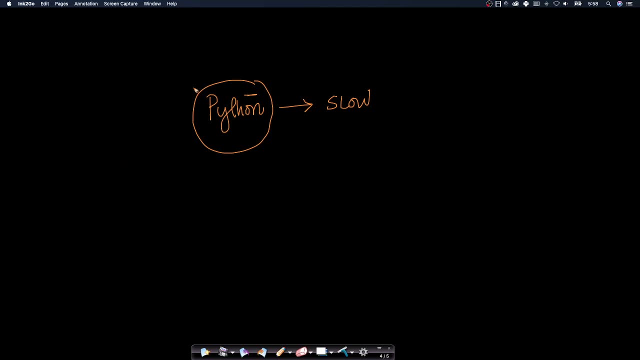 structures a lot of numerically intensive computation that we use in Python. for example, take a list right or take a dictionary in Python. all of them are internally implemented using C, C++, Because that's where the speed comes from. Again, don't think that Python is. 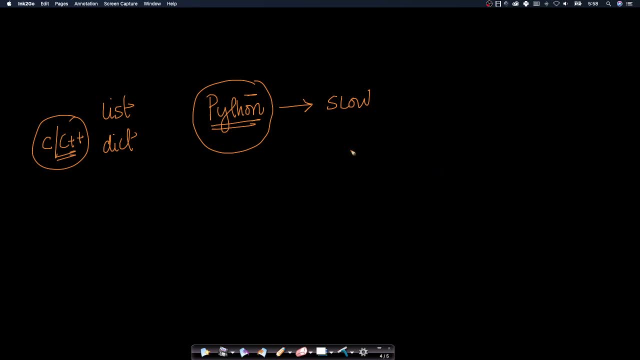 not production quality. There are a lot of companies which use like, for example, take, take Google right- probably one of the best software engineering companies in the world- that they have right, They write most of their production code in C++ or Python, Of course, 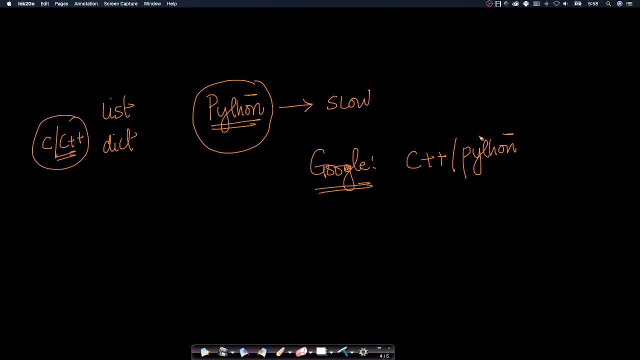 they also write some in Java, because Android is based in Java, Right, But they use Python in production, Right. Look at, look at TensorFlow and Keras, right, which are, which are some of the most popular machine learning libraries. The reason everybody created Python interfaces for. 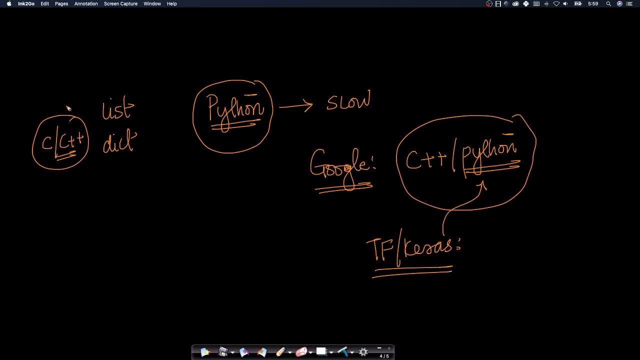 that again, the core implementation itself is in is in C, C++ for speed. But Python is much more easier to run, easier to maintain, easier to pick up and the the the breadth and depth of libraries that you have in Python are are like I don't think any other programming language today can even come close, especially for 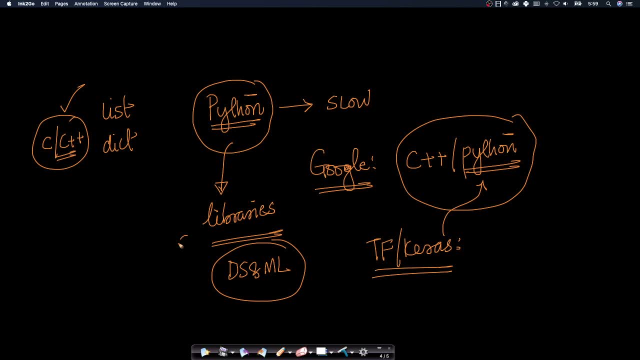 data science and machine learning applications. This is almost one of the best hands down, Right? So don't think Python cannot be productionized. It can be productionized if you use the right data structures and right libraries. For example, there is a lot of NumPy code which is actually 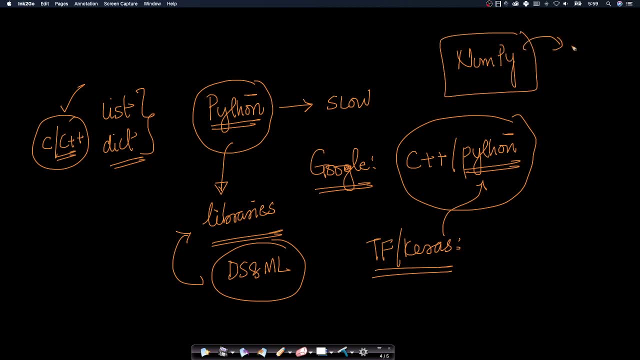 productionized because all the internals of NumPy, as we have seen in the previous live sessions, is implemented in C and C++ Right. All of the operations underlying NumPy are actually written in C, C++, making everything much, much faster. So Python as long as the critical time. 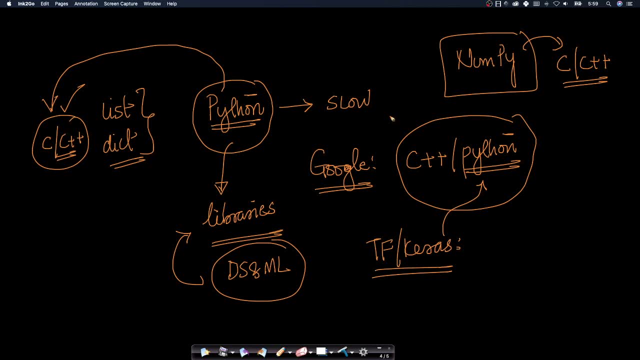 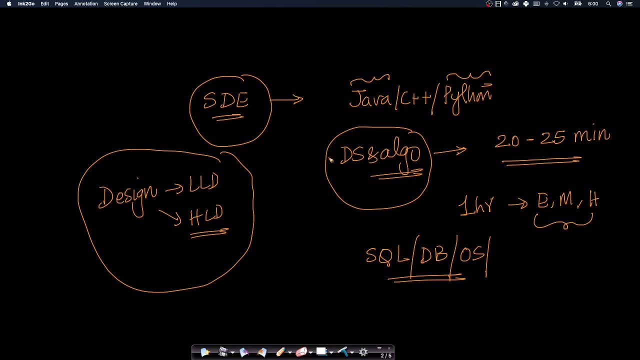 intensive stuff is implemented in C, C++. Python is more or less production ready, Right. So again, if you go to an interview, if you say, Okay, I'm a Python guy, I prefer writing code in Python, nobody will hold it against you. But you should know the limitations of Python, Right, You should. 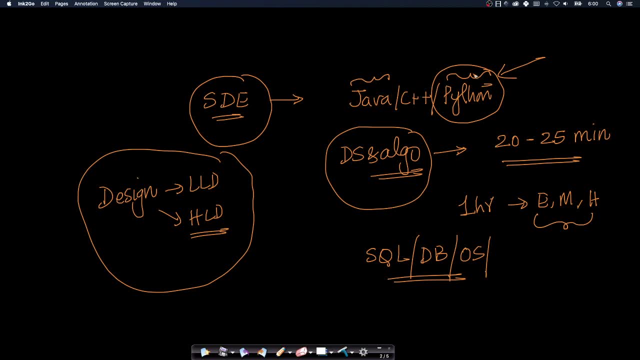 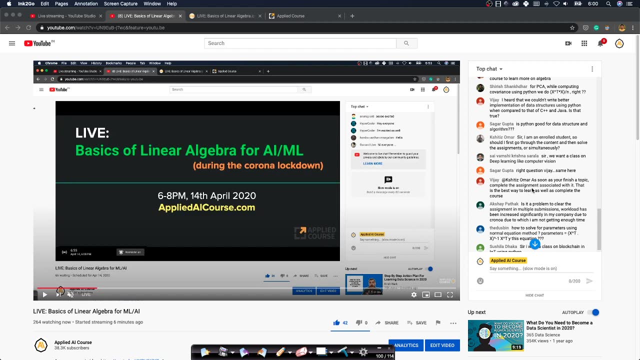 know where Python lags, where Java is better, where C++ is better. that high level understanding is good enough. Nobody will hold it against you that you're using Python. Okay, somebody says You want a class on deep learning using computer vision. Again, as I mentioned to. 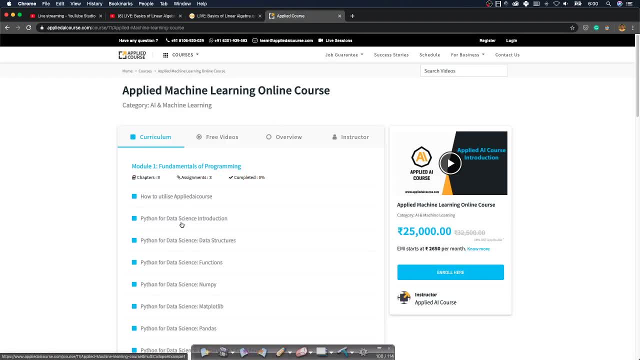 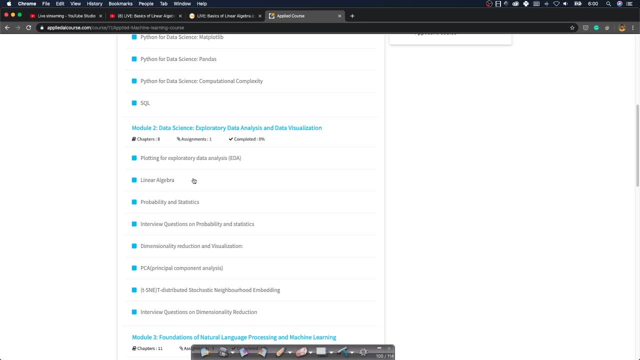 you earlier. we are going in a sequential manner. we completed most of module one, which is basics of Python programming. Today I'm in, sorry. today we are doing linear algebra. So I'm going step by step, chapter by chapter, in our course video. 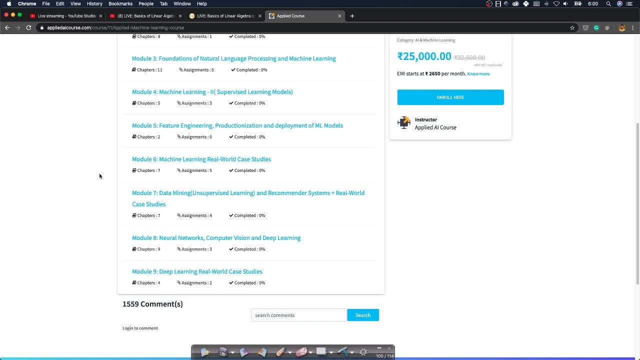 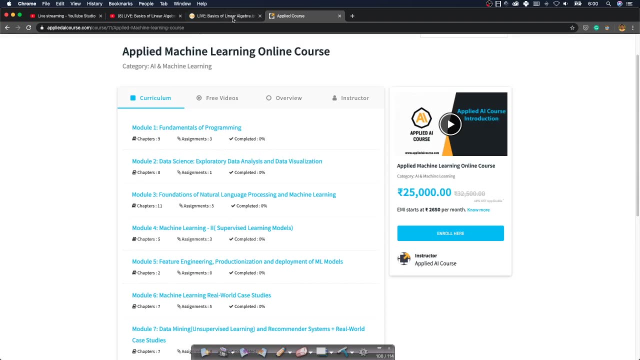 and certainly hopefully, since the lockdown is also extended to may 3rd, we will be able to complete most of the chapters that we have in our course videos by the end of the lockdown. right, so we are going step by step. okay, that's important. there is no point me jumping directly to deep learning. 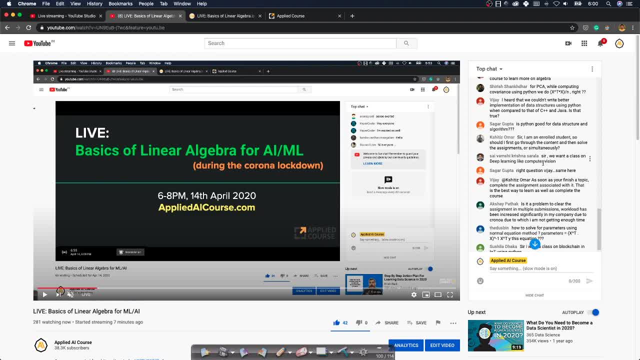 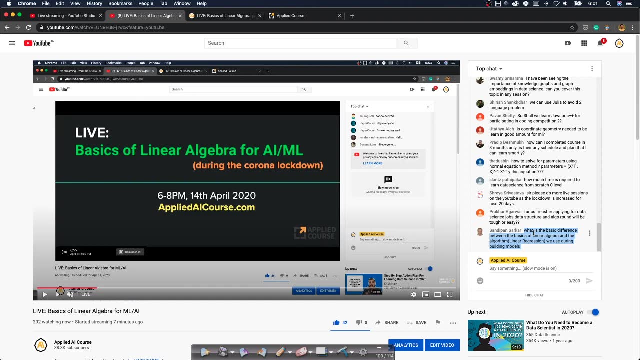 we'll do that again today. we'll see a very simple in linear algebra how computer vision, how a lot of computer vision operations are actually simple linear algebra, right, we'll see one of the examples in today's live session, also cool, oh, so okay, good question, Sandeepan. so what is the difference? 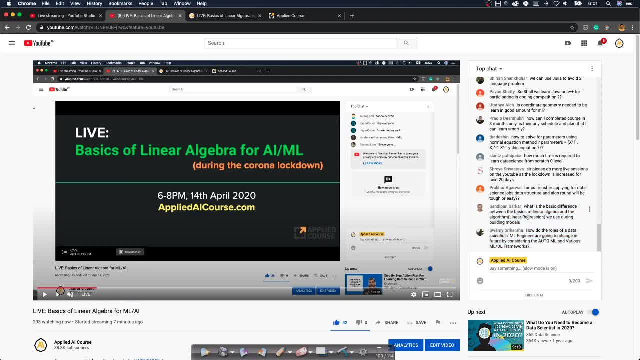 between basics of linear algebra and linear and linear regression. I'll mention this again. we'll wait for a few minutes. let everybody join in couple of minutes. it's 6.01. so I have- I have a detailed notebook. I'll share this notebook. by the end of it, I'll tell you what we will cover. 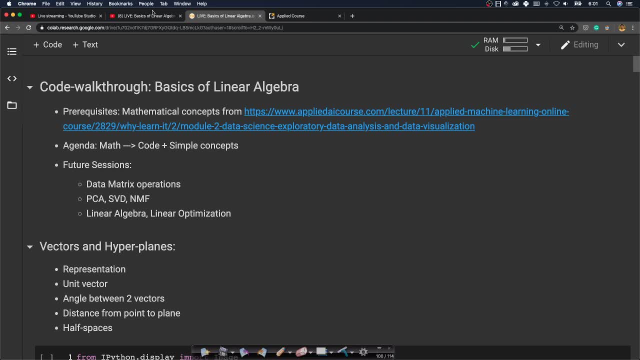 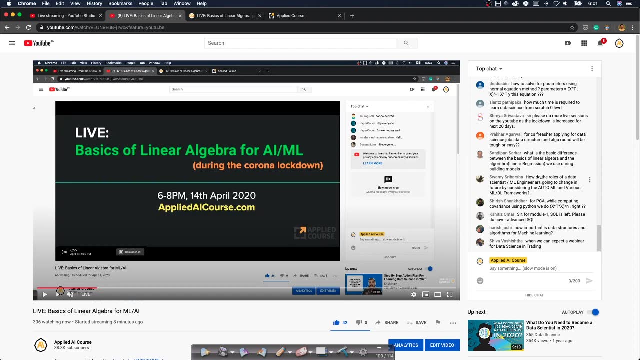 today. what are the future sessions in which we'll cover other topics? okay, of course, linear algebra. if you look at a typical linear algebra textbook, it covers a lot of things. it covers even linear regression, right, so we'll do that, okay? so somebody says: okay, I've 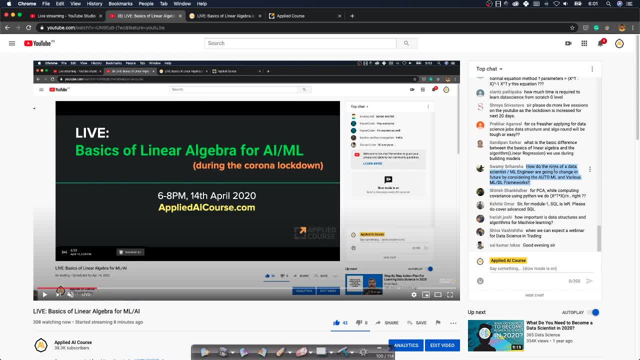 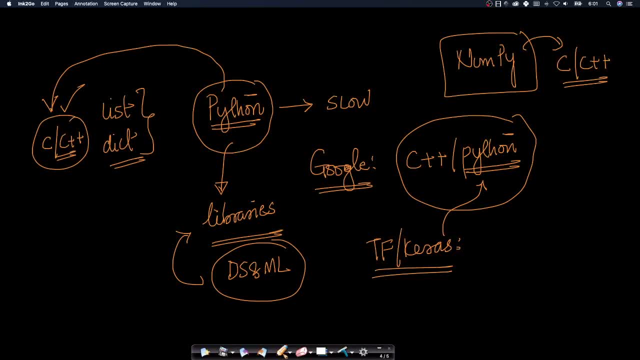 answered this question multiple times: how do the roles of data scientist, ML, engineer going to change with Auto ML? again, the most important thing here is: even if you are using Auto ML architectures, look at any Auto ML architecture in the world. right, even the best of the best at Google, right? 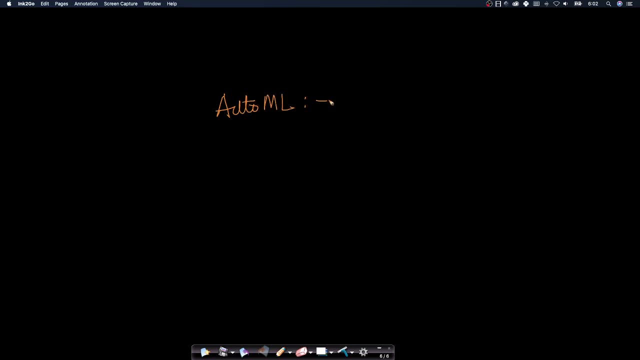 so Auto ML speeds up the the pipeline for you. okay, I worked in a world where we did not have scikit-learn like libraries. okay, in that world we had to implement a logistic regression function. okay, we had to. I mean, I also. I also implemented simple multi-layer perceptron, simple convolution neural network. in again this: 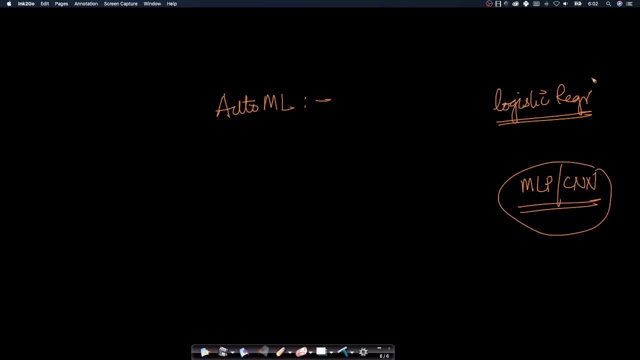 is before tensorflow, before ksds. so what happened in the world is: these libraries made our life simpler. okay, because I have scikit-learn, I have a pipeline for you. okay, I worked in a world where scikit-learn because I have tensorflow, or carers because I have xgboost again, we have implemented. 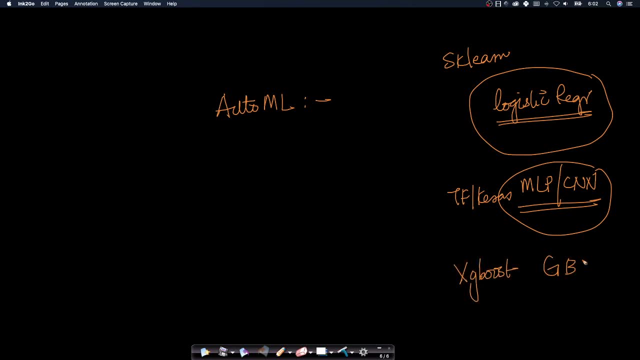 GBDT at scale. in my previous company right, we implemented GBDT at production scale before we used xgboost. so even before these libraries existed, the machine learning folks were implementing these things and using them internally within the companies. so what these libraries did was it's 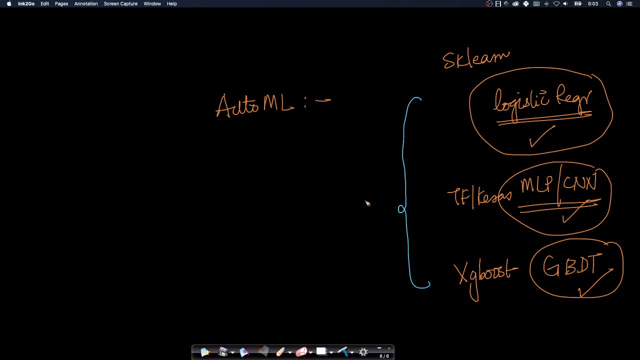 it's. it sped up. it speeded up the whole thing, right. so what it gave us is speed in terms of trying out new models, again without tensorflow, carers and pytorch, today, building building deep neural network models from scratch is fairly non-trivial. okay, because we have tensorflow. 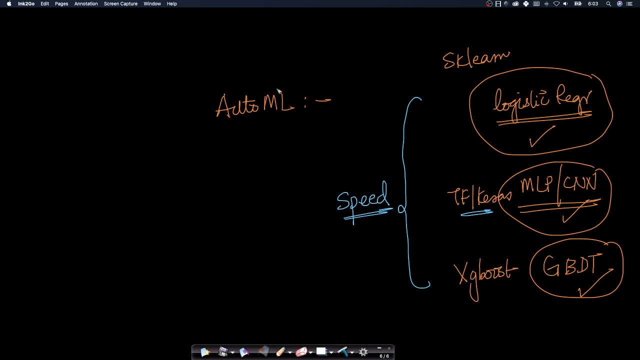 carers and pytorch like libraries. we have simply improved it. AutoML, as we see it today, is mostly being used in the, in the framework of, in the framework of deep learning, for architecture search right. so for the, for the task of architecture search right. so what is architecture search? for those of you who know a little bit of deep learning, 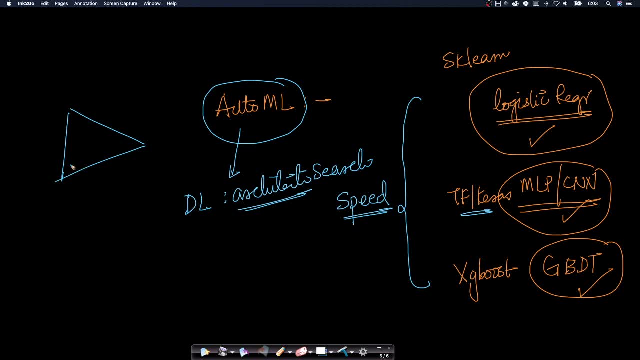 suppose you train a deep learning again. there are a bunch of very popular deep learning architectures that you have, but if you want to search for the best architecture for your problem, it requires a lot of hyper parameter tuning. right, it requires a lot of hyper parameter tuning and lot of experimentation. what AutoML is doing is it is simplifying and speeding. 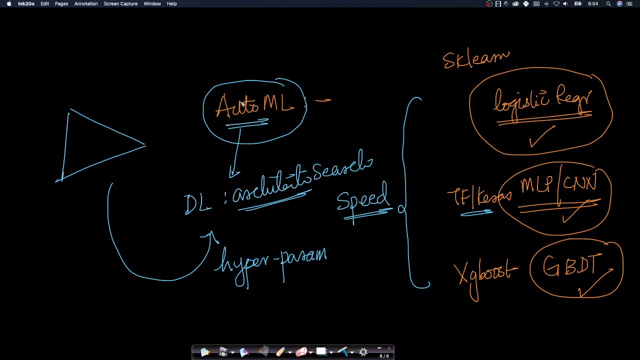 up that process. see, look at what is the scope of AutoML today. right, can AutoML design a features automatically for you from tabular data. right, can AutoML, given a real world problem, can AutoML pose the problem and solve it end to end? we are not yet there. we are actually far from it. 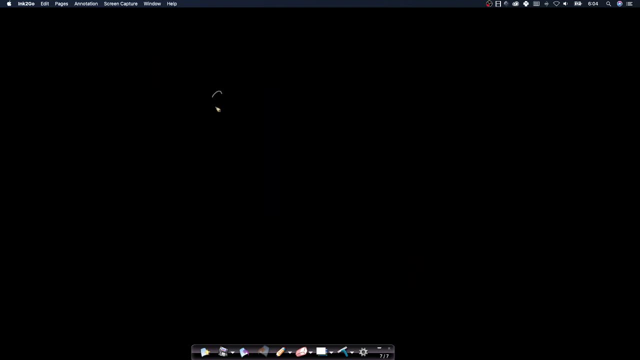 okay, just because, okay, the- the analogy that I give here is: just because there is compilers doesn't necessarily mean that there are no software development engineers today. compilers, what did? what did modern compilers do? right, pre compilers, people wrote software, but compilers made life easier and it made programming accessible to many, many people, people who didn't know how code. 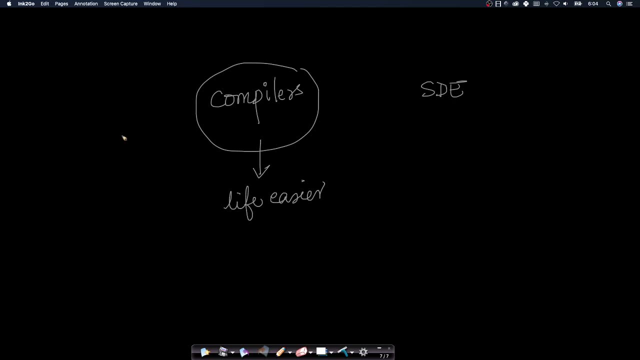 works internally. people who didn't know- linkers, loaders, the system software, okay, how the operating system works. now somebody can write code in python and not care about how things work internally. the compilers, interpreters, loaders, linkers, everything- take care of it. so they made life easier. 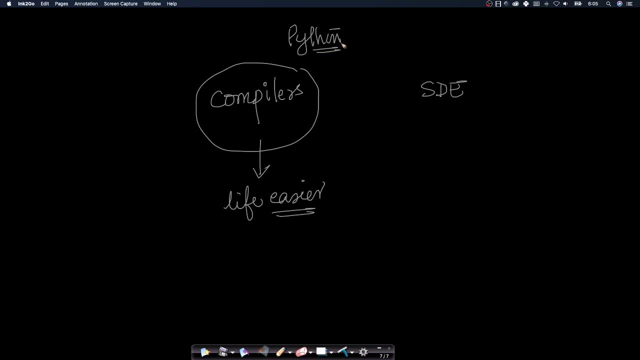 democratizing access to programming. but even with all of this, there is a huge demand for software development engineers. I think something very similar will happen: right, people who have core expertise in machine learning, AutoML- whether it is AutoML or whether it is libraries- right, like tensorflow, they. 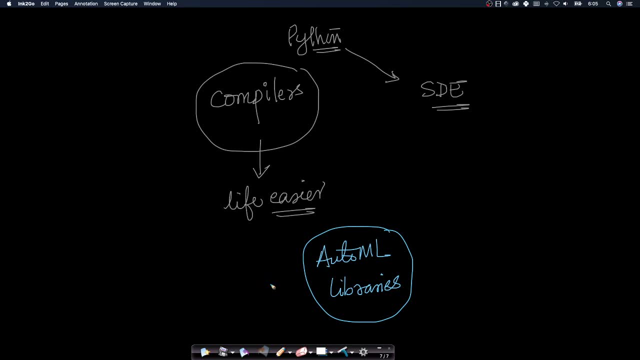 make our life simpler and faster. okay, this also makes the, the whole technology accessible to a wider set of people, but that does not mean that the demand for machine learning engineers or data scientists decreases. because of modern compilers and modern programming languages, the demand for software development engineers actually skyrocketed, right. so look at python or look at Java, because there are so. 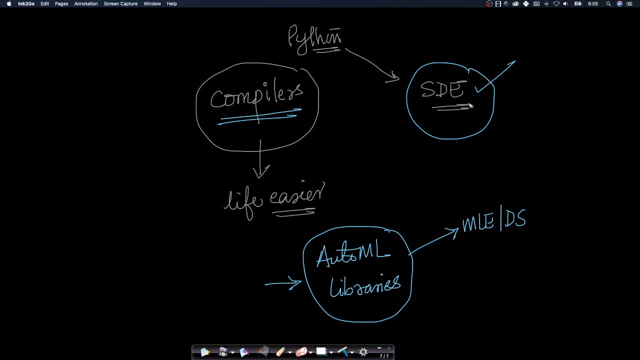 beautiful languages, where compiler takes care of so many things. there is more demand for software development engineers today. I think all of the libraries, all of the AutoML stuff today will increase the demand for machine learning and data science folks because more people can access it, more companies can build these technologies at a lower cost, right, cool. so, uh, somebody says, is it? 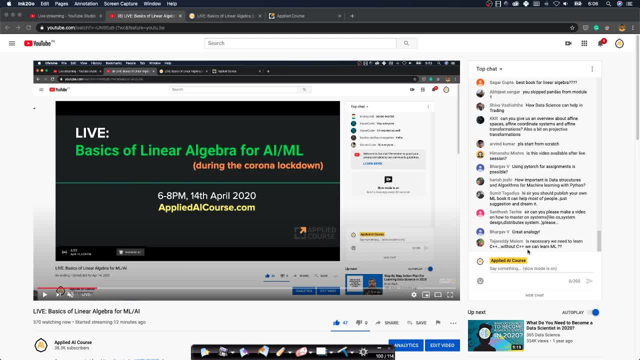 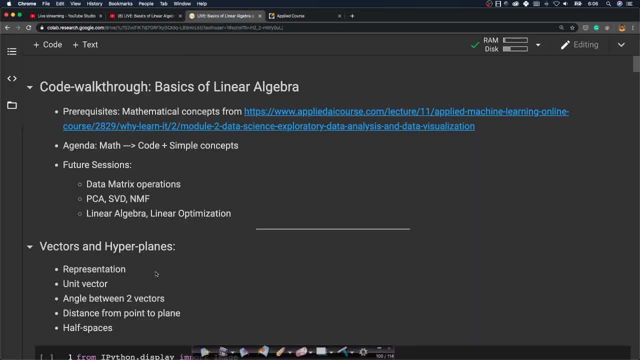 necessary, okay, so. okay, it's already 606, so let's dive into it. I'll take these questions again after a while, all right, so okay, so let's dive into the session itself. uh, okay, this is the. this is by. again, I'm writing this in collab so that it's easier for me to share it with all of you. as I've mentioned, 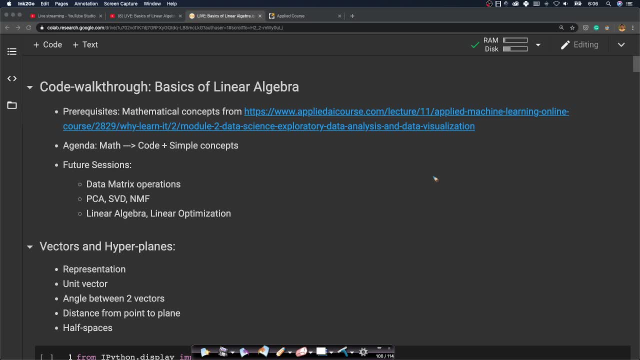 in the previous sessions also, I will share this collab notebook at the end of the session, right? so at the end of the session I'll share this collab notebook with all of you in the comment section itself, also in the description section of this video. so let me, let me list down the scope of today's session. so this session is called basics of. 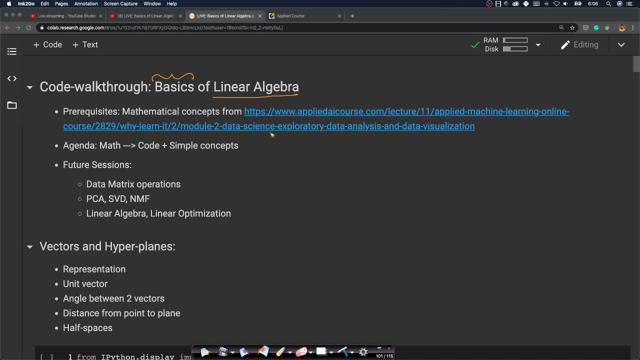 linear algebra, because it's impossible to cover a lot of concepts in linear algebra in just one session. that's why, even in our course videos, we broke it up and and taught various aspects of linear algebra at various points in the course, right? so I'm assuming that you've already gone. 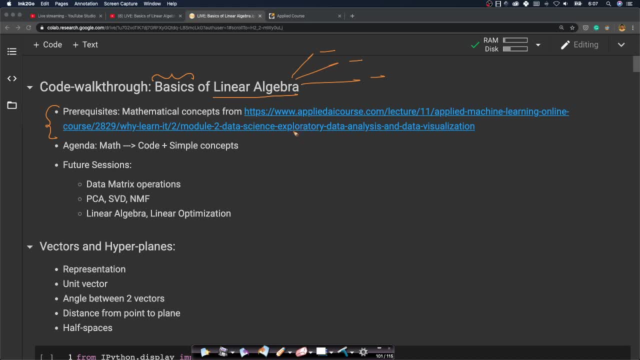 through the link that I've mentioned in the uh uh, uh, so, uh. again, somebody is asking: can you send the video? don't worry, you'll get the video. also, it will be on YouTube. okay, so this is. this is a public live session. you can access it even after the live session is over. okay, so, uh, okay, so I'm. 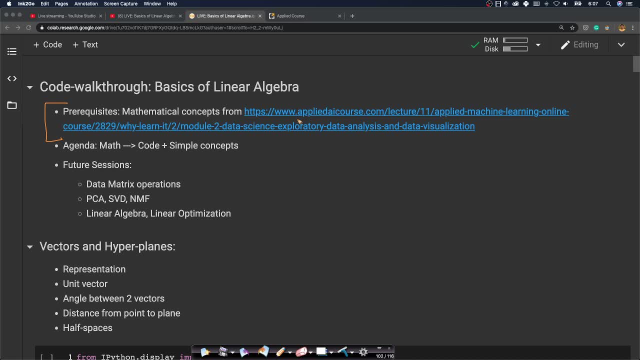 assuming, in the announcement video I gave you a link to free videos on our course. I hope everybody have gone through it, because I will not be repeating the mathematical concepts that are there just in the interest of time, and the agenda today is to take the mathematics that we have. 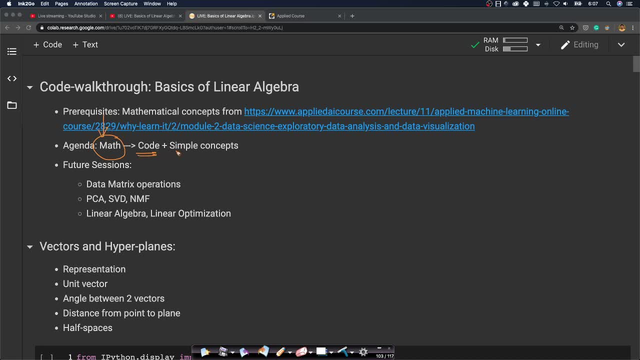 already covered in the course videos and convert it to code again. all this will be simple concepts. linear algebra is a beautiful topic with lots of areas, right. so what we limit ourselves to is only the linear algebra basics chapter in our course, right more, there are lots of other concepts for. 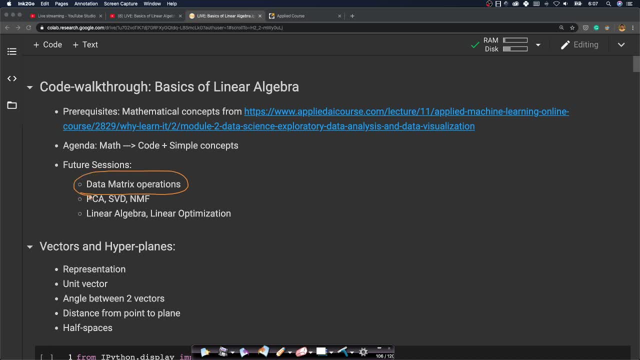 example, there are tons of operations like normalization, standardization, Etc that you do on data matrices. this is what we'll do in future sessions. there is a lot of matrix algebra like principal component analysis, singular value, decomposition, non-negative matrix factorization. again, we have covered these concepts at different points in our course, for example in dimensionality. 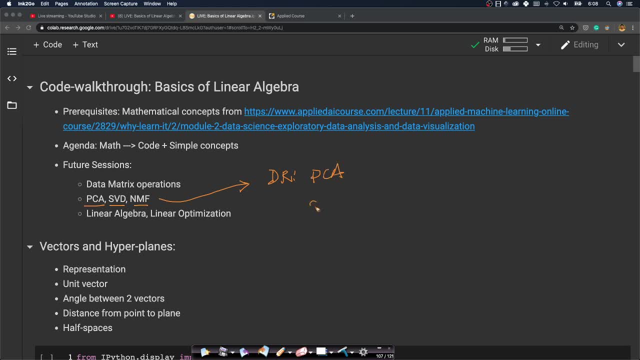 reduction chapter. we covered PCA, right. so SVD and nmf we covered in. we covered in the chapter of recommender systems, right? so there are tons of concepts if you open a standard textbook like Gilbert Strang's textbook. again, this is one of the best books, but again, remember that this book is 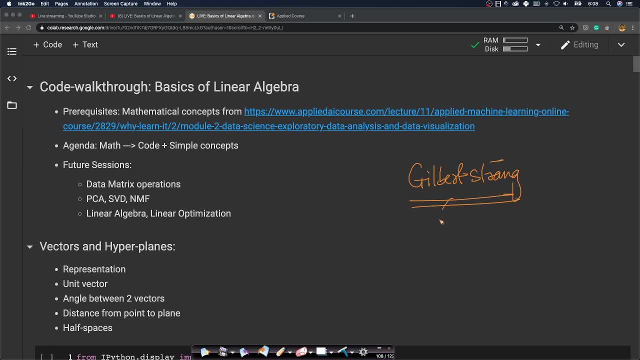 written for applied mathematics students. this book is written keeping in mind two courses, two undergraduate level courses or two courses in general at MIT. right, so it's. it's, this is just two courses, just of linear algebra. so my suggestion is, if you want to be in machine learning or if you want to be in 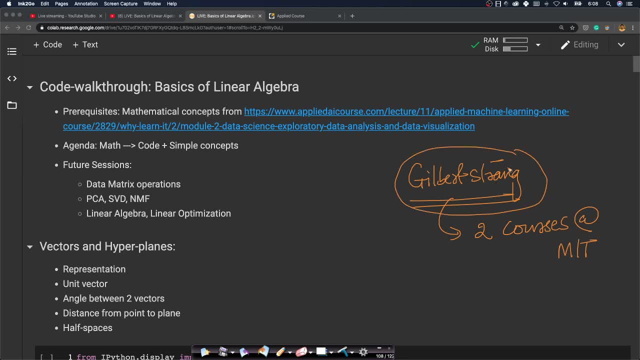 machine learning. again, the problem here is if you start watching just Gilbert Strang's videos and if you just start solving his problems, you will become very good at linear algebra. but remember that linear algebra is just one of the many topics that you need to know to become good. 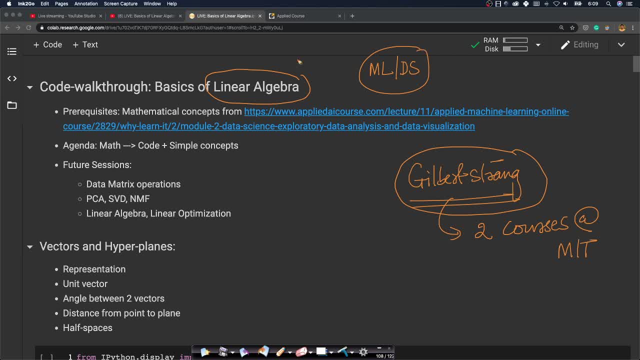 at machine learning and data science. so my suggestion to all of you is this: first learn the basics which are needed in the context of machine learning and data science. once you learn all of that, if time permits, go ahead and read Gilbert Strang, right? so please don't do again a lot of. 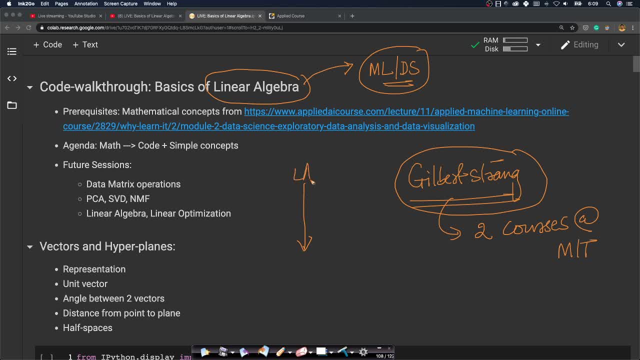 people do this. they do depth first, they just go into linear algebra and they learn everything in linear algebra. this will take you one year- to be honest with you- to finish Gilbert Strang's book comfortably. if you put in one or two hours every day will take you easily one hour to do it. 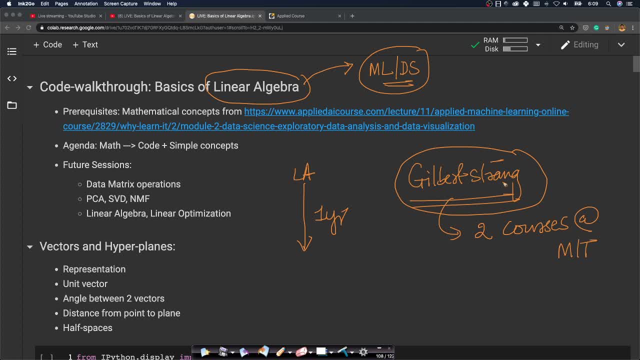 comfortably. if you do assignments, if you do the code part, everything J perfectly right. so my suggestion here is: linear algebra is just one of the many aspects that you need for machine learning, data science, so learn all of that later on. my suggestion always to anybody who is learning a concept is first to do breadth, first learn all the concepts that. 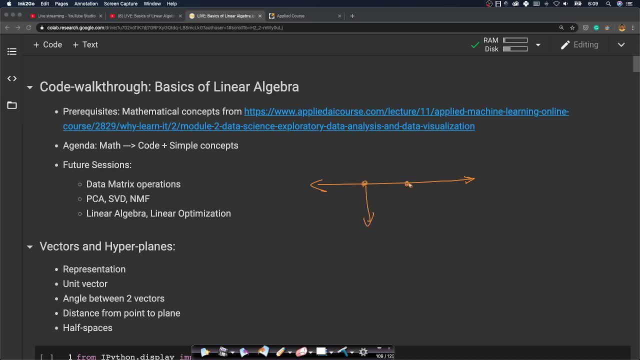 you basic concepts that you need. then for every concept there is a depth go for go. first, get the breadth so that you can start transitioning to machine learning, data science jobs or data science roles, and then there is a whole lifetime to learn depth. right, I'm learning again. 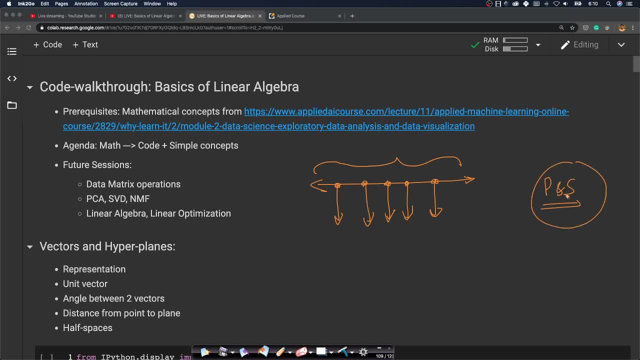 if you think probability and statistics, right, I'm learning some causal inference based models even today. I mean, this is lifelong learning, right? so there is no end to it. okay, so instead of going depth first, I recommend you do breadth first. okay, so what we'll do again? that's also the philosophy. 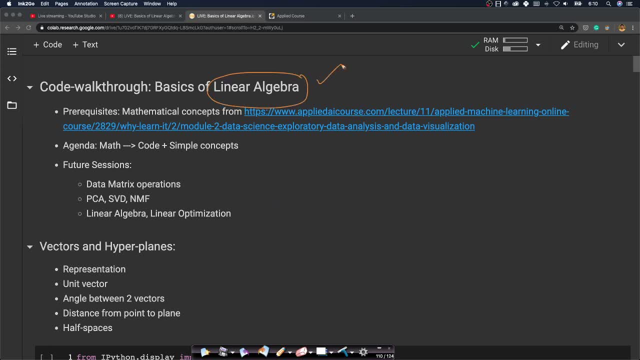 that we have taken in our course videos. first we explain the basics of linear algebra and then we would go into each of these concepts later. okay, so in future live sessions we'll cover a lot of data, all the factorization methods, again, a lot of a lot of linear algebra also has linear regression, if 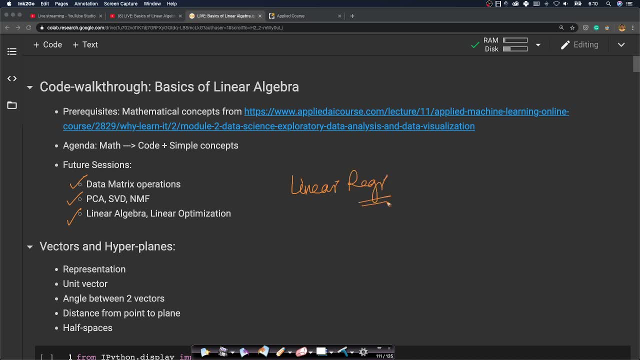 you look at standard linear algebra book, you have linear regression. again, this linear regression can be covered from linear algebra perspective, also from optimization perspective, right? so in our course we cover it both from optimization and linear algebra perspective and we'll cover it in the future sessions. there is also linear optimization, okay, which is related to linear. 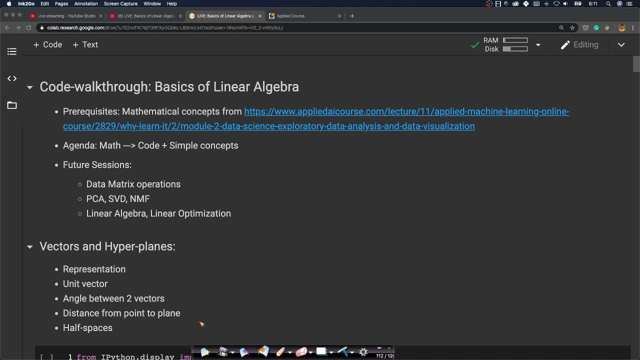 concepts in linear algebra. we'll cover that in future sessions, right, so this lesson is going to be very. that's why I wrote basics of linear algebra. there are many other concepts that we'll cover in future sessions as per our course syllabus. okay, cool, so second: very. 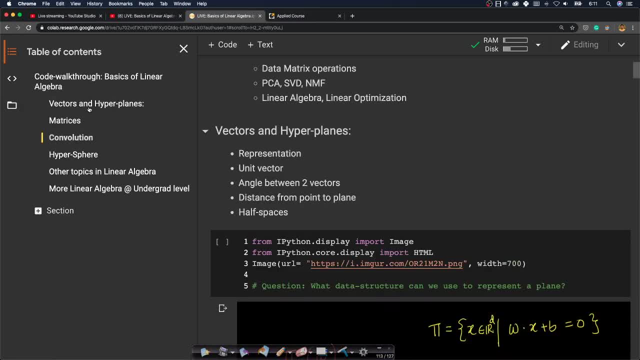 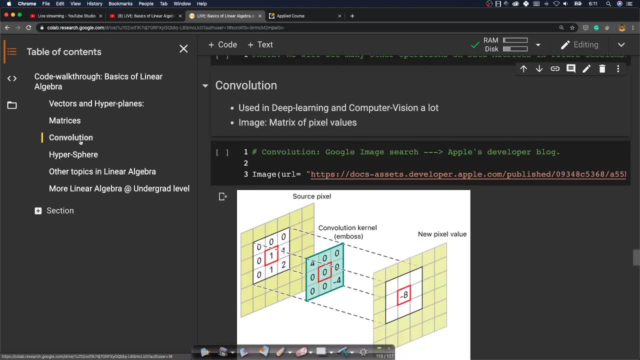 importantly. so we'll let this. this is the agenda that I have today. okay, first we'll go to vectors and hyperplanes. we'll learn a little bit about matrices. we'll take a diversion and I'll explain you about the concept of convolution, because I want to show you applications of matrices to image. 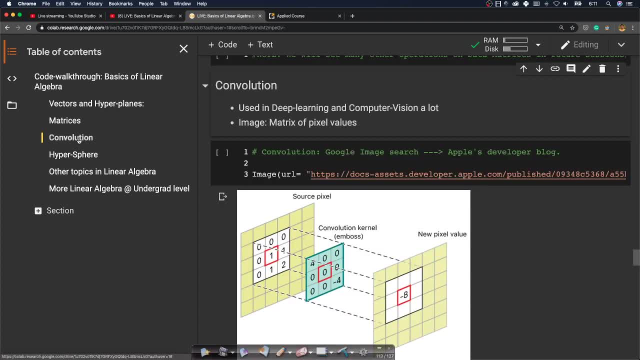 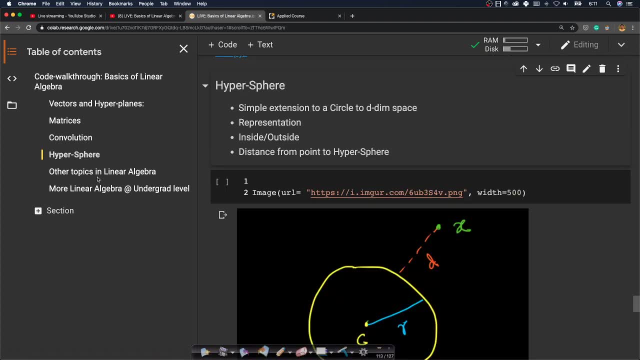 processing and computer vision. just one application, of course. do one whole session on just one or more sessions on computer vision and image processing. I just wanted to do a simple example here. then we'll do some basic hypersphere stuff. I'll also tell you other topics and people who want to learn more undergraduate level linear algebra, we have some. 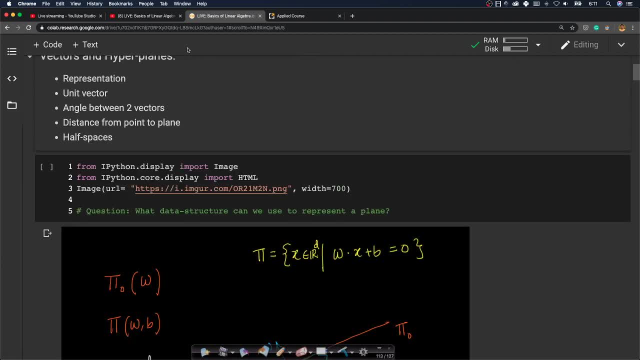 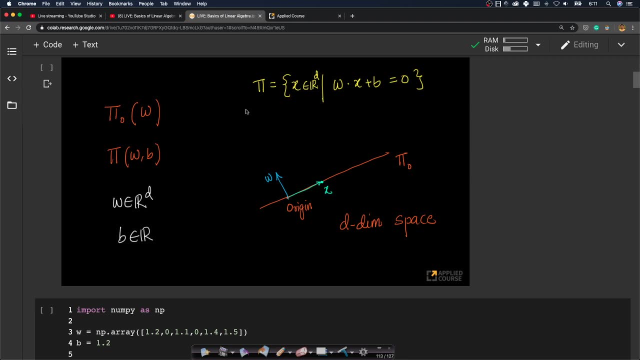 videos for that which are publicly available. I'll share that also. okay, that's the whole agenda. so let's start here. let's start with vectors and hyperplanes. right, so very simple. so imagine again. I'll not be repeating the mathematics that we've already discussed in our course videos. okay, just. 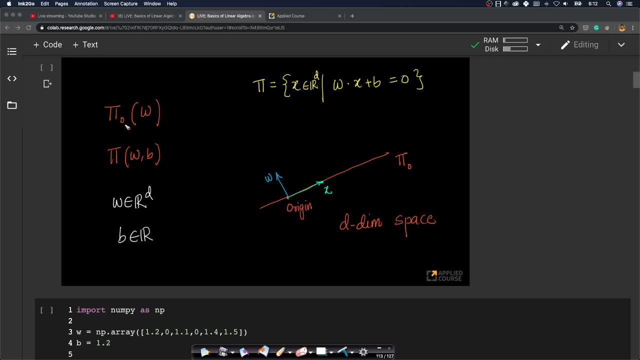 so let me represent this way: pi 0, basically, is a hyper plane that passes through origin. for a hyper plane that passes through origin, you just require the normal to the hyper plane. okay, that's good enough to represent the hyper plane. I'll represent pi like this, without the zero, if it: 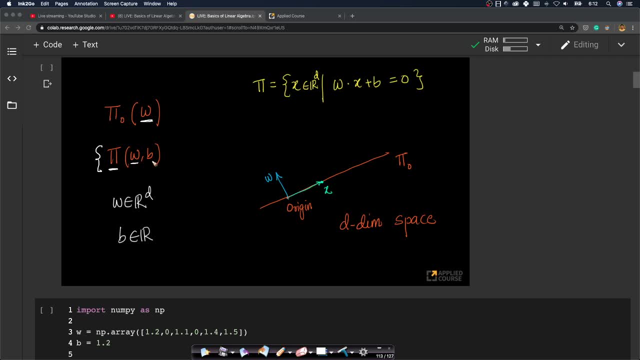 is a hyper plane that doesn't pass through origin. okay, so it requires both W and B. and what is the equation of of the hyper plane? it is very simple: W dot X plus B equals to zero. this is So all the points. so the way you represent is all the points x, such that, oh, I have already. 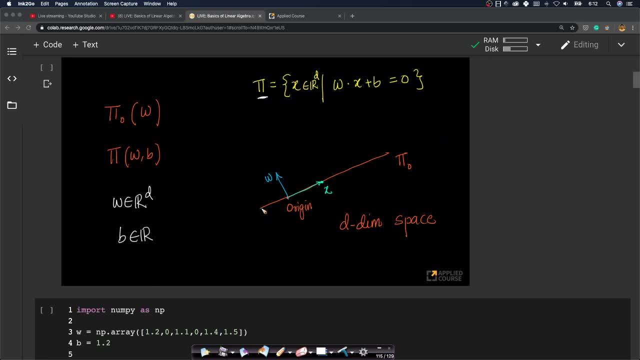 written it here, sorry. so pi is basically or a plane, pi is a set of points or d-dimensional points, such that the dot product with w plus b equals to 0. This is one simple way to define a hyperplane, right? So I will be using this notation and I am assuming that w is a d-dimensional vector. 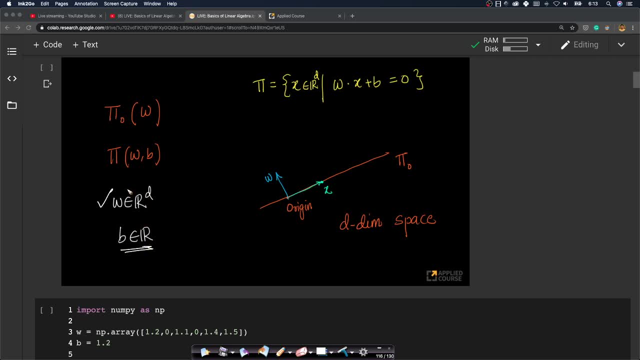 b is a scalar right Again, we have discussed this in the course videos- right, And I am always going to assume a d-dimensional space. So let us take this plane, for example. if you take this plane, again, the formulation is very simple. imagine if I have a plane like this, pi 0, which is passing through origin. 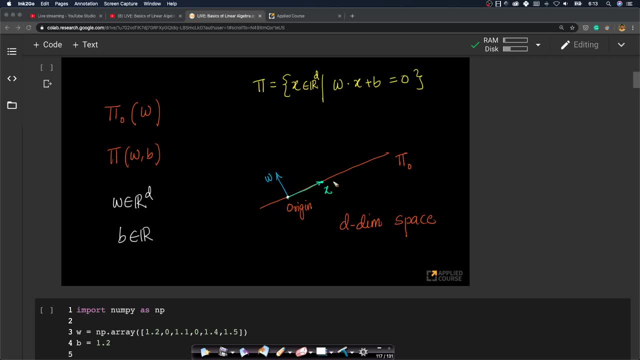 and I have my w here again passing through origin- any point x on this plane- again, I am not, I am just using a 2D representation here, but this is a d-dimensional space, right? So any point x here will be a d-dimensional space. 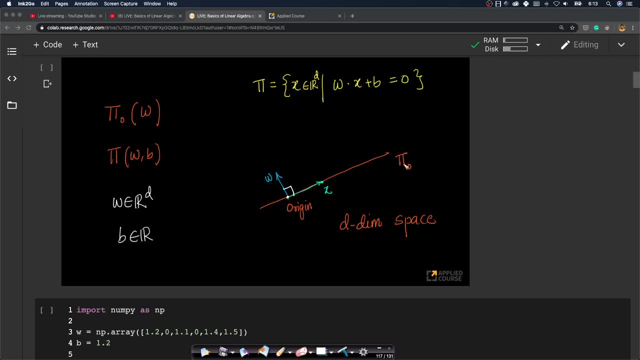 Any point y here will be normal or perpendicular to w. So for pi 0 it is w transpose x equals to 0, or you can also write this as it is a dot product of w and x. you can also write it as w transpose x, just a different notation. 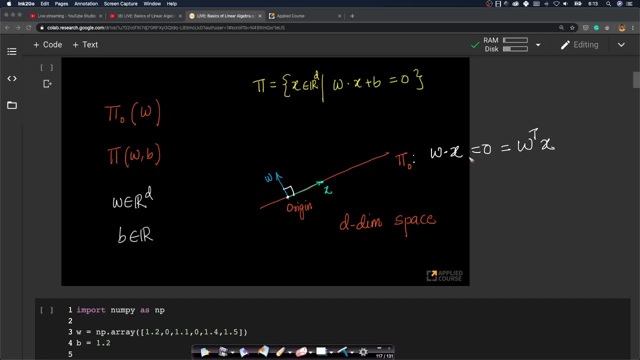 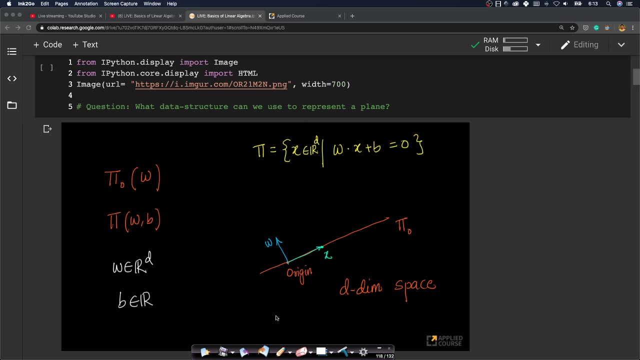 of writing it right. So when I say dot, it means dot, product right, very simple stuff, nothing fancy. Now I have a question here for you. So if you were to represent again, given this basic background, what is a good data structure? 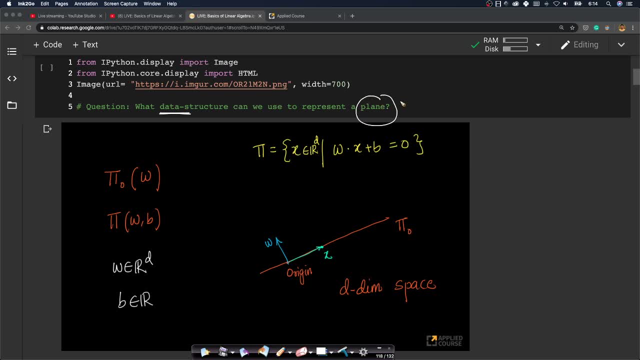 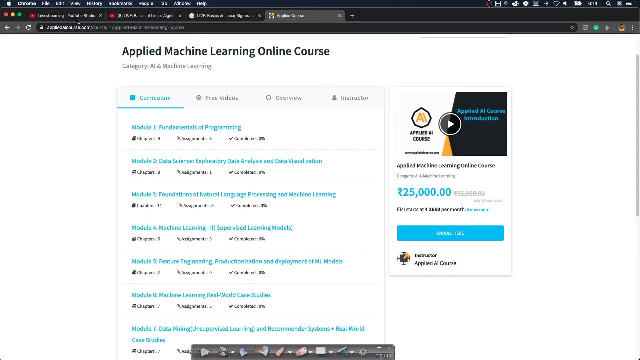 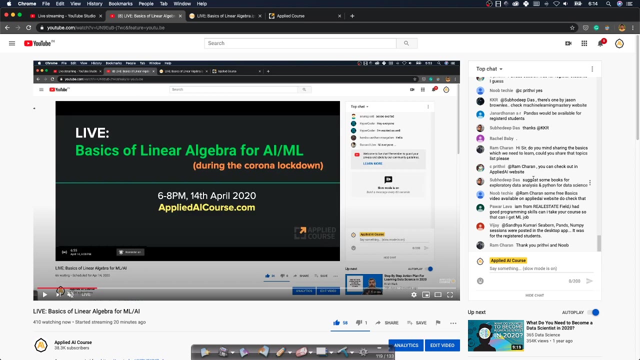 you can use to represent. How do you represent a plane? I would like to listen to your thoughts Again. I am seeing the chat window in the- sorry, I am also seeing the chat window here. So what do you recommend? What do you think is a good data structure to represent? 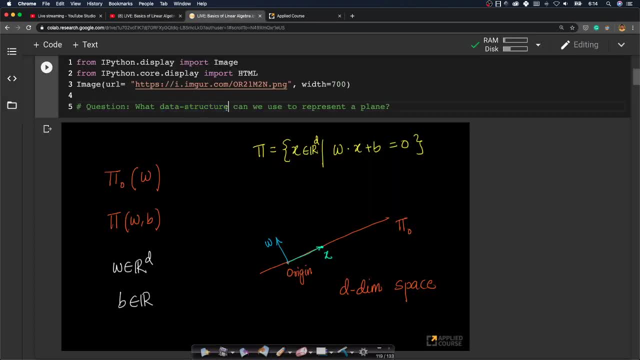 So the question is simple, right, What is a good data structure? Again, we have studied data structures in Python, right, basic data structures. What do you think is a good data structure to represent a plane? That is the idea here, right? 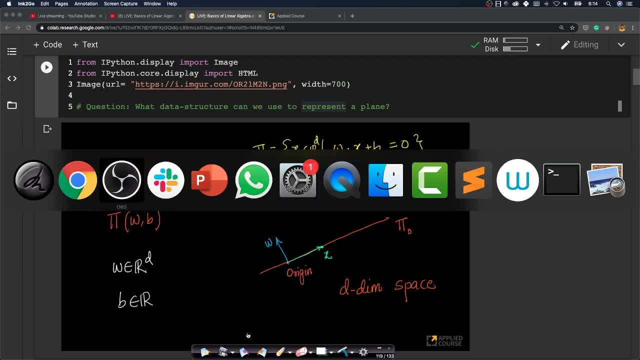 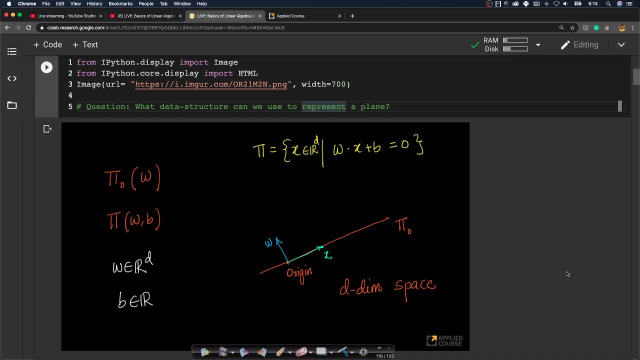 So what do you think are good ways of doing it? Let me just check the internet speed. I hope there are no hiccups. yeah, no hiccups, okay, So I am looking at the chat window on a different computer. 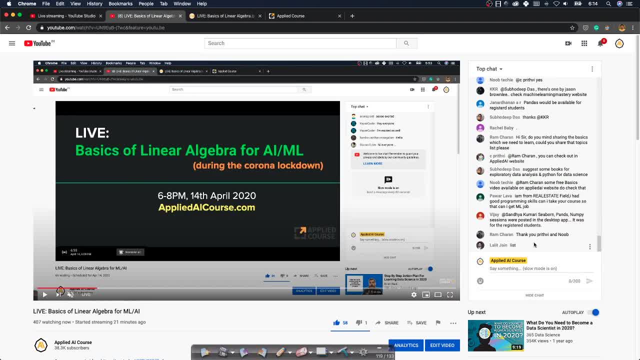 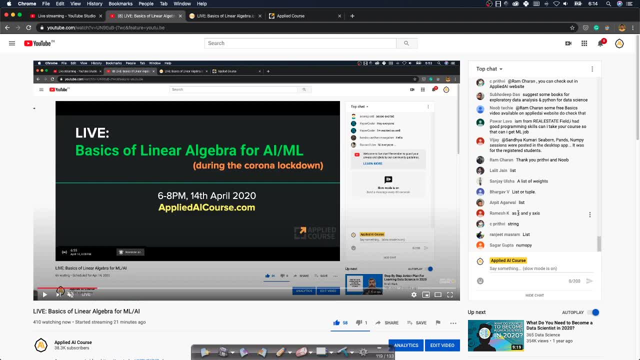 So if anybody has ideas, do let me know. Somebody says list- okay, a list of weights list, or tuple list: okay, as x and y axis. Again, guys, this is not a 2D plane, this is a hyper plane. numpy array, tuple- okay, look. 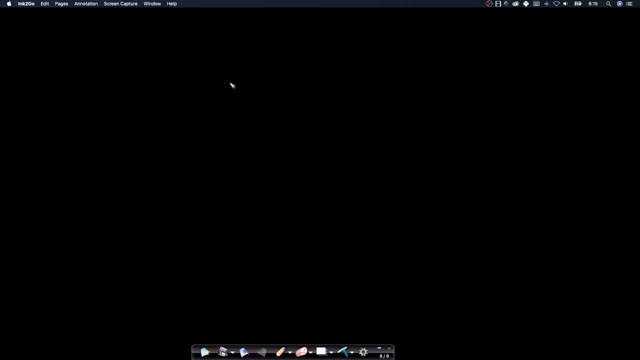 at this. Okay, These are good ideas, So let us go down, okay. So what do you need To represent a general pi? okay, which may or may not be passing through origin? you need two things: You need w, which is a d-dimensional vector, and you need a scalar right. 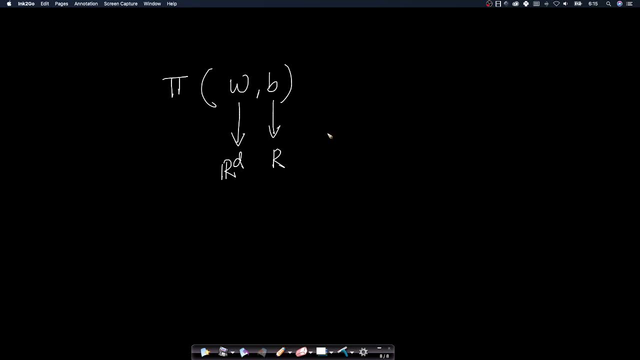 How do you represent this? Again, when you choose a data structure, very importantly, you should also ask: what operations do you perform on it? The choice of data structure just should not be based on how you store the data. It should also be on operations. 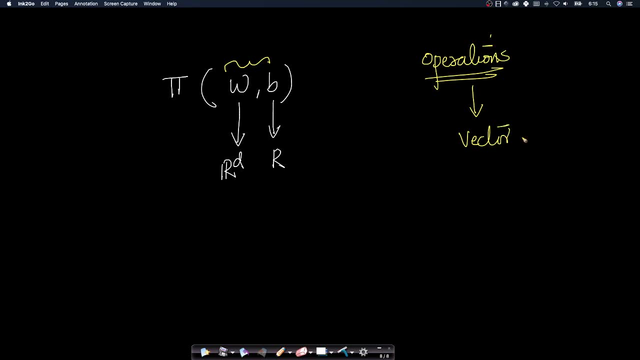 So you will mostly do vector operations, right, like dot products, all of that stuff, So vector operations. You will also be doing a bunch of matrix operations, right. So these are the typical things that you will perform. So, given that the operations that we perform are vector addition, vector dot product multiplying, 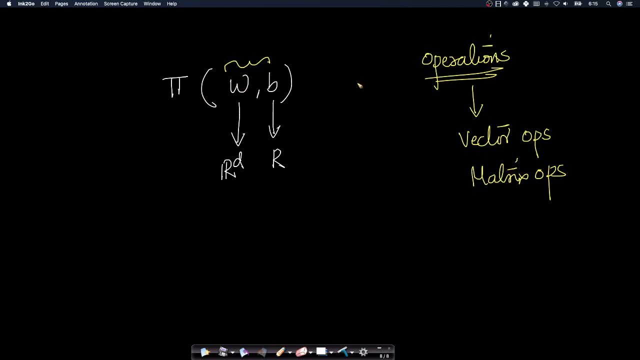 this with a matrix, all of those things. what do you think is a good thing? So I am just looking it down. So people say: tuple dict. okay, let us take this down right. So let us understand this. So some of you are suggesting list. okay, 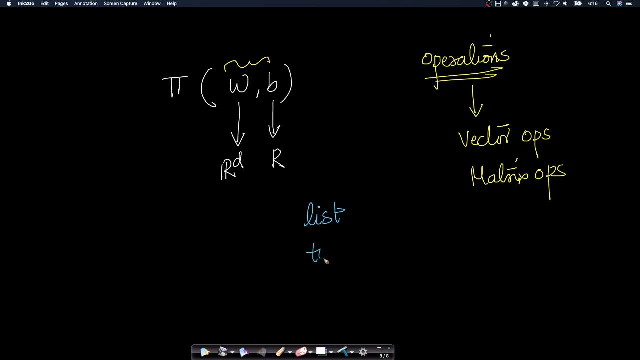 Most of you are suggesting list or tuple. okay, So, tuple. So how do you store the tuple? okay, So would you store w1, w2, again, let us assume w1 is the first component of this. Let us assume w is w1, w2, so on wd, okay, just for simplicity. 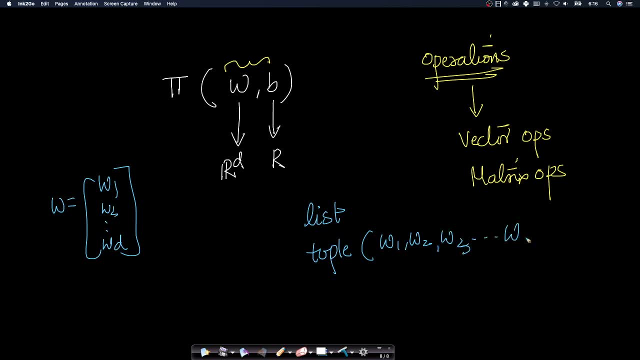 So would you store it as wd, so on, so forth. sorry, w3, wd, comma b. This is one way to store it. But are tuples good? Are tuples good with vector operations? Are tuples optimal for matrix operations? 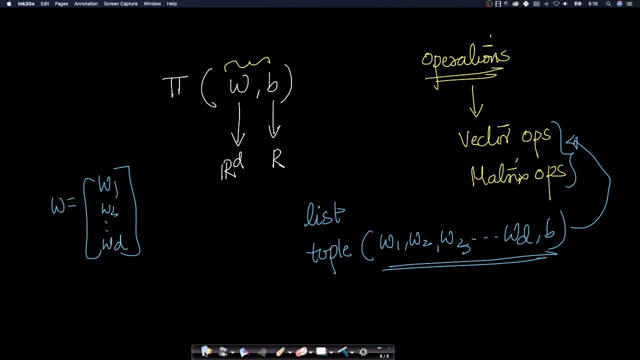 Right, So how do you do it? Okay, So, if you think again, some of you are suggesting, very nicely, a good thing is actually numpy. What is the purpose of numpy? Numpy was designed for numerical operations on matrices and vectors. 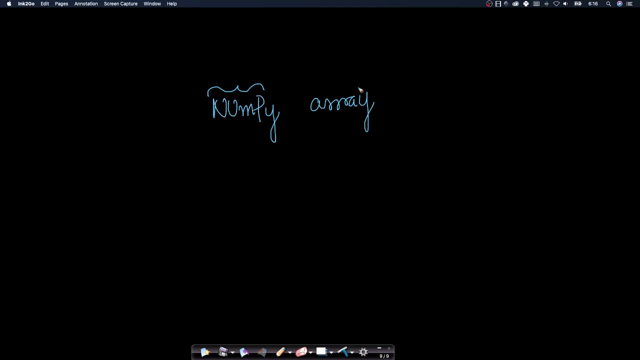 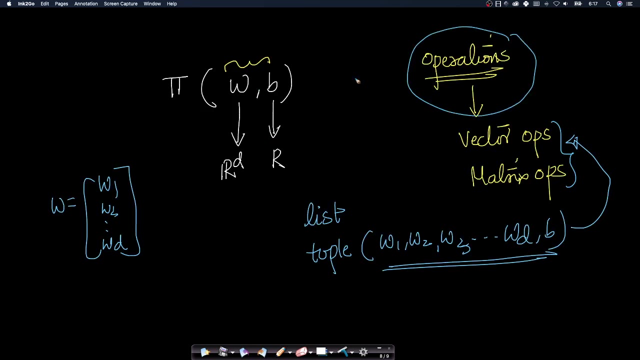 So numpy array is a very good thing, because numpy array is designed with the purpose of these operations. Right Numpy array is designed with this. So if I represent w as a numpy array, not an n-dimensional array, just a one-dimensional, 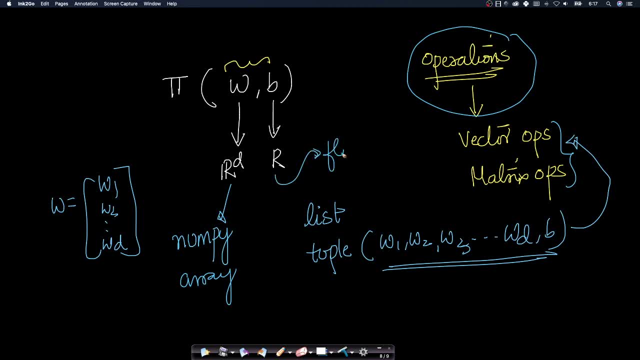 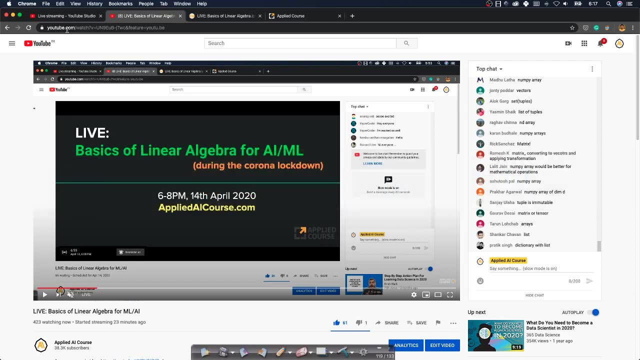 array right. I can represent this as just one float right. So the idea here is, as many of you rightly pointed, it is a very simple thing. It is a very simple concept, right? Nothing fancy here. Again, it should always depend on operations. 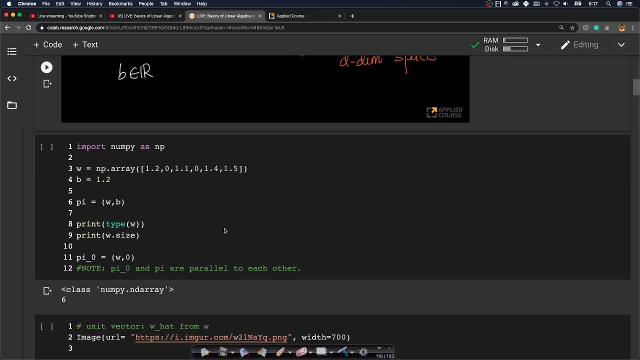 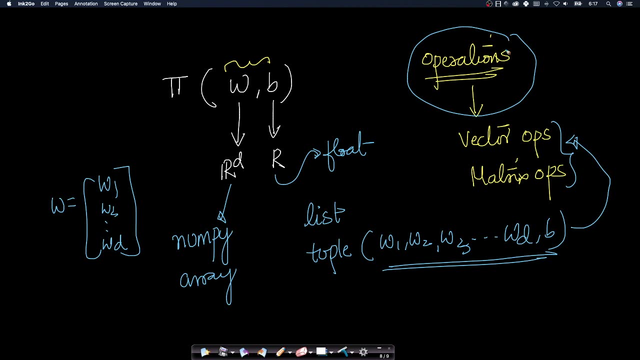 If you represent it with a list or a tuple, one of the challenges you have is access to libraries. Again, we can always represent it with list or tuple. But then the operations that you perform: you have to write code for everything. 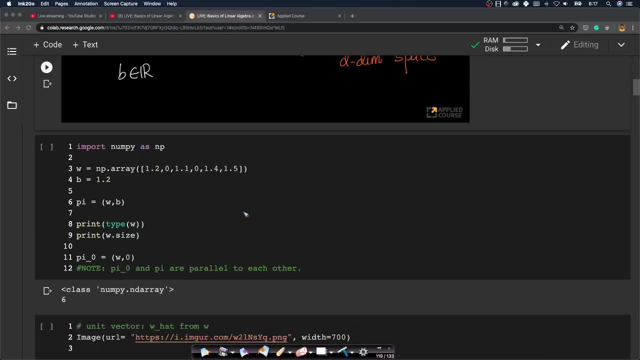 Instead of that, if you do use a numpy array, there is a lot of functionality that's readily available for you, okay? So look at how I'm just representing it right? So my w is this: okay, np array. So I pass a list here. 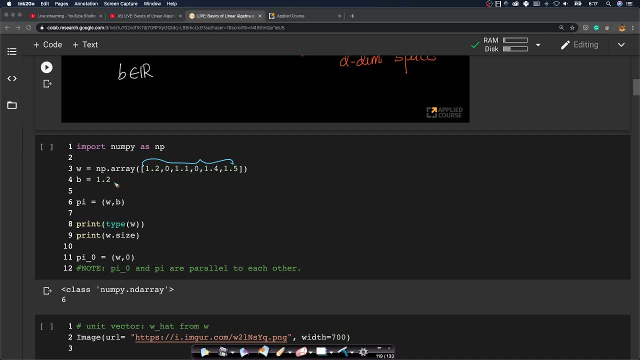 So the list is converted to an array. Very simple, Nothing fancy. B is represented just as a float. Cool, I've just taken some numbers here. Now my pipe plane can be represented as a tuple. So what have I done here? 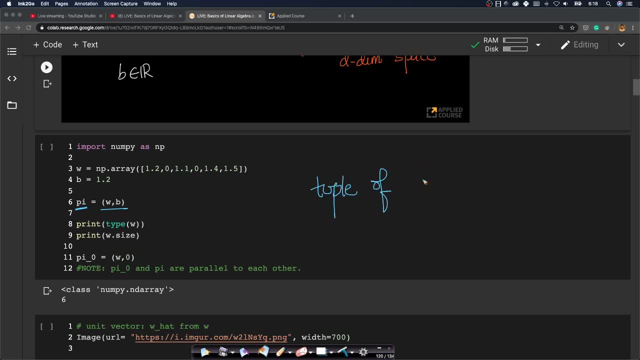 I've created a tuple of two elements. okay, So I've created a tuple of two elements. The first element is a numpy array. is a numpy array. The second element is just a simple float. okay, The first element represents w. the second element represents b. 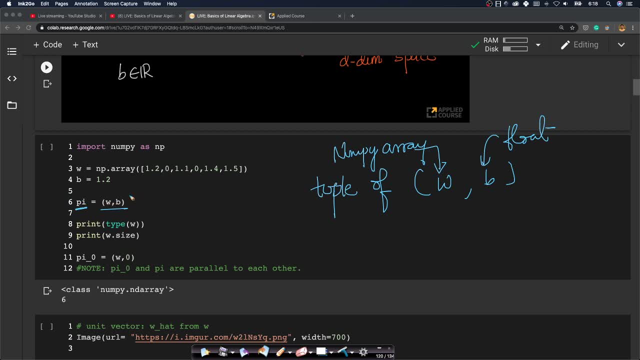 So this is one way, because I need both w and b in many contexts, right? So very simple way Again. see, I'm just creating a numpy nd array, But if I want to just store pi zero, what is pi zero? 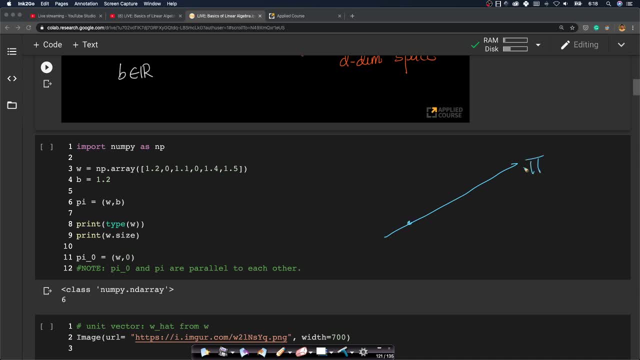 Imagine if my plane passes through origin. if this is my plane, my plane passes through origin. right then I don't require the b term, Because the equation of my plane now is w. transpose x equals to zero, right. So to represent that I just need w. 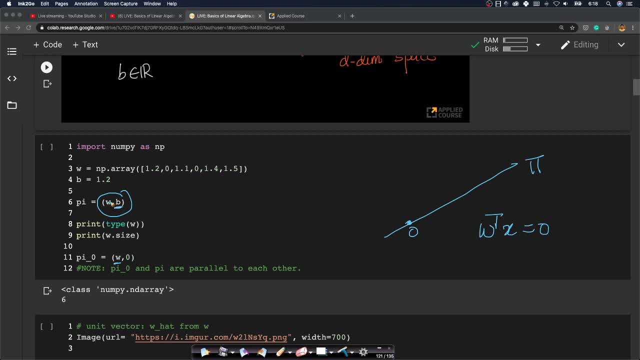 In such a case, what am I using here? I'm using a tuple rate. Look at this. I'm using a tuple where the first element is a numpy array, The second element here is a float. Okay, I can also use the same representation with zero, or I can just say for pi, zero. I don't. 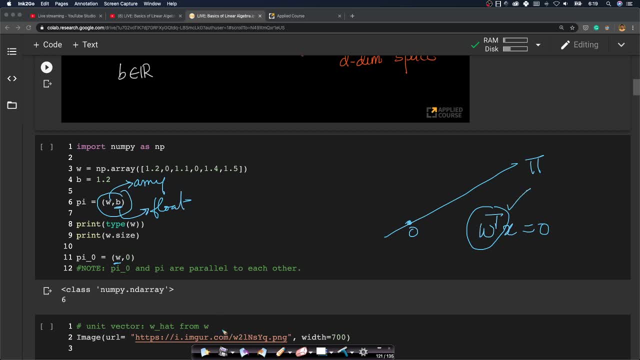 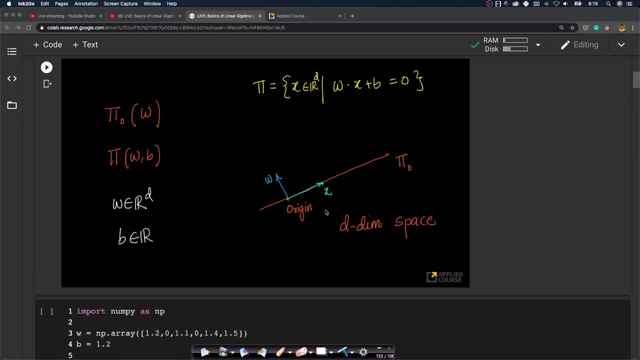 require b. So I'll just represent it using just one numpy array. Very simple. right Now, one interesting fact. okay, So imagine if I have two planes like this. okay, Just a quick question. okay, So just as observation, I should say: okay, imagine if I have two planes pi zero, which? 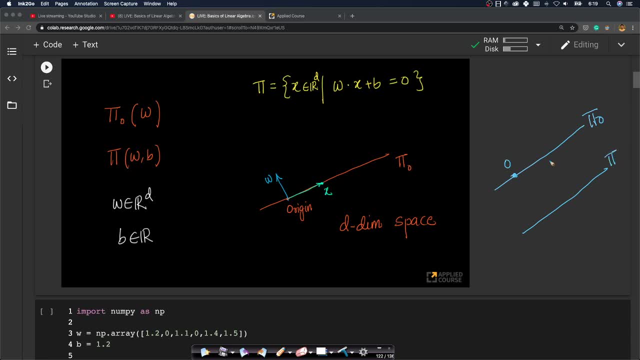 is passing through origin and this is pi, If these two planes are parallel to each other. again, I'm just drawing 2D diagrams, but you can imagine them to be 3D planes. Beyond 3D nobody can imagine, right. 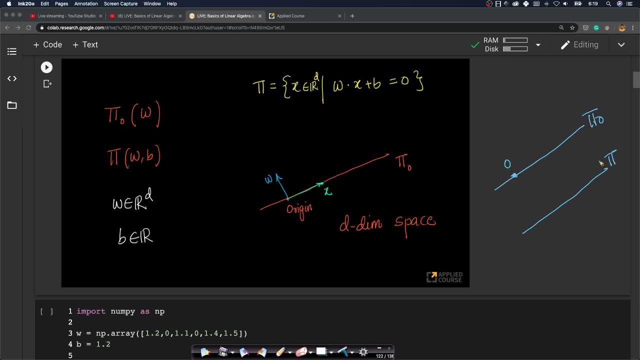 So imagine this: So this is one plane, this is one plane, right? Both these planes are. how do you say both these planes are parallel to each other If this plane is represented just with w and if this plane is represented using w and. 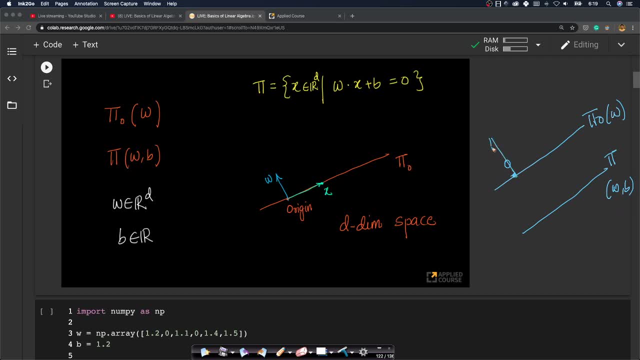 b same w, So w is normal to this plane, w is also normal to this plane. Okay, So if two planes have the same normal, then they both are parallel to each other. Simple, very simple concept. I think fancy here, right. 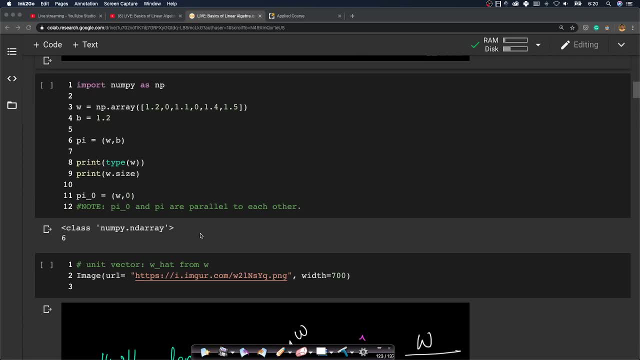 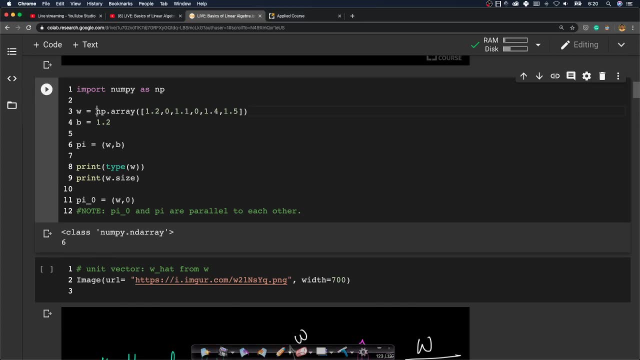 Okay, cool. So just wanted to show you how to represent. Now let's go into some simple stuff. Okay, we'll do simple operations Now. taken our, if you look at our w here, our w is not a unit vector. 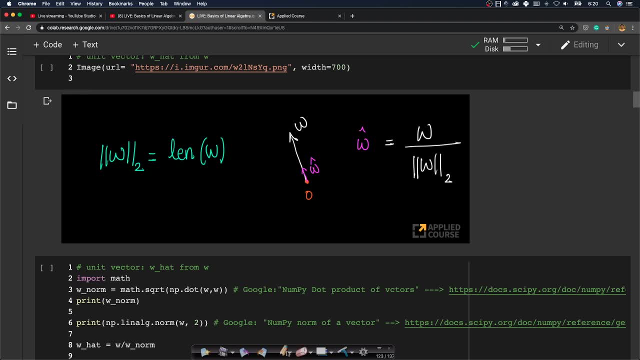 Now, what is a unit vector? Very simple concept that we discussed in the course videos also. Suppose: imagine: take this vector w passing through origin, Take any vector, okay, this is basically a vector w, right. So this vector w can have any length. 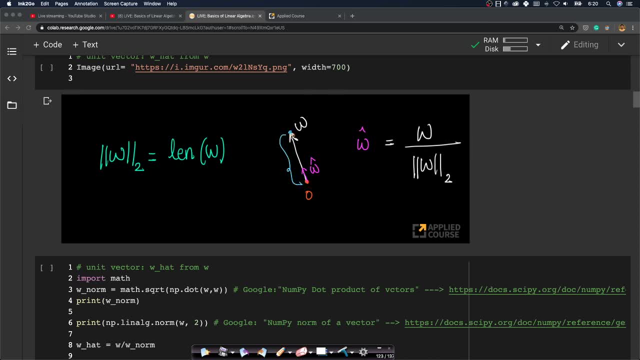 So this whole thing, this length, the distance from here to this, this is called the length of w right. So how do you get the length of w? You take the L2 norm of w right or you take the Euclidean distance between this point. 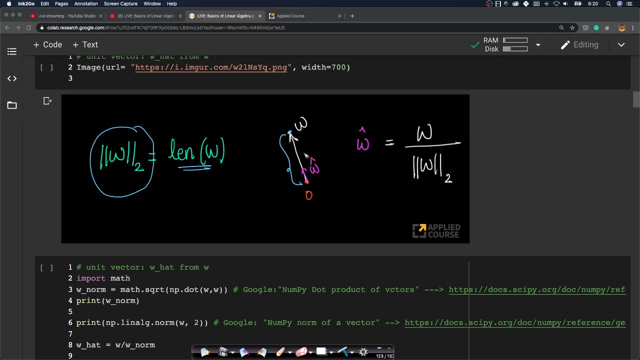 and this point: Okay, that's also written as the L2 norm of w right. we have discussed how to compute this. Now, what I want, so, given this w, if I want to get a w hat, which is nothing but the w. 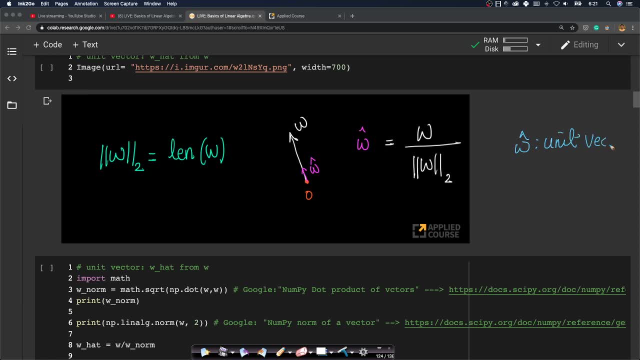 hat is a unit vector, is a unit vector in the same direction as w. okay, it is a unit vector in the same direction, in the same direction as w, If I want to get that. so look at this, look at our previous definition. 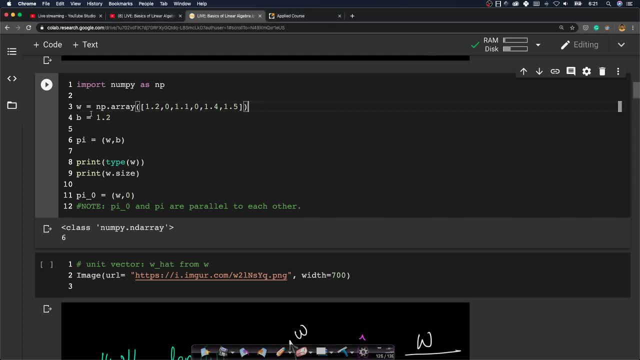 I did not, so I just created an umpire array right, so I did not ensure that it's it's. it's is 1. I did not ensure that anywhere. I did not ensure that anywhere. very simply put, 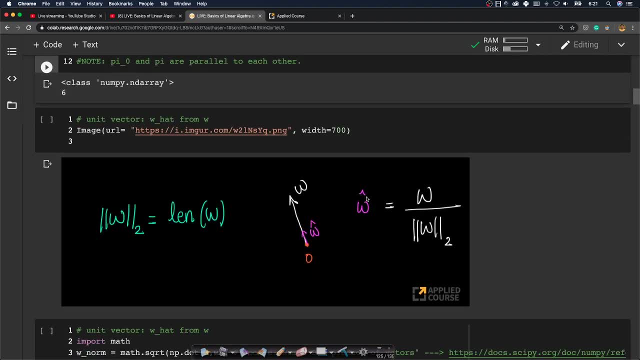 Now, since I did not ensure that, if I want to create this w hat, which is nothing but a unit vector in the same direction as w. So what is a unit vector? Its length should be 1.. The length of a unit vector is equals to 1.. That is why it is called unit, because 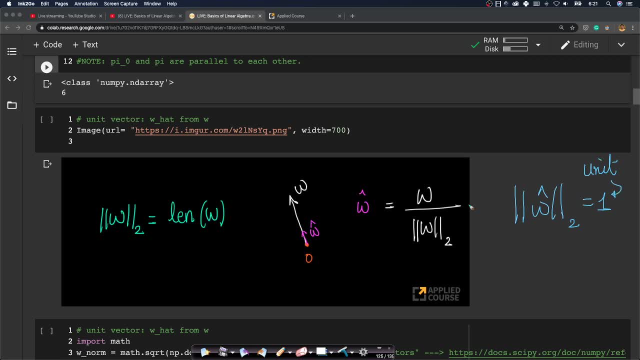 unit in math mostly means 1 in most of mathematics. So the idea here is: how do you compute that? It is very simple. So given any vector w if you want the unit vector in that direction. again, we discussed this in the course videos. that is why I am not going into the mathematical. 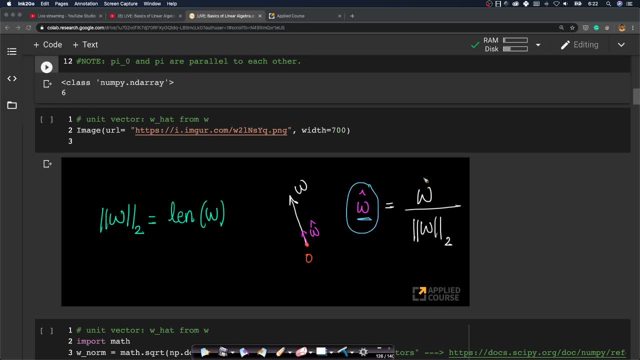 proofs. I wanted to show you the code walkthroughs more than math, So I have taken screenshots which are very similar to the course videos, and I am trying to explain the math here So that you can translate math to code, Because once you do that, you can translate any math. 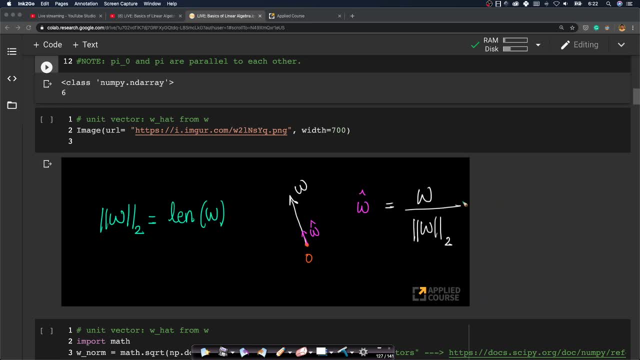 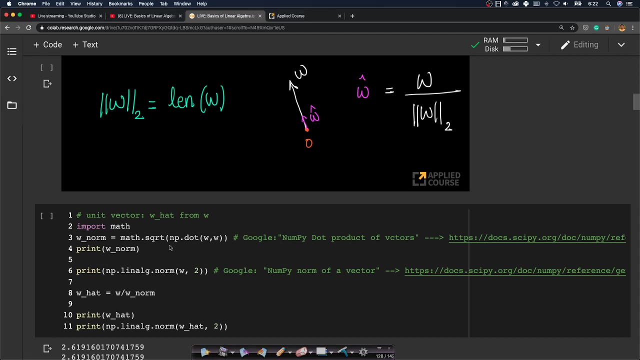 to code. One of the most important objectives of this code walkthroughs is to translate concepts to code. So you have w hat equals to w by norm w. Basically, this is the equation. Now how do we implement this in code? It should not be very hard. It is actually fairly simple, So let me implement. 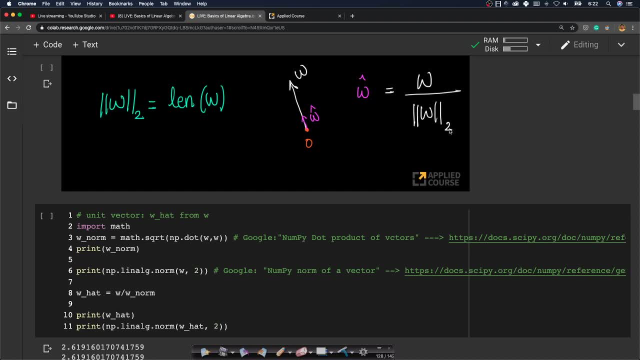 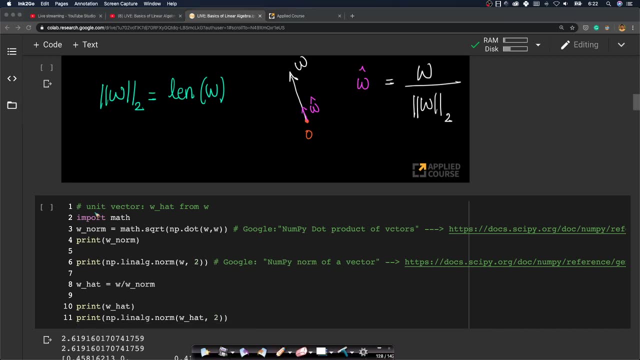 it myself from first principles using this definition. I will also implement it using an inbuilt function. Let me show you both the stuff. So let us go step by step first. So I am importing math here. Nothing fancy, nothing complicated here. So first I am computing. 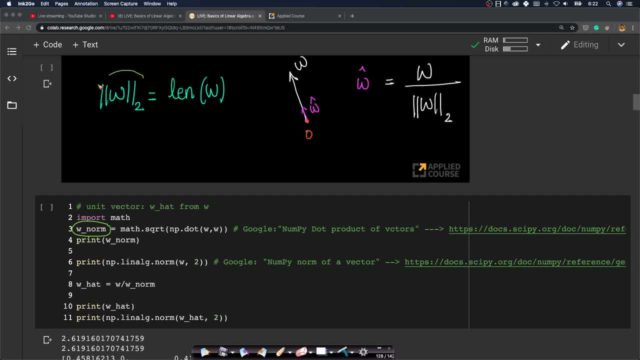 the norm of w. I am just computing this norm, w which some people also called as the length of w. We use the norm terminology because in mathematics or in machine learning we have L2 norm, We have lot of norms. You have L2 norm, We have L1 norm, We have Frobenius norm. 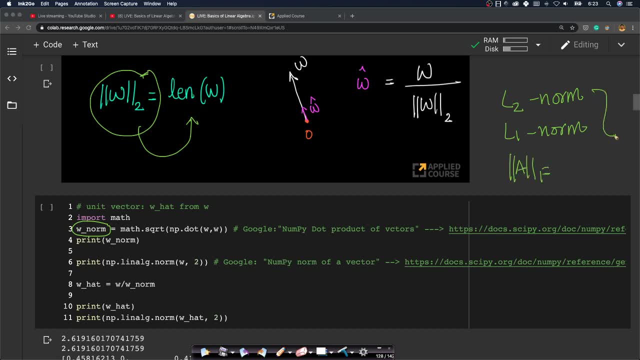 So there is something called Frobenius norm of matrices. Again, these are concepts that we will encounter later in our course and we will revisit these concepts. I prefer to use the norm terminology rather than the length terminology because it is more widely used in mathematics. 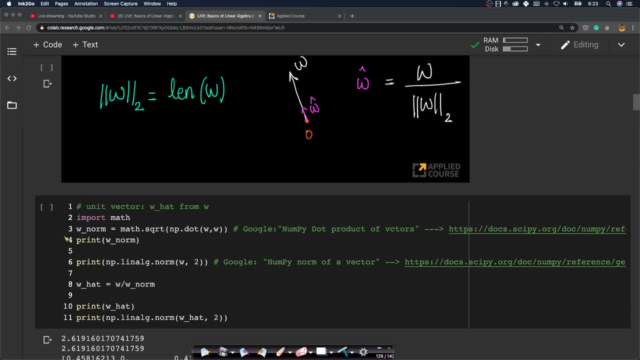 So the concept is very simple, So let us translate it into code. So what is W norm? W norm is you take. say what is the definition of W norm? You take W, do the dot product between W and W, do the dot product which is equal to W, transpose W and take the square root of it. 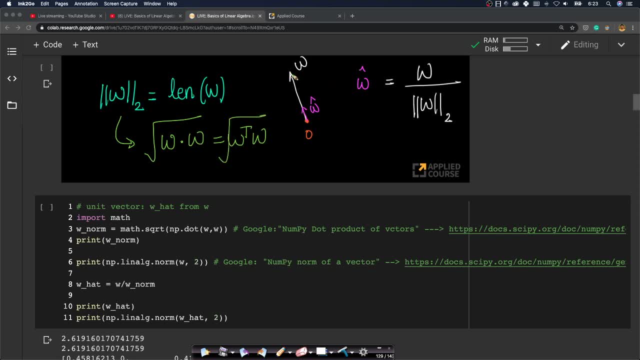 This is the mathematical definition. This is basically what is the distance between this point and this point? W minus 0, or this is origin. So subtract everything to 0.. So you are just computing the distance from this point to origin. And how do you do it? 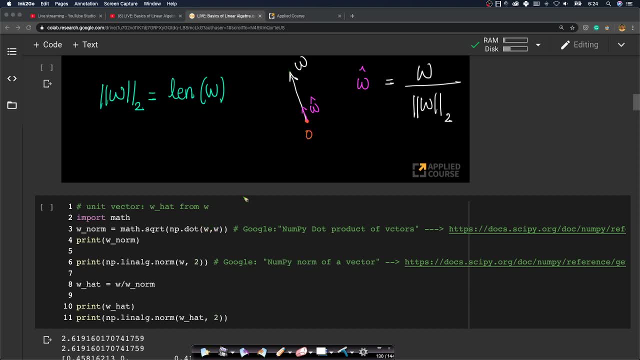 Again, you can do it using, of course, you can implement the dot product also. Look at this. So what is this? As I just showed you here, this is this: Now you can implement this dot product or this W transpose W yourself, also using for loops, But it is already available in NumPy. 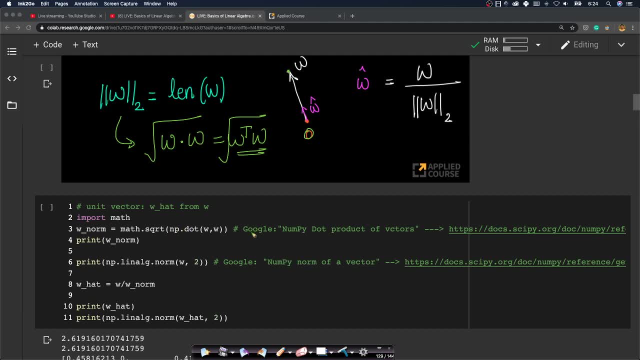 If you do not know what function to use, just google. Again, I am trying to simulate. what if I am a beginner? I know the concepts, I know the mathematical concepts. How do I translate it into code? Suppose, if I do not know what? 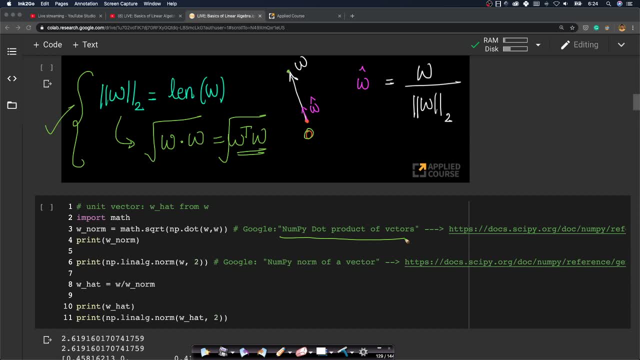 function gives me dot product. I just say NumPy dot product of vectors. I get some documentation. The documentation is for dot, npdot, So given two vectors, it will do the dot product. Again, dot is a very general purpose thing. You can read the documentation here. I will share this. 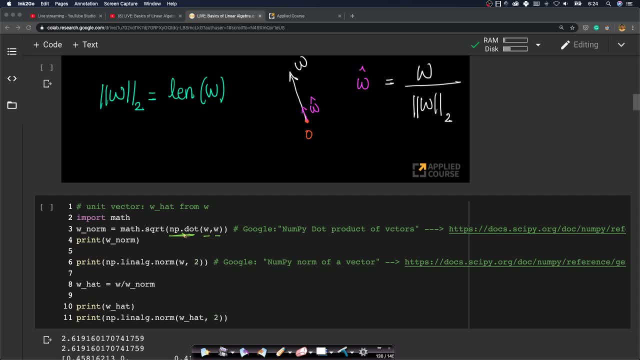 document with you, But if I do not know what function, again, it is almost impossible for anyone to remember every function that is there in numpy right. if i were a beginner, i would just simply google search, find the right function, read the documentation, as we have done in previous live. 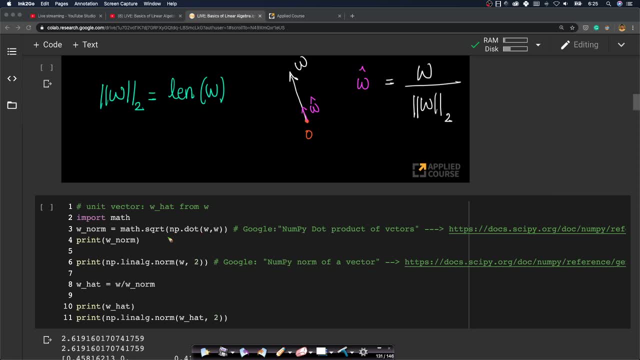 sessions and i will just do here. so what do i get? i get that i. so what am i getting here with this? i'm getting this part: w dot, w dot w or w transpose w. now, on top of that, i have to do square root. we know math dot square root. so if you print this, if you print this, what i'm getting here is this: 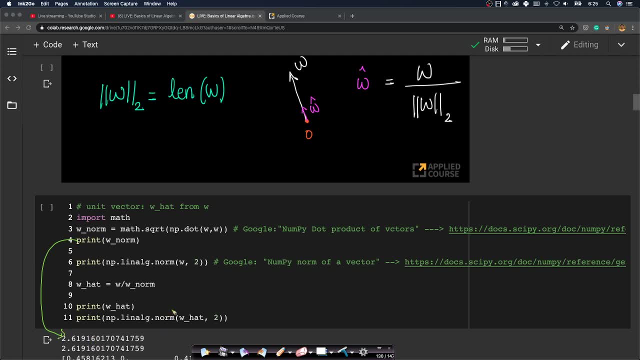 2.6191. blah, blah, blah. cool. now i have a question, which is: is there some other function? because numpy, the whole of numpy itself, numpy and scipy are designed for numeric and scientific computations, and in most of scientific and numeric computations, matrices and vectors are extremely common. 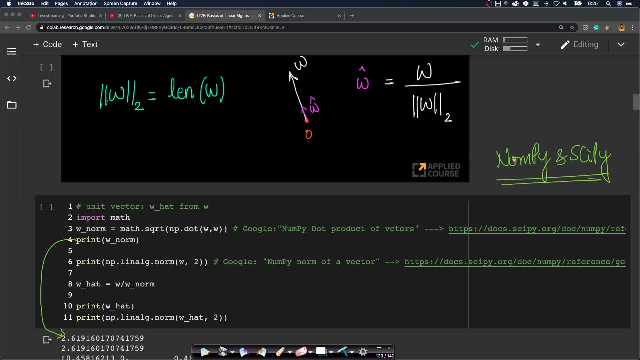 right, any part of mathematics, right. so i i had this question: is there, is there some inbuilt function to compute the norm directly? why should i worry about it then i i just googled this. imagine if i were a beginner. okay, i would just say numpy norm. 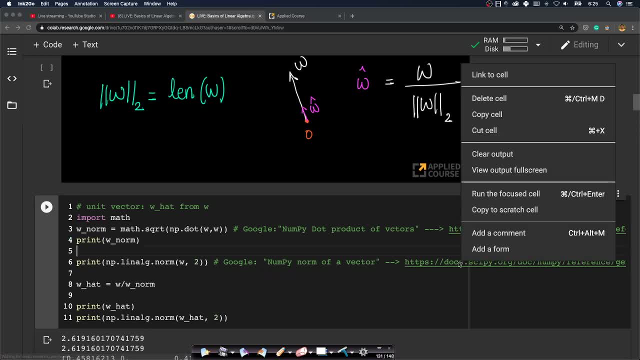 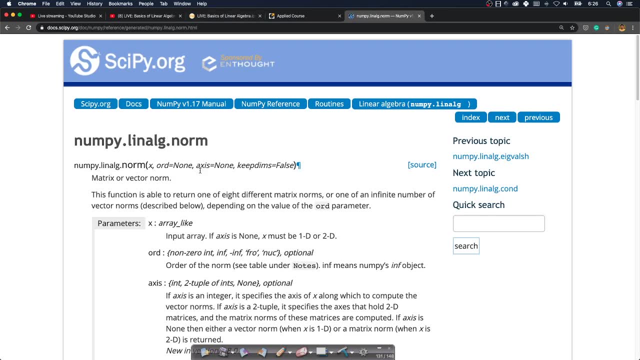 of a vector, right? so i just get this documentation. sorry, so let me just copy this. this is basically okay. again, you can just google search it and you'll see all of this, right? so i read the documentation. you should always read the documentation. it says: okay, x is an array. 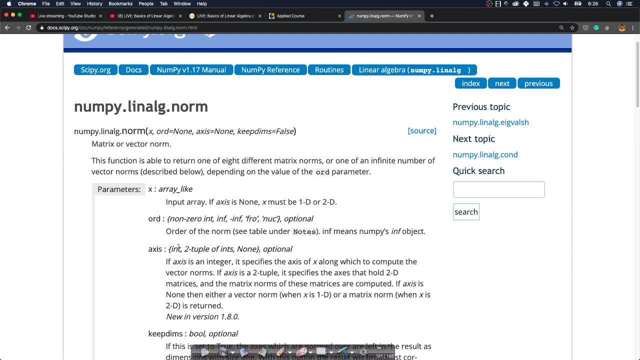 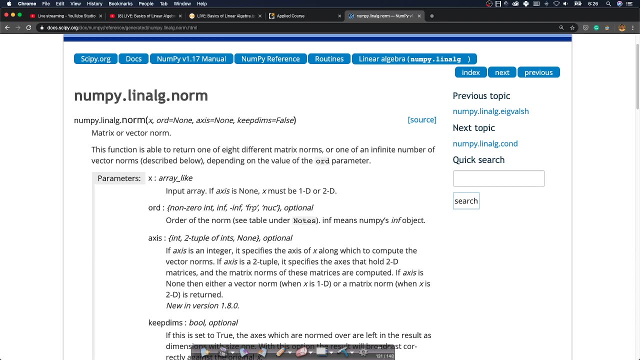 like object. okay, the odd. odd basically means okay, order of the norm. now, what all are possible? non-zero, integer, infinity minus infinity fro nu c. there are lot of norms, as i told you, right, there is something called as infinite norm. okay, there is something called as frobenius norm, right? so there are lots. 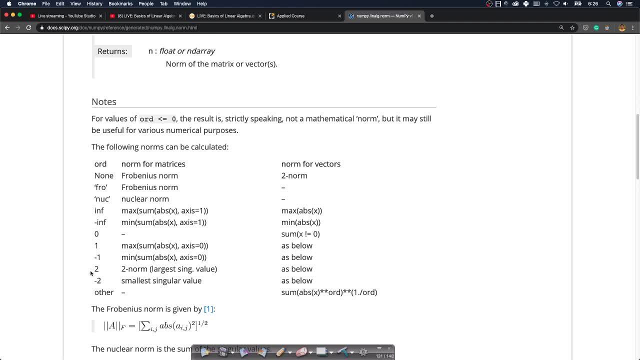 of norms. so if you just go down, it says, okay, what is this? so if i use two here, it says okay, two norm. what we want is a two norm, right, or also called as a l2 norm. again, here is the definition of lots of types of norms that you can compute right. so if you just so, two norm is 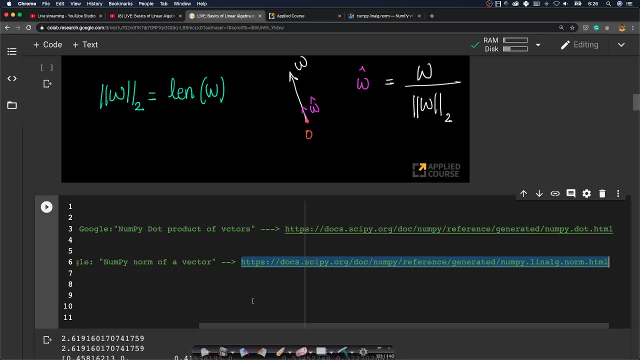 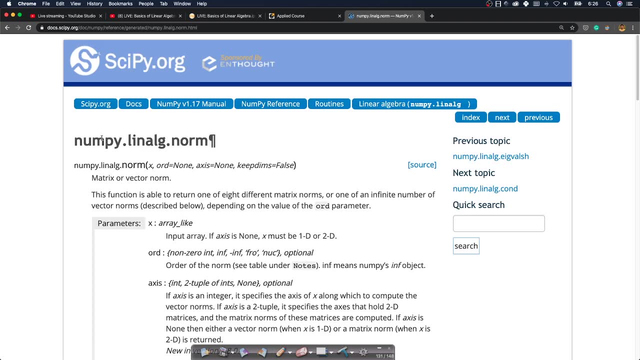 what we are looking for. so what do i do now? i just say, okay, there is some inbuilt function, let's just use it. so what is? where is this function? this function is in numpy module. within numpy module, there is a sub module called linear algebra. within that there is: 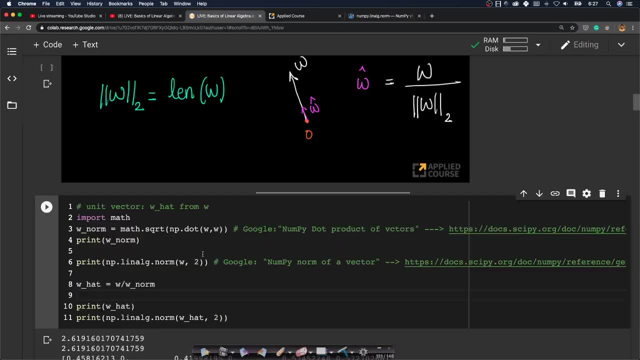 a function called norm. right, this is what we have to use. so let's go back and i just say np. dot linear algebra, dot norm w comma 2, because i want two norm. i just printed this. now what do i get? when i want two norm again, there are two ways of implementing it. one: 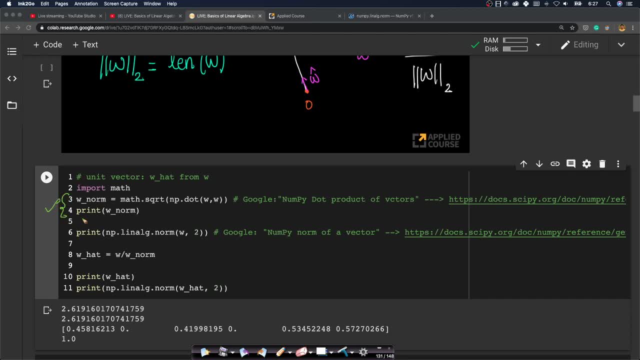 we wrote it from the formula here. what did we do? we wrote it from the formula that norm w is nothing but square root of w dot w. we wrote it using the formula here. we wrote it using the inbuilt function, right? i just wanted to verify if both of them are same. yes, they. 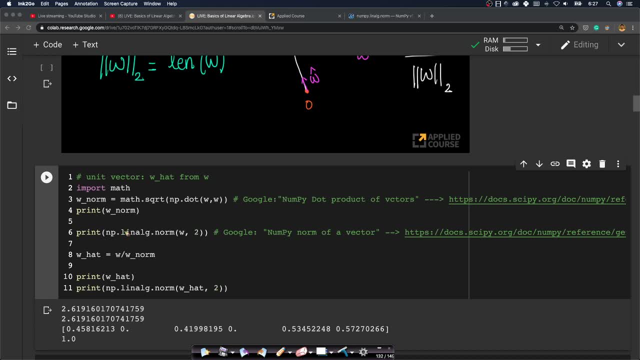 both look exactly the same cool. so in the future i am assuming that the numpy guys have implemented it much better within within c, c plus, plus again. whenever there is an inbuilt function, it's always a good option. in one of our previous live sessions we have shown where we implemented code ourselves complex. 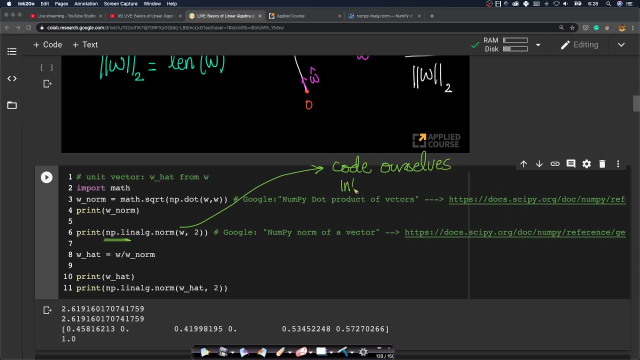 code ourselves and we use the inbuilt implementation. and we and we saw that inbuilt implementation, especially with respect to numpy, scipy, can be extremely optimal. right again, here also, we are not writing the code from scratch, we are using some inbuilt functionality which can be fairly fast and fairly quick. right, so the idea here is this: okay, now we have. 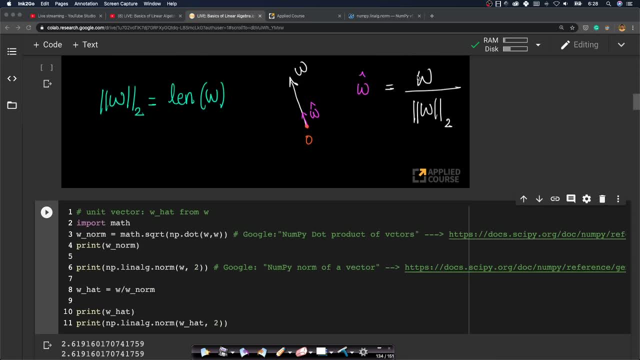 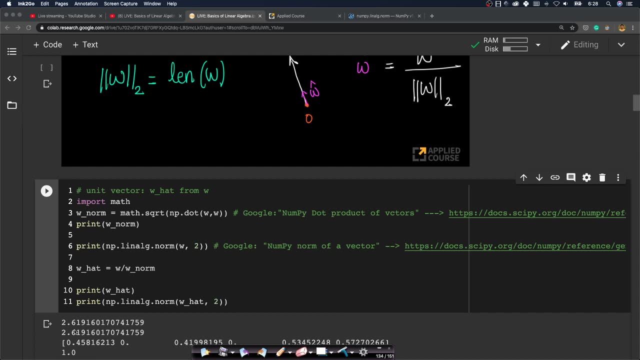 generated the numpy sistemas. okay, if we want w hat, what is the formula for w hat? we know that w hat is nothing but w by norm. w norm, w is just a real value. norm w a. w norm is just a is just a real value. so what do i do? w hat is w by norm, that's it. so i get this. 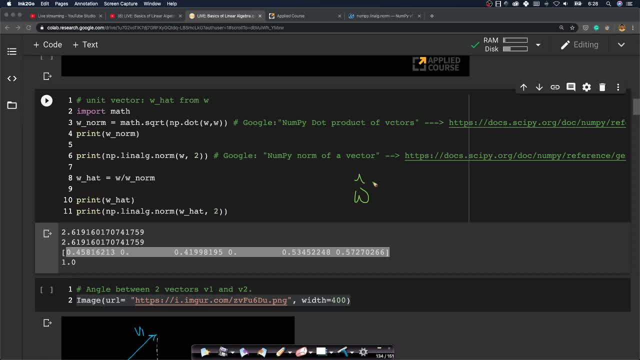 now i get this. now, what is the property of a unit vector, the unit vectors? the l2 norm should be equal to one. let's just verify that. okay, so i printed the w hat. okay, this is my, But I also wanted to verify this. So what do I do? 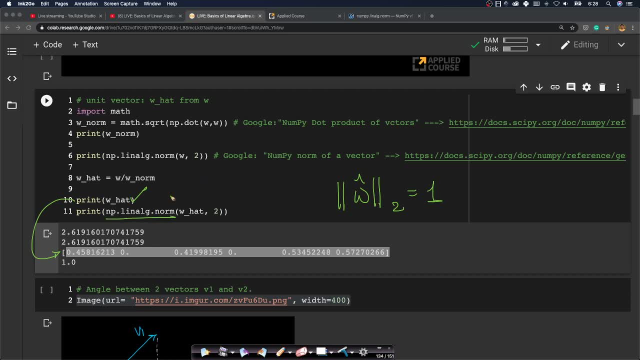 Again, we have this function, which we'll keep using now whenever we have to compute norm. Okay, that's what we figured out using the Google search, right? So w hat 2. And I'm using numpy linear algebra norm, And when I do this, this returns this print statement. 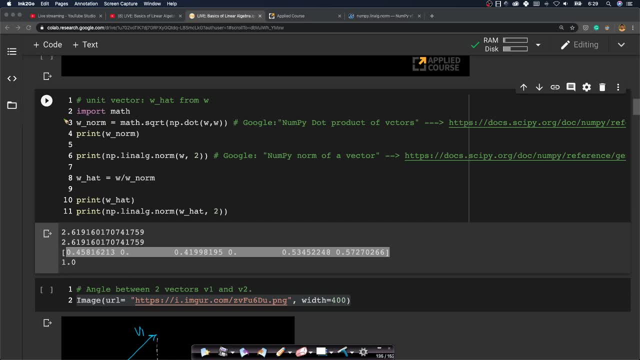 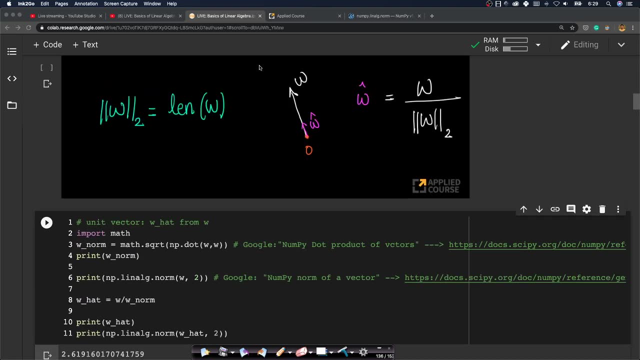 And the norm is 1.. That's it. So, whether you use our own code or whether you use the inbuilt function, again, this is how you translate simple equations. The equations that we are learning here are very, very simple. Going forward, we'll encounter much more complex stuff. 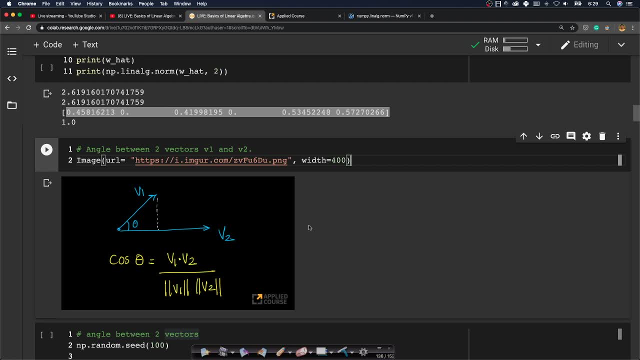 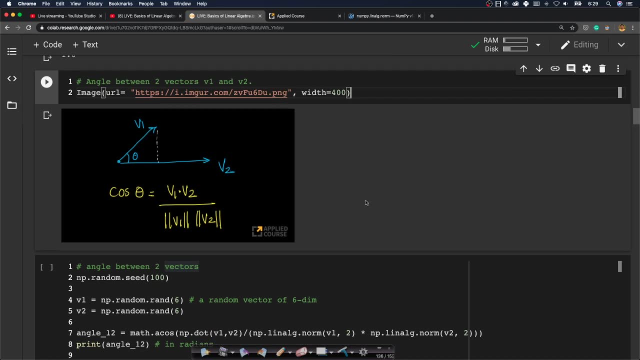 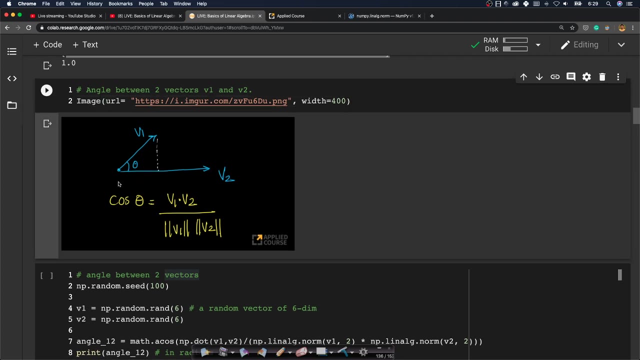 Okay, cool. Next very important operation that we perform a lot right is angle between two vectors. So if you have angle between two vectors, if you want to find angle between two vectors, how do we do that? Again, we prove this in the course videos that if you have two vectors- v1, v2, need 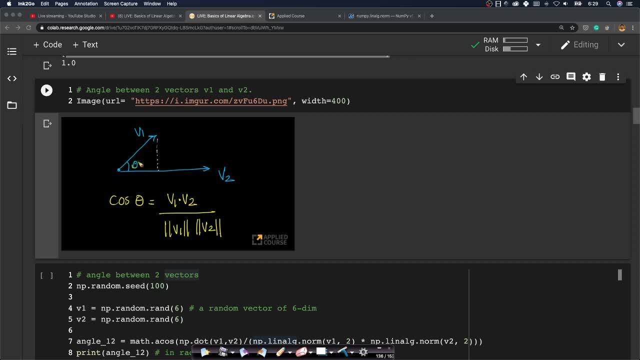 not be unit vectors. If you have two vectors, v1.. v2, the angle between them, let's assume, is theta, then cosine of theta is the dot product of v1, v2. by again, if I just write this, if I don't put any number here, this basically: 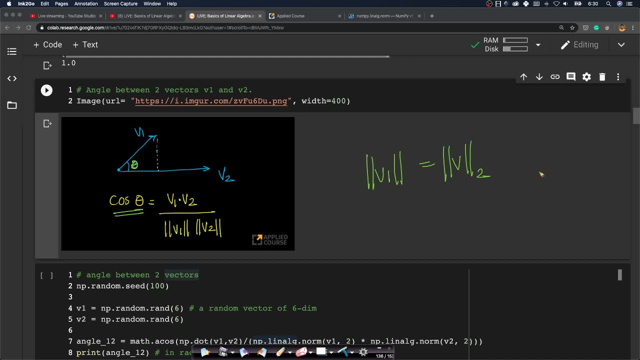 by default means l2 norm, unless otherwise stated. If it is l1 norm, people actually put l1 norm here. If it is Frobenius norm of a matrix, people put f. If nothing is placed here, that means automatically the default norm is always 2 norm. 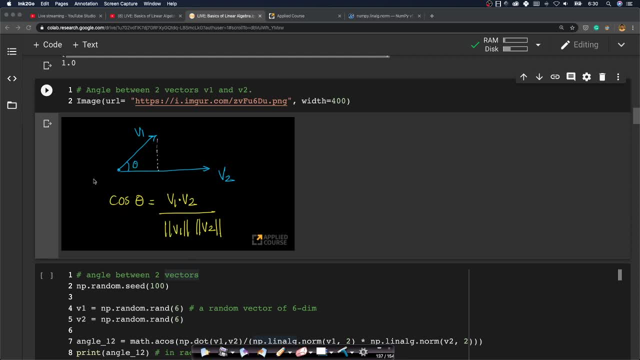 Unless otherwise stated right. So let's just get that clear. Okay, so we have derived this formula in the course videos. We have understood this, this very simple concept. This is literally high school level mathematics. nothing fancy here. Now let's take two vectors and actually translate this. 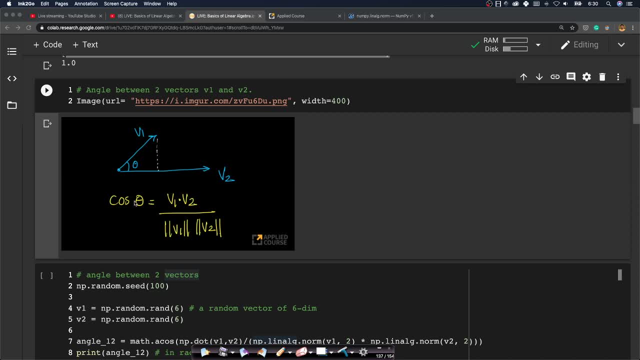 Imagine: if I'm given two vectors, how do I get the angle between them? Should be straightforward, right? It should just be cos inverse of this term. It should just be cos inverse of this right. So that shouldn't be too hard. 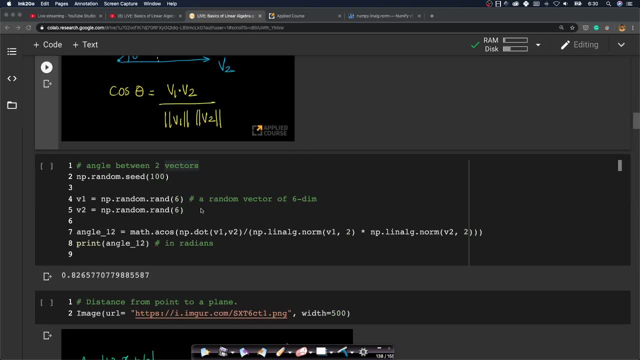 Again. okay, let's go step. Okay, let's create two random vectors. first, Again, I'm just creating a random seed so that every time I run this function, I run this snippet of code, I get the same values. Then I'm creating two random vectors: v1, v2.. 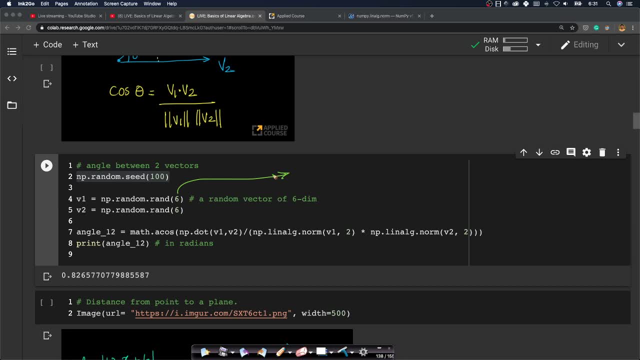 Again, random vectors will play a very important role when we learn about other concepts like locality sensitive hashing in k-nearest neighbors, right? So there is a concept called as locality sensitive hashing, which is basically a randomized algorithm which uses the concepts of random vectors, right? 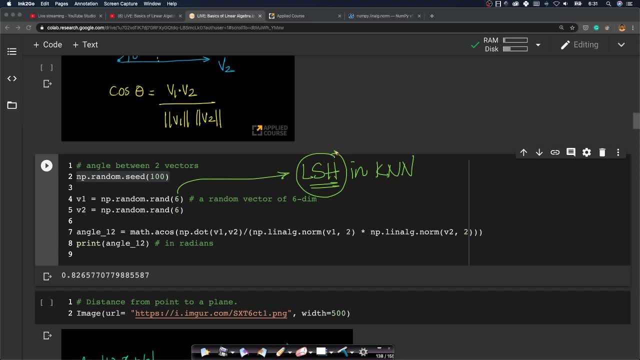 Again, we'll revisit the concept of random vectors when we look at locality sensitive hashing in the context of KNN later, when we do a live session on KNN itself or probably multiple live sessions on KNN. For now, what we'll limit ourselves to is 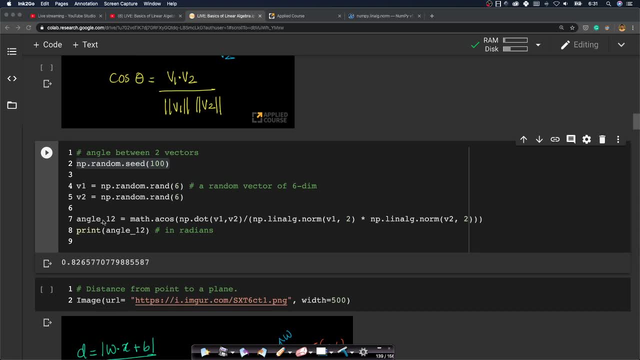 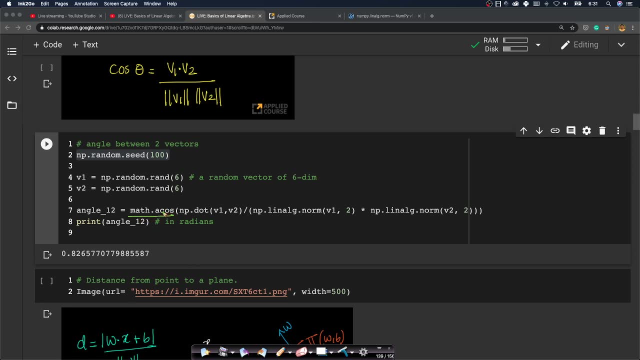 let's assume I have two vectors, v1, v2, if I want to get the angle between both of them, It should be simple, right Again, I'm just implementing it from first principles. I'm saying: mathacos, Acos is nothing but cos inverse, right? 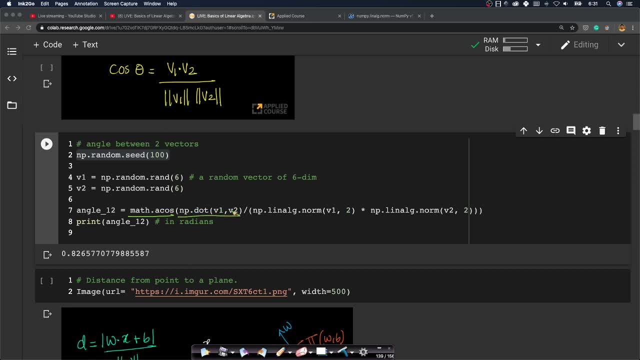 And what do I do? Dot product of v1. v2.. Look at this: Dot product of v1. v2.. Same thing Again. this is literally a very simple translation, Divided by norm of v1, multiplied by norm of v2.. 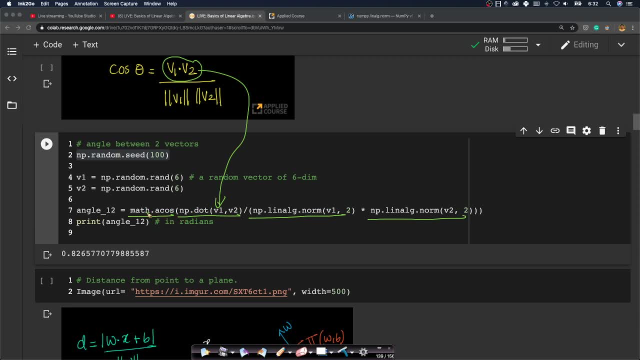 Again, NumPy gives me NumPy and math give me all this functionality. Remember, whatever angle you get here, angle 1, 2 is in radians, not in degrees. Okay, Most scientific computations are done in radians and not in. 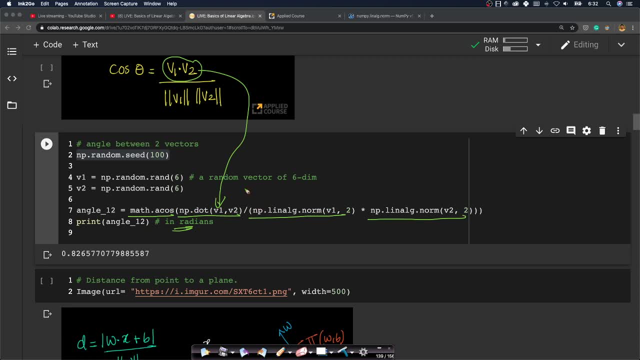 they're not done in in degrees, right. Very important, Okay, Cool, Okay, Somebody. okay, I'm happy that some of you are answering questions in questions in the in the live chat window. Very happy about it. 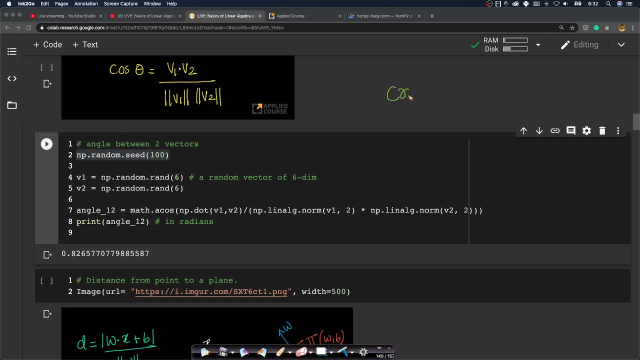 Thank you folks. Somebody is asking this question: Do we use cross product anywhere? Do we use cross product? Not the dot product? Remember the cross product that you have learned in physics in your 11th and 12th class, Right? 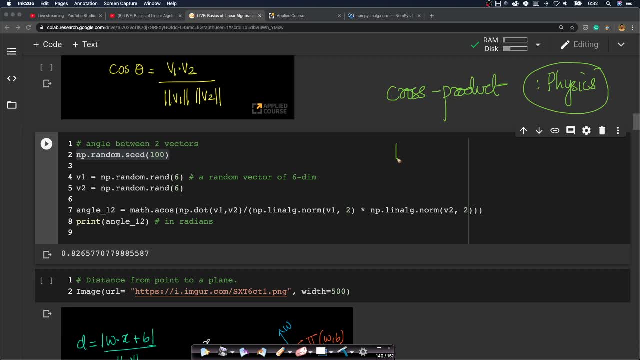 If you remember, we had this: F equals to B I L. right In electromagnetism, F equals to B I L. I forgot how to write this. Uh, this B is a vector of magnetic. I think this is how it looks. 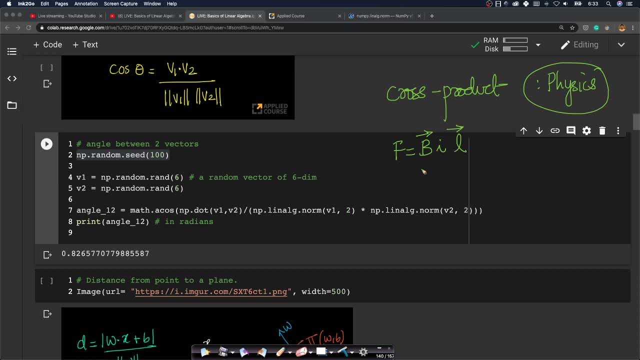 This is the length of the. this is the B, I, L. Okay, I think this. this is sort of the formula. I forgot It's. it's been a while I looked at this formula right. So you have the right hand thumb rule and all this. 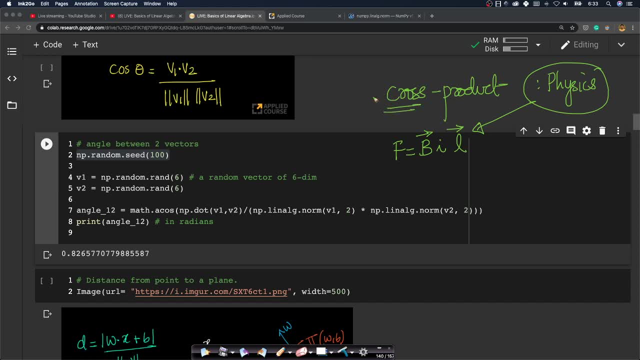 So cross product is not very often encountered in machine learning- Okay, And deep learning and all the concepts, but it is something that is used in physics a lot. dot product is what we use extensively because we want to find angles between lines or angles between hyperplanes- all of that stuff much. 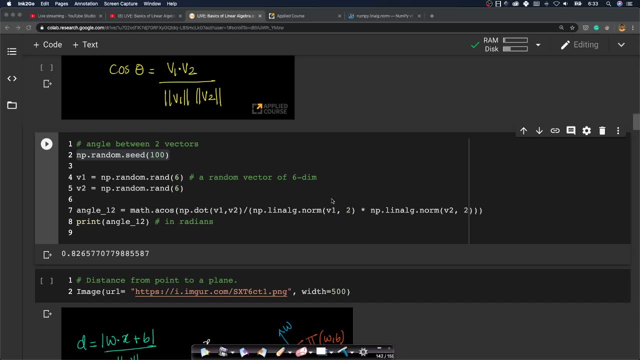 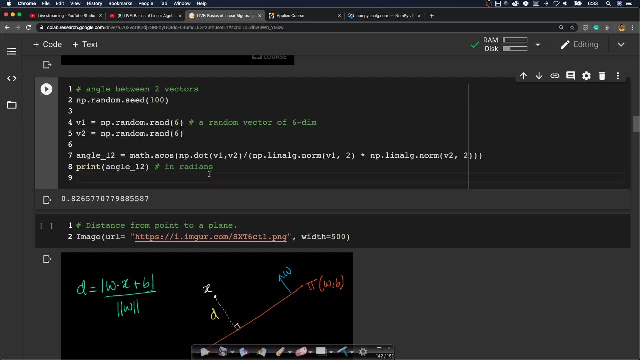 more extensively in machine learning. We don't use cross product much. Okay, Angle is always in radians, by default. always Okay, Because all of scientific computation happens in radians and not in degrees. Okay, In any scientific computational library all angles are represented. 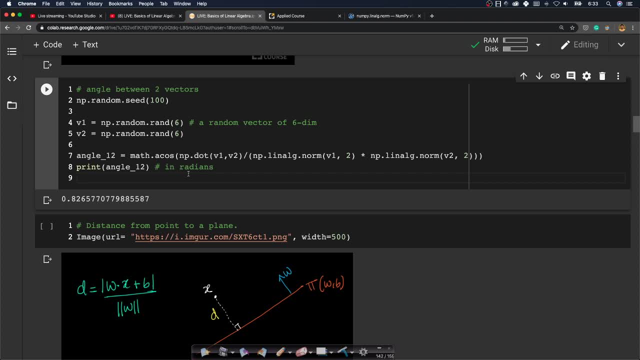 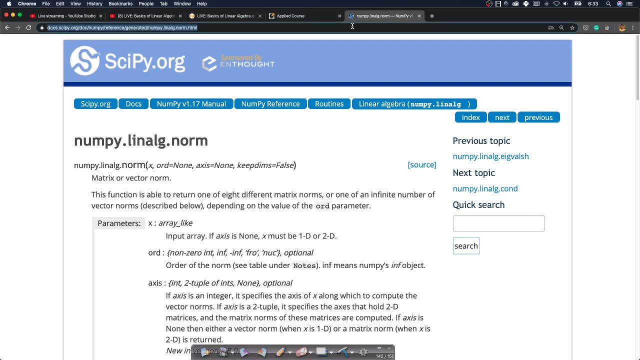 in radians by default, Right? So, uh, yeah, it's F. So yeah, as somebody rightly pointed out, I think, uh, just let me Google it, It's been. it's been almost 20 years. I saw this almost 20 years. F equals to B I L. 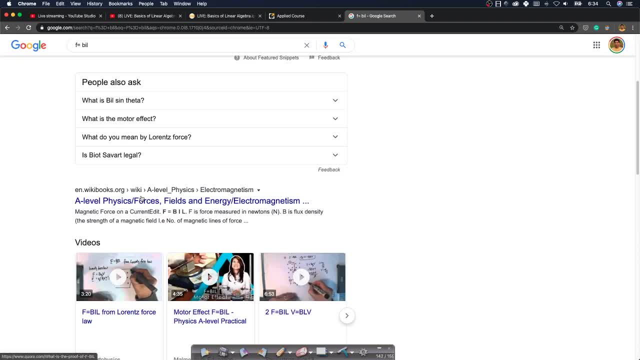 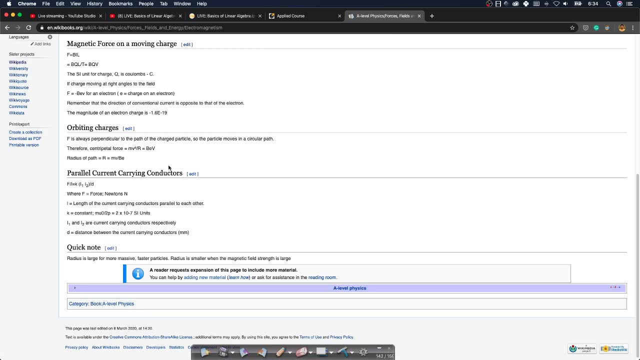 Right, So I think there's a cross product between: uh, okay, I think there's a cross product between B and where is this? Okay, There is sine theta, That's the intensity, but where is the direction? Okay, I think it is okay. 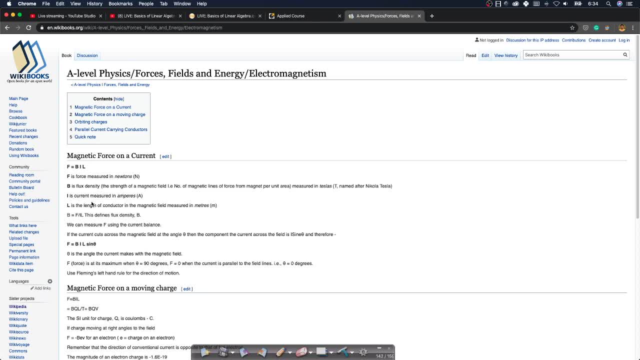 B is the flux density. Uh, B Is flux density, F is force in Newton's. Okay, Yeah, There is, there is cross product somewhere here, If I recall, if I recall uh, force on a current in a magnetic field. 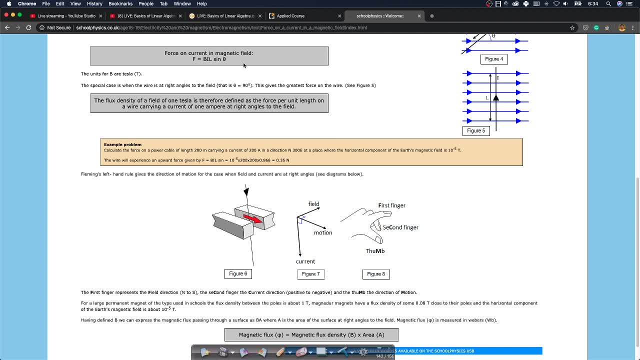 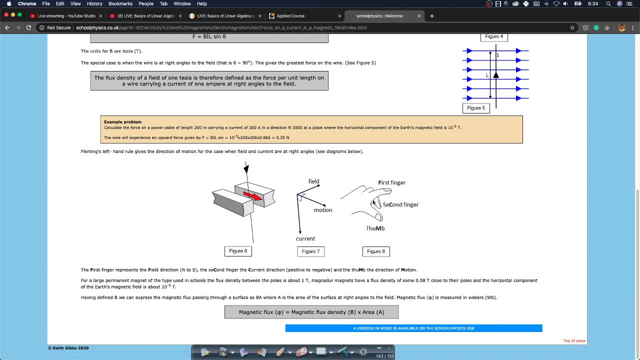 Oh, this is school level physics, Cool, Okay, B I L the. the reason you have sine theta here is because of the cross product and not the dot product. Oh, there is this. yeah, Right-hand rule. I think it's called thumb rule or something. 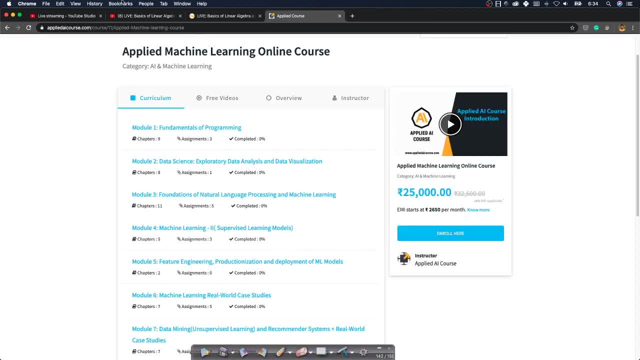 Oh, so look at this. So yeah, it's. it's encountered in physics a lot. We know that. right, I forgot the exact formula from level 12th class math. It's been years I've done it, Okay. 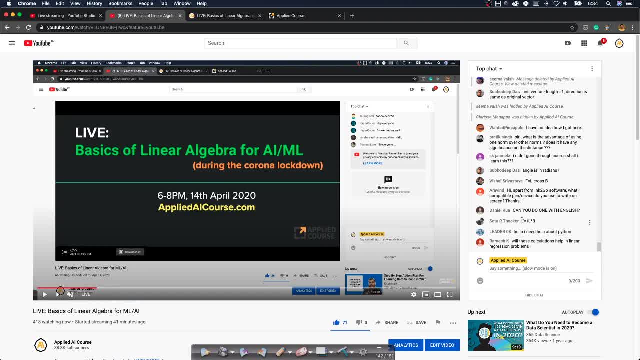 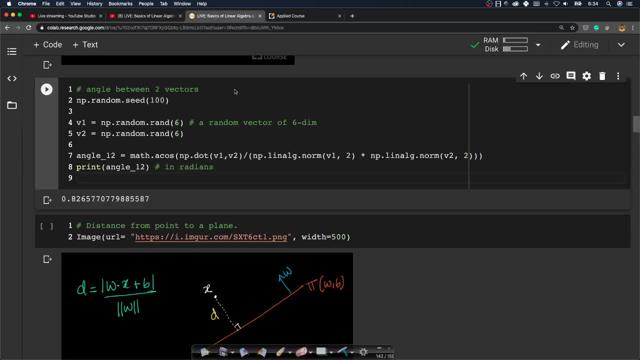 Sounds good. Yeah, Somebody says F equals to IL cross B. I'll take your word, assuming that your electrical engineer, who knows this much better than us. Okay, We have. we have after, after our 12th class. I've not encountered this myself. 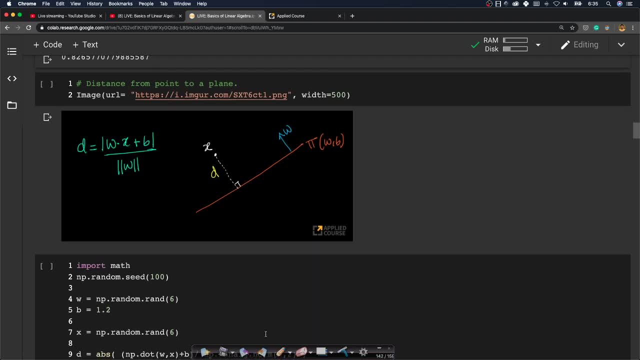 Okay, Cool. So let's go back to, uh, data science, specific stuff. Okay. So the other thing, right Given up, suppose, if I have a hyperplane pie like this, which I'm not saying is passing through origin or anything- it is represented by W and B. 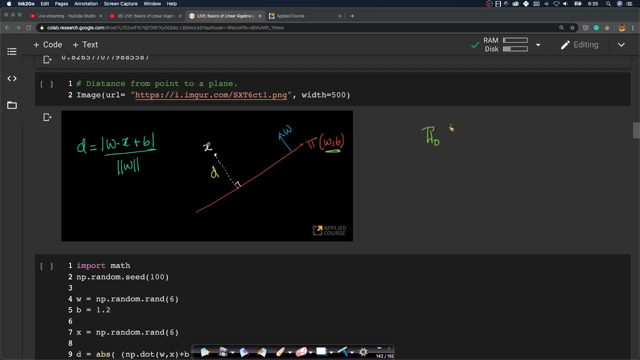 Okay, General pipe. When I say PI zero, only Then It passes through origin. If I just say PI, it is always uh, parameterized using W and B, both Okay, And let's assume W is the normal to this. 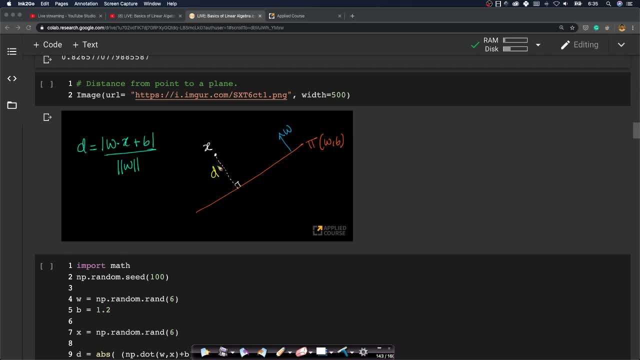 There is a point X. What is the distance? What is, what is this distance from X to this? Again, this is something that we use a lot, whether we are doing logistic regression, right, whether we are using linear regression, whether you are. 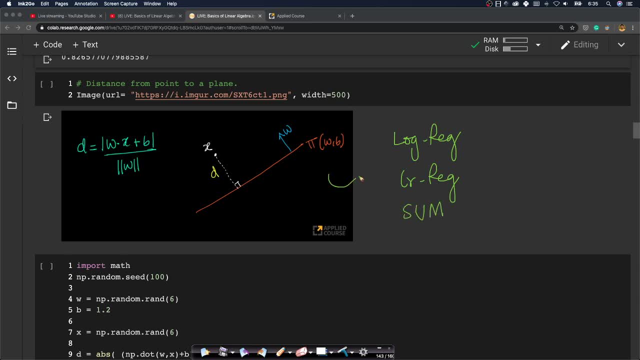 using support vector machines. you know all these techniques. this mathematics is extremely important. A lot of machine learning techniques that we encounter a lot. They try to find a plane And to do that, distance from a point to a plane is very important. 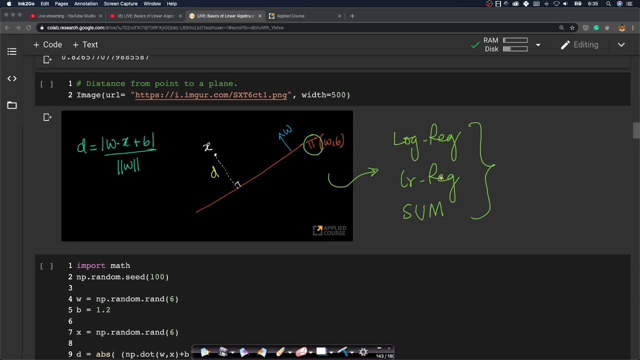 Again, when we do the logistic regression sessions, linear regression and SVM- we'll see this reoccurring again and again and again, Right Cool. So first let's learn the basics. What is the distance here? Again, we have proven this in the course videos using a very simple diagram: et. 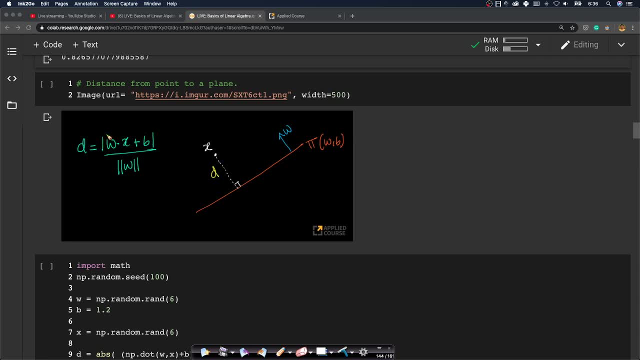 cetera. The distance is absolute value of W trans W dot X plus B. Okay, So the distance here is just W dot X plus B by norm of W, because I'm not saying that W, W is a. uh, I'm not. I'm not saying that W is a unit vector. 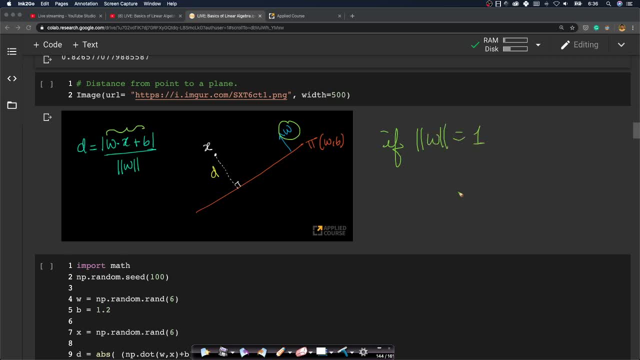 If W is a unit vector, if norm of W equals to one, then the distance here is just W dot X plus B absolute value. Why are we putting the absolute value here? Because distance is always positive. Okay, So that's why we are putting the absolute value here. 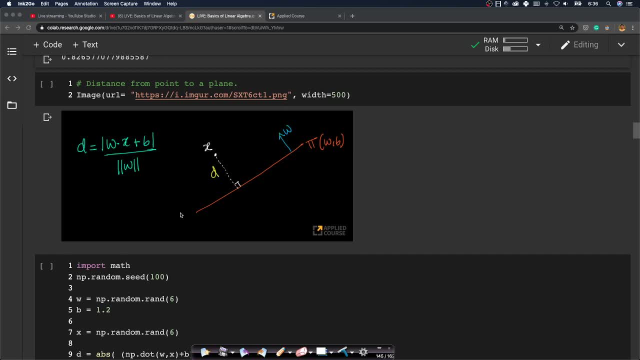 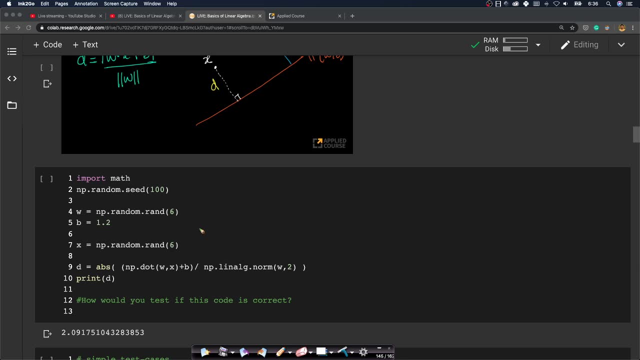 Right. So again, let's just create some random planes. Let's just compute the distance, Okay, cool. So what am I doing here? I just wanted to show how to translate this simple formula to equations. It's very, very simple action. 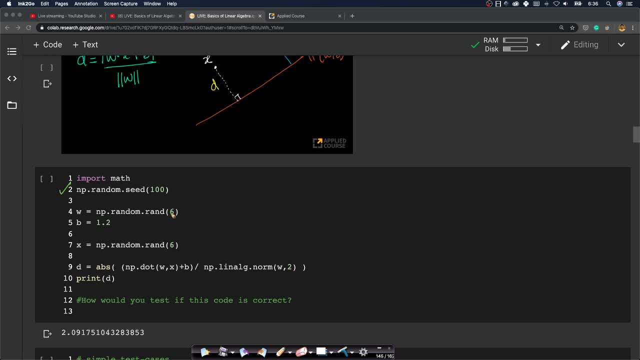 Okay, Again, I'm just creating a random seed and I'm creating this W, which is a six dimensional vector. Look at, this W is a six dimensional vector. B is just a real value number and I'm creating a random point X. 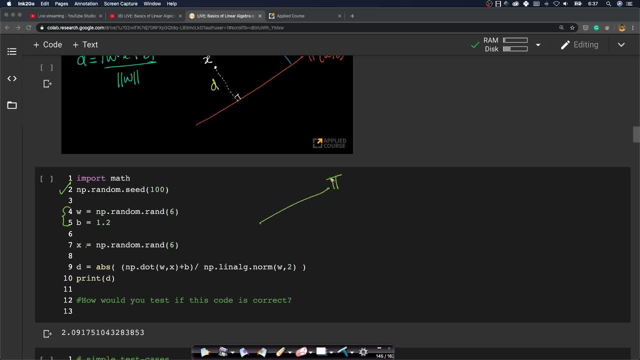 Okay, I'm just so. using this W and B, I'm getting a plane pie right. Using this X, I'm getting some point X, some point X, Okay. So now, using this, I can compute the distance using- I'll just translate this formula- that: 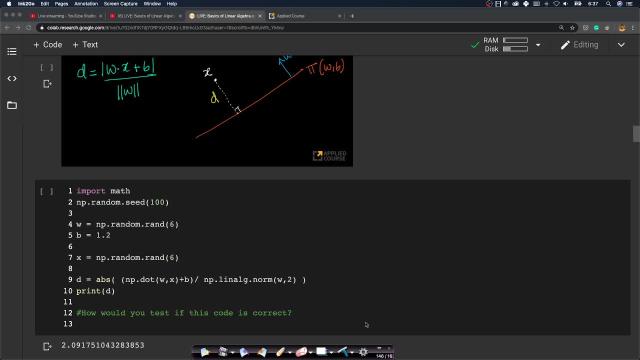 we have seen It's. it's a very simple translation. It's just simply translating this formula to equation. Again, NumPy gives you most of the heavy duty stuff, right? We don't have to worry about it again for the mathematical proofs of this. 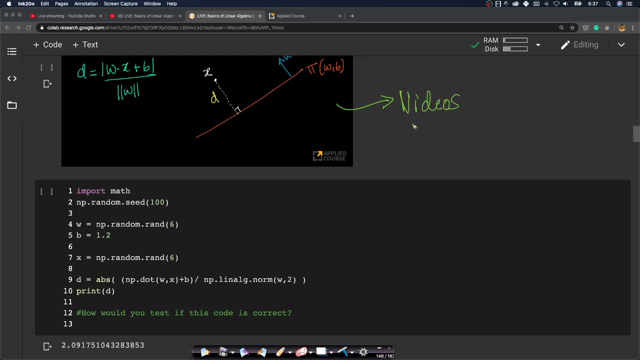 Please look at the videos that we have posted as part of our course, videos publicly available to everyone. Please go check out those videos for proofs of this. Again, I requested you to do that before the live session itself, right? So I'll not. 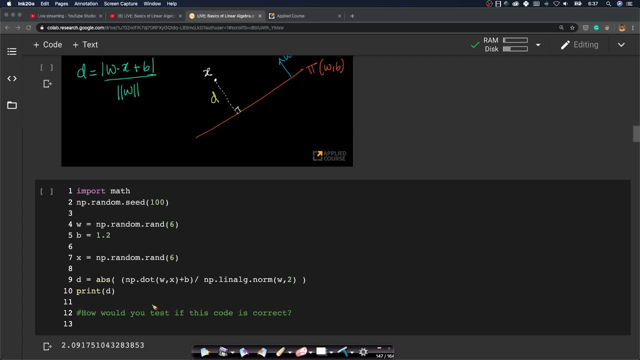 Be covering those mathematical proofs and details here, Cool. So how do you do it? It's very simple. Again, I'm covering the basics. We'll keep going to more complex cases as we progress. Right, So it's actually very simple. 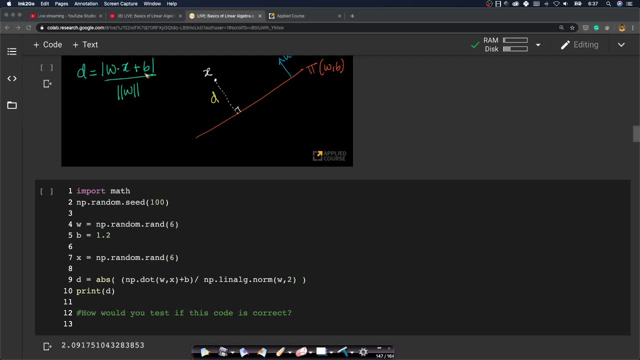 Now let's look at this right. So what? what is the formula W, dot, X plus B? So it is basically dot product of W and B plus B. in the numerator, in the denominator It is norm of W or L2 norm of W. 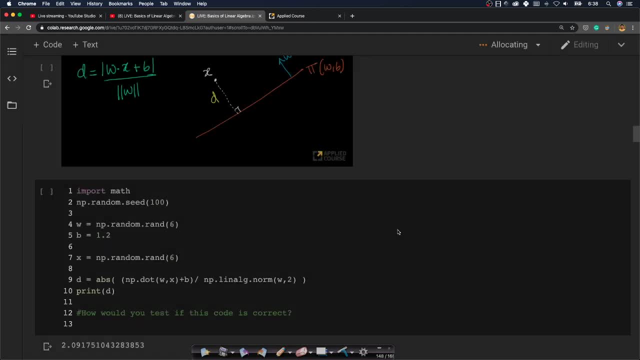 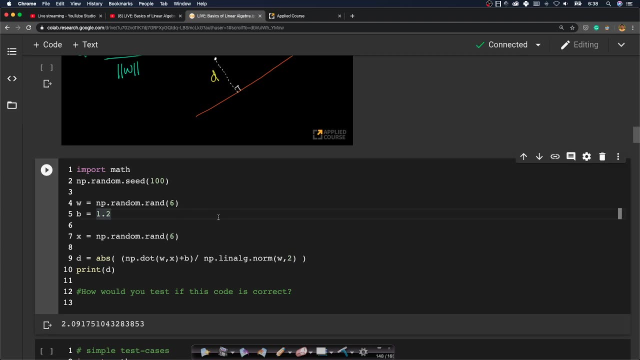 Oh, okay, I think I did not reconnect. Okay, I hope it reconnects and everything works. It does. Okay, If you don't have enough activity for, I think, a few minutes collab, uh, automatically disconnects. 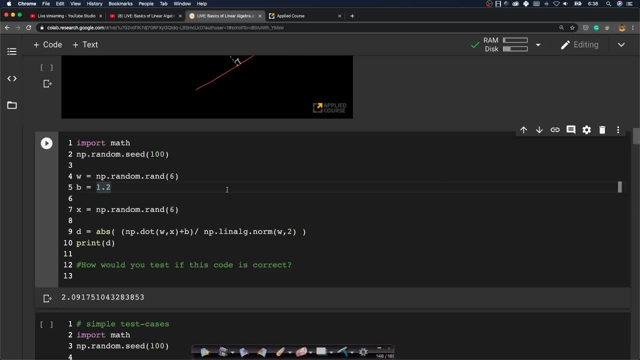 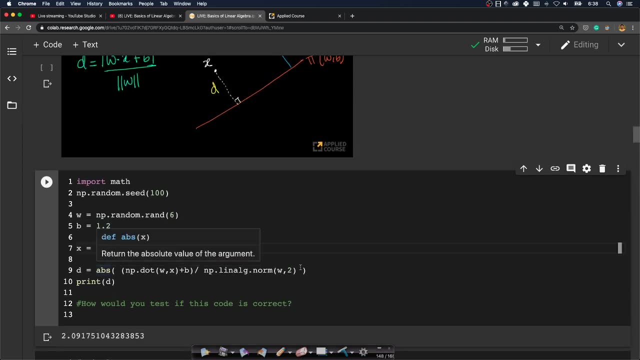 There's a way- I don't- that I can change the JavaScript here to make sure that it doesn't die. There are some hacks around it, Cool. So very simple. I have the code here. It works, Okay. So I'm just. I've simply translated what we see here. 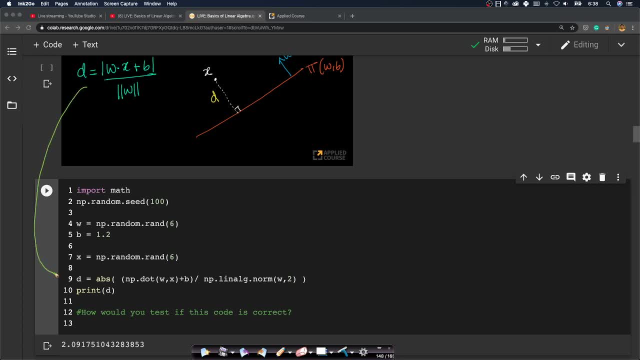 Very simply, the equation that we see here. I just wrote it as one, one simple line of code. Now, the big question that I have Here Here is: you've written this code, Okay, Seems logical. How do you test this code again? 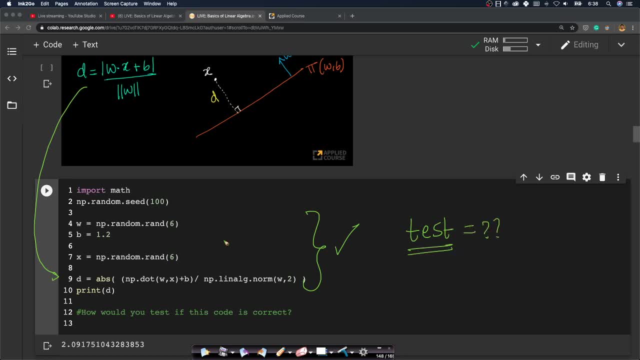 As I mentioned in the previous live sessions, for any problem or any snippet of code in any function you write right? How do you test it? Right? How do you test it? How do you test that this code actually works? or maybe you've done a small mistake instead? 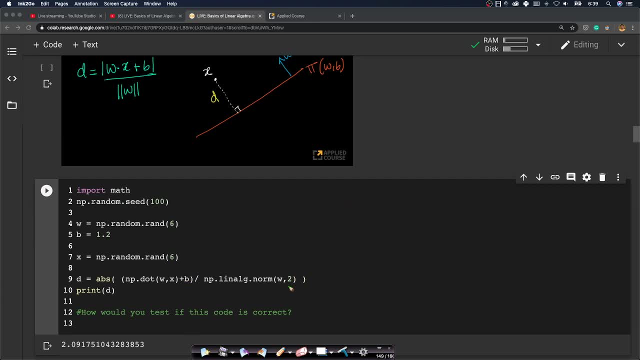 of plus, you wrote minus, and everything goes for a toss. Instead of norm two, you did norm one, and everything goes for a toss. How do you test this code again? You can. For most of this functionality you can just uh, yeah, somebody's asking about random seed. 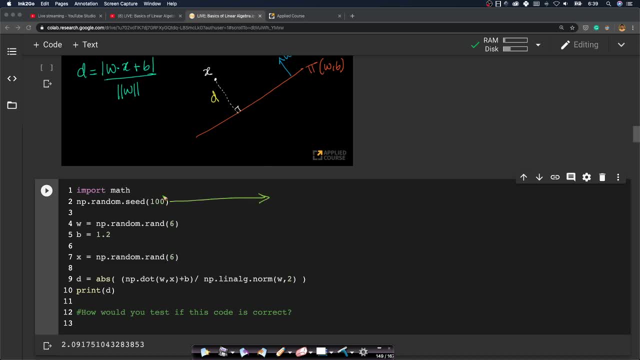 So what random seed does? let me just explain this. You can give so random seed. I've explained this in the in the previous live sessions also, but let me just repeat it quickly, right? So random seed. I can use any number here. 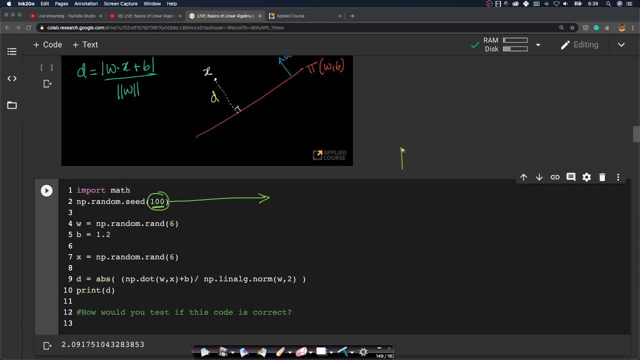 This basically so your random number generator, also called a pseudo random number generator- pseudo random number generators that you have in most programming languages and in most libraries. they generate a seed. It's a sequence of numbers. So every time I run this code- if I did not have this line, every time I run this code I get a different set of random numbers, right? 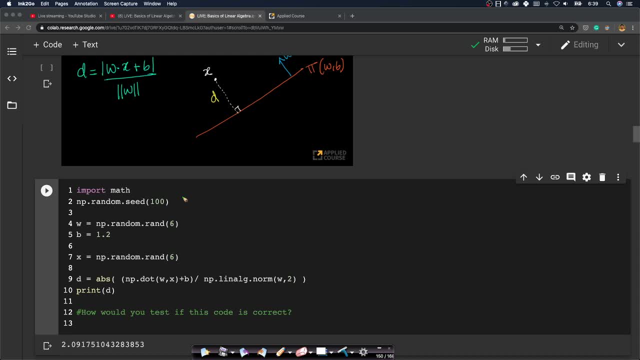 I get a different set of random numbers by using this line and fixing the number always the same. So this number says intuitively: again, I'm not telling you how, uh, in this context I'm not going into the depths of how pseudo random number generators works, how seed works. 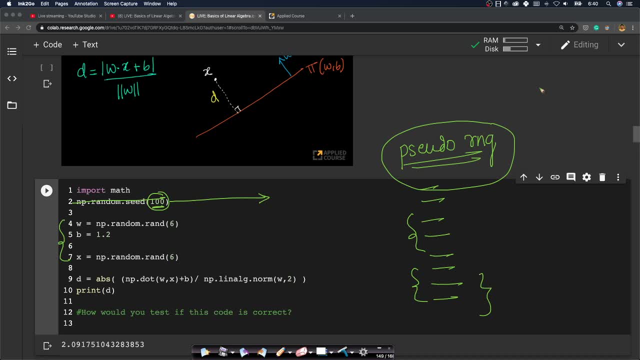 I'm not going into the mathematics because that's a fairly in-depth mathematical uh description And it's a very simple discussion onto itself, but intuitively, what it does is very simple. The moment you you set this 200, okay, next time, whatever numbers you generate, every time the same numbers are generated. 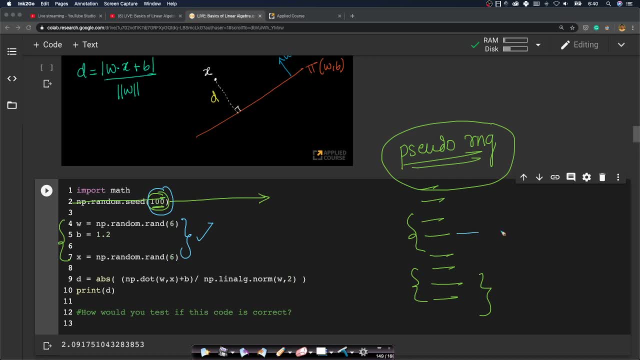 This is like ensuring that the random number generator starts at some specific point. You can think of this point as a hundred from this point. So when I say CD equals 200, it will always go to this point in a sequence of random number, random numbers, and it will always generate random numbers from that's, from that location. 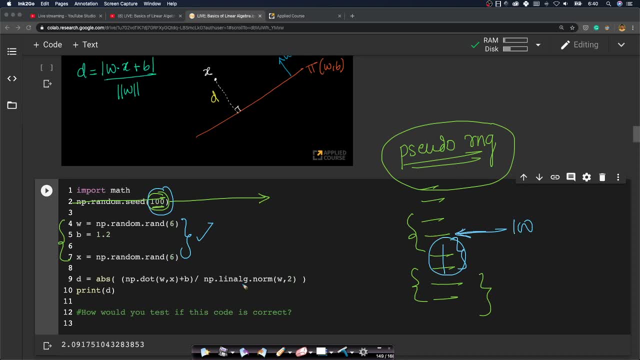 Think of it. Uh, I mean that the easiest way to think about it. so this is: this is written so as to ensure that every time I run the code, I get the same random numbers. otherwise, when you run, you get different random numbers. I get different random numbers and things. 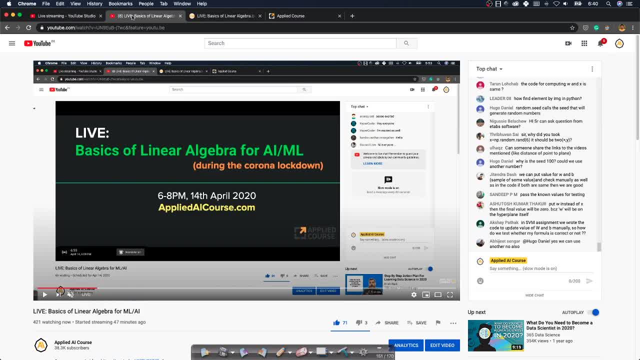 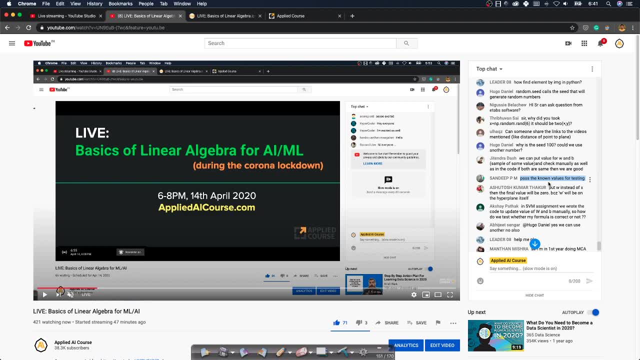 like that cool. so how do we test it? okay, let me see. let me see. okay, pass the known values for testing. can you suggest me some good known values, folks? again, you can use any seed, guys, you can use any seed. you can use 10, any number just. 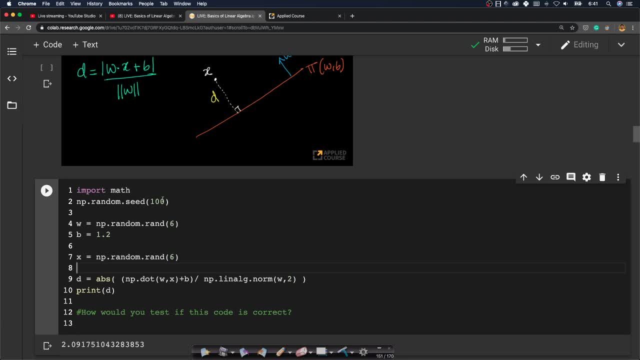 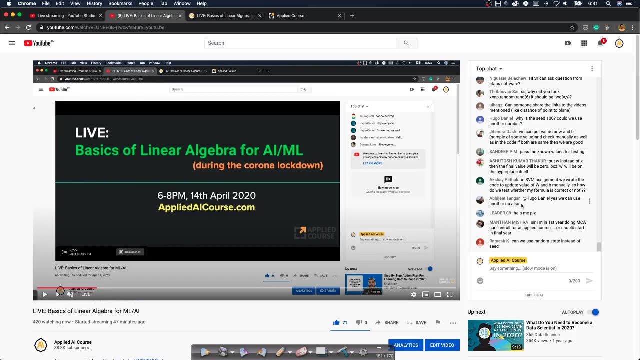 look at the documentation for NP random seed. you can use any number here, just fix that number every time you are running it. that's it. yeah, you can use random state random seed. all of them do mostly the similar stuff, right, so don't worry about it again. I'll try to answer only questions which are in the context. 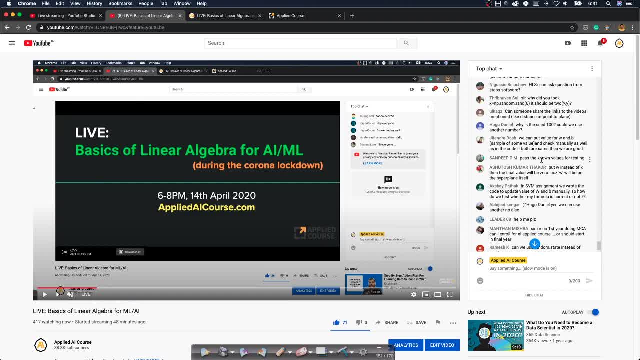 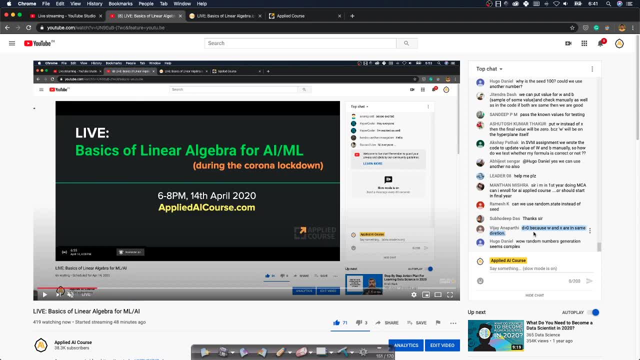 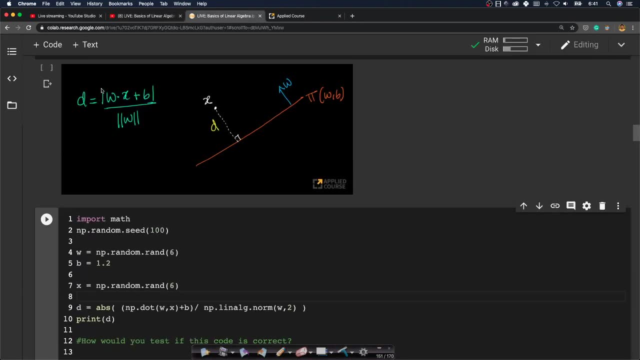 of the discussion for enough, because we are in the middle of it. pass the known values for testing. what are some simple values that you can pass? D greater than 0, because W and X are in the same direction. no, no, no, no, no, no, no. somebody is mistaken here. look at the code that we have written. there is an. 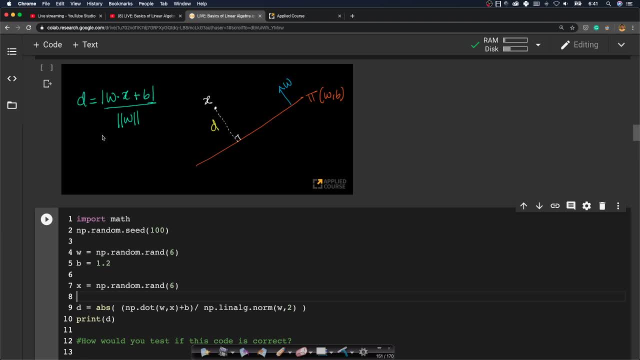 absolute value here, which means D will always be positive. I just mentioned this a few minutes back. right D I am placing because the distance is always a positive number. we'll come to half spaces will come to which side? a point is little later. okay, please don't confuse those two now. oh so somebody. 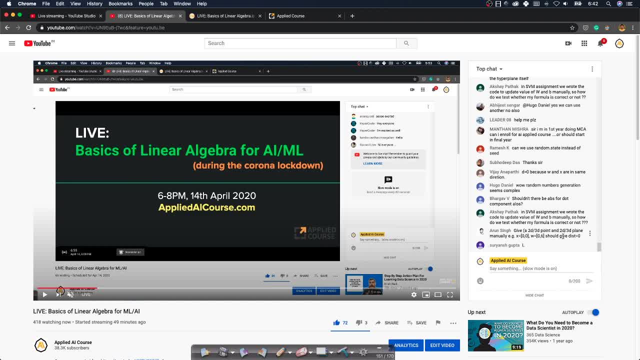 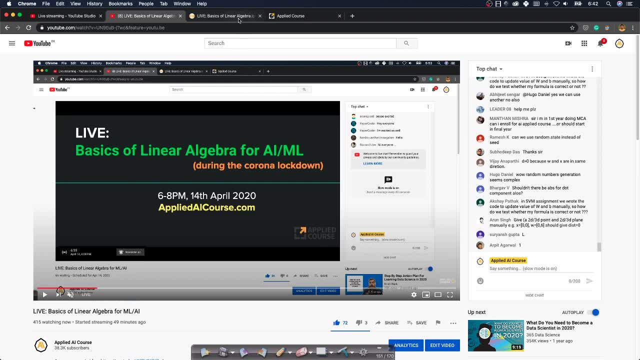 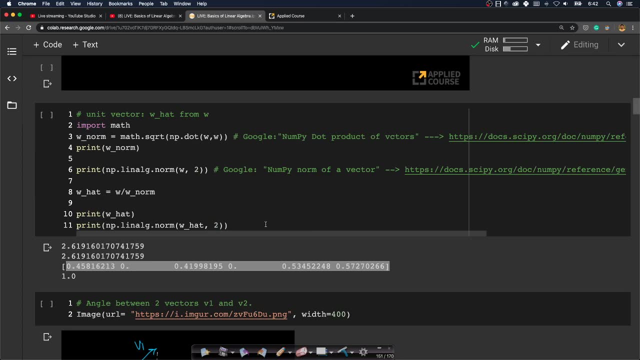 says 2d, 3d point. you should give this blah, blah, blah. okay. so this is so for dot product also. why do you need the distance, the this thing for dot product? because you're taking the you don't require for dot product, right? why do you need absolute value for? 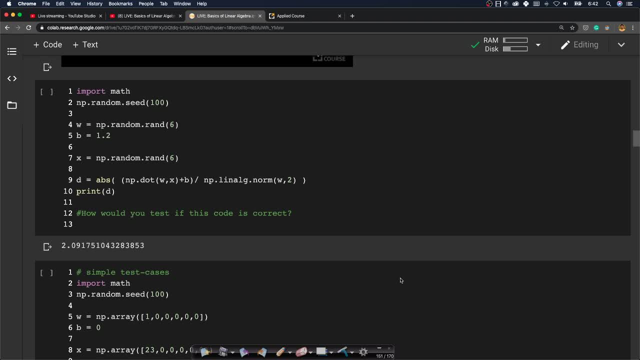 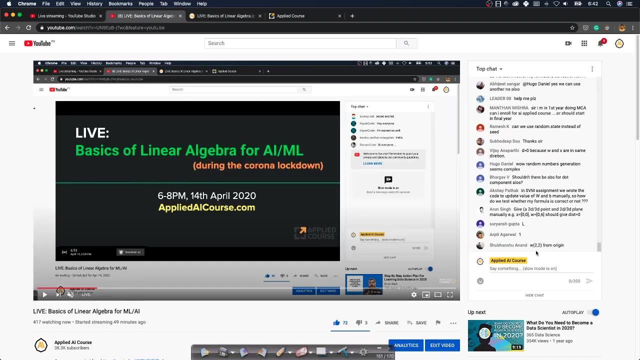 dot product. you don't need it, so okay, so where were we? okay, so how do we? how do we test this? how do we test this? very easily, okay, some simple test cases. that you guys w22 from origin. okay, okay, that's a good idea. okay, just just write a function for this and pass. 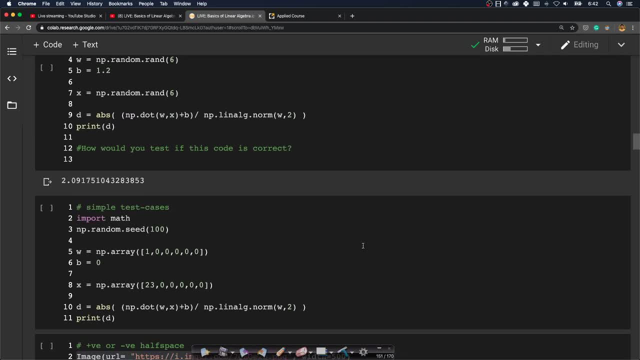 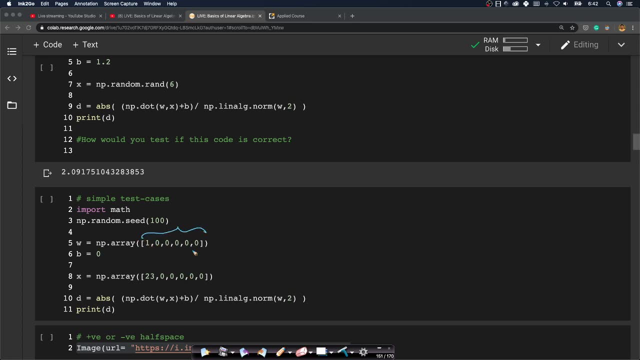 different vectors. that's a good idea. one simple thing that I'll suggest you is this: look at this very simple suggestion right again, this is a six-dimensional. remember, this is a six-dimensional vector. so my vector w is such that the x axis, the first axis, so this is six dimensional, of course I. 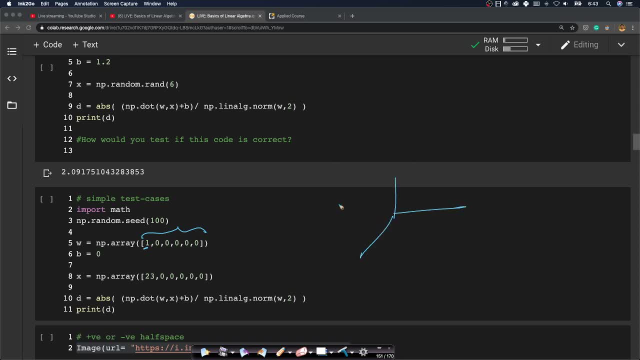 can't draw six dimension, I can't draw anything more than 3d, right suppose? Let's say there is first dimensions, second dimension, third dimension, there is 4, 5, 6 dimensions also, so two dimensions. so that makes per discussion somewhere. So I am creating my w such that my w only is on this direction. Look at this. 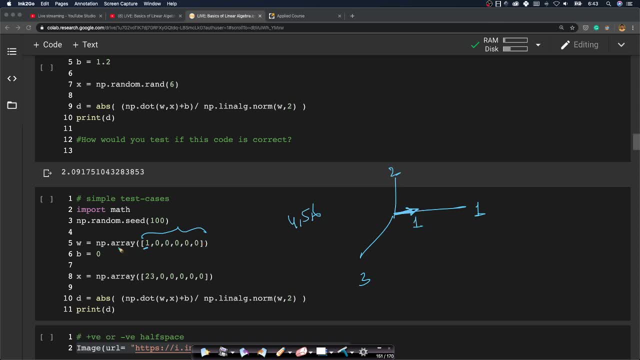 my w is such that its length on the first dimension is 1, rest all dimensions- is 0, which means it will be on this axis. If you think about it, it will be on the axis corresponding to the first dimension. Now, if my x is also on the same, so the way again. you can test it in many. 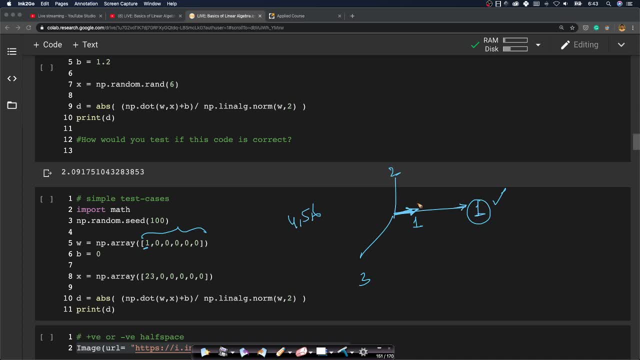 many ways. If you want to test it in high dimensional space, this is one simple technique. So my w is again. remember that norm w here is 1 for me. Cool. Now look at this. I am also choosing my x such that my x only has component in the first dimension, All the other, 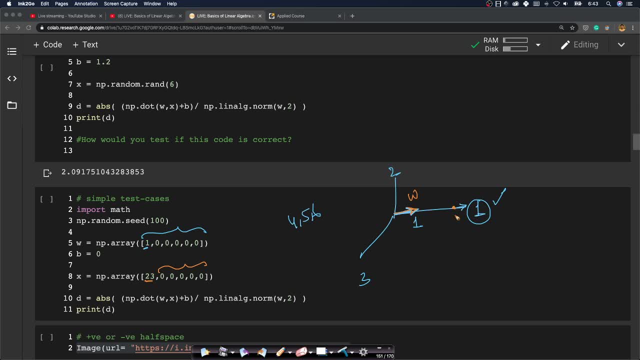 dimension components are 0.. So which means where is my x? My x also will lie in this, in this, on this axis only, because rest of all the axis- 2,, 3,, 4,, 5,, 6 axis- are all 0, right. 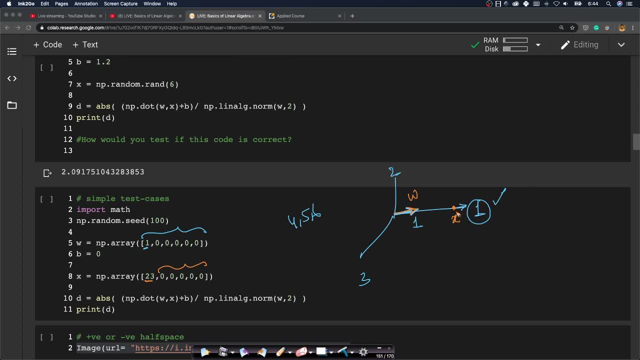 So what happens now? What should be the distance of x now? Look at this. So what should be the distance of x now? Look at this. So what should be the distance of x now? Look at this. What should be the distance of x from w? That is what we want to compute, right. What should? 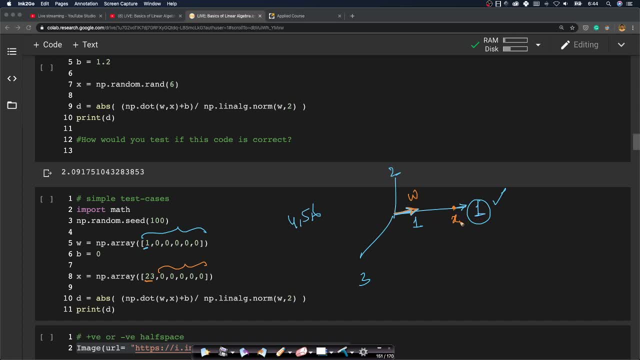 be the distance of x from w, Right? Very simple. I hope the question is clear, right? So I am representing my plane, Remember I am. so instead of saying distance of x from w, let us say distance of the plane represented by w. So my plane has this normal. Look at this. Let us imagine this. 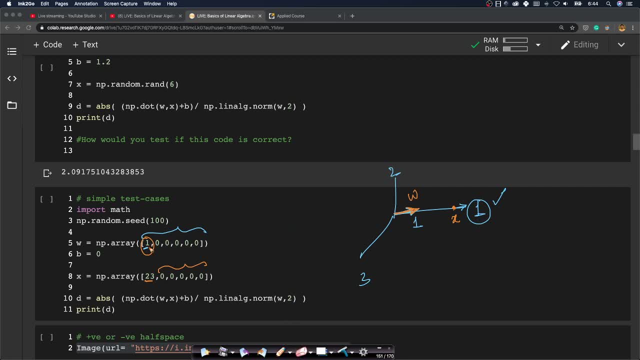 in 3D first, because 6D is anyway impossible. So imagine I have only 3 dimensions here. My w is represented like this, which means: where is my plane? My plane is actually here, right? Which means my plane is actually here. My plane is the axis that my plane is spanned by, or my plane is. 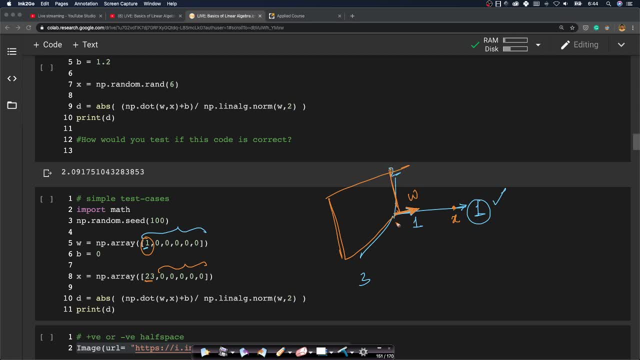 this plane, which has vector 2, or axis 2 and axis 3, because this is perpendicular. Again, I am trying to draw a 3D diagram here, right? So this is my plane now. right Now, my x is here, So what? 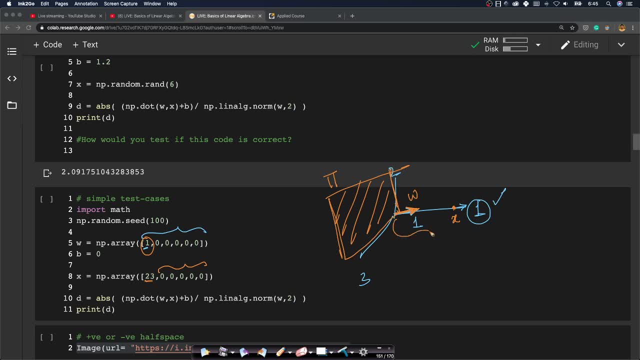 should be the distance of x from the plane. It should be the distance on the x axis itself. The distance should be 23,. right, Again, this is one simple case that I am building here. right, The distance should be 23.. Again, you can write lots of simple test cases like this. I am trying to 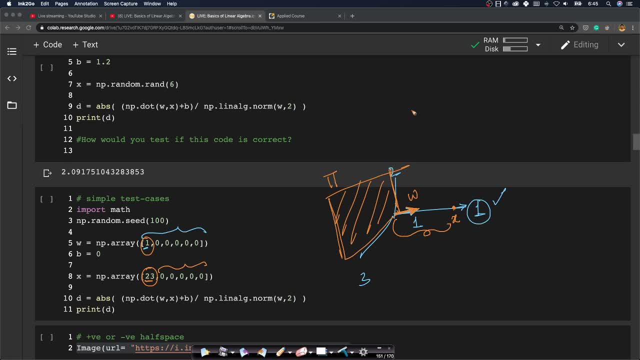 show you how to think of test cases in d-dimensional spaces. The easiest one is to test cases in 2D and 3D spaces. That is easier because you can simply come up with something that you can visualize easily and do it, But you can also construct examples in high D spaces like this: 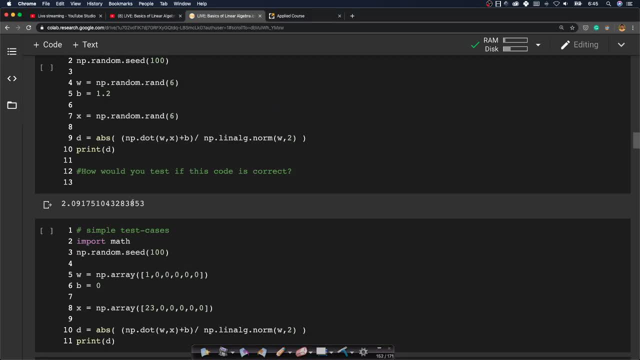 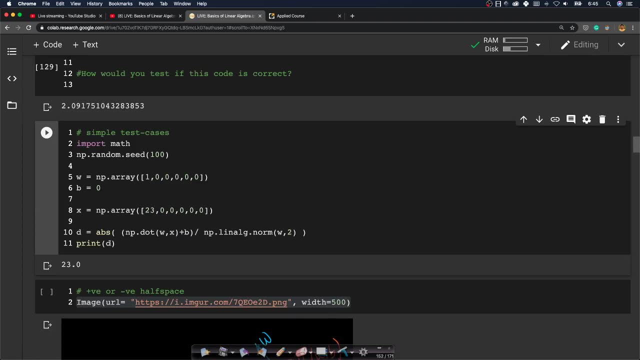 right, So you just do that and the answer should be okay. so where is this? Oh, it got here, So let me just run this once. So let me run the snippet of code. The answer should be 23. 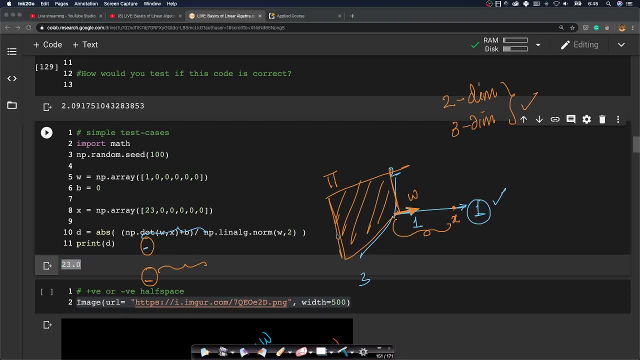 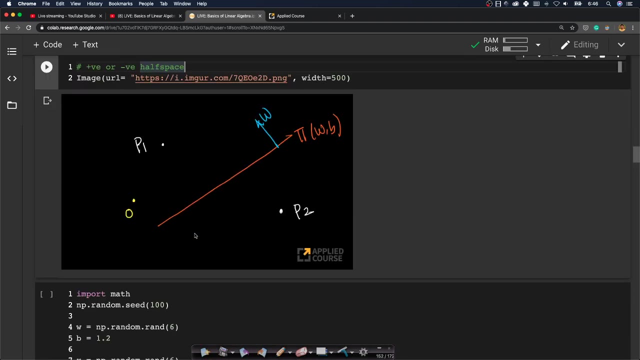 as I just explained a while ago, right The same concept that you can imagine in 2D and 3D scales to 6D, right, Especially with respect to planes and distance from planes and things like that, right, Very, very simple case. Now, somebody was saying about half spaces, right? So what is? 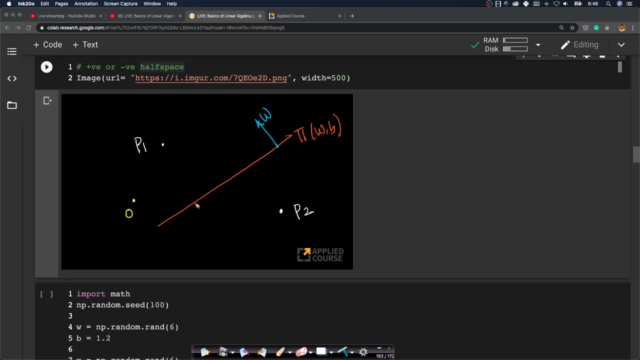 the concept of a half space. Look at this. Imagine if I have a plane like this. I have a plane like this, which is represented using W and B right, And my W is pointing in this direction. let us say My W is pointing in this direction. Now, all the points which are there on this side of the plane. 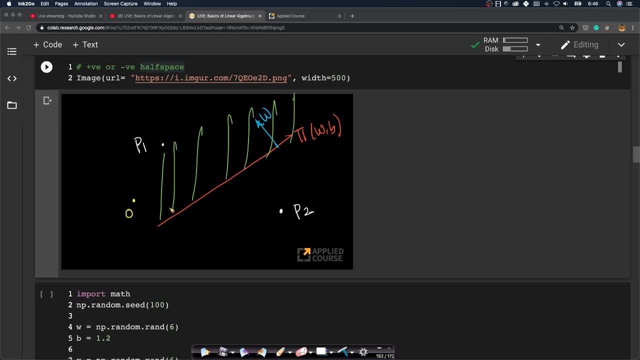 all the points that are there in this side of the plane is called one half space. It is also called as positive half space because this plane, effectively this plane, is breaking the whole space into two half spaces. Look at this, This plane does not stop here, right? This plane? 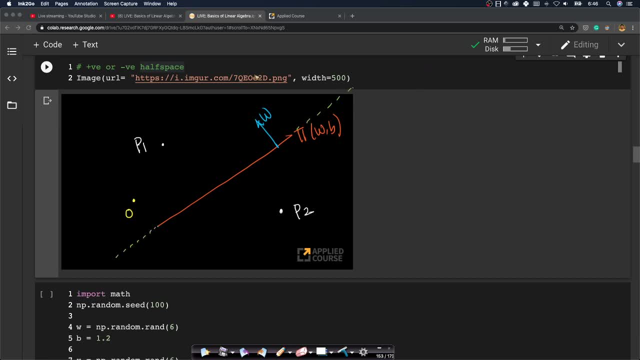 just keeps going on like this. This plane keeps going on, Given this whole in 2D space. this is breaking the 2D space into this space, and this space, The space in which the space towards which W is also present or W is pointing to, is called the positive half space. The other side is called 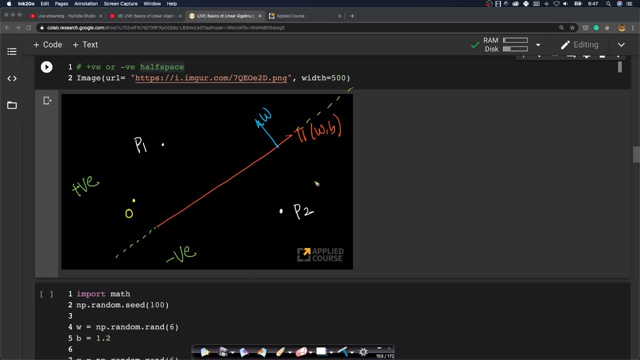 negative half space. We have discussed this in the course videos also. Now, given any point P1 or P2,, how do we determine whether a point is in positive half space or negative half space? Negative half space Because, again, this concept is very, very important when we do logistic. 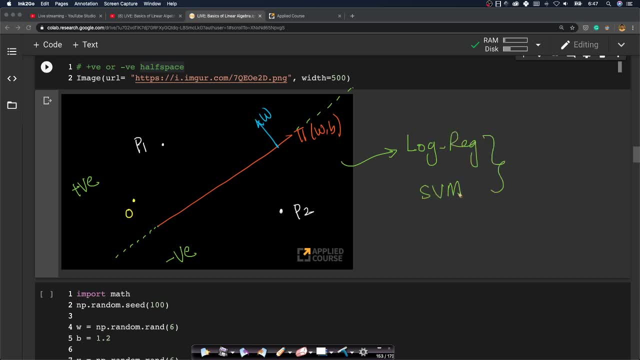 regression when we do SVMs and concepts like this right. These concepts will play one of the most important roles when you learn machine learning algorithms. Again, I am not teaching everything randomly. I am trying to limit myself to concepts that we encounter again and again in 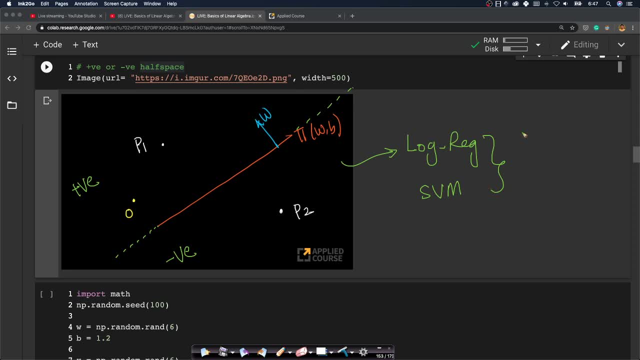 machine learning. So this is like the basics that you need for future stuff, right? So again, this is very simple. It is a very similar formulation like earlier. It just says: okay, so given this P1, I just take W, dot, P1 plus B, If this is greater than 0,. 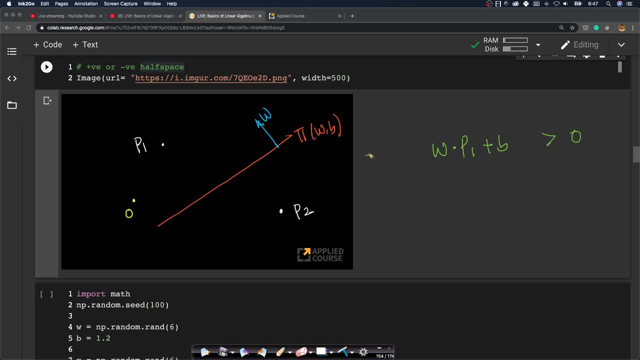 look at this: If this is greater than 0,, then it is in the positive half space. okay. If this is less than 0, W dot P2 plus B. If it is less than 0, it is in the negative half space. If it is. 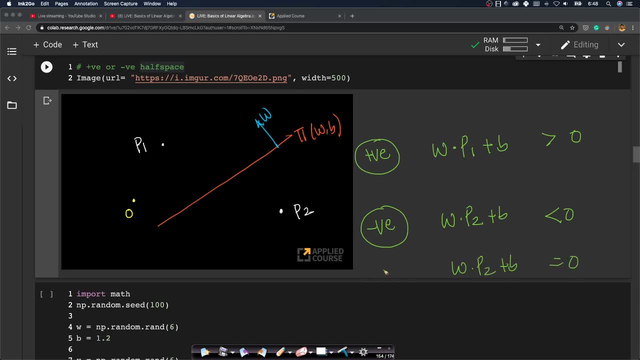 exactly equals to 0, it is on the hyperplane. It is on the hyperplane Because all the points here- look at this- all the points here, like if I have a point P3 here, okay, So let me write it as P3, okay, If I point P3,? 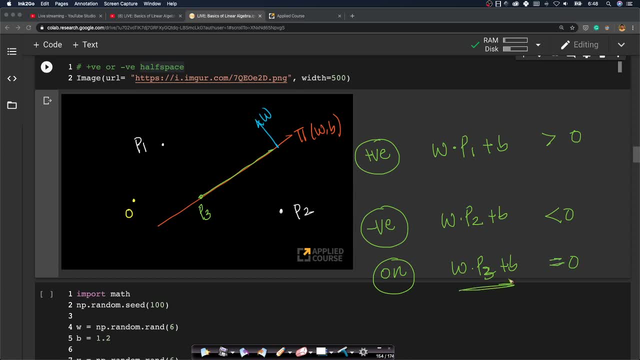 this will be equal to 0,. right, That is a definition. That is a definition of a plane as we discussed and as we derived it. And again, why is this so? We have discussed in the course videos. I am not going to repeat that proof here, But this is the general idea, right? 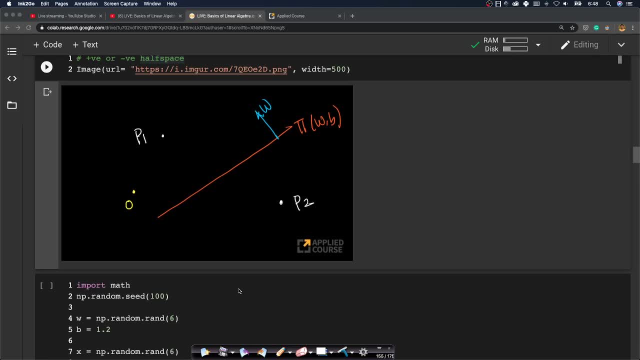 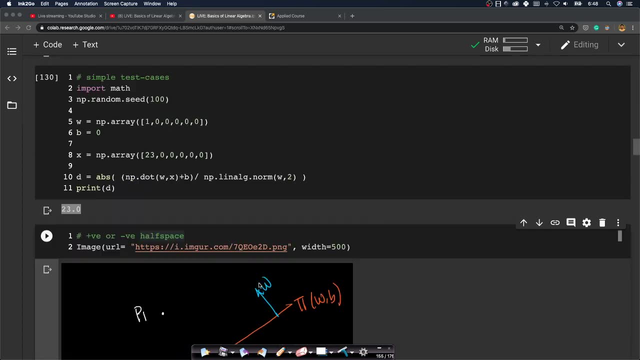 So now let us see. So somebody says: if angles are in 90 degrees, I did not understand. What about if plane is not on a particular axis? Again these. so again, this is just a test case that I have shown you on how to test that the 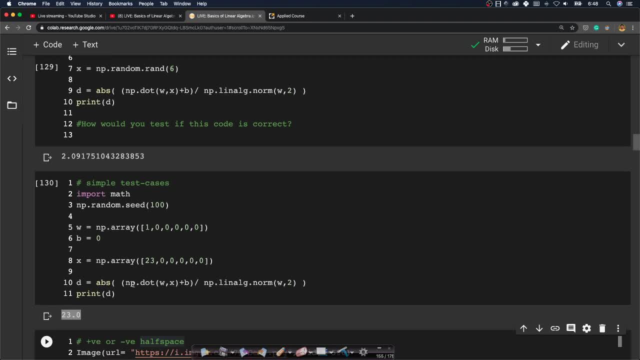 code we have written is correct. The test cases: we will try and pick the simpler test cases. If you want more complex test cases, try it in 2D and 3D. In higher dimensions you cannot even visualize what is happening, right? So coming back to the half spaces concept now, okay, So 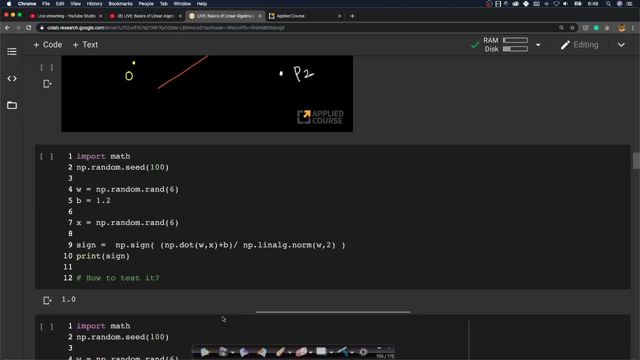 let us again, let us just do it okay. So it is very simple. It is very, very simple. The logic is also very, very straightforward. okay, Let me just erase this. The idea is as follows: So I am just generating again a random vector, a random vector- w and b. 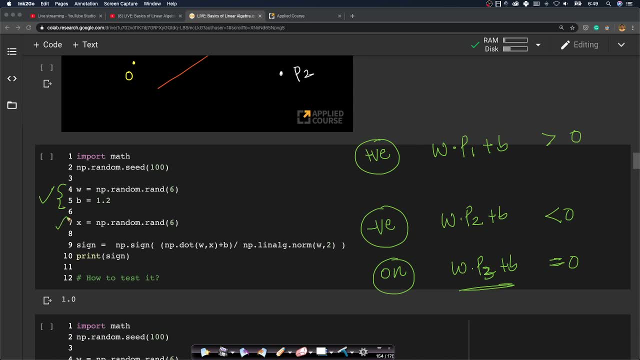 So this generates a plane pi. So both of them generate a plane pi. I am generating a point x, right, Just randomly. right Now I am saying: okay, what is the formula here? Dot, product of w and b. sorry, w and x plus b divided by norm of w. Oh sorry, I forgot to mention this. Okay, So 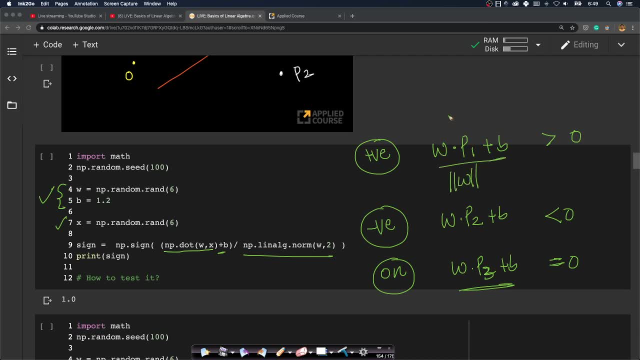 this by norm of w. I keep assuming that w is a unit vector, right? So the right thing is, if w is not a, if w is not a, not a unit vector, you have to divide it by norm w. But again, this division does not change the sign. Let us not forget this division does. 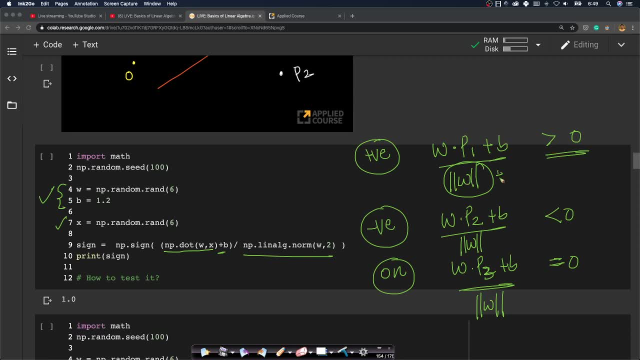 not change the sign right. That is important Because norm w is always positive, This is always positive, So this will not change the sign right, So you can actually skip this whole thing if you want. Nothing will change, okay, Cool. So by doing this- and again I am using 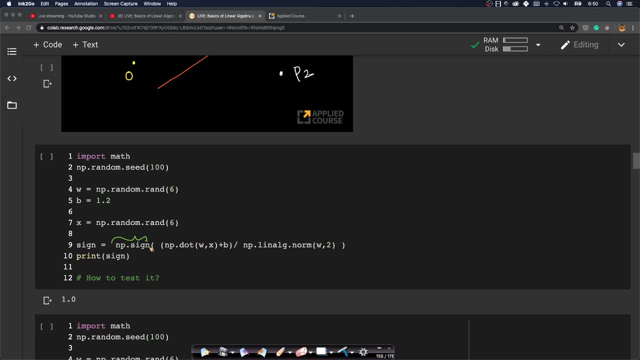 numpy sign. Numpy has this function called sign and which will give me whether it is positive or negative. okay, So I have just taken some random hyperplane, I have just taken a random point and it says that this is on the positive side. How do you test this now? Again, it is very. 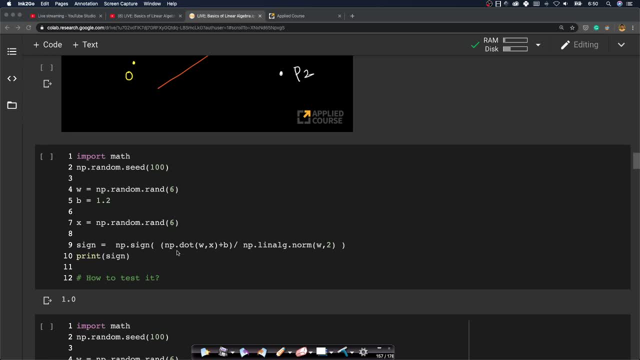 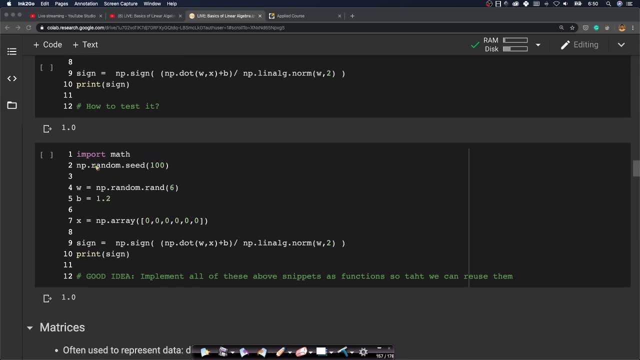 important. Whenever you write anything like this, it is important that you test it right. Again, it is very simple. If you think about it. there is a very simple way to test it. okay, The idea is this: okay, Suppose I have taken a random hyperplane like this: Look at this. I 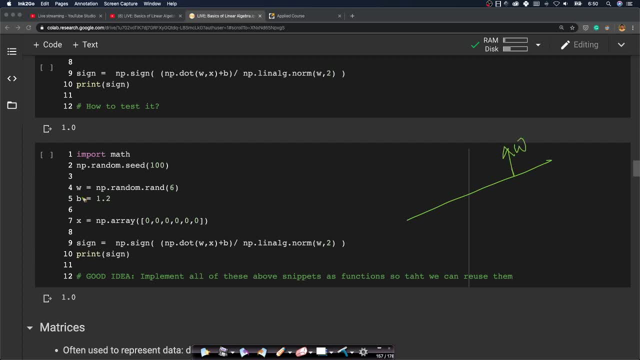 have a w right And I have a b also associated with it. My b is 1.2,. okay, If the point that I have- look at this, the point that I have- is origin. okay, Look at this, The point that I. 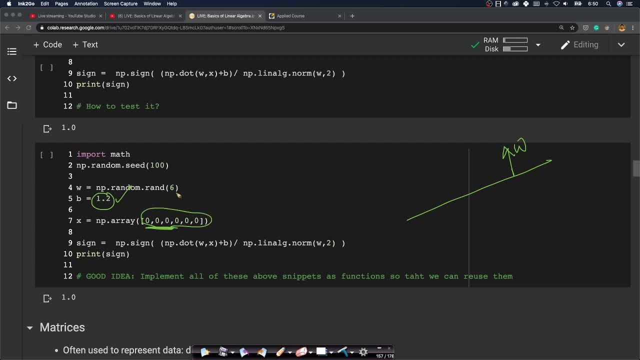 have here is origin, right? Very simply put, okay, The point that I have here is origin. Now we know that. okay, so if I plug in: if my x equals to origin, what does w transpose? x plus b will be equal to If x is origin, which means x is equal to 0,. 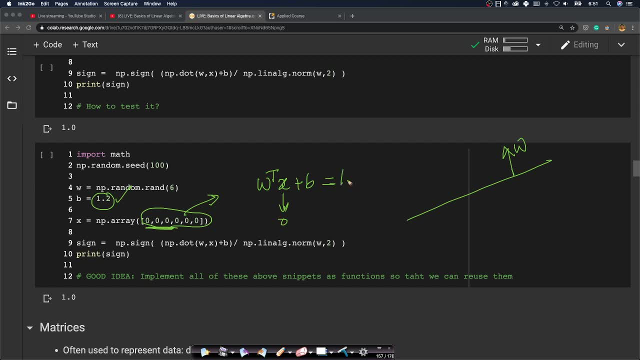 x equals to 0, w dot 0 is 0. So this will become just b itself, right? So whatever is the sign of b, look at this. whatever is the sign of b, that is the direction in which origin is. If I have, 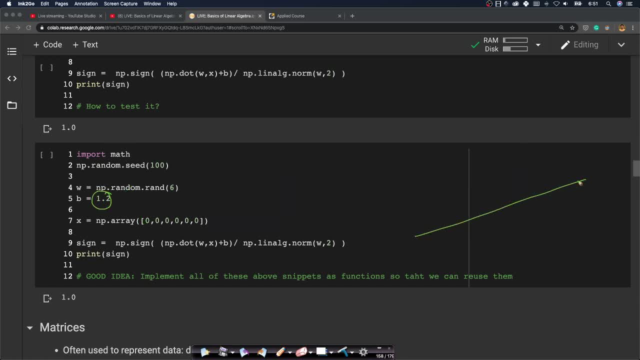 taken b equals to positive value here. if I take b equals to positive value, right? If b is positive value, my origin lies on the same direction as my w. If b is negative value, then sorry. if b is negative value. 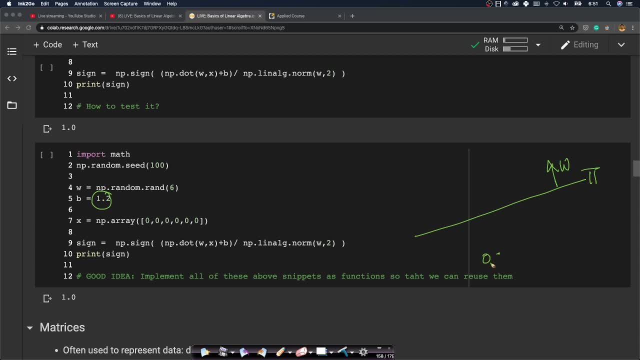 then my origin will lie in the opposite side as compared to w. Very simple concept. So for test cases, you can use these boundary cases to test if everything is working all right. So if I choose b as positive value, I get positive. If I choose b as negative, I get minus. 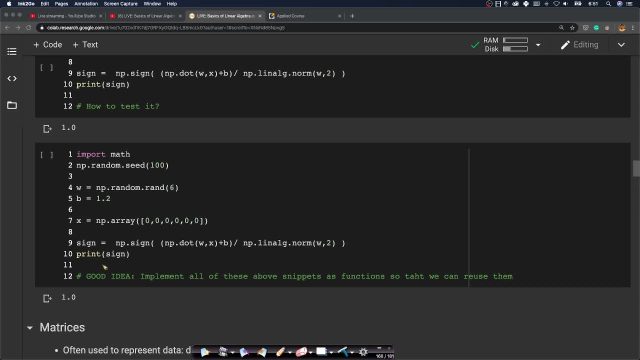 1. Again, it's always a good idea. all the functionality that we are writing, whether it is distance between a point and a plane, all of these things- try to implement all of these snippets as functions so that you can reuse them in the future. right, I'm just writing it as: 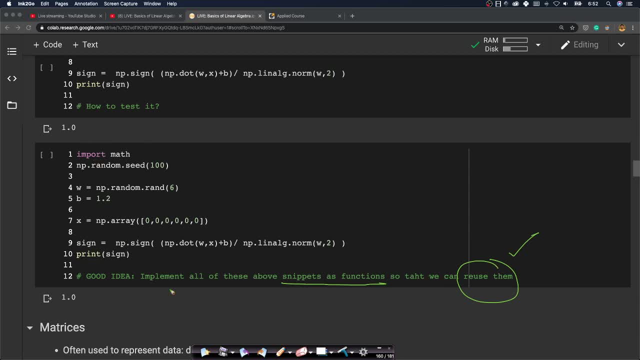 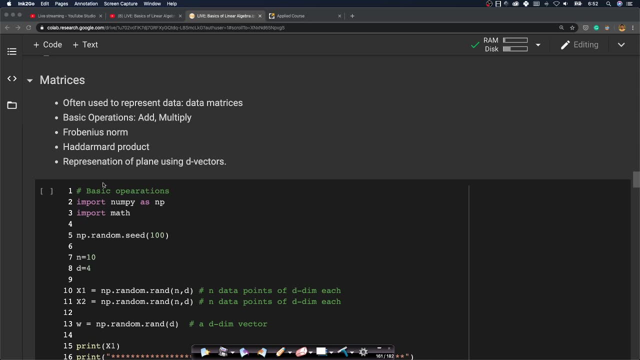 simple code just to show you right. Very simple concepts, nothing very fancy. Now let's go on to some simple matrices. okay, with the basics out of our way Again. one of the biggest applications of matrices, right in whole of data science, is to represent data matrices. Again, we'll see what. 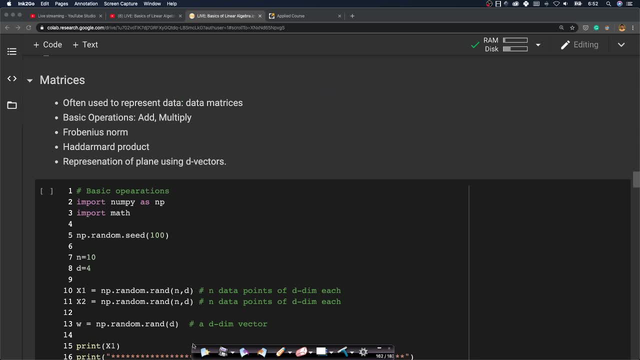 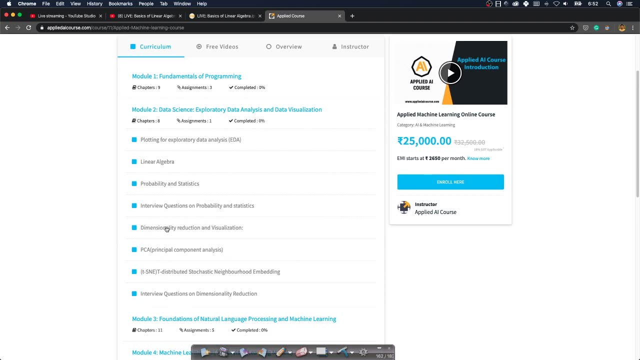 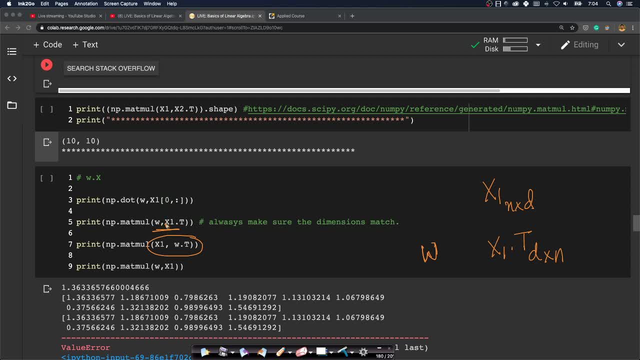 there is this chapter called as dimensionality reduction. If you just go to our course videos, go here: linear algebra. okay, so here w in numpy, the w is represented as one cross d, one row, and so it's not represented as a column vector. this w here in numpy is represented as a row vector, so one row and d. 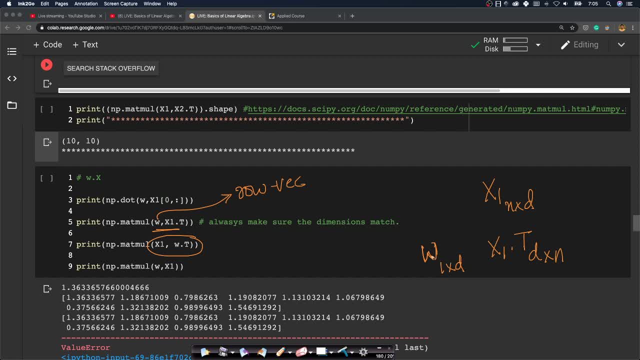 columns. so that's why, when i do a dot product between, so when i do a mat multiplication between this and this, this is working. this will work right. remember, if w is a row vector of one cross d, this will work right. so when i print this, i get this answer. now just check. just check the first value. 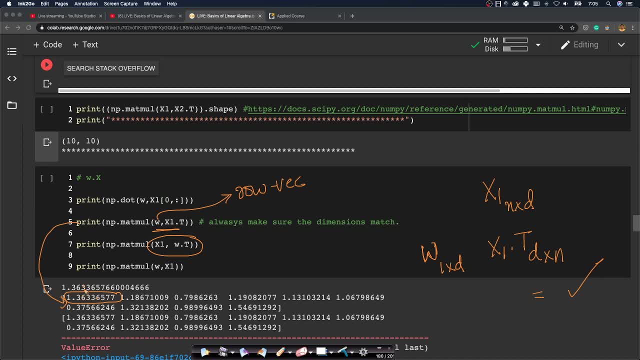 that we get here. this value matches this value as it should. this value and this value should match right, because obviously the first row when i multiplied with w, i got this result. that result should be the. in the output also, the first cell should be that value. now i could have written: 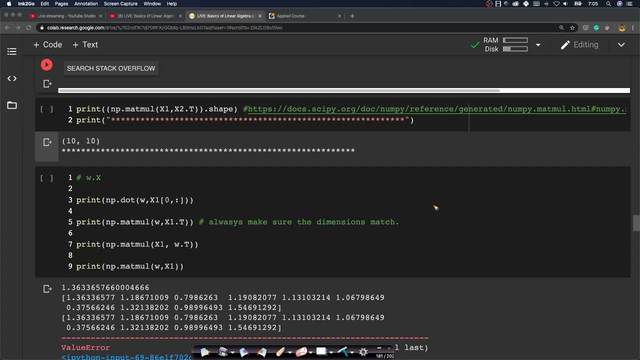 this differently. also look at this. if i wrote it this way now, what is x1? my x1 is n cross d, my w dot transpose. okay, so my w dot transpose is: so my w is one cross d, so w transpose is d cross one. now this will also work. so whenever you are doing this, just make sure whether w is a row. 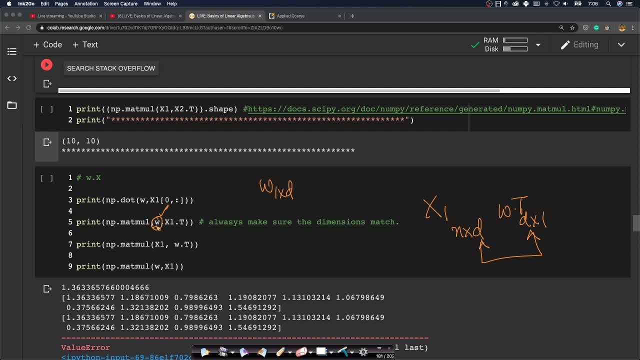 row vector or a column vector. just make sure numpy uses row vectors. mathematics guys use column vector by default. that confusion can kill you, right, i've seen. i mean, this is a very common problem. people try to do this. suppose if i just did this, this will throw an error, because w is a one cross d, x1 is an n cross d, so this will throw you an. 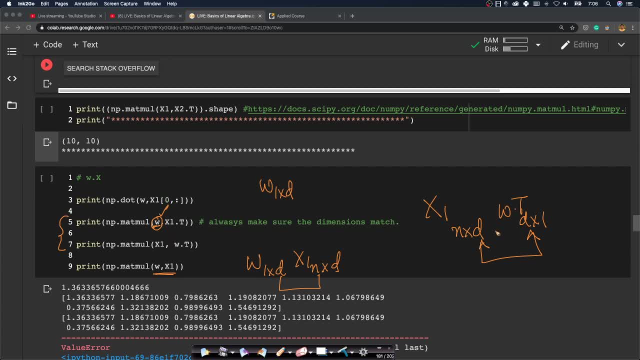 error. so the moment things throw an error, just make sure that you write what it is. it's always important when you're translating this into equations, always check for this sanity. i mean, i do it even today, after many, many years, whenever i'm writing matrix multiplication, because this 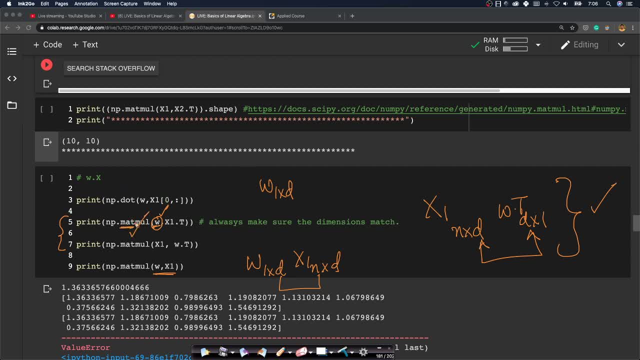 is one of the most commonly used things, whether it's matrix multiplication or tensor multiplication, right? please make sure that you don't mess up these dimensions, right? so whether you write it this way or write it this way, you get the same result, but the moment you write it this way again, 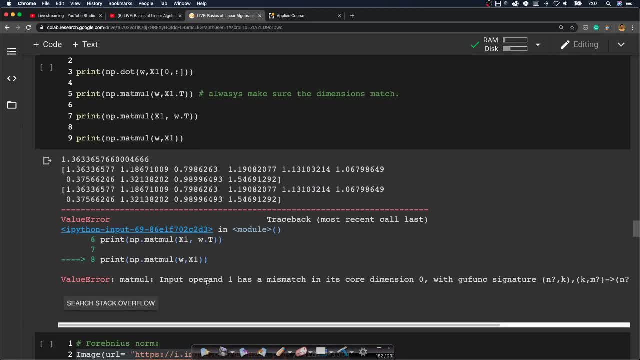 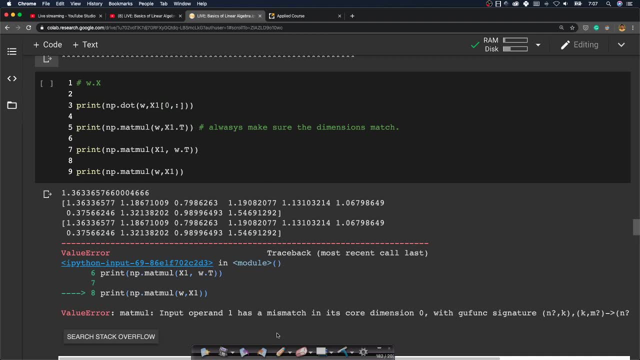 you get this very common error, which is okay: input operand mismatch in dimensions. basically, this is a typical error that you get the moment you get this. make sure to write these equations. very common mistakes that people do is they don't write these equations, they don't write this and 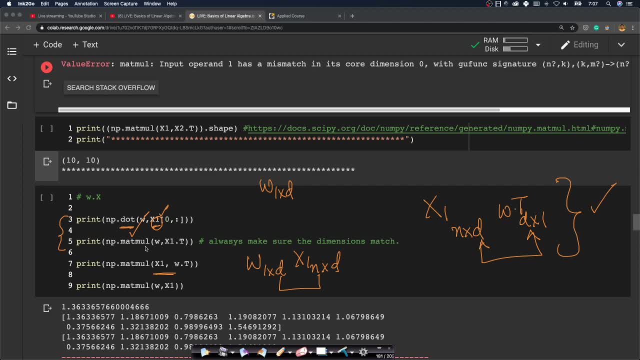 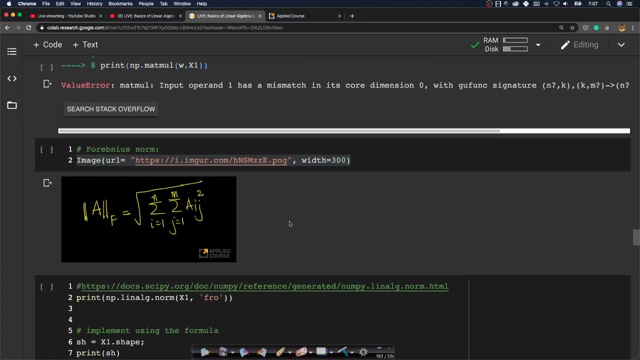 clearly understand whether w is a row vector or a column vector, or a column vector or a column vector as represented in umpire, and mess up things. very common mistake, so please be careful. okay, then there is this concept called as frobenius norm. okay, frobenius norm. this again, this is one fancy. 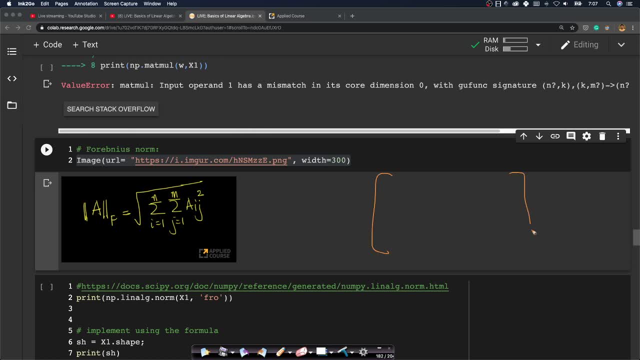 name given. what does the frobenius norm actually mean? imagine: imagine i have multiple entries in a matrix a. suppose i have a matrix a and i have multiple entries. i take each entry here. look at, look at what we do in l2 norm given a vector. look at this: if i'm given a vector, what do we do? we 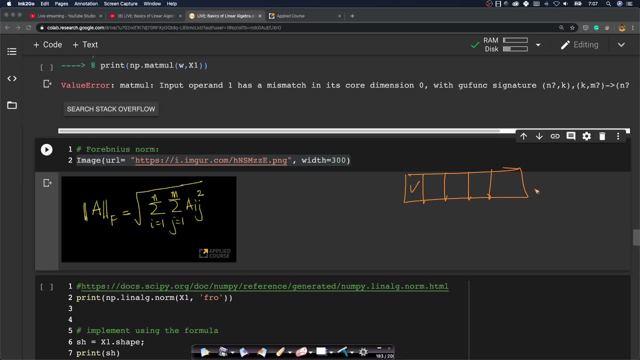 square each of the vectors and then we divide them by the number of vectors. we divide them by the number of vectors, the elements: we square each of the elements, right, we sum up everything and we take square root. basically, that's, that's what is your l2 norm. right, that's what is your l2 norm. 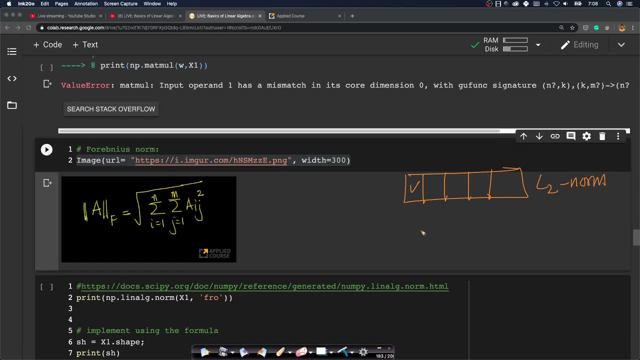 so the same concept of l2 norm. if you extend it to matrices, what do you get? take each of the elements that you have in your matrix. suppose if my matrix is a. suppose if my matrix is a right, take each. so i throw jth column, i throw jth column. this cell is called aij right. this cell is: 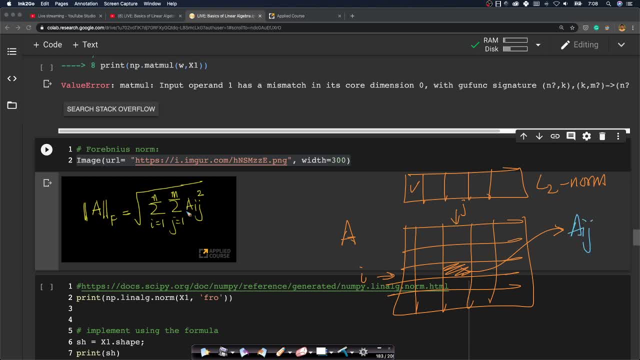 called aij right? very simply put so, for all i and j, i goes from 1 to n if you have n rows. j goes from 1 to m if you have m columns. if this matrix is an n cross m matrix, take every element, square it. 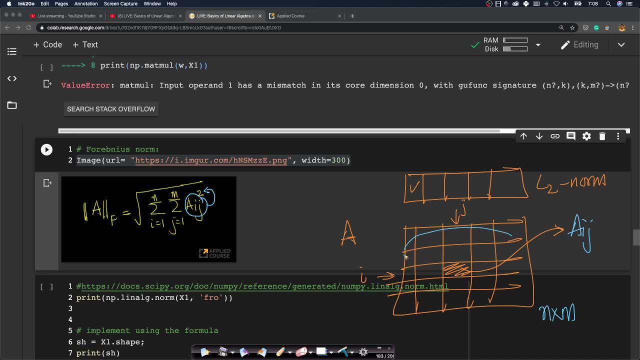 sum this up across all the rows and columns. basically, you're taking all the elements that are there in the matrix, taking the square and summing up all of them and you're taking the square root of it. that's what is called the frobenius norm. again, this definition is valid if. 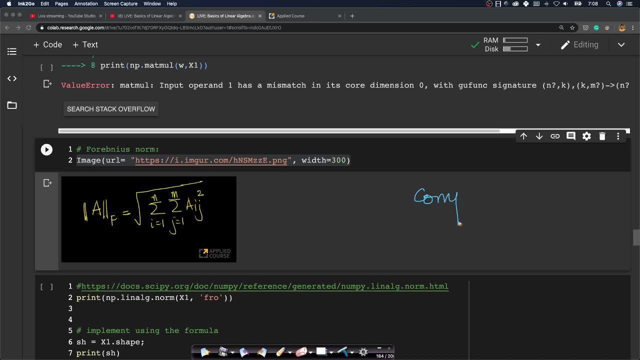 you have real numbers in a matrix. there are complex matrices that we do not encounter much in machine learning, but complex matrices are used in electrical engineering, electronics engineering, even mechanical engineering, etc. right, so if you have a complex mat, what is a complex matrix where the entries can be complex numbers, right? for example three, uh suppose complex numbers, right we? 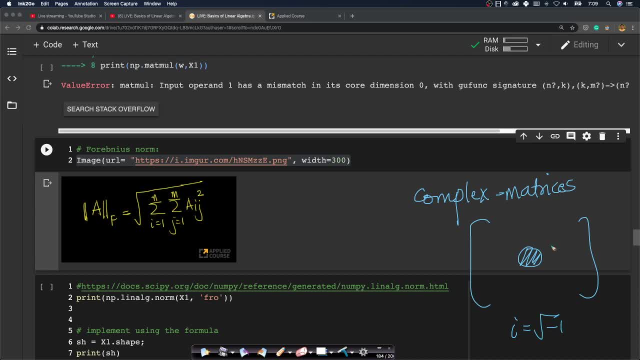 know i, which is square root of minus one, right. so complex numbers have a real component, for example right. so frobenius norm can also be defined on complex matrices, wherein the definition is slightly different. but we do not use complex matrices much in machine learning, but frobenius. 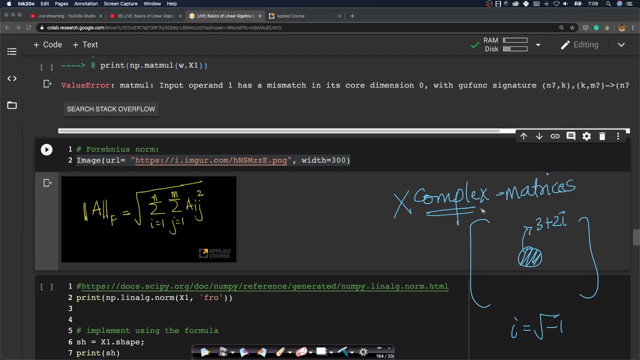 norm is a concept in linear algebra. again, remember, linear algebra is used in many, many places, not just in machine learning. ai. we are limiting ourselves to the discussion in the context of machine learning and ai. right again, frobenius norm is used in machine learning for some errors. 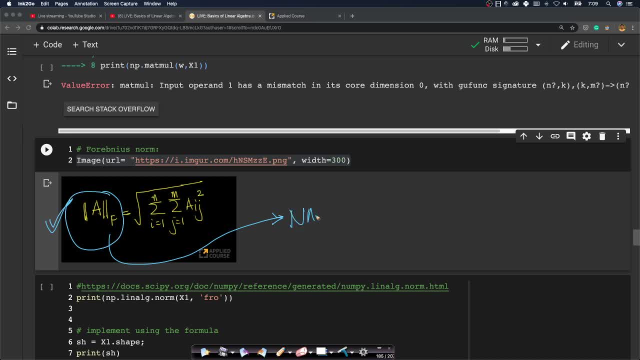 we actually use the frobenius norm in our course videos when we learn about non-negative matrix factorization. okay, there is a whole, there is a whole chapter called recommender systems where we learn about the concept of non-negative matrix factorization, which is again a concept that is also taught in some linear algebra advanced courses. 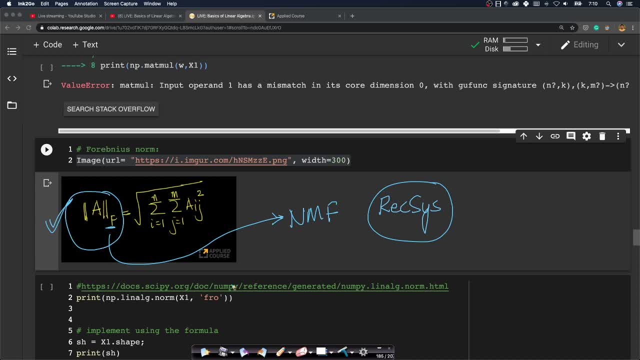 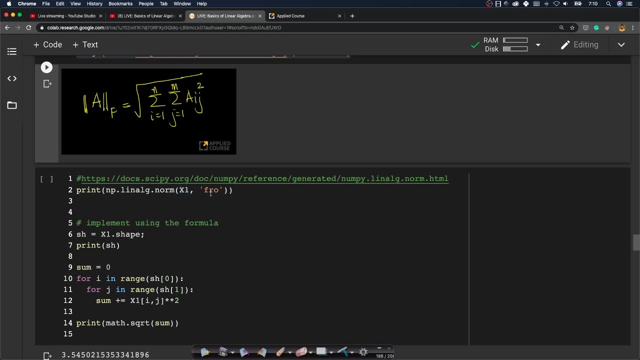 where this frobenius norm is encountered. i'm just connecting the dots for you, right? so i can get frobenius norm very easily. look at this: if i have, if i have a matrix x1, i can get the frobenius norm by just using the norm, because we saw this definition earlier, right? so the 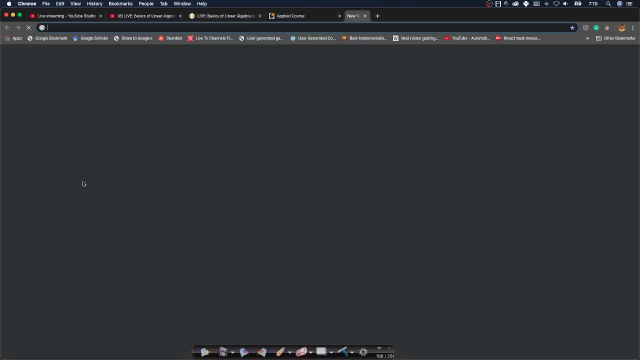 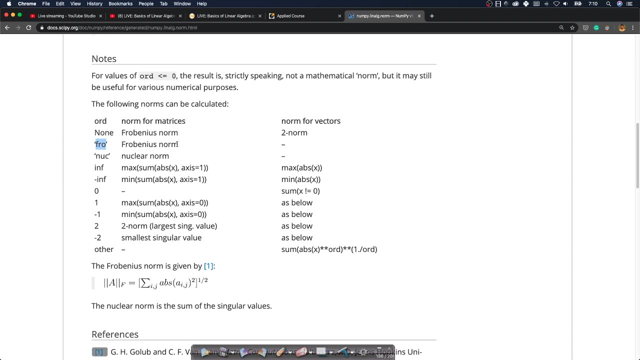 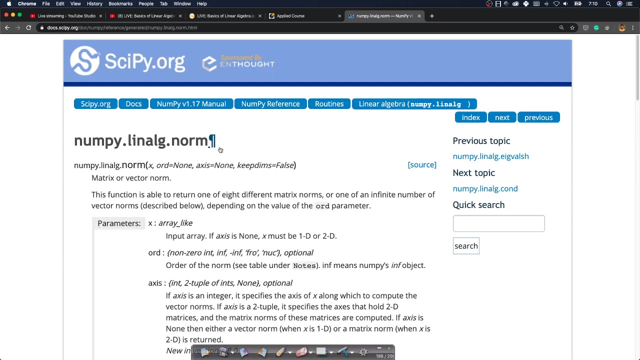 linear algebra norm in numpy can compute lots of norms. we saw that a while ago, right, so the linear algebra norm can compute lot of norms. if i just give fr row, it computes frobenius norm. if i give 2, it gives 2 norm. right, so this norm can compute norms on vectors as well as matrices. 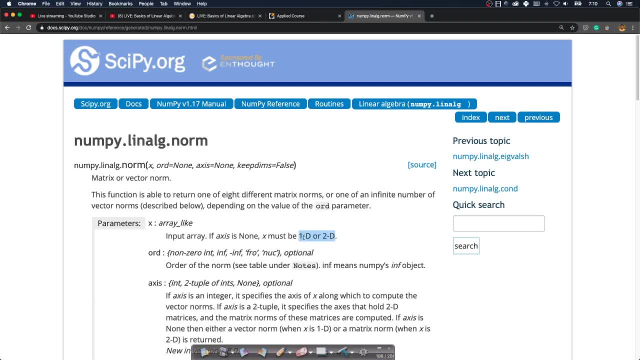 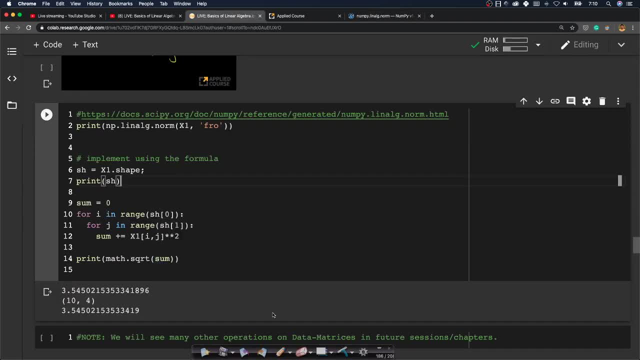 right, it can be 1d or 2d. look at this: x must be 1d or 2d, not for tensors, right? so what do we do now? we just say frobenius norm, we print it. what value do we get? look at this: we get a value which is 3.54. but let us also implement it again to understand a concept. 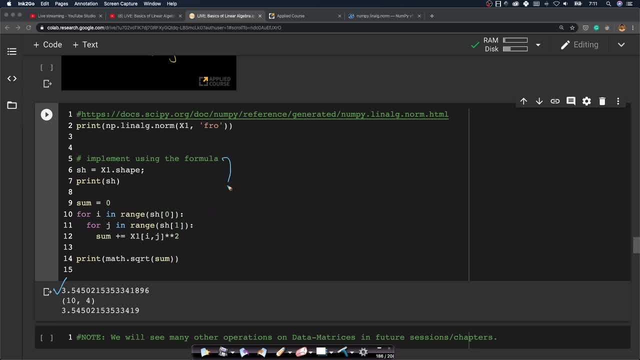 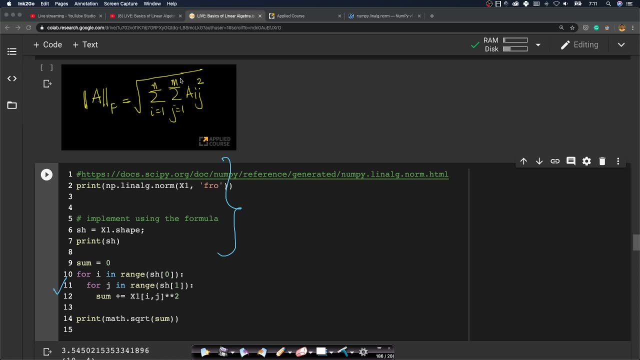 in depth. it's always a good idea to implement it. so i'm implementing the formula here. what does the formula say? the formula is very simple. it's right above here, for all i, for all rows, for all columns. take the square of each of them, sum up everything and put in a square root, right. we have seen how. 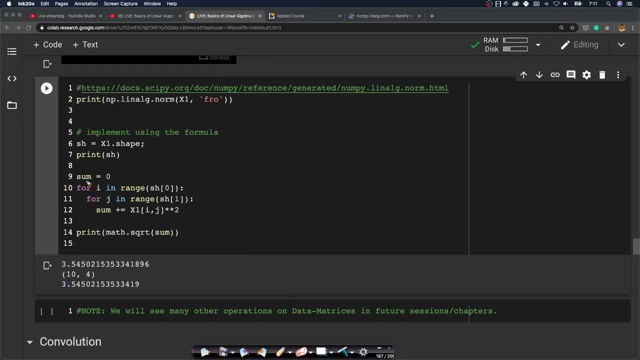 to do simple for loops right in in the previous sessions. so i just so i get shape. so, given x1, i am printing the shape. x1 is a 10 cross 4.. we know this. x1 has 10 rows and 4 columns. we know this. 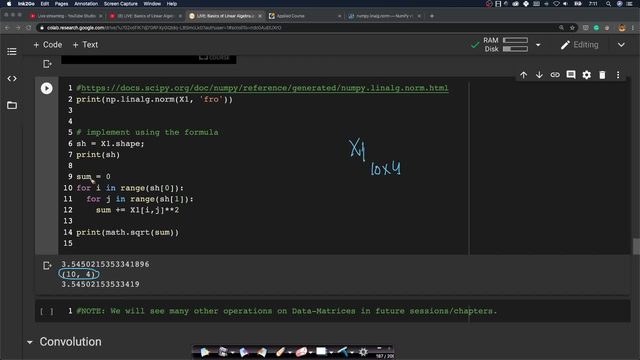 already because we just created a random matrix like that. i am creating a sum here for i in this right, but when i say x1 dot shape, what does it give? it gives a tuple. always remember what is the data type that is given. i get a tuple. so if i take sh, sh 0 should give me the number of rows. 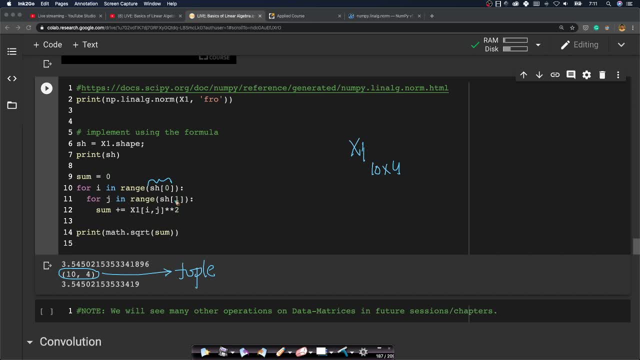 so what am i doing for i in rows, for j in columns, because i'm using sh 1 here. all i'm saying here: to this sum: keep adding x, i, j square, just keep adding x, i, j square. now, at the end, i just take the square root and print it. i get the same value here, except for small rounding. 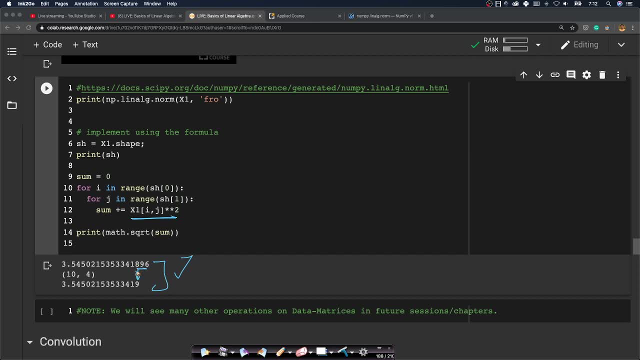 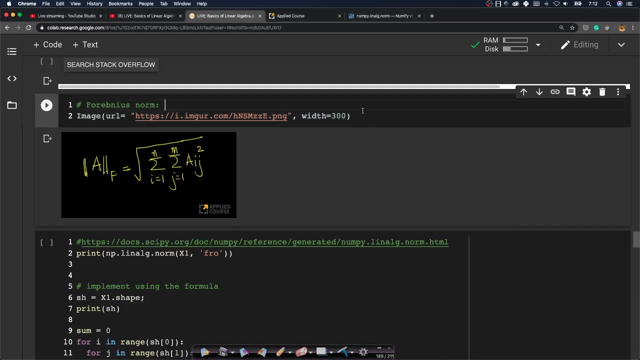 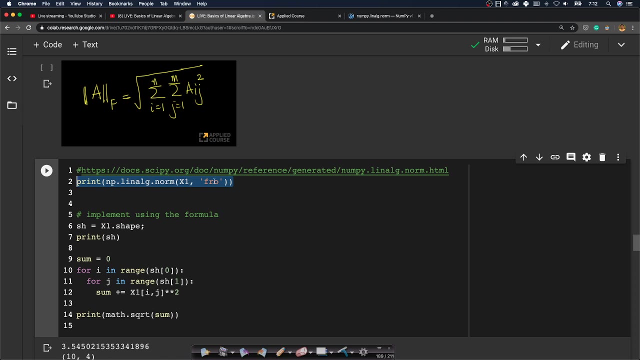 error, right? so this is 896. this is rounded to 1, 9, right? so whenever you have a concept like this, it's also a good idea to implement it so that you understand better the concept. it's always a good idea and, of course, in practice, when you are writing production quality code, i would rather use this: 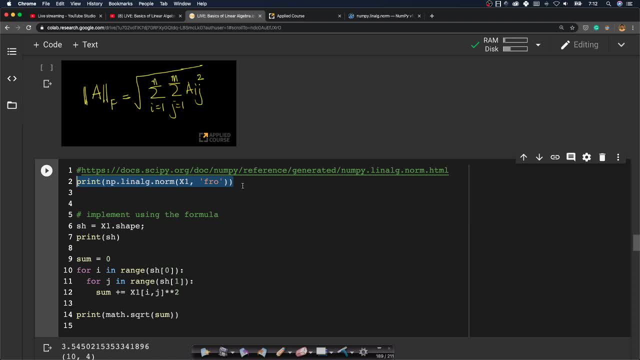 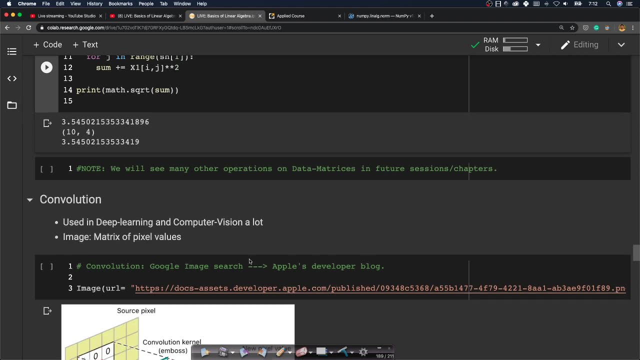 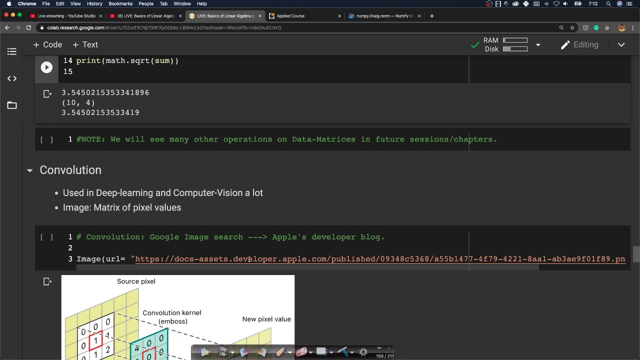 instead of writing my own code, because, as we have shown earlier, this is going to be slower than inbuilt code, because inbuilt code is optimized using c, c plus, plus in numpy, cool. so the next operation that we'll go into is convolution, right? so, yeah, somebody is asking about, uh, yeah, where we use frobenius norm formula in machine learning. 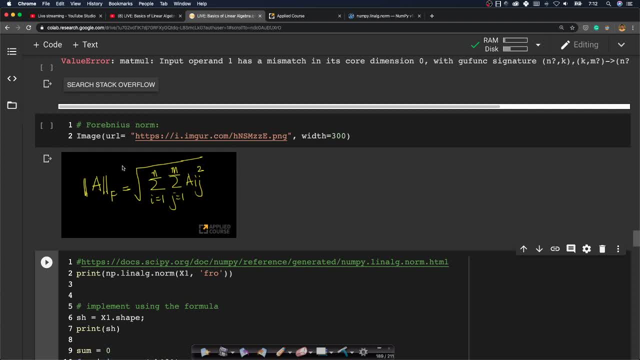 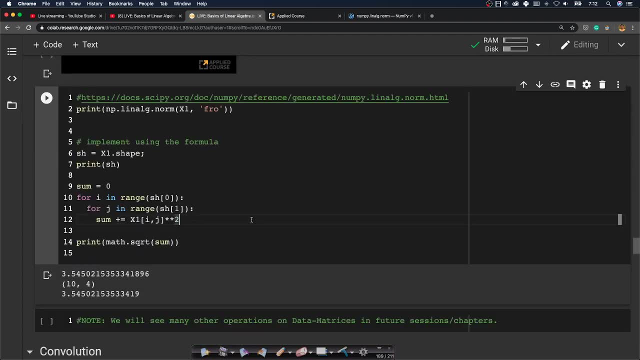 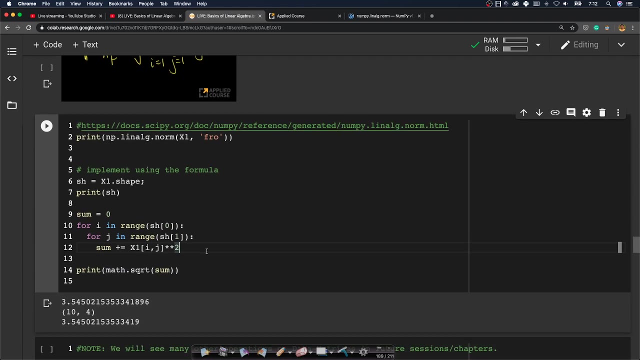 i just mentioned this a while ago. right, we use it in non-negative matrix factorization, cool. so what we're going to do is we're going to use the frobenius formula. what is one digit? i didn't get what one digit you're talking about, why we are getting one extra digit in. 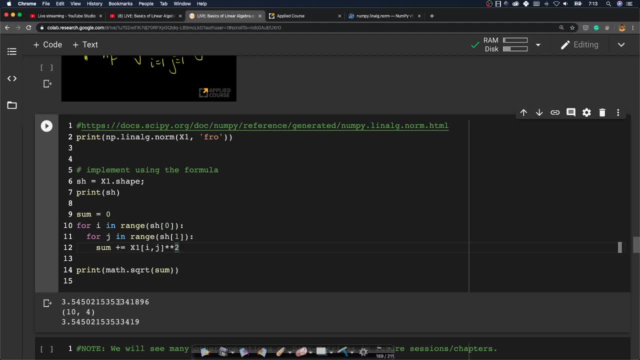 in the frobenius formula. again, you can. you can all this. if you want more digits in the decimal value, you can always get it right. so this print is just rounding it off and printing it. you can always get more digits if you want. that's not a problem, cool, um, okay, by default w is a column. 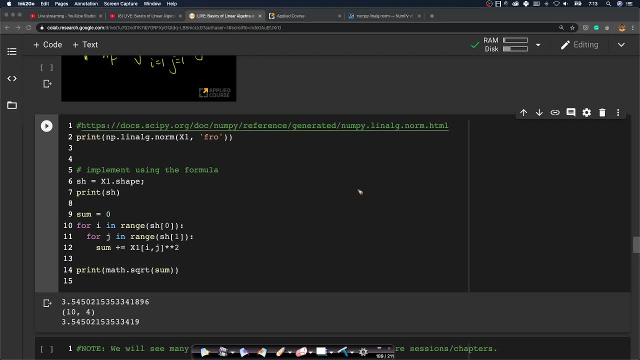 uh, importantly, in whole of again, there is this dichotomy that w in mathematics is always taken as a column vector right in mathematics, in most of mathematics. but please also remember that it depends on the implementation, the way. a numpy again. how would we represent w here? you, we represented. 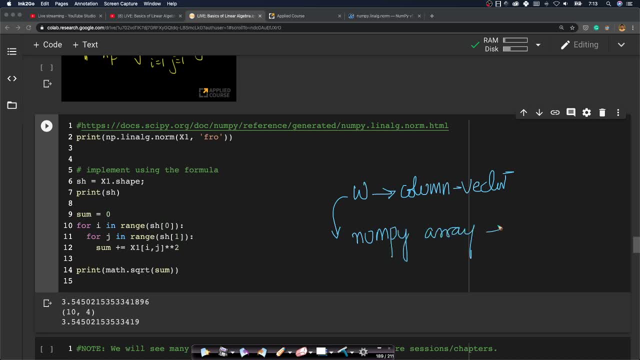 using numpy array. numpy array creates a row vector by default, not a column vector, because it is trying array, not a vector. remember: numpy does not have numpy. what we, what we used, what class did we use or what object did we use to represent w? we are using numpy array. numpy arrays are row. 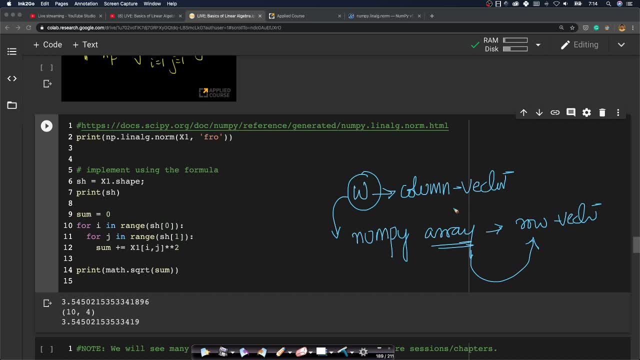 vectors by default. so we just have to be careful with the dimensions when we are writing numpy based code. that's it. otherwise, mathematicians, or even in our course videos, we assume that all vectors are column vectors by default. right, so? okay, sounds good. okay, so let's go to convolution. i just wanted to show you the power of matrices. 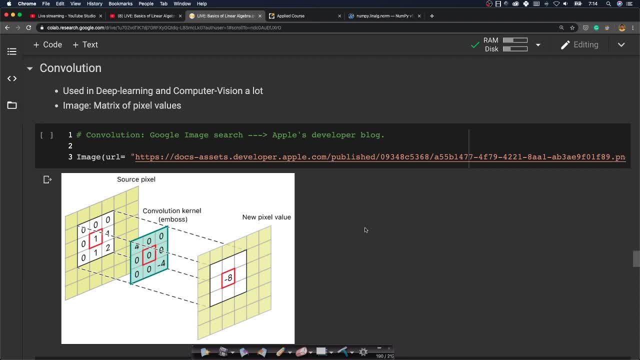 in the context of image processing. again, please understand that this is not whole of image processing. we are just touching the iceberg. i just wanted to show you an application so that you can connect the dots here. convolution as an operation is used extensively in in whole of deep learning. 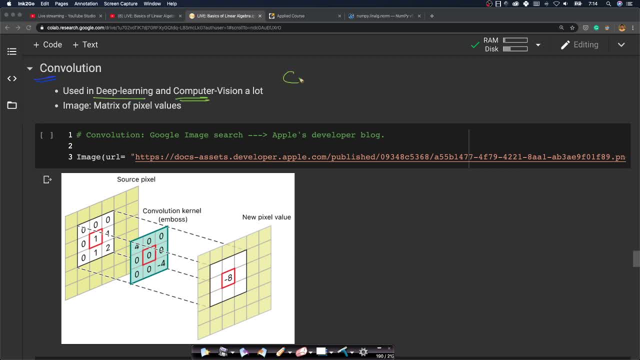 and computer vision a lot. again, there is a whole network called as convolution neural network, which is based on the operation of convolution, but convolution as an operation is actually studied in signal processing. look at how the whole thing is connected. it is the electronics engineers and signal processing guys who actually came up with the concept of convolution, right? so the image. 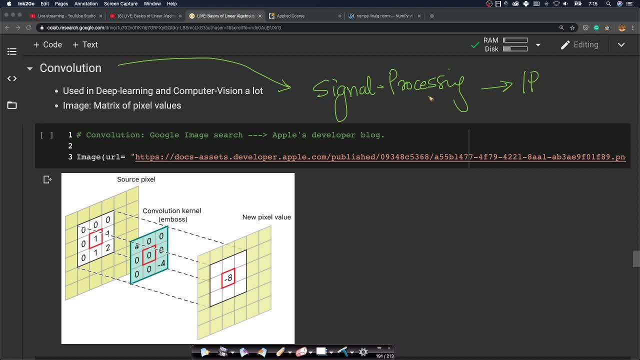 processing guys, right, the people who are doing image processing work. they borrowed this concept from signal processing. the concept from image processing was taken to computer vision, which is now used in deep learning. convolution- again, the convolution operation, from signal processing. they also borrowed it from applied mathematics, from linear algebra. okay, they borrowed it partially from linear algebra, partially. 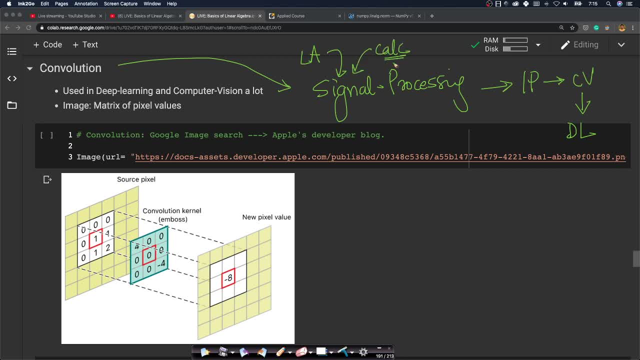 from calculus, right? so the signal processing guys who know signal processing, the many ways of looking at convolution, right? so here we look at something called as discrete convolution, or we look at convolution in the context of image processing and computer vision, not from a pure signal processing perspective. that's a different beast altogether. 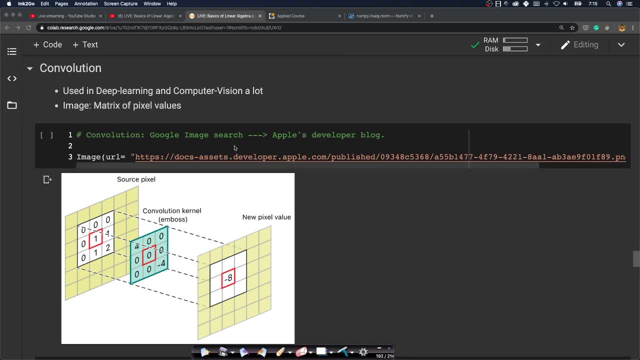 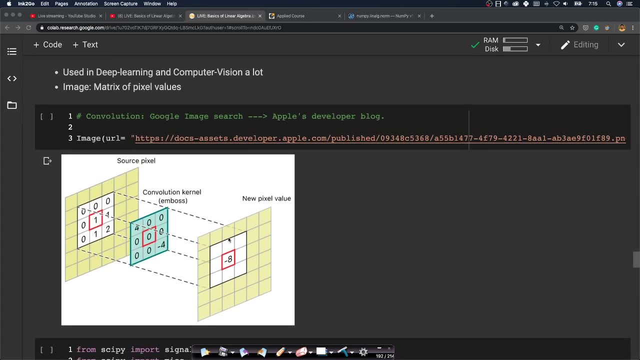 okay, so let's, let's look at this, right? so what does convolution do? again, i'll show you a very simple example of convolution, how it's powerful, but i want to explain the power of matrices in the real world, right? so let's, let's look at a very simple example here. cool, uh, let me use this, okay. 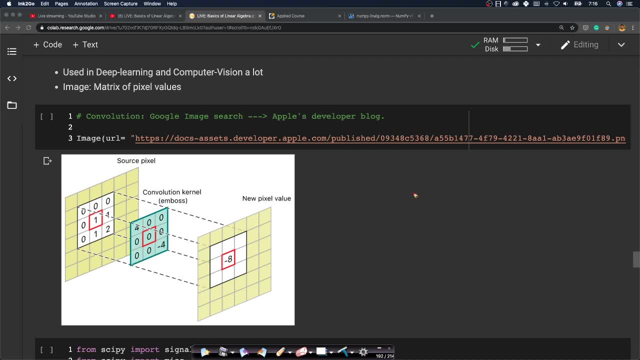 suppose, imagine if this is my image. what is an image, effectively? let's take a. let's take a simple black and white image, also called as grayscale image, right? so let's take a simple image. color images we learn later. okay, it's slightly more complicated. let's 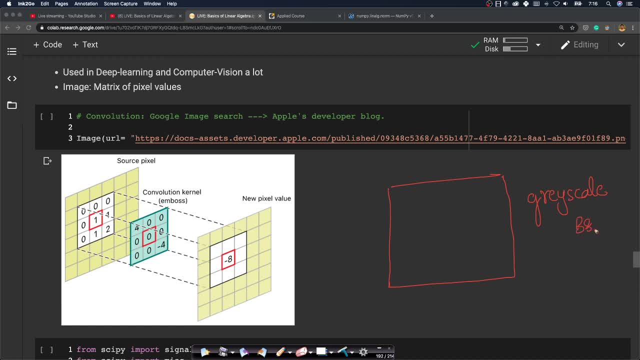 take the simplest grayscale or black and white images, as as we often refer to them as in colloquial english and india, but they're technically called grayscale images. an image is actually a bunch of rows and columns. an image is actually a matrix. an image is basically a matrix. 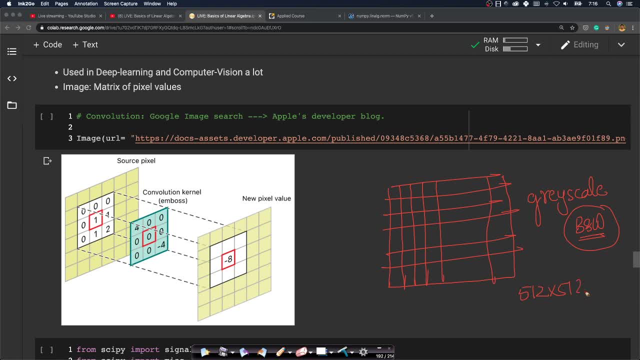 suppose, if i have an image which is 500 of size, 512 cross 512, what it means is i have 512 rows and i have 512 columns, and each of these cells contain a value which says how bright this pixel should be. this is what is called as a pixel. right, each of these is called a pixel. this is how. 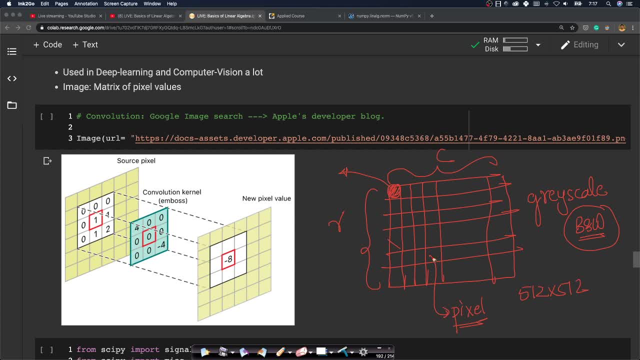 your monitors, your screens, everything also work. each of these is called a pixel. if you have a grayscale image, which means you have a, you have, you don't have color here- each of these values each of this. so a grayscale image can be represented as a matrix where, if you have an image of 512 rows and 512 columns, or this is the image size- 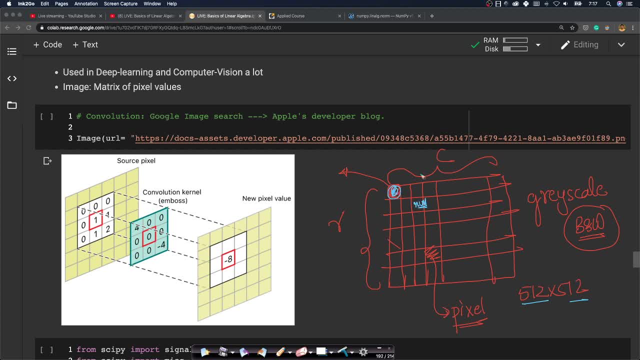 every cell has a number. every cell has a number inside it, so you can actually think of an image as a matrix, and all the beautiful mathematics of matrix algebra can be applied on images for image processing and computer vision. one such operation is called as convolution. okay, convolution is a very beautiful operation. it can do a lot of things. okay, we'll look at one simple. 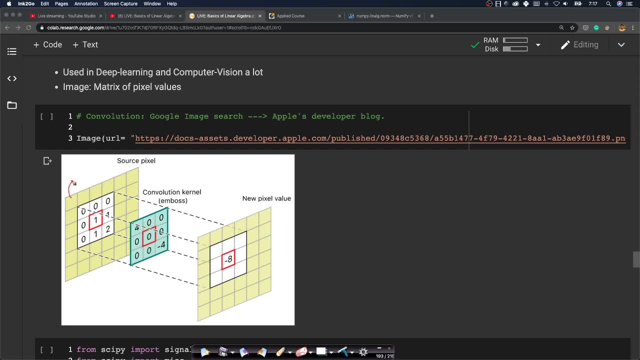 example, suppose. imagine that this is my image. okay, so again, just to give credits, i've taken this image from the apple's developer blog. it's again. i try to use all the urls here so that i'm fully transparent about it. i did not draw this, okay. so other diagrams: yes, i drew them and i put it here. 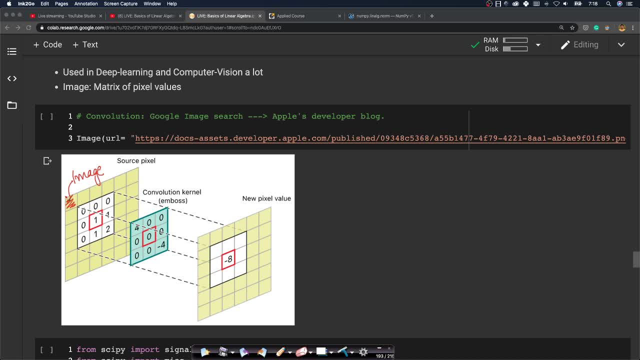 so imagine if i have this image. each of these is a pixel in image. let's say you have a grayscale image, we'll see how everything works if you have color image. when we learn about tensors, when we learn, learn about convolution in the con in the context of tensors, etc. that we'll see later, right? so if 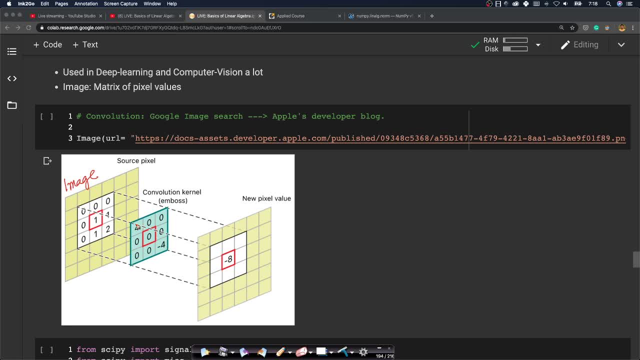 this is my image, and each of these is my pixel. now this thing is called as a convolution kernel. a convolution kernel is also an other matrix. look at this, this is my image matrix. right, let's call it as img. okay, i have something called as a kernel. it's also called as a convolution kernel. 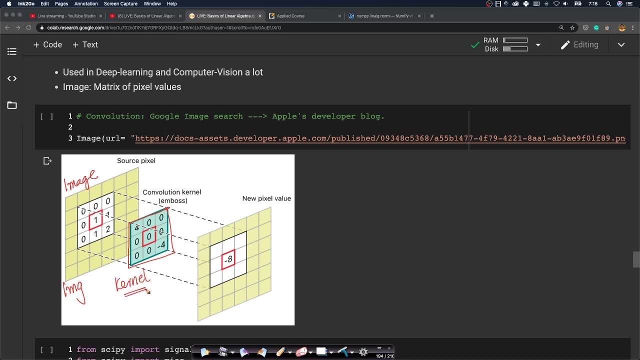 okay, so please don't confuse this kernel with kernels in svm. those are different concepts. this name came from image processing, okay, so remember that a kernel is a smaller matrix, right? so you again, let's assume this kernel is a k cross k matrix, right? my kernel, let's assume, is a. 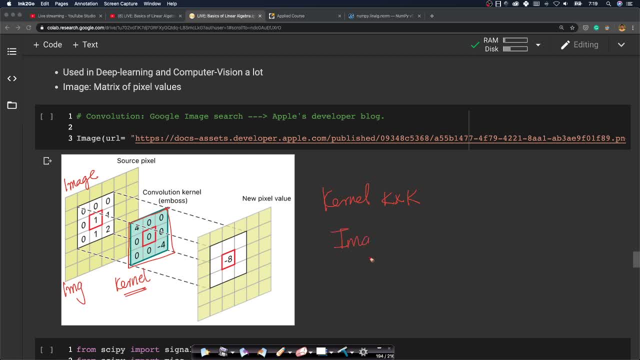 k cross k matrix. imagine that my image is, let's say, some d cross d image. okay, d rows and d columns again need not always be same dimensions, but i'm just taking it for simplicity. now, what does convolution operation do? so convolution operation, it's also called 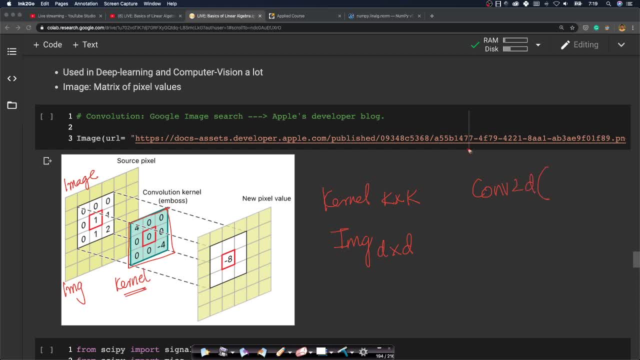 as 2d convolution, because there is a concept called 1d convolution. also there is a concept called 3d convolution also. first let's look at 2d convolution. we learn about others when we learn tensors, etc. in deep learning we learn all sorts of convolutions. so conf 2d takes an image right. 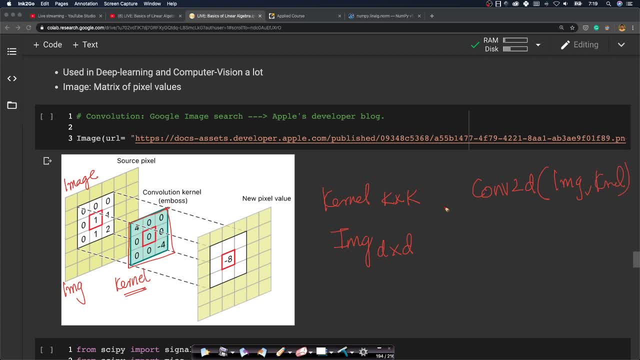 and it takes a kernel. it takes a kernel as input and it generates an output. again. this is my output here. look at this: this is my output. and how does it generate the output it takes? look at this: suppose right, corresponding to this pixel. look at this: my kernel here is 3 cross 3 corresponding to this. 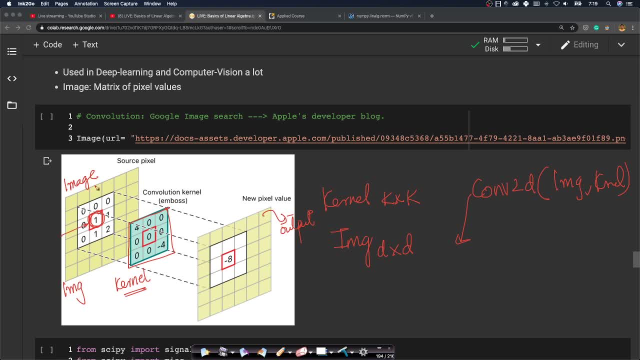 pixel. look at this. this pixel is third row, third column right. so it takes one pixel here. third row, third column right. it takes all the pixels that are around it. look at this. it takes all the pixels around it, right. cool, now it multiplies again. i have a kernel here, right. the kernel is sort of: 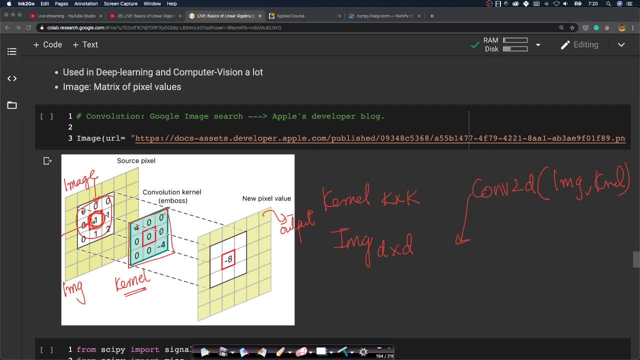 fixed kernel. i might. i do the hadamard product. what is the hadamard product? i do. i look at this, i do this. multiplication, like this element, wise multiplication. so 0 multiplied by 4, look at this. so 0 multiplied by 4 is 0. again, 0 multiplied by 0 is 0, 0 multiplied. 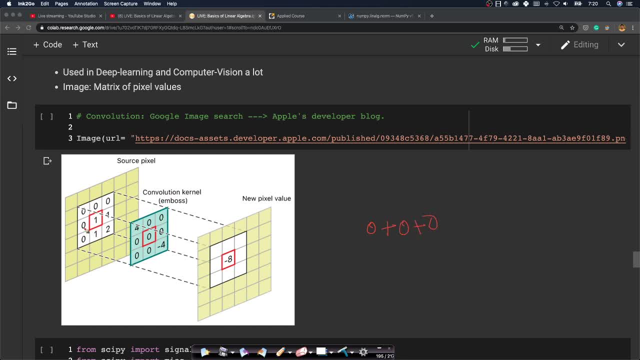 by 0 is 0. so first row i have multiplied. let's look at second row: 0 multiplied by 0 is 0, 1 multiplied by 0 is 0, 1 multiplied by 0 is 0. so i get second row also all zeros. third row: 0. 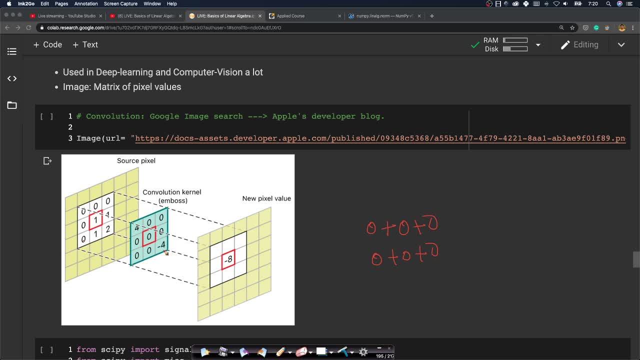 multiplied by 0 is 0. 1 multiplied by 0 is 0. 2. multiplied by minus 4 is minus 8, right, so now i, i add up all these, add up all this. so, plus this, plus this, what does it return? it returns minus 8, right, this minus 8 is present here. this is how i generate one pixel value in 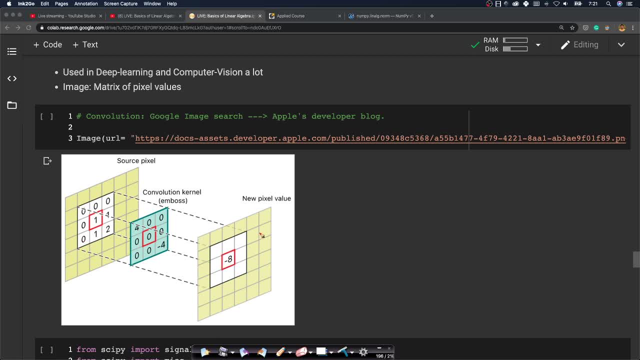 the output. now, if i want to generate another pixel value, suppose if i want to generate, let's say, this pixel value, how do i generate this pixel value? i go to the corresponding pixel here. i draw a 3 cross 3 matrix around it. look at this: this is my 3 cross 3. 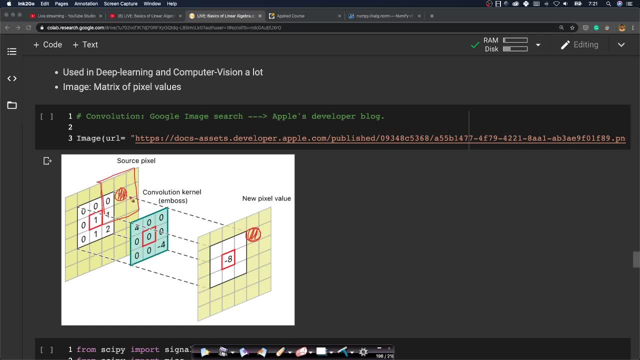 matrix. i'll do the hadamard product we just discussed, or element wise product- right, we just discussed that right now, right? so i take this 3 cross 3 matrix, i do the element wise product with my kernel and sum up all the values, and what i get here is my output. right again, the way this. 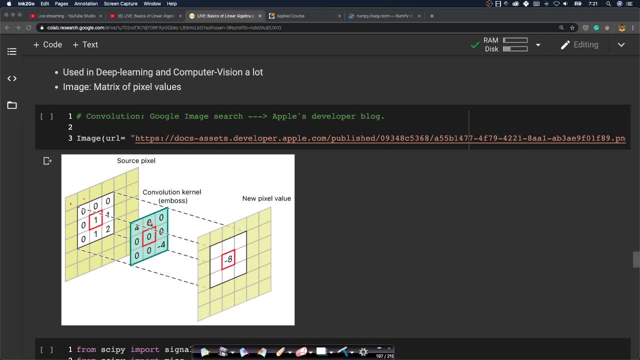 output is generated is we go from one pixel to another pixel, for on every pixel we try to put this kernel so effectively. what are we doing? on every pixel? we are drawing this 3 cross 3 grid because my output is 3 cross 3 grid and i'm drawing this 3 cross 3 grid and i'm drawing this. 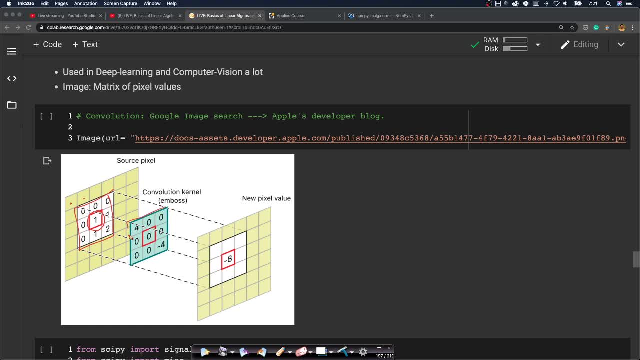 my kernel is 3 cross 3. i'm multiplying element wise with this convolution kernel and i'm generating an output. so this operation is called as convolution 2d. right again, remember what is this based on? if you think logically, this is basically based on your element wise product of matrices, because 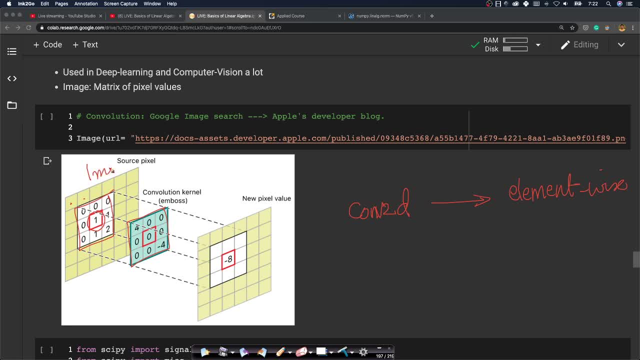 element wise product. right, you can think of this as one matrix, you can this. you can think of this as another matrix, right, you're doing element wise product and you're doing this for every pixel here to generate the output. now you might say: what the heck are we learning? why are we? 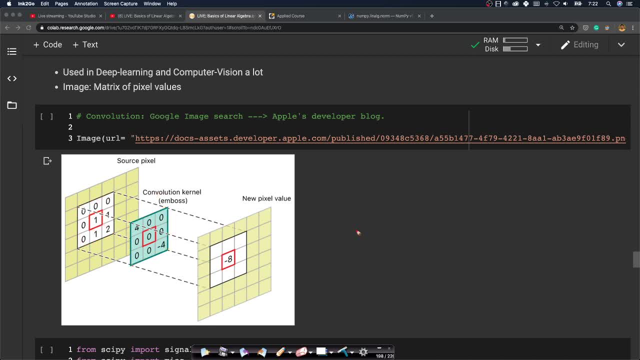 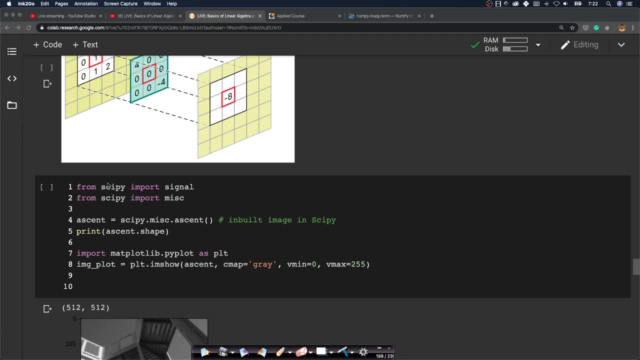 learning all this? this sounds too theoretical. i'll show you some simple application of this very simple application. let's actually take an image. okay, i've taken this example from sci-pi. okay, so i'm importing sci-pi and sci-pi miscellaneous, so sci-pi has an image called. 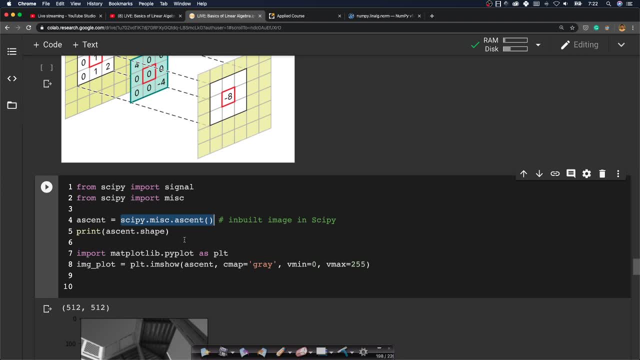 as ascent. i'm just loading an image. look at what i'm doing here. i'm just loading an image here. now, if you want to look at what is the data type of ascent, okay, let's actually look at that, right? so, print type: ascent. yeah, let's see. okay, so what, what? so i'm just loading a nd array. look at this. 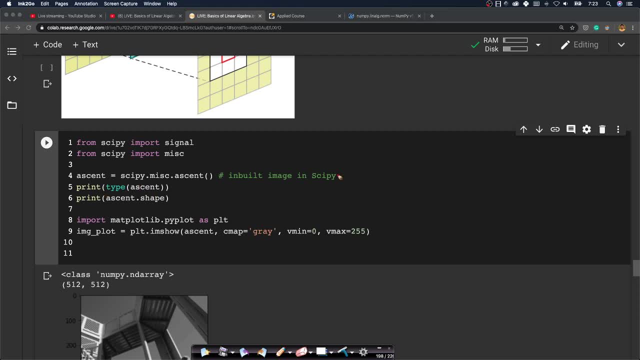 what am i loading here? i'm just loading an nd array. okay, so there is actually an image which is already inbuilt in sci-pi. i'm just loading that image. but what is that image? an image is nothing, but it's a numpy nd array. what is the shape of the nd array? fight well, cross, fight well. 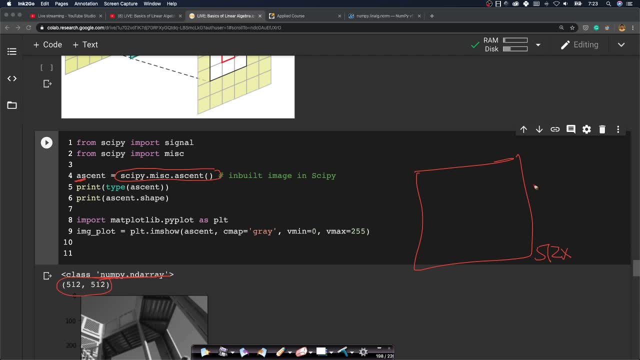 i have. i have an array which is of a two-dimensional array which is of size 512 cross 512. if i want to visualize this image, it's very, very easy using matplotlib. right again, we have discussed this in the course videos. when we learn some image processing algorithms, it's actually 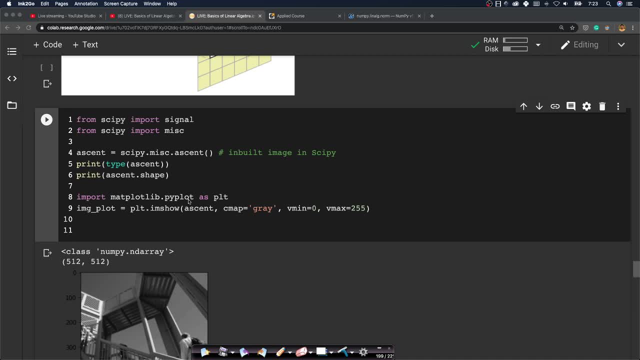 one line code. all i have to say here is: import matplotlib as plt. i just have to run this plt dot image show. so i am show is a command that matplotlib borrowed from matlab. actually i am show i actually used im show. it's been there in matlab for many, many years, right, so matplotlib. 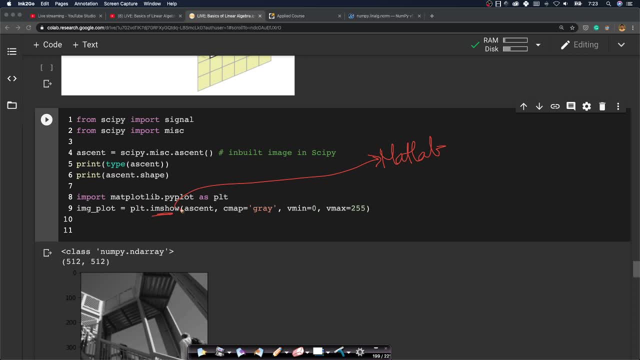 borrowed the same syntax from matlab. it's the im show function is also there in matlab, so they just use the same thing, because a lot of people who are using matplotlib used to use matlab earlier, right, matlab is a completely different tool. okay, we don't have to worry about it. so what am i saying? 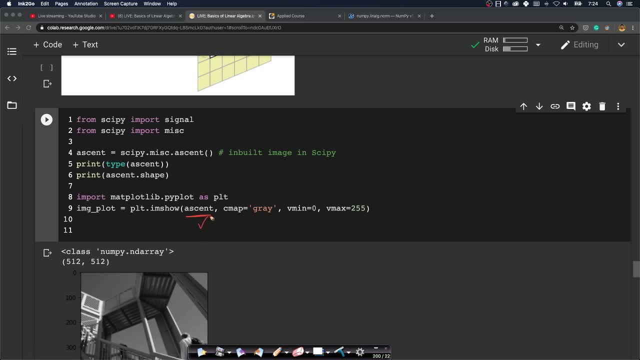 here i'm again. you can read the documentation here. the first parameter has to be: what is the image type? sorry, what is the? what is the image, what is the matrix that you want to show? you want, i am show basically means image show. right, and i want to say that the color map for 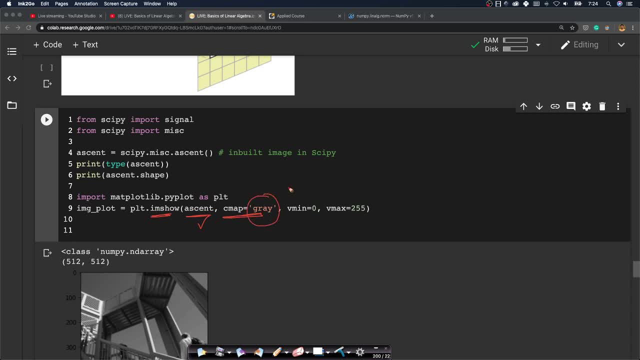 this is grayscale. this is not a color image, this is a grayscale image and i'm saying the minimum value is zero. the maximum value is 255. again, this is very specific to image processing, that in each of my values. look at this when i'm representing an image, right? so this the value. 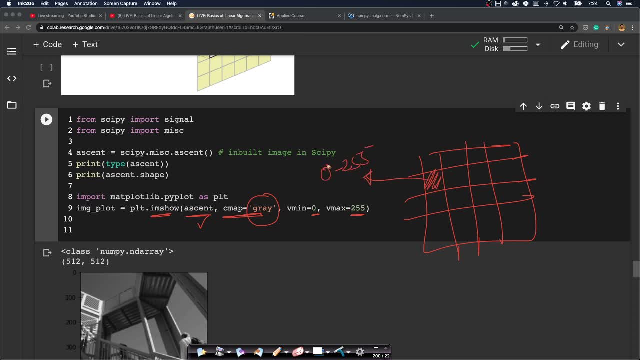 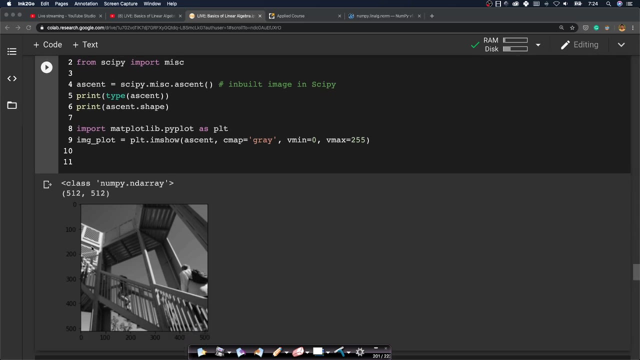 that is here, rise between 0 to 255. 0 means full dark black right, 255 means full white. that's what it means, right, so cool. so if i just do this, what do i get? i get an image like this. this is an image of a staircase that somebody is climbing onto right. very simple, very simple. 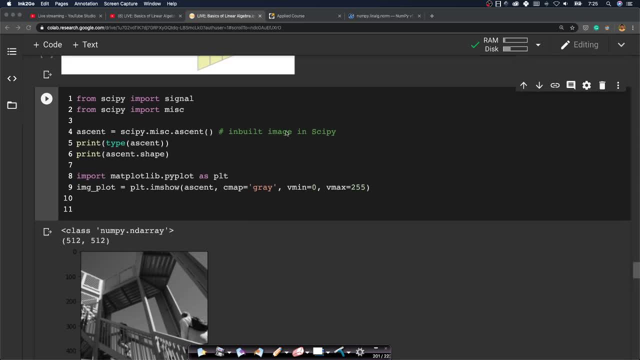 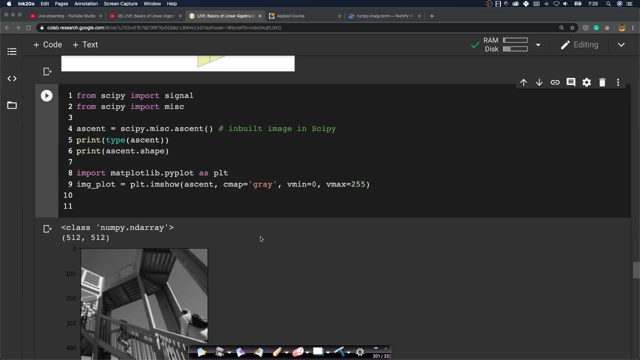 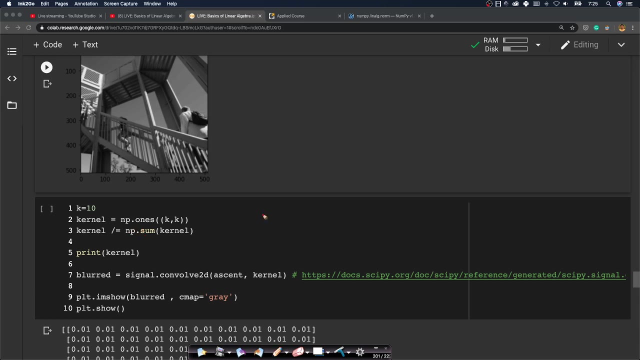 concept. so what i've done here: i've loaded an inbuilt image in scipy as a 2d array. now let's apply a very simple convolution operation. okay, so first let me create a convolution kernel. okay, again, there are lots of convolution kernels that are available in matlab, so i'm going to. 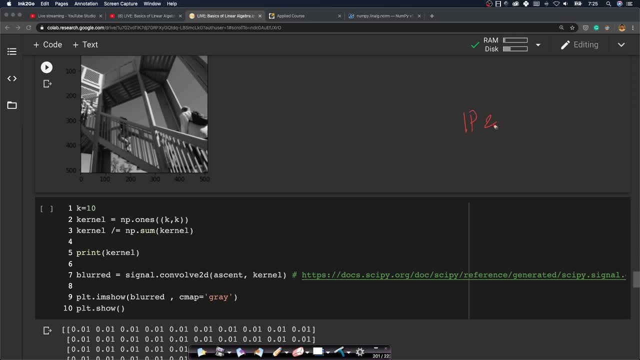 machine learning and data- sorry, in image processing. in image processing and computer vision there are like tons of kernels that are there. one of the simplest kernels is this: so what am i saying? i want to create a kernel like this. my kernel is is basically np1s, kk and k is 10, which means i'm 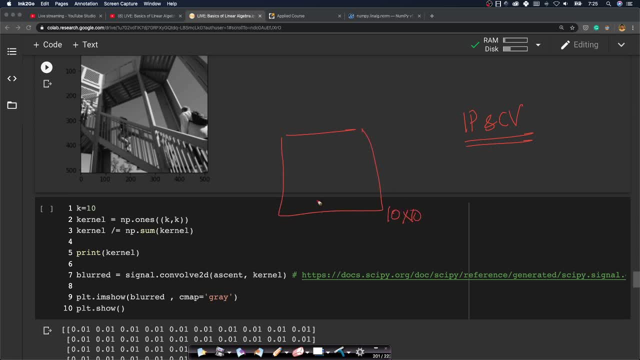 creating a kernel which is of size 10 cross 10. my kernel is a 10 cross 10 matrix, with all ones, with all ones. then what am i doing? i'm saying: how many ones are there here? there are 100 ones, right, think about it. 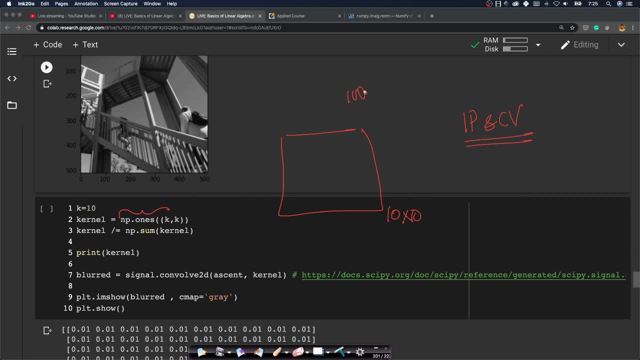 if, if matrix is all ones and there are 100 cells here, the sum is 100, then i divide all of these values. look at this: i divide all of these values. kernel equals to kernel divided by np sum kernel. so what happens to each value here? each value becomes 0.01, right? so if i print, if i just print, 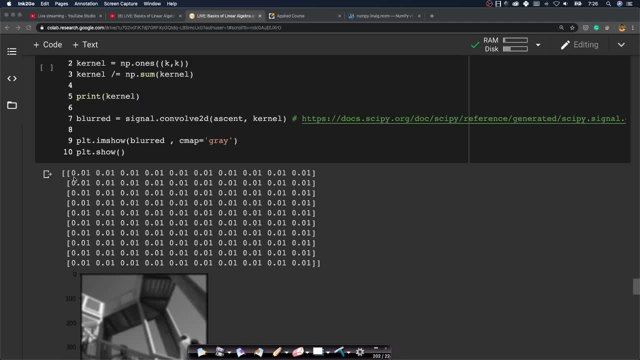 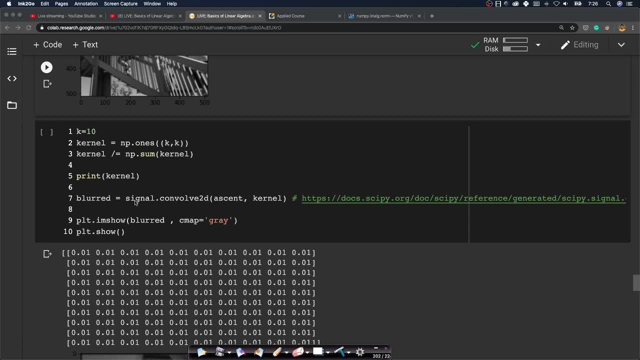 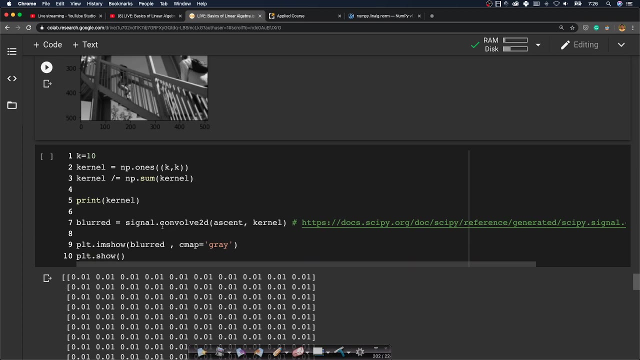 my kernel. i get this. it's a 10 cross 10 matrix. look at this, it's a 10 cross 10 matrix with very small values here. now i'll apply this kernel. look at, look, i can apply this very easily again. the signal is in. look at, this is in, is in scipy. scipy has a way to build. 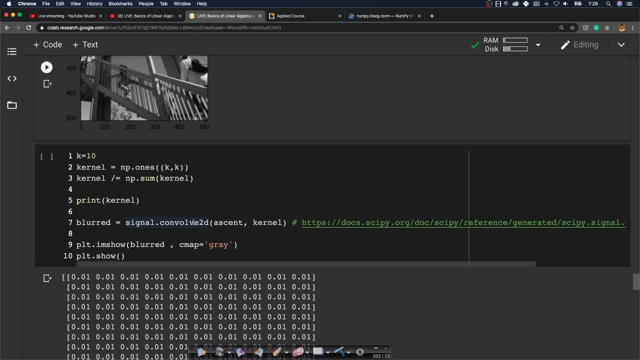 2d convolutions again. they are also available in tensorflow, keras, etc. but let's use scipy now. okay, scipy and umpy are like siblings. so signalconvolve 2d, which means it's doing 2d convolution. and what do i want to do? i just want to do a 2d convolution between ascent. ascent was. 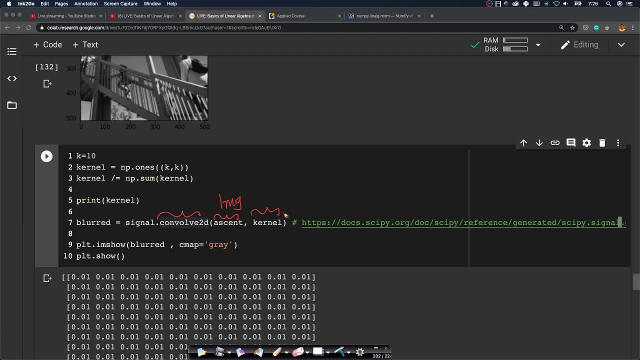 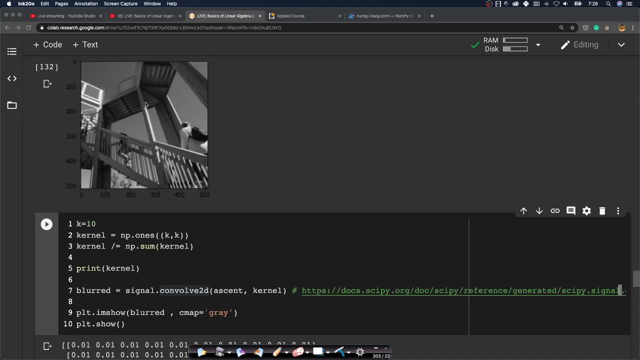 my image, right, and my kernel. what i get? i get my output as blurred. okay, so i'm just calling. i'm just calling this output as blurred. let me, let me show you the image. what happens to this image? if you look at this image, this image looks like a blurred version of this image, right? so the kernel that we create is called as a. 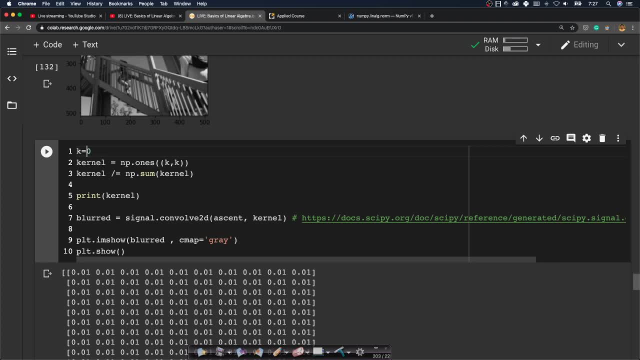 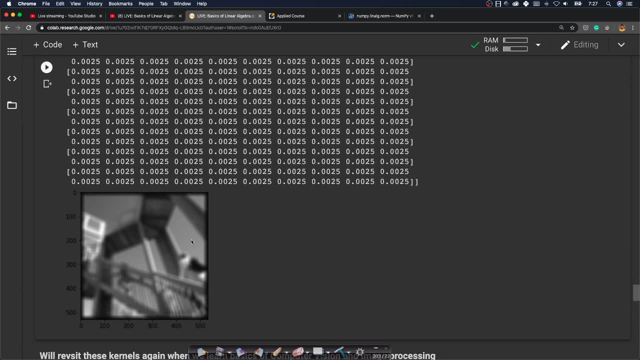 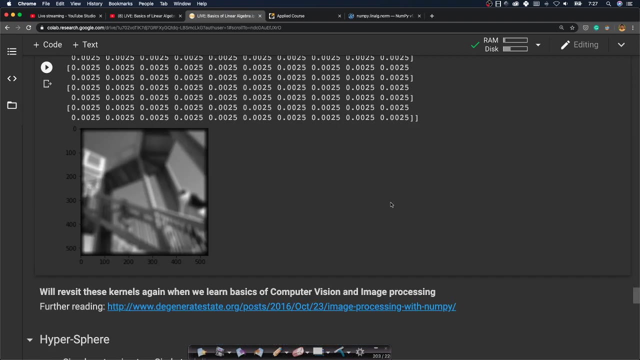 blurring kernel. right, if i just increase this size, if i just increase the kernel size and re-execute it, it will take a couple of minutes. look at this. it is more blurred now if i increase the size of the kernel. look at this: if i increase the size of the kernel, it becomes more and more blurred. 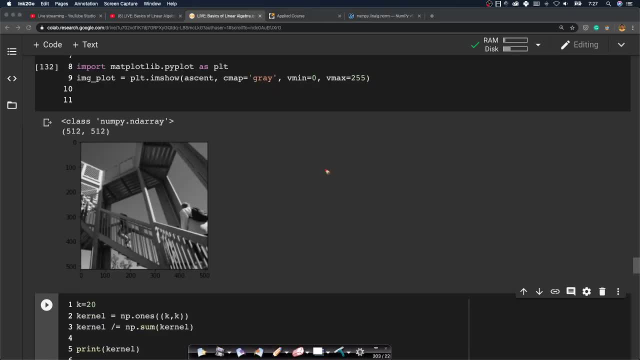 so the the the operation of image blurring. look at this: the whole operation of image blurring, the whole operation of image blurring can be represented as a simple 2d convolution operation. you can represent it as 2d convolution and 2d convolution is nothing, but it is simply. 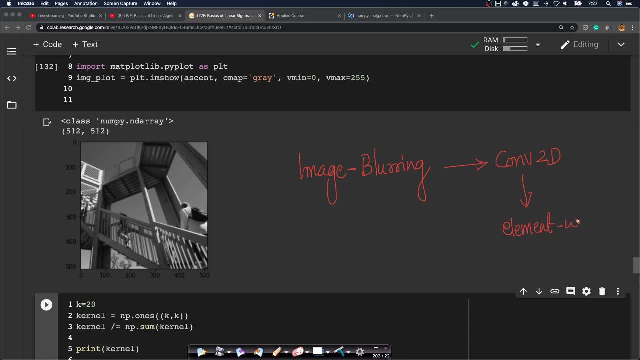 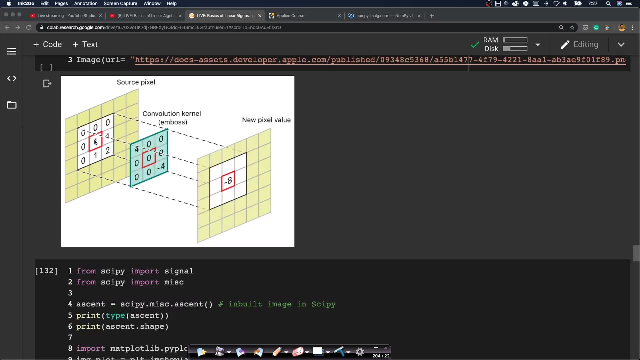 element wise matrix multiplication. it is element wise matrix multiplication, also called as had a mat product. it is element wise matrix multiplication plus for loops. right, because you have to do this for every element in the input image, right? so look at this: for every element in the input image you have to do this element wise product. 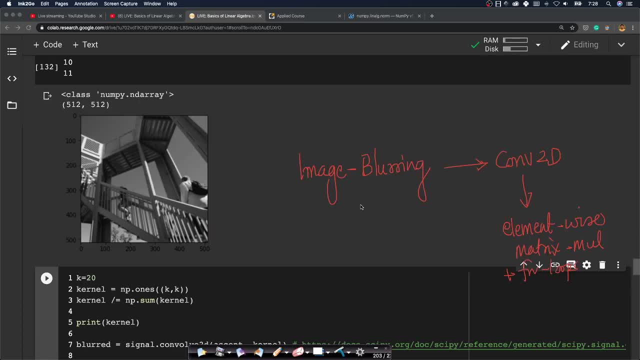 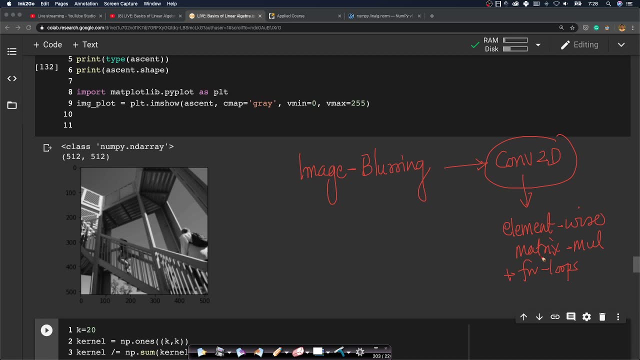 and then get the output value. so if you think intuitively, intuitively, what is image blurring? image blurring is simply 2d convolution. and what is 2d convolution mathematically? it is simply mathematical. if you think about its score, it's simply matrix multiplication with a bunch of for. 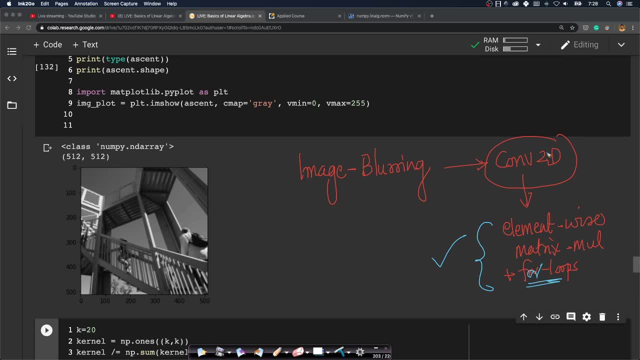 loops. so most of mathematics that you learn, most image processing algorithms are at least a good number of them, if not all of them. similarly, if i want all the edges in this image, which is called edge detectors, which is called edge detectors again, there are kernels for edge detectors there. 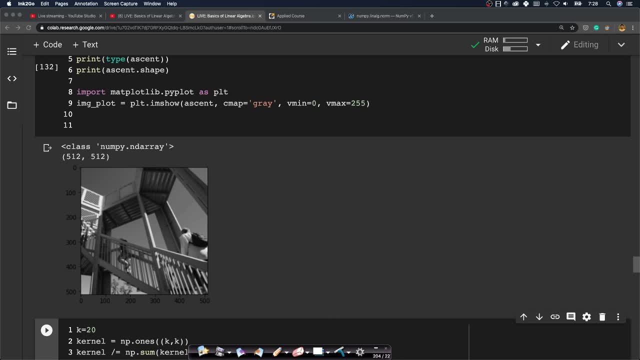 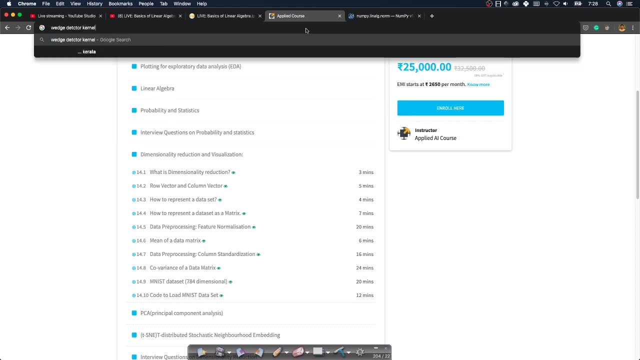 are a bunch of kernels called edge detectors. again, you can just google, search for them, you get kernels for that and you can try it. so for example, let's say you do edge detector kernel, edge detection kernel, okay, let's go to. okay, there is something called sobel operator. 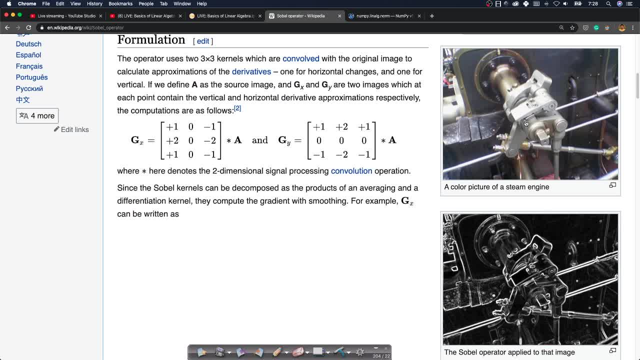 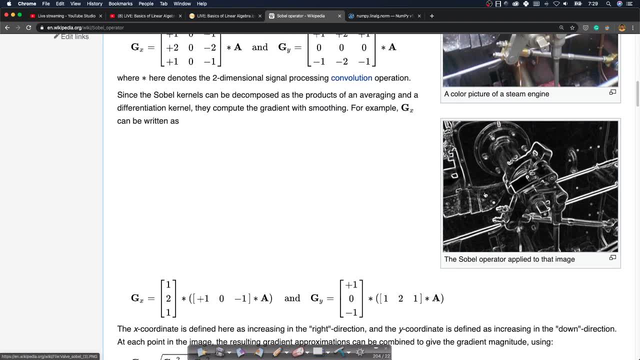 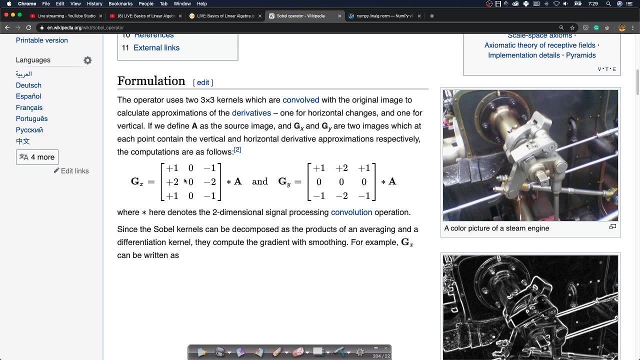 okay again. so look at this. if this is my input image, look at what sobel operator does. okay, so if this is my input image, i can get my output image like this, where all the edges are highlighted. look at this. i can do this using two, using two kernels called as, which are called sobel operators. 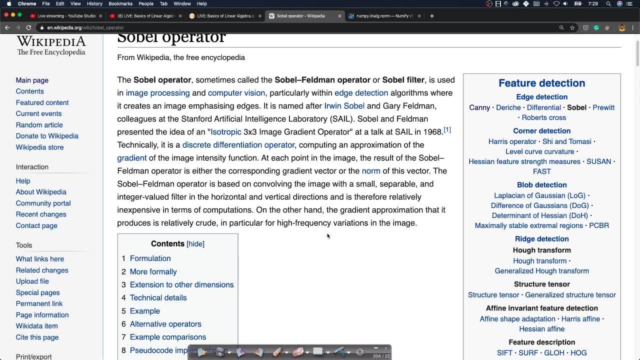 or you can call it sobel operators, if you are using a kernel which is called an original kernel, Sobel kernels which is named after Irwin Sobel and all these things, right. so edge detector is also nothing but convolution operation. there are a lot of operations. 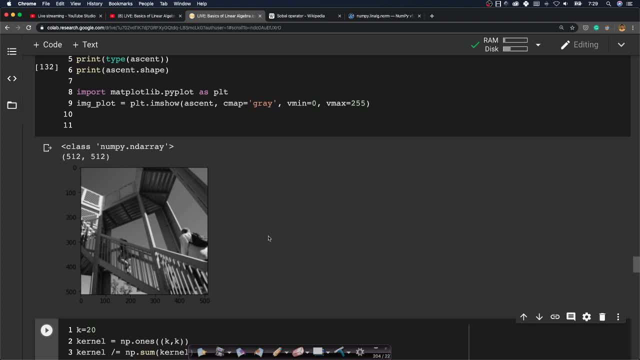 actually convolution is such a foundational concept of image processing that convolution is the core concept. it's the core concept behind most of deep learning on images. it is at least one of the most important concept today. deep learning techniques or images are able to work because of the concept of 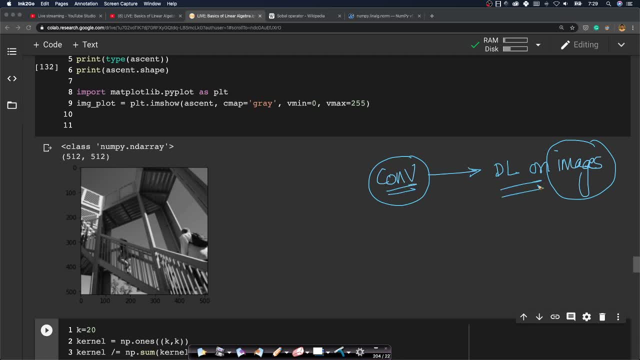 convolution. if we did not have convolution it would have been extremely hard to make it work, and convolution itself is nothing but matrix multiplication is nothing but matrix multiplication or Hadamard product and things like that right. so a lot of complex concepts in machine learning, deep learning, can be broken down to simple linear algebra again in the 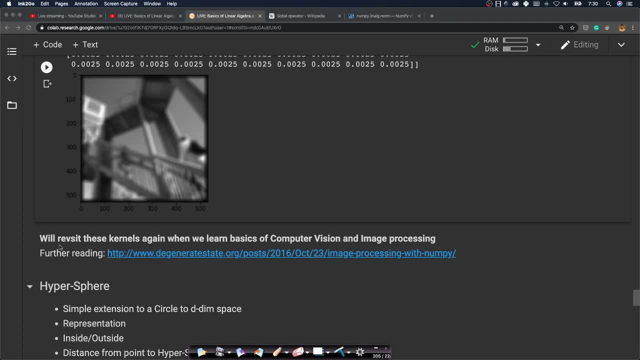 interest of time I cannot cover more examples here. so what I've done here is we will revisit these kernels again. we'll do some sessions on basics of computer vision and image processing right in these again. we'll revisit the concepts of convolution. we'll learn many more convolution operators. we will learn OpenCV, or foundation basics of OpenCV. 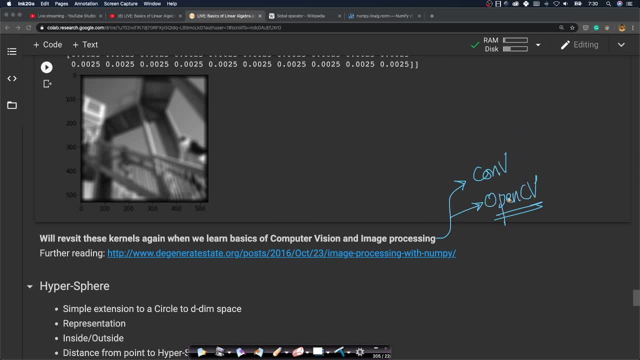 OpenCV is a huge library for computer vision. we learn some of the basic operations in OpenCV in the context of machine learning and AI right, so we'll do some sessions on these in the future. but if you want to read some nice examples, here is a very nice blog that I came across. 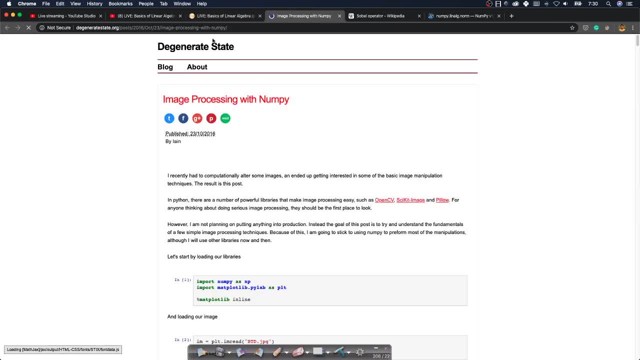 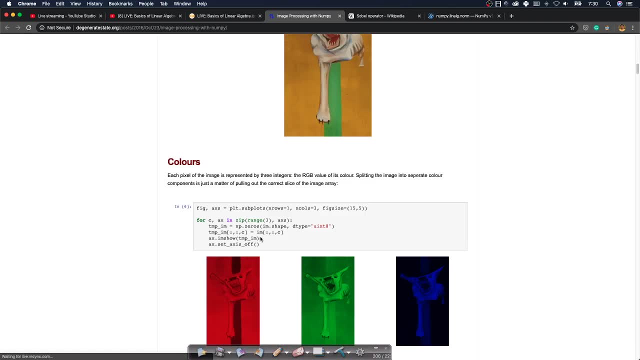 you can go to opencvcom and click on the link in the description of this video. just look at it. I'll share this whole document. this document is image processing using numpy. they have taken an image- again very simple, very easy to read code. they get RGB colors again. they do it on color images right, so very nice. 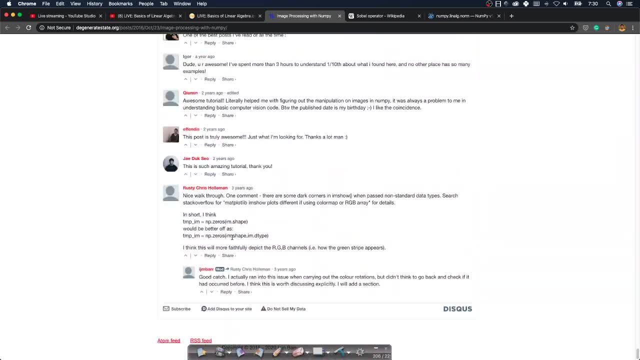 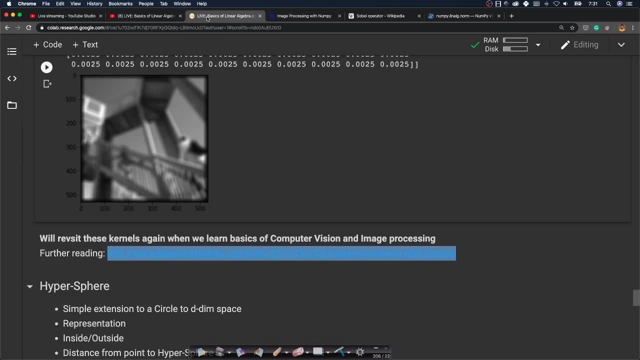 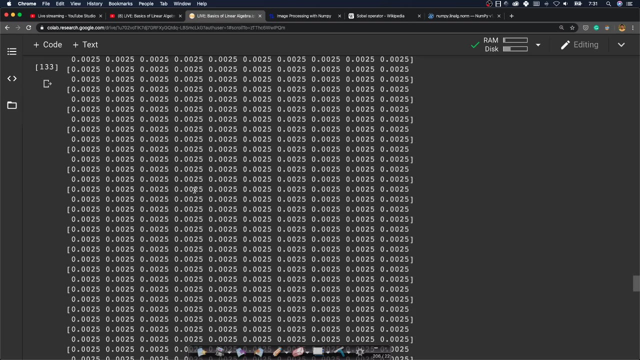 they do. they do a lot of operations on this. it's a nice post. if you are interested to look at more operations on image processing and don't want to wait for that live session, here is a nice link for additional reading. cool, so now let's go to let's again. the reason I put this concept in front of you is: 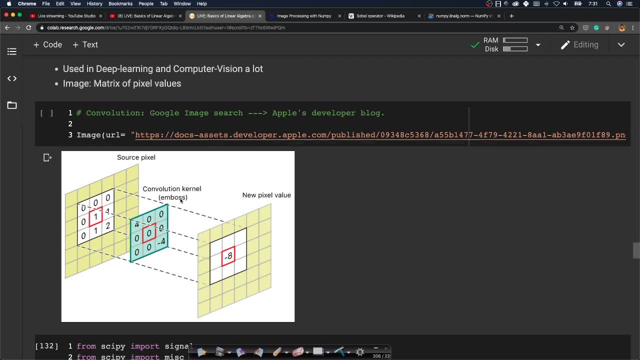 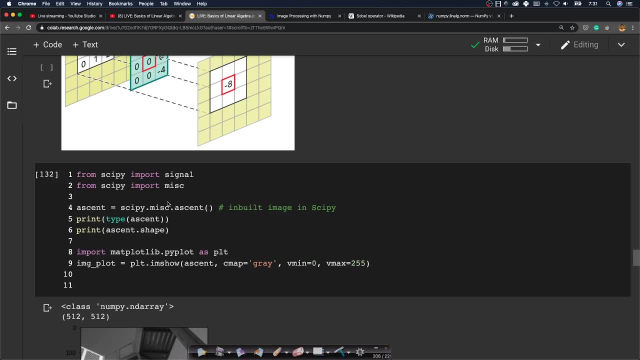 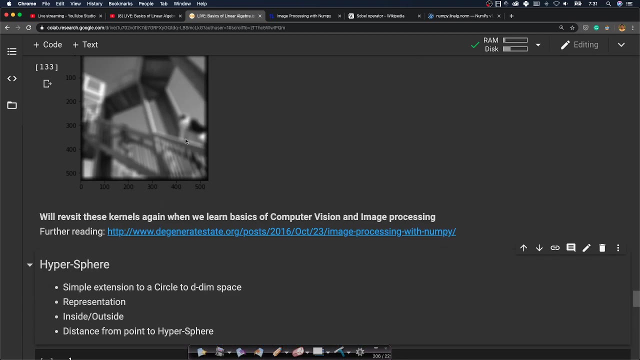 because I wanted to show you how powerful simple, simple matrices that you may think, hey, what the heck are we learning? right, something that is as simple as this is extremely useful. okay, yeah, somebody says, finally, I have something to play with. yes, you can play with this example. there are tons of. 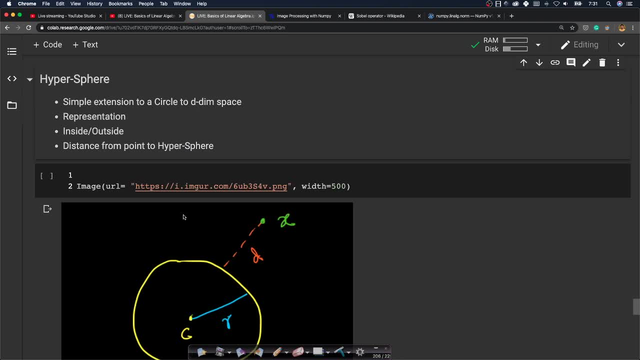 links again. you can do it very easily, okay? I know a lot of people love to play with image data. that's why I have shown this example. okay, cool again. I'll try to add more and more image data in the future sessions also. I know it, it is. 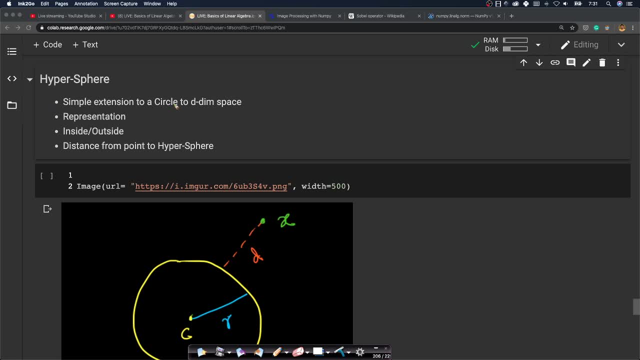 very interesting for people to play with. I understand that. okay, again, we have done. in the previous sessions we talked about circle point in a circle, all that I just wanted to extend that again. it's a very simple extension because spheres are sometimes used in machine learning not as much as planes, but in some 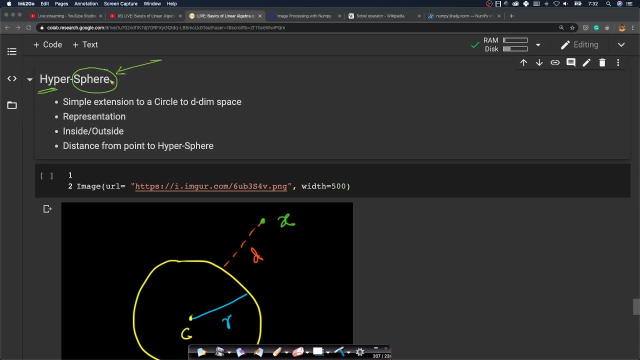 instances. we do use hyperspheres concept, not as much as planes, to be honest, but I just wanted to quickly cover it because, anyway, we have it in the course videos also. okay, so what is a sphere? sphere is a simple extension of circle to d-dimensional space. right, so you have circle in 2d. the similar shape is sphere. 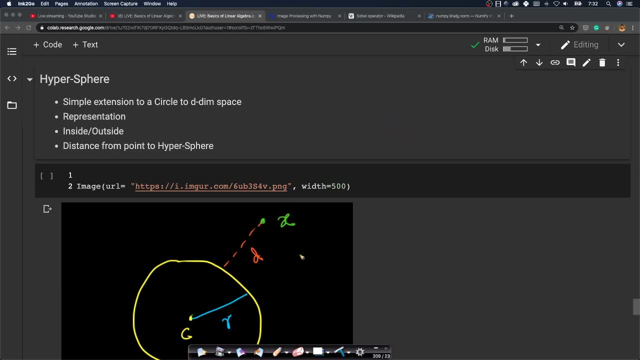 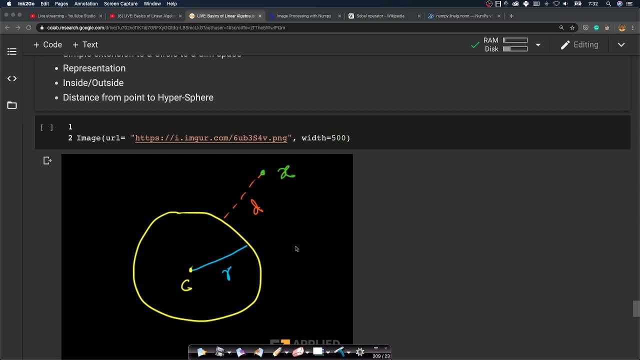 in 3d and hypersphere in high dimensional spaces. right again, since we can't draw high dimensional spaces, hey, I'll share this notebook with you at the end of the live session, in the in the comment section itself. so please don't worry about it. right, I'll surely share. okay, cool. so a couple of ways to do this. 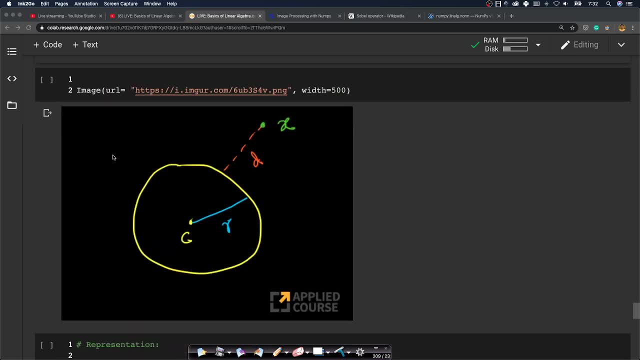 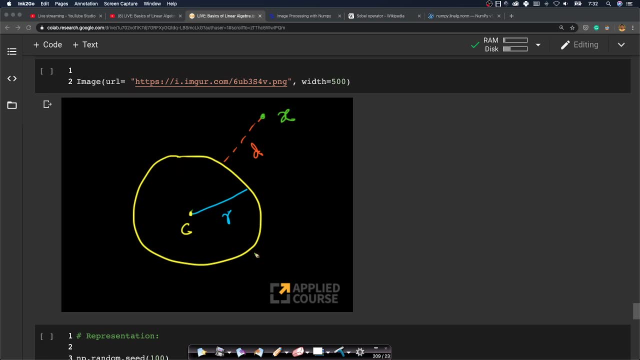 couple of very simple operations, we learn some very basics. these are commonsensical. so imagine if I have a. so I can't draw a hypersphere. so let's look at this. suppose if I have a hypersphere like this with center and radius. of course the center can be represented using a d-dimensional vector, because the 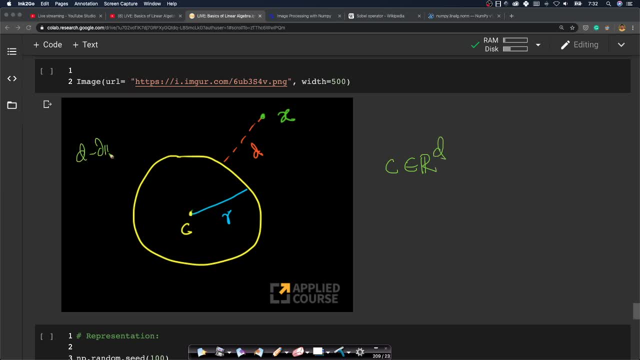 center is because let's assume this is d-dimensional space, right? if this is d-dimensional space, I can represent the center as a d-dimensional vector, like this. R is also a d-dimensional vector. the radius is also a d-dimensional vector, right, because it says in each dimension, what is the radius of this circle? right? 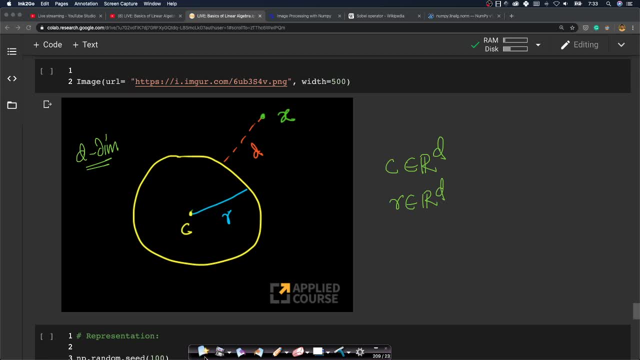 so that's important. okay, cool, actually, you can think of radius. you don't have to think about like this because for a sphere, okay, sorry, so you can think of radius as just one number. radius is a float, I'm sorry. so radius is simply a float value if you think about it logically, right? so because your circle. 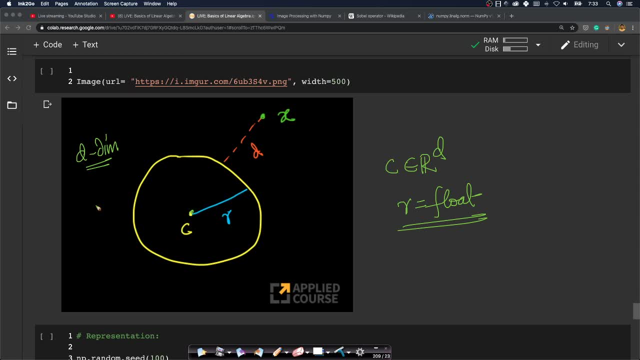 is fixed in all dimensions. so, basically, what is what is a sphere? sphere basically says all the point should be all the points which are at a distance. R from here is within my sphere, right? so R is not a vector, R is a float. it simple. and how do you do some simple operations on this? it's very simple, so I. 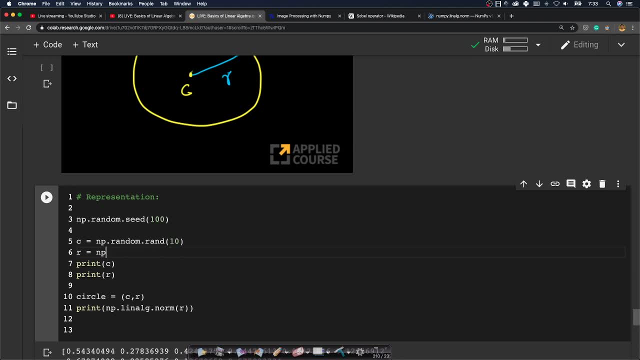 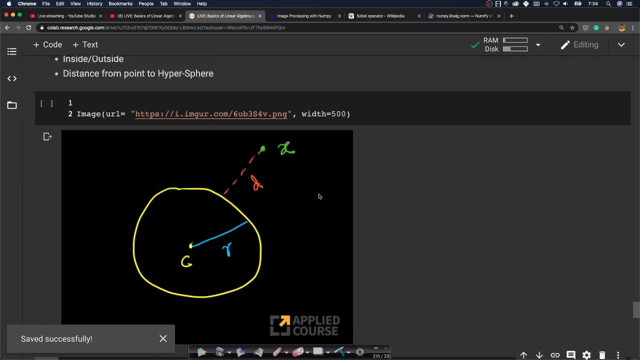 think I did a mistake here. okay, let me just say R equals to 10. I did a small mistake here because, again, the radius. let's just think about it. just give me a second. I hope I have not made a mistake. I was in a hurry when writing notes for 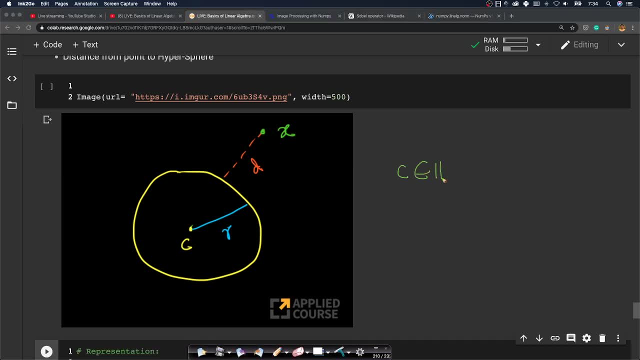 this because I was running out of time. So the center obviously belongs to Rd. My radius has to be a single scalar value, right? Because what it means is given this circle all the points which are there in this radius, in all directions. yes, R is a scalar, R is not a. 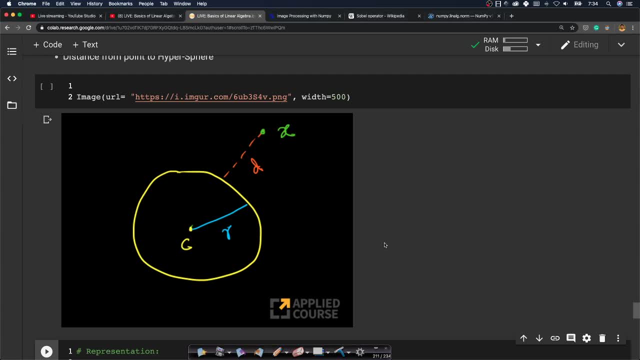 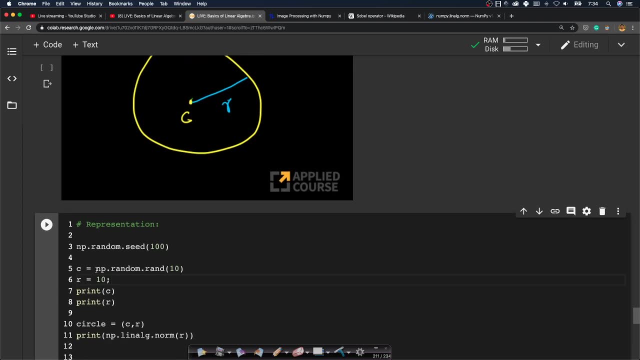 vector. I will write the code. I will modify the code as we go. okay, So a couple of operations that we wanted to read. no, So how do you represent? how do you represent a circle? Very simple, You represent the center using a vector: radius. 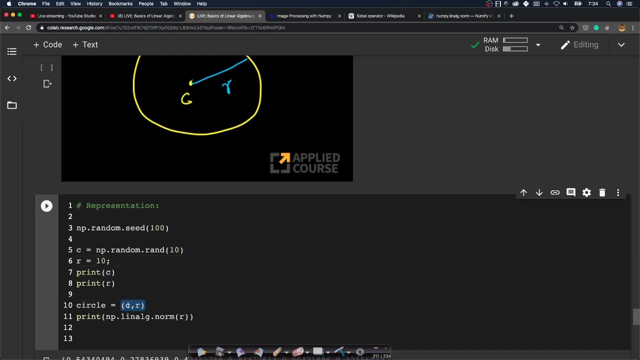 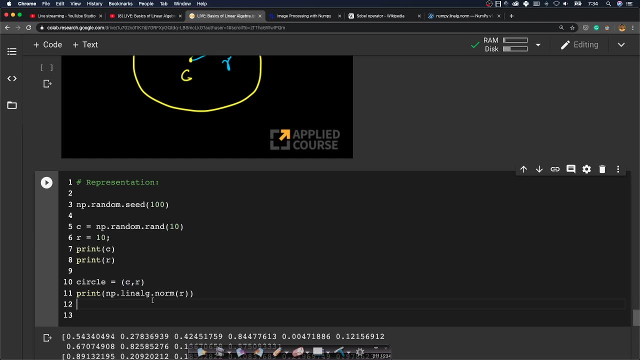 using a scalar, and a circle is basically a tuple of a tuple of the center circle. So I use C for circle, C for center, R for radius. Very simple, right? So I do not have to compute linear algebra, norm R, all of that stuff. I do not have to worry about this, okay? So 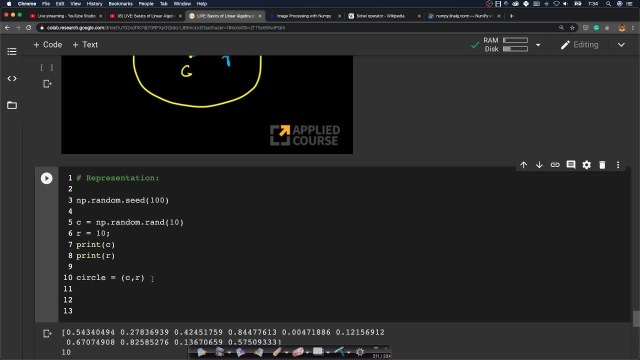 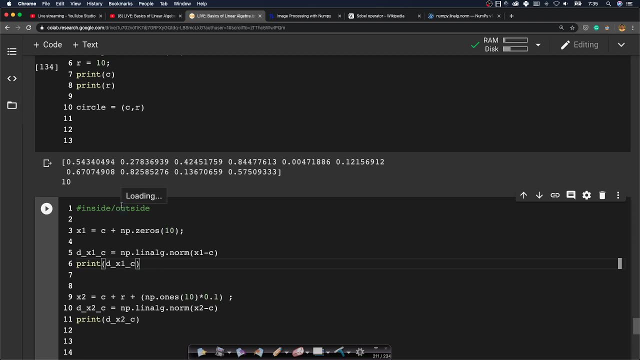 some very simple stuff. You can represent a circle very easily using the circle center and radius- nothing very fancy. Now, if you want to find if a point is inside a circle or outside a circle, how do you do that? Next, very simple question: right, If you think about it logically, how do you do? 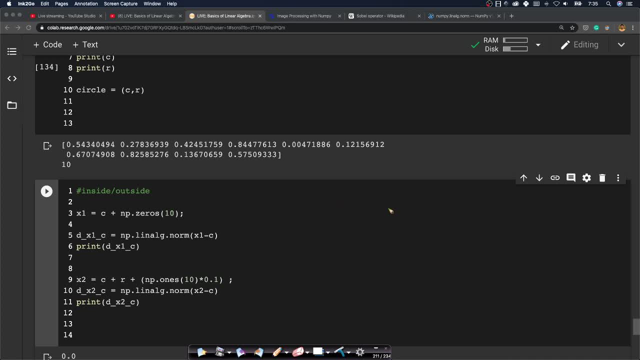 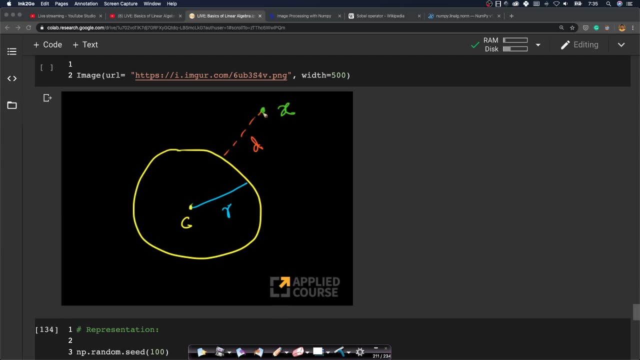 it? How do you decide whether a point is in a circle or outside a circle? It is a very simple concept, right? So you just compute. So, given a point like this x, right, You want to say whether this point x is inside a circle or outside a circle. That is an important 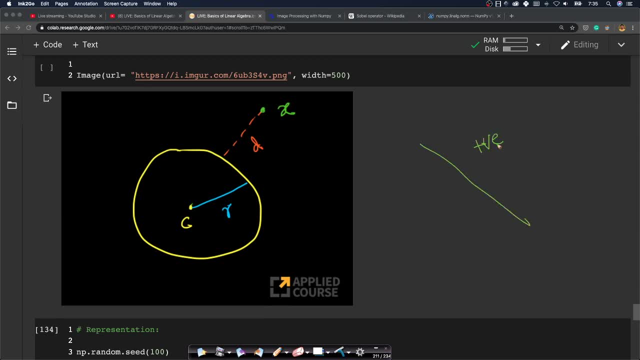 operator, just like for planes, right? You have positive, suppose, if my w is in this direction, if this is my plane, I have positive. So you have negative half space and negative half space. So a plane literally divides the space into two parts. Similarly, a sphere divides the space into inside the sphere and 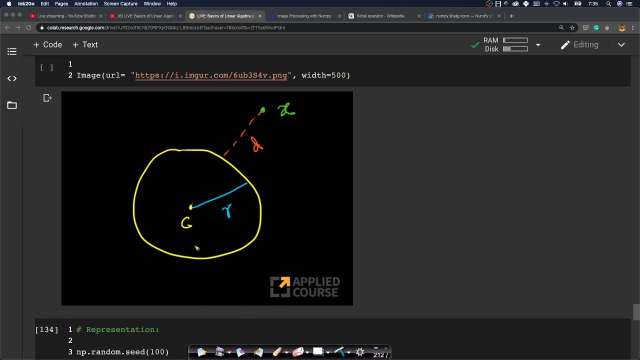 outside the sphere. It divides the space into two parts, and that is what is useful in some machine learning algorithms- Not all, it is seldom used, but I wanted to introduce the concept so that, even if you read a research paper in the future, you can understand it. 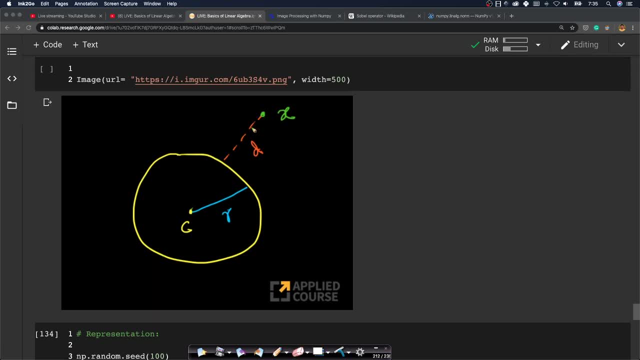 So what is the distance of a point x? So there are two things right. So how do you determine whether a point x is inside the circle or outside a circle? So what is the distance of a point x? So there are two things right. So how do you determine whether a point? 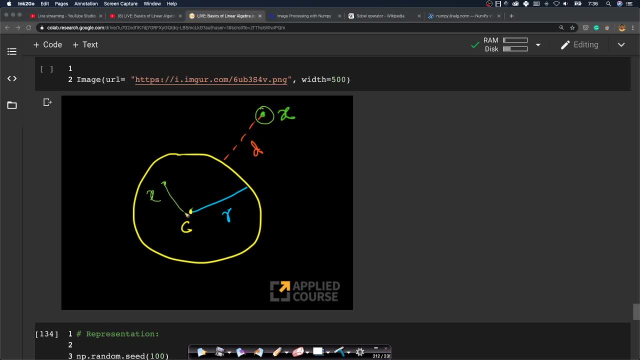 x is inside the circle or outside the circle? Very simple. If this is my point x, compute the distance. Compute the distance from x to c. Just compute the distance. If the distance is less than r, it is inside. Very simple. We have seen this for circle earlier, right? 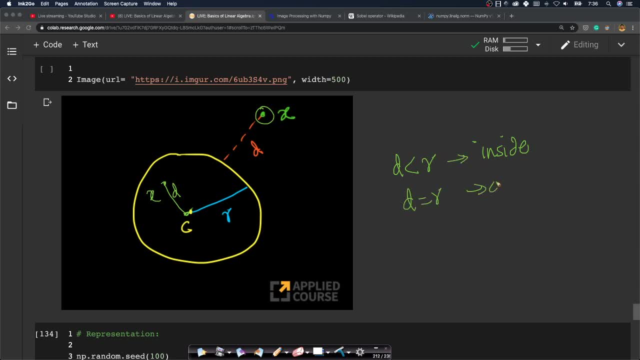 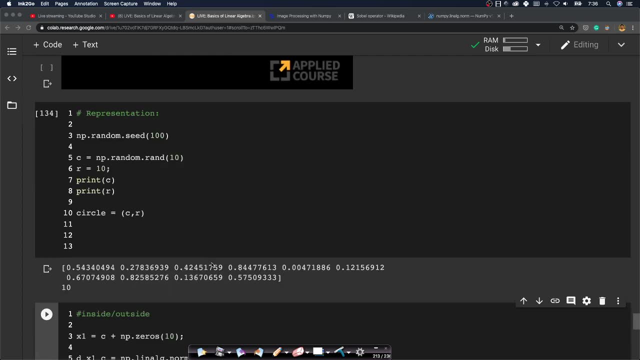 In the previous live sessions. If d equals to r, it is on. If d is greater than r, it is outside. Very simple, Nothing fancy right? Very simple, So we can easily write the code for it, right? So imagine if I have a point like this. okay, So I am creating a point. 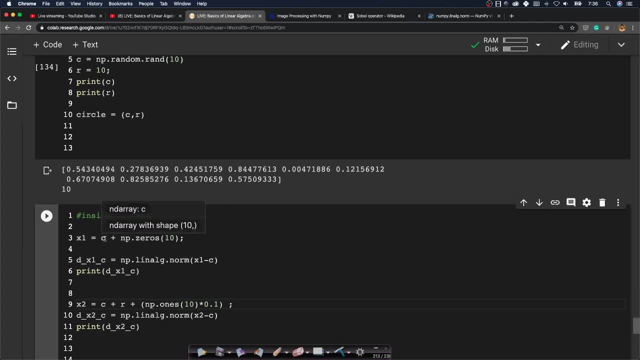 x1, right, I am just creating a point x1. And what am I saying? It is center plus zeros, which means x1 is same as center. right Now, how do I compute the distance? How do I compute this? How do I compute the distance? Suppose if this is my circle, if this is my point. 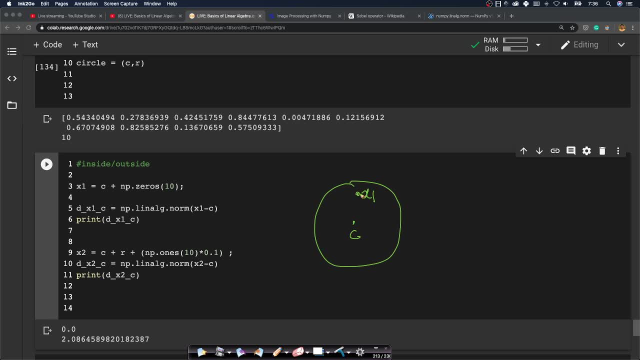 c. if this is my point, x1, how do I compute it? The distance is nothing, but do x1 minus c. If you do x1 minus c, what do you get? You get this, You get this. And if you take, 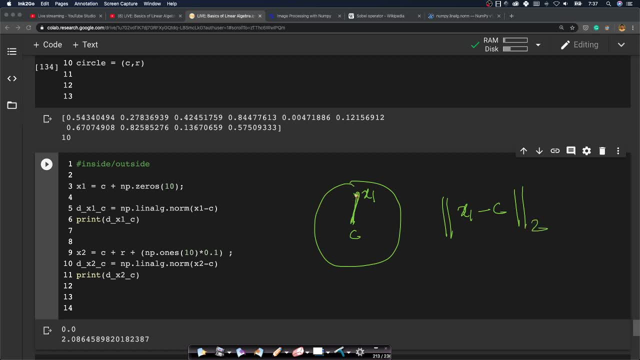 the norm of x1 minus c, norm 2, what do you get? You get the distance between these right. Just simple vector algebra. Look at this. If you have vector like this, if you have vector like this: v1, v2,- right. If you compute v1 minus v2,, right. And if you take v1 minus, 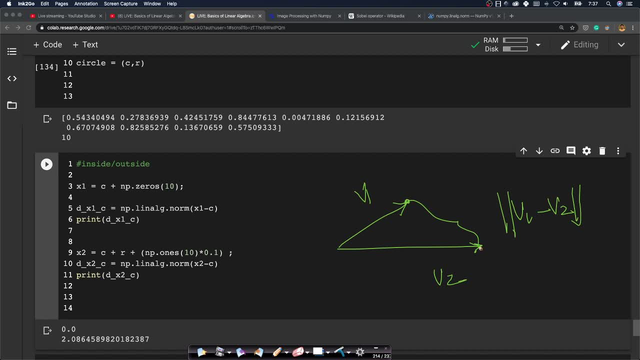 v2, norm 2, what do you get? You get this distance, You get this distance right. That is what v1 minus v2 gives you right. Similarly, same concept here. Same concept: here: c is represented by a vector c, x1 is represented by a vector x1.. If you want the distance between both, 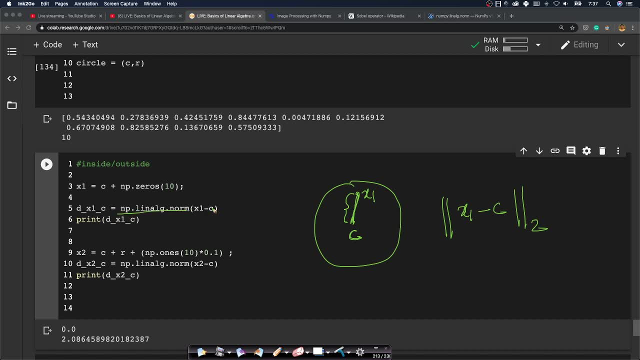 of them. it is very simple. Take the norm of x1 minus c. Very simple, right. So what is my x1 here? My x1 is c plus 0s, which means my x1 here is c. So I am computing the distance. 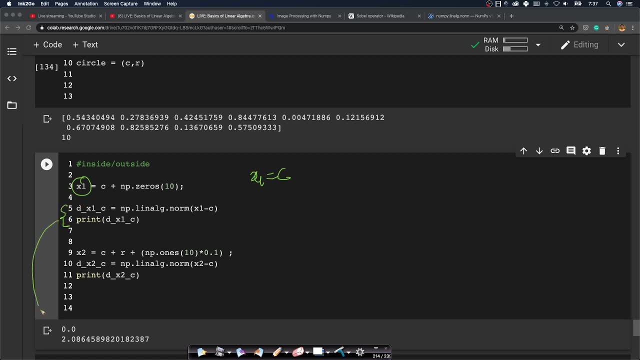 of c to itself. Just a test case. It should give me 0, right? Yes, it gives me 0.. On the other hand, let me create one more. So, let me create one more. So imagine if I create my x2.. 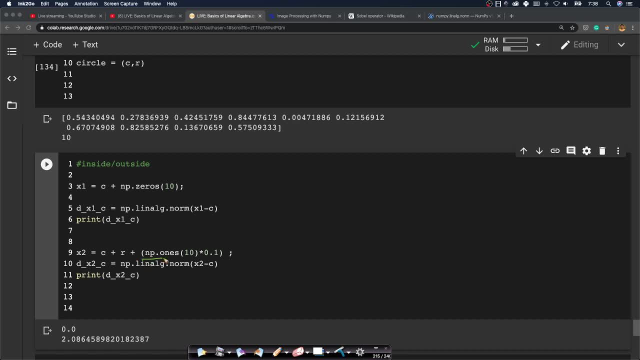 Let me create another point, x2, right, How do I create my point x2?? I create my point x2 as the center plus all the radius values, all the radius values that I have, Center plus the radius value that I have. Okay, let me just execute it once. Does this lead to? 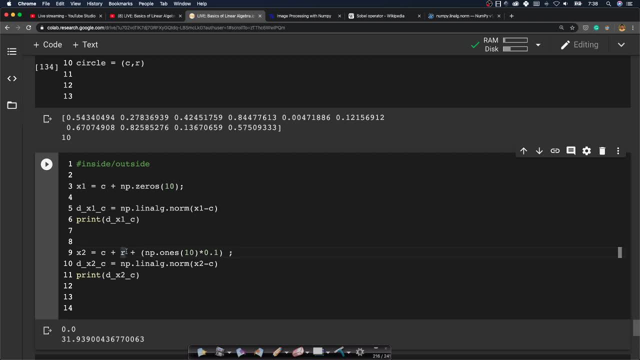 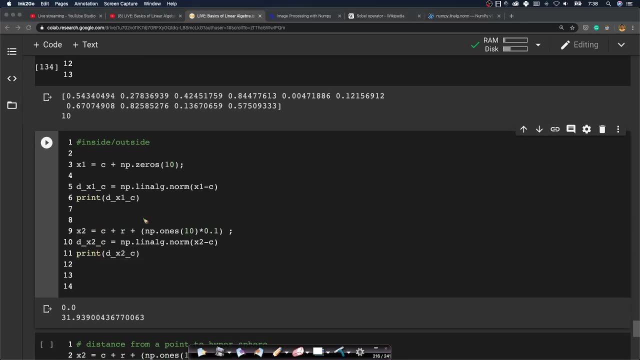 an error, Because I, oh, it does not clear. Okay, cool. So or else let us just okay, that is okay. Center plus radius. Let us just change this, It is okay. So if I do this point. 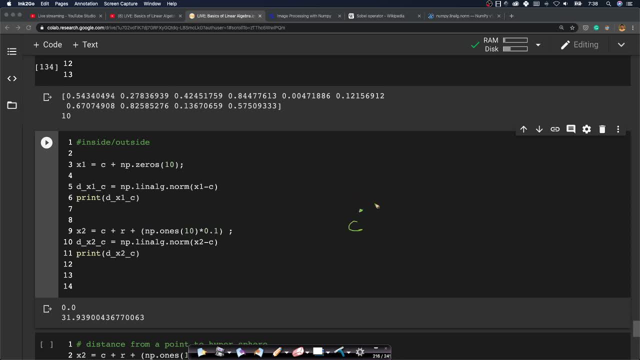 this point is So. I have now declared it as a center. I am adding radius, which means I am adding. So if this is my sphere, I am saying, add our on all the dimensions and then add some more value to this. Obviously, if I add our, if I add our to each of the dimensions, this 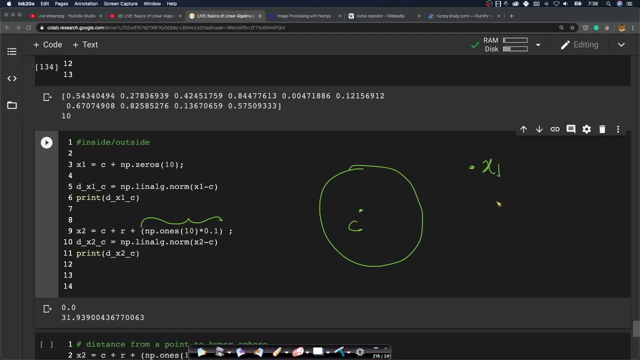 point x1 has to be outside. obviously it has to be outside, right. It has to be outside, I mean by design right. So now, if I do x2 minus c, look at this or this point, I am. 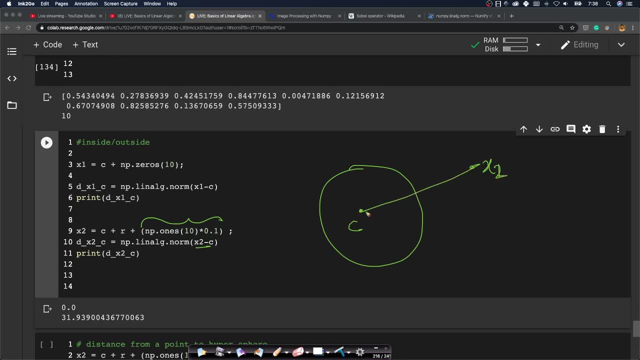 calling it x2, right. So if I do x2 minus c and if I take the norm of it, norm of x2 minus c will give me this distance right. norm of x2 minus c will give me this distance. now, if this distance is greater than r, look at this: how do you determine whether you are inside or outside? 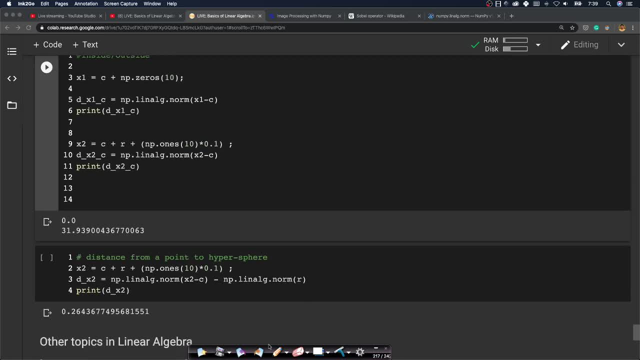 my r here is 10. okay, if the distance is, as we have just seen a while ago, again, very simple. this: whatever you learned in with circles, same concepts hold here, also when the dimensions become very large. there are other problems that we discuss when we when we handle high dimensional data. 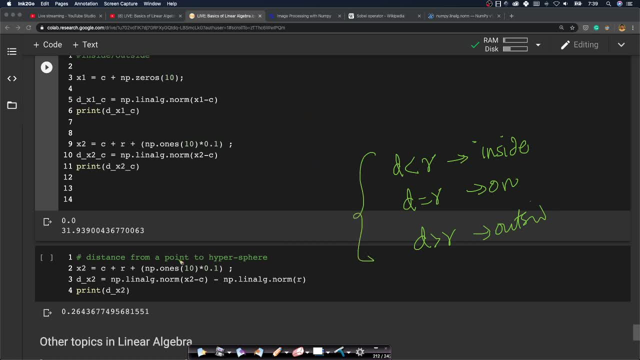 right, you, you get something called as cursive dimensionality and others that we learn later. for now, as long as the dimensions are not too large, this logic certainly works well. now, how do you, uh, how do you find the distance? okay, this is, this is an interesting thing, right? 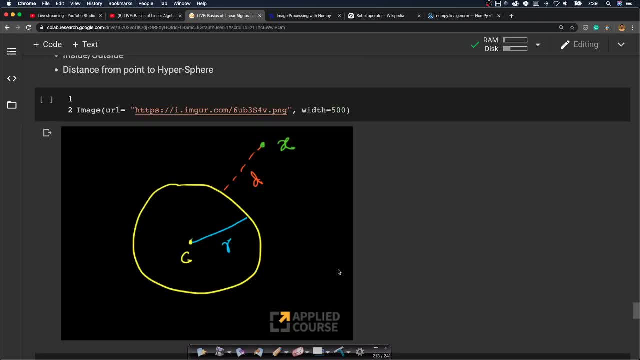 how do you find the distance from a point to a hypersphere? suppose you are given a hypersphere with center r and radius- sorry, center c and radius r. you want to find the distance from point x to the, the shortest distance. you want to find the shortest distance to the surface of the sphere. 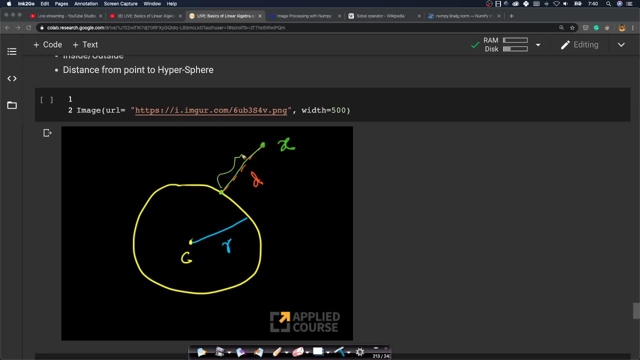 to the surface of the sphere. so if this distance is d, how do you find this distance d? how do you find this distance d? again, please understand that this is in d dimensional space. this is not in 2d. okay again, i'm only talking about d dimensional space because it's easier. 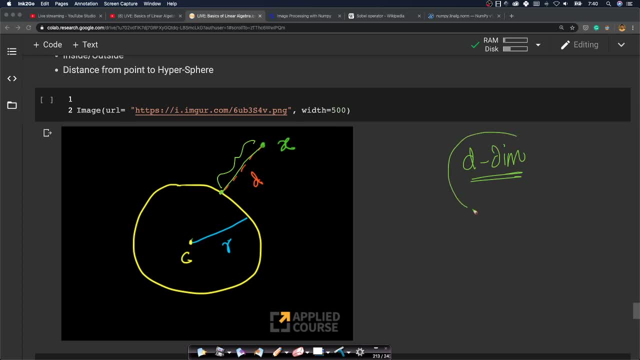 to generalize, the whole objective of learning linear algebra is to operate in high dimensional spaces and to operate on data matrices, right? so how do you find this? okay, this is a good question. can anybody help me with this? what is this distance? so i want the shortest distance. i want the shortest distance between a point. 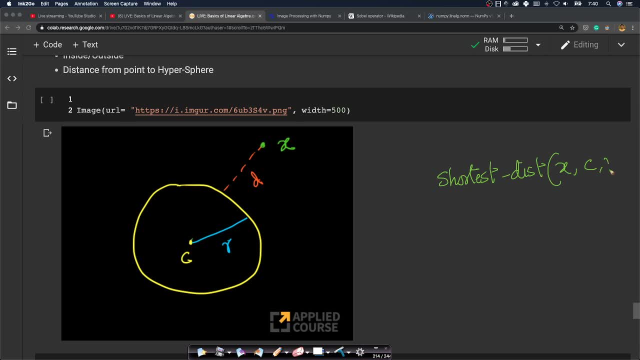 x and a circle represented with c and r. okay, let's assume this is how i represent a circle. i represent a circle with the center and radius r, if i want this. how do i compute this? can anybody help me with this? i'm looking at the comment section. so if 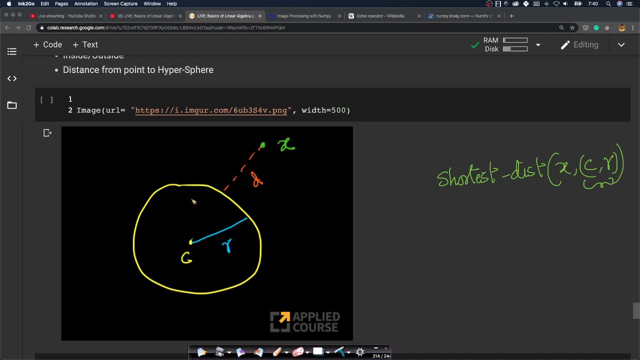 somebody can help me with this. oh yeah, very simple. i'm glad you guys got it like in no time, right? you just compute the distance between. so this is very simple. this is basically the distance between center and x. what is the distance between center and x? it is nothing. 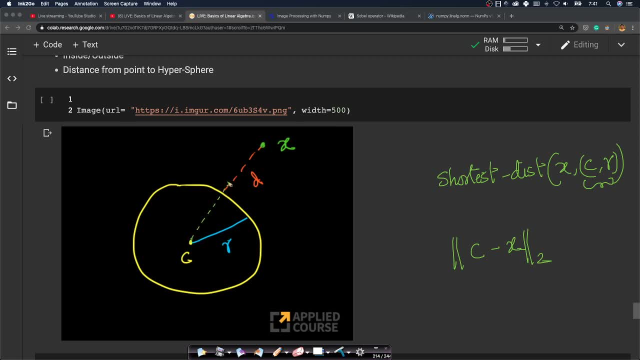 but this, this is basically this distance, this is basically this whole distance. from this distance, we know that this distance is radius. you subtract r from this subtract r, you get this remaining distance. that's it. it's just, it's just literally this like one line code. again, this is sometimes used in: 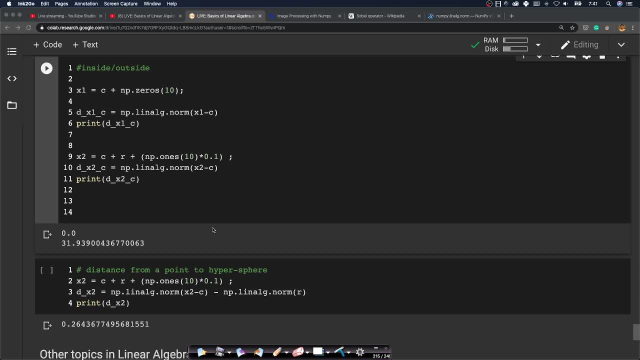 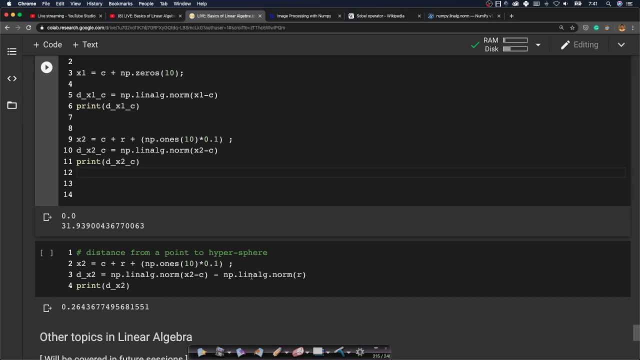 machine learning. that's why- or or i should say in in clustering algorithms and things like that, this is sometimes used. okay, so let me just show you that suppose, if i take a point like this, cool, so okay, i don't have to do this, i just have to say minus r, okay. 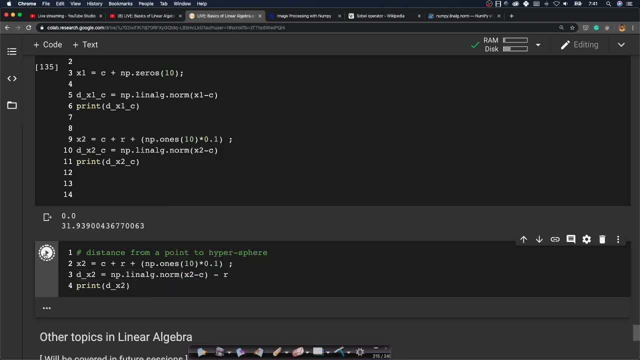 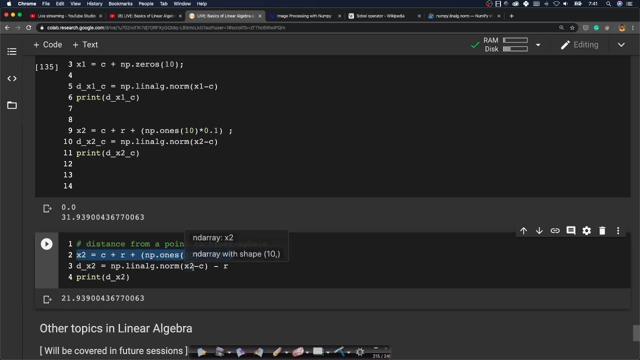 linear algebra: norm x2 minus r. yeah, so this will work. okay. so what do i get? this is my distance. so i'm just creating a point here. right, i'm saying the distance between the point to the circle. how do i get the distance? it is basically x2 minus c or c minus x2, norm minus radius. done, problem solved. again what? 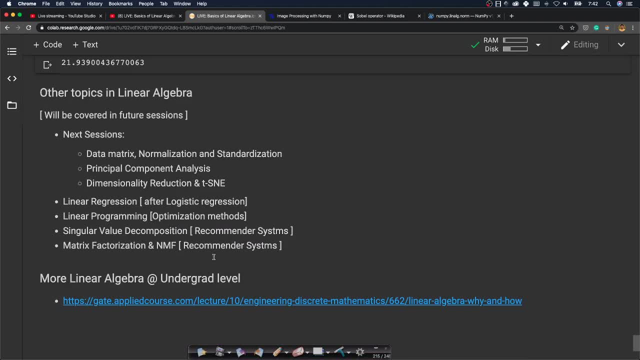 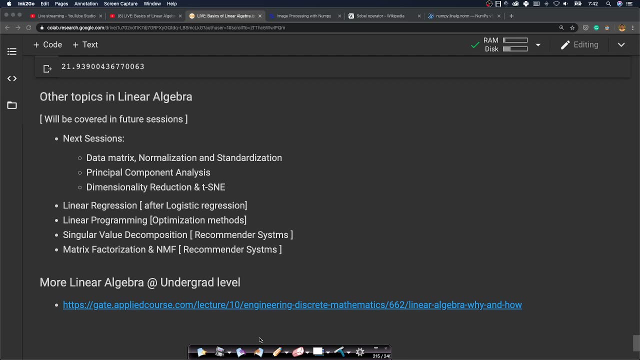 we're doing right now is just a surface touch of linear algebra. let me tell you other topics in linear algebra and how they're extremely powerful. okay, again, this list is not exhaustive. this is just some of the topics. okay, again, we'll try to cover these in the future sessions. 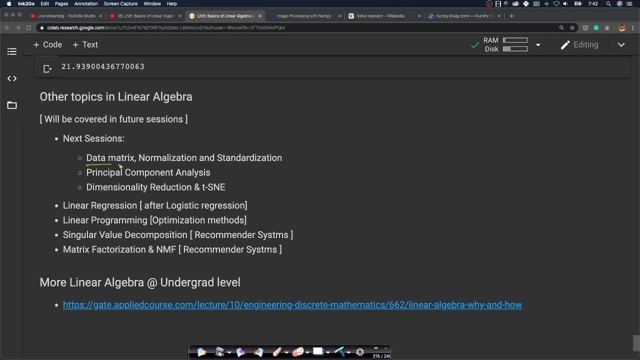 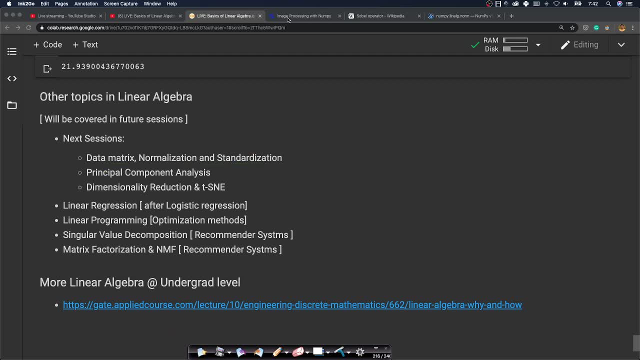 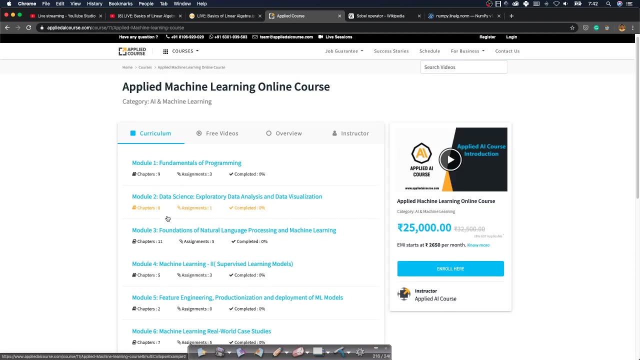 you can watch some of these free videos of our course that are readily available, so you can just go to applied a course. you can just go to applied a course. go to view course. some of these videos are freely available, so please feel free to check it out. look at this dimensionality. 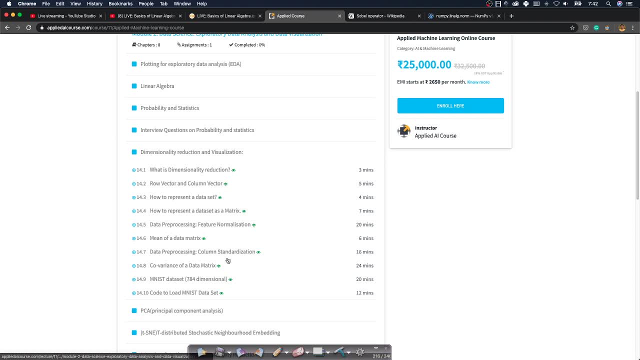 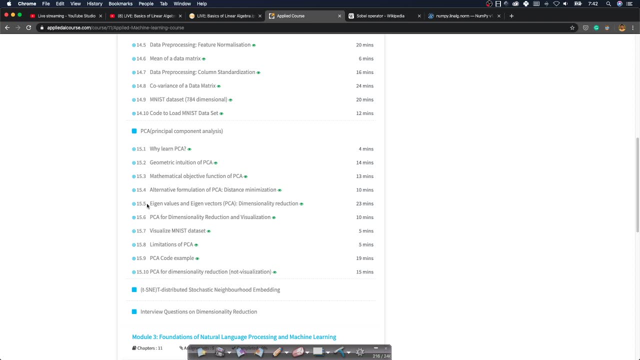 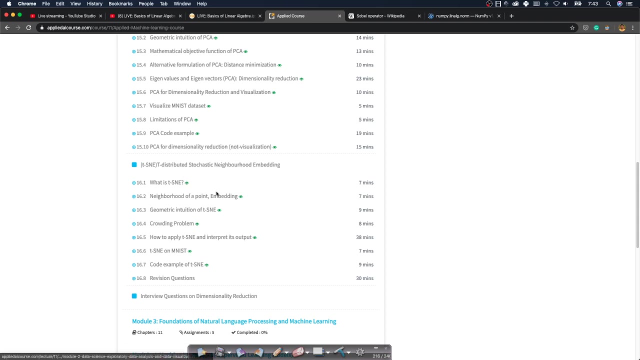 reduction and visualization. all these videos are available. you can learn about the basic operations. you can also learn about principal component analysis. again, we go into the mathematical depth with some code, examples, etc. there is also pre-distributed stochastic neighborhood embedding. again, this you cannot call it pure. you cannot call it pure linear algebra method. 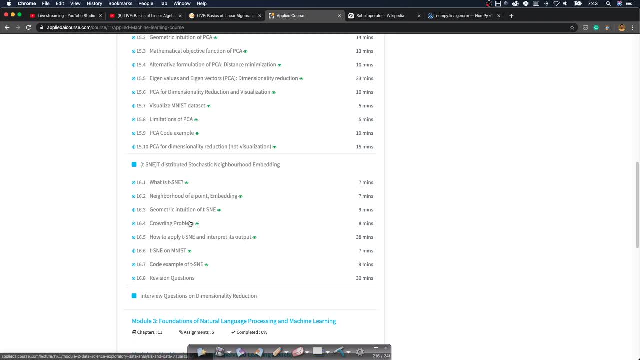 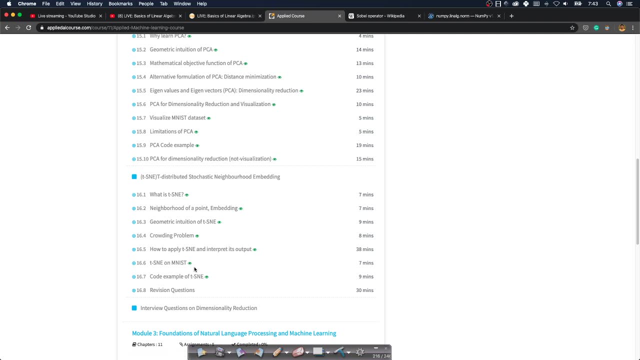 because it's more based on other concepts, like it's based on optimization, etc. but we thought, since we covered pca, we thought we'll cover tc also. so tc is not a pure linear algebraic method, okay, while dimensional reduction is a concept in linear algebra, for sure. so some 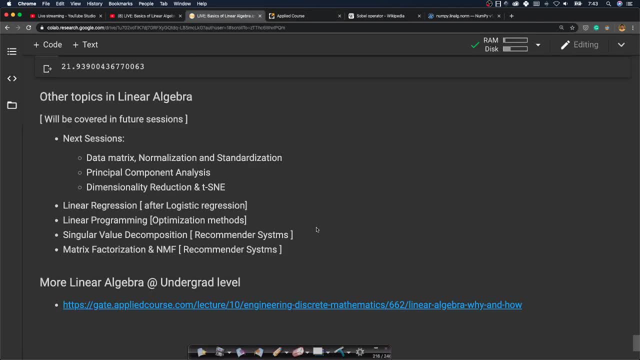 of the free videos are available, so please go check it out if you're interested. so these are some of the concepts, for sure, right? so we'll do a few sessions on these topics next. then, if you look at linear regression, if you pick up any major book on linear algebra, they 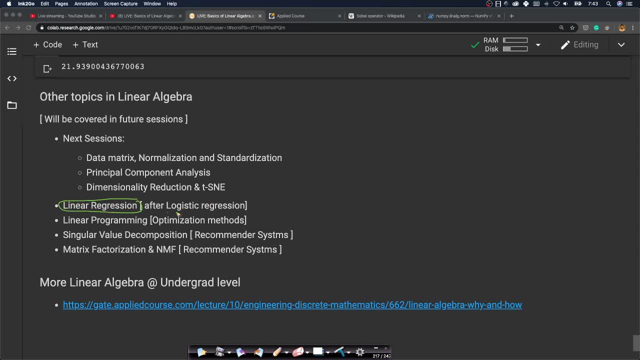 cover linear regression. right again, we covered linear regression after logistic regression. error course, you can pose most of linear regression as, again, linear regression can be studied from three fronts. there are three ways to study linear regression. you can read it from a pure linear, algebraic perspective. you can read it from a pure probability and statistics. 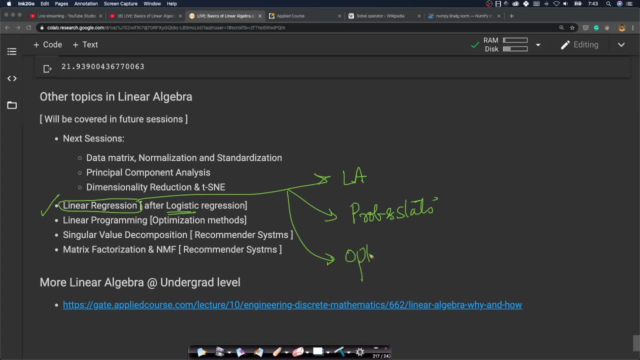 perspective. you can look at it from an optimization standpoint. there are three ways of looking at it. okay, so we focused more on the optimization way of looking at it and linear algebra way of looking at it. we also gave hints about probability and statistics way of looking at this concept. 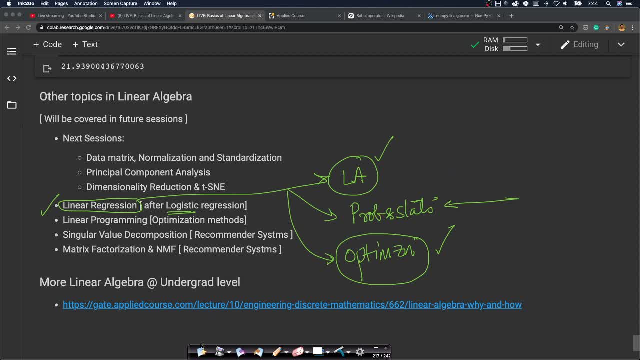 in the course videos, but we didn't go too deep into it. okay, then you have this whole concept called as linear programming. again, we'll do a live session on linear programming when we come to optimization methods. then you have this singular value, decomposition, matrix, factorization. the linear algebraic concepts are extremely useful in the, in the, in the area of recommender. 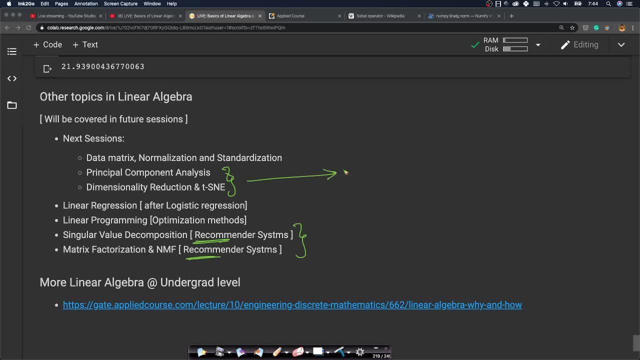 systems. again, these, these are useful in data visualization. in data visualization, if you want to visualize a 100 dimensional data, how do you visualize it right? so a lot of linear algebraic techniques like principal component analysis, dimensional reduction, t-SNE, are used in that context. again, those of you who are interested in more undergraduate level, because 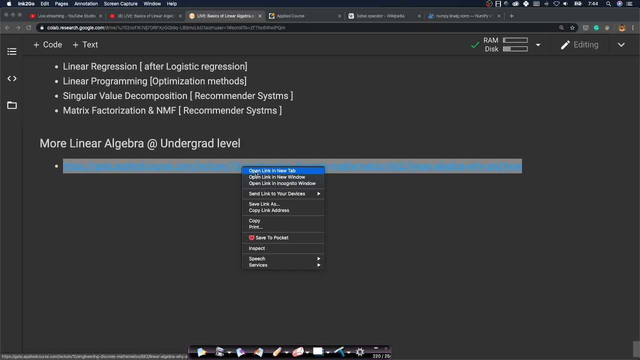 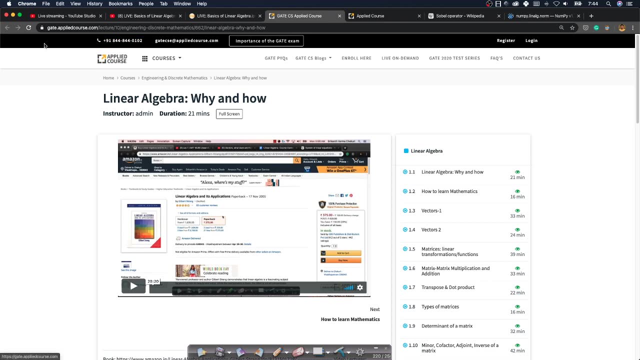 i believe some of so. let's look at this. so we have done one more course. let me open this here. we have done this for gate computer science students, okay, so you can just go to this. so I shared this link with you, where these videos of linear algebra freely available. 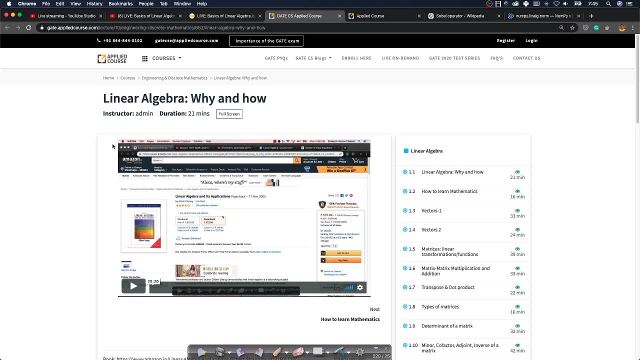 so this is more of an undergraduate level, not necessarily computer science. so whether you are a CS student, right, whether you're a CS or any engineering student- eC, mechanical, name it- any of these engineering students who want to learn. you know algebra from a more undergraduate syllabus. 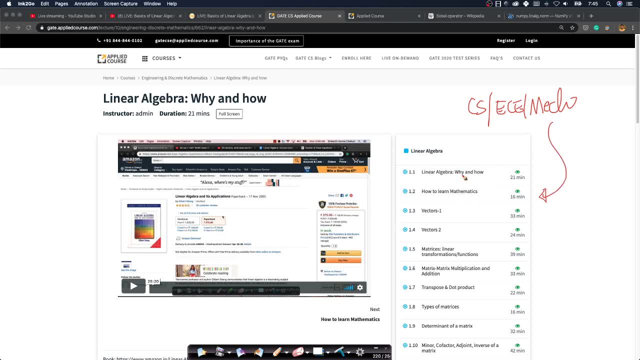 perspective, have a bunch of videos here. Again, I try to explain all of this from the geometric intuition perspective. right? Whichever videos I do for any subject, I try to do it from a geometric intuition and practical application perspective. So the videos here are more like your undergraduate. 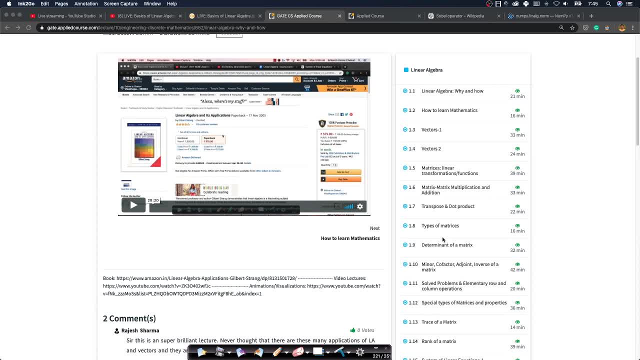 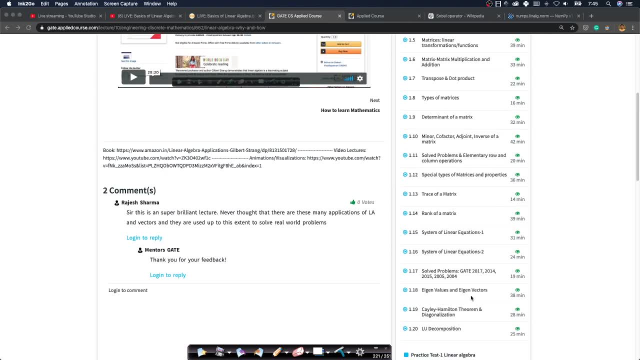 syllabus So we learn about vectors, linear transformations, determinant of a matrix. why do we need all these right? Again, rank of a matrix, solving linear system of equations, decompositions. Again, this is done more from an undergraduate perspective. So if you're 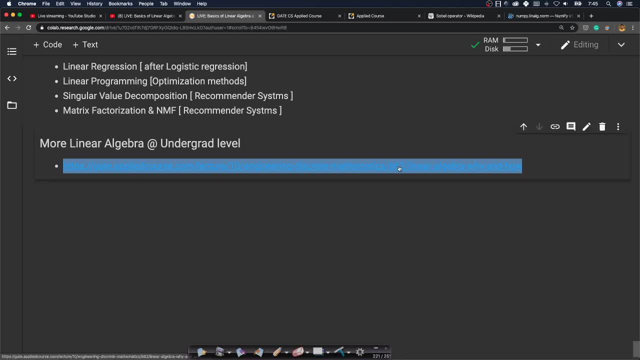 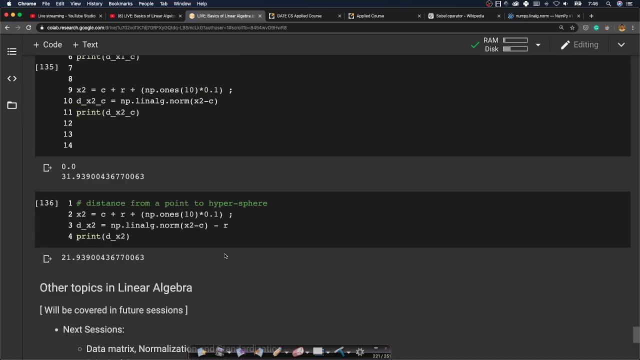 interested. these videos are also freely available. Please go check it out And if you think somebody will benefit from that, please share it with them, right, So okay, So that's all I had for today's session, So I hope again, let me just share this with all of you, Anyway. 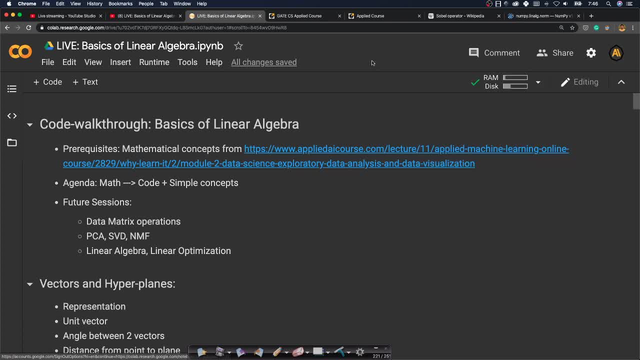 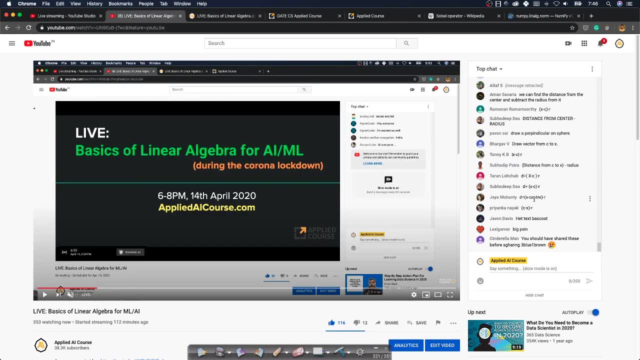 since we are at it. Anyway, I'll share this with all of you, right? So, please, please, give me a few minutes After this live session. I'll share it with you. So any questions related to this? Oh yeah, 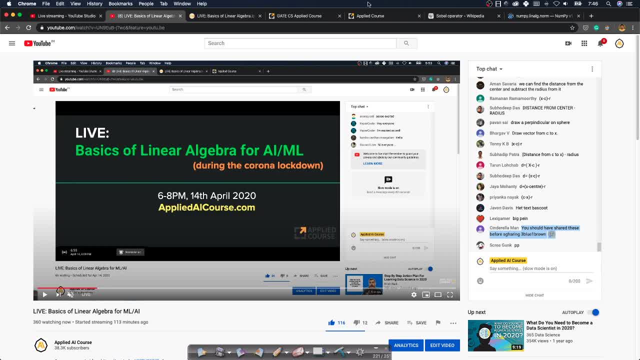 So somebody said you should have shared three blue, one brown. Yes, So that's a good point. I forgot to mention that three blue, one brown. linear algebra is also very good. I'm happy you mentioned this right. So three blue, one brown is a phenomenal channel which talks about linear. 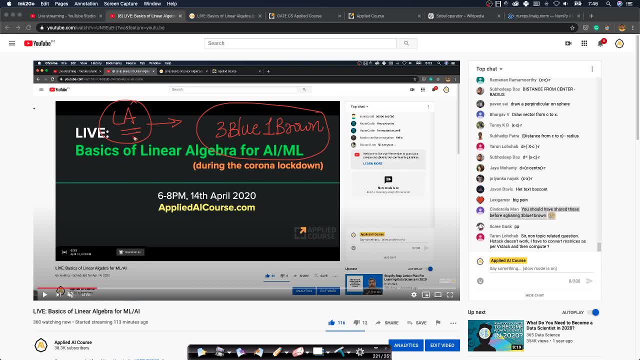 algebra videos: Again, all the linear algebra that you learn there may not be applied in machine learning and AI. Please don't forget that. right Again, we have also referred to three blue, one brown in these videos. Somebody says you should have done it, So don't worry. 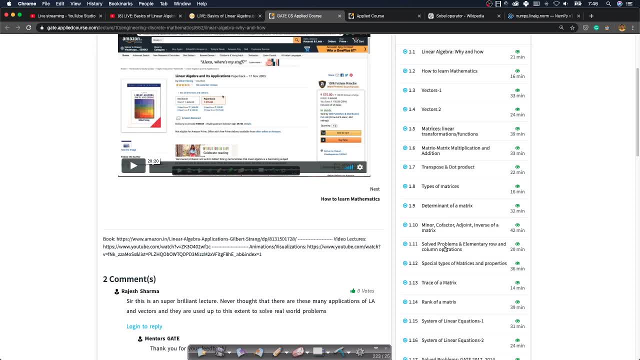 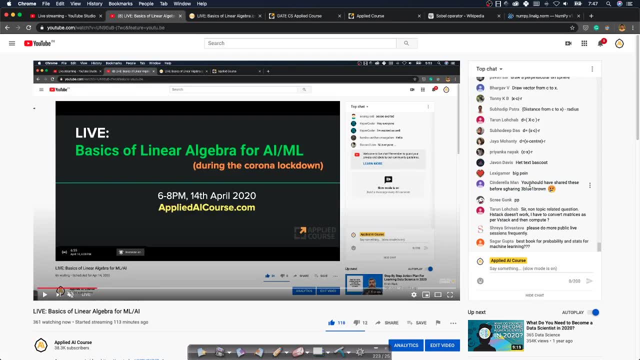 Even in our linear algebra videos. here we do refer to multiple textbooks, We do refer to multiple external resources. So we try to always point to good resources, not just our own. I hope you understand that. So somebody says: please do more live sessions more frequently Again. 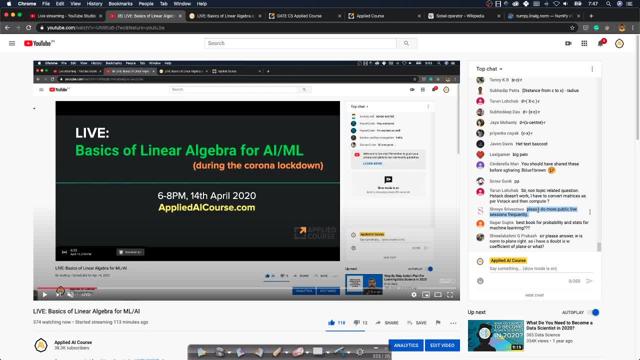 we are trying to do live sessions mostly whenever the topic is basic that anybody external to the course also can understand right. So if it requires students to go through our videos extensively, done our assignments, then we are not doing it externally because people may not benefit from it. 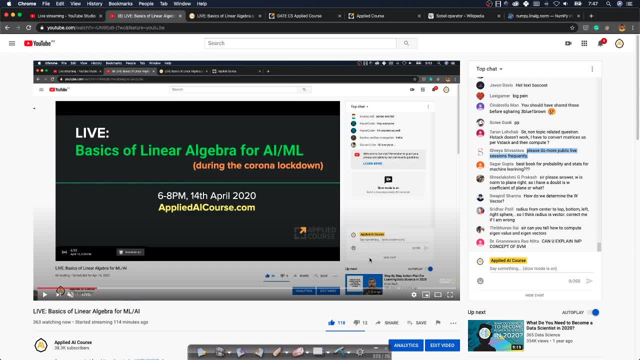 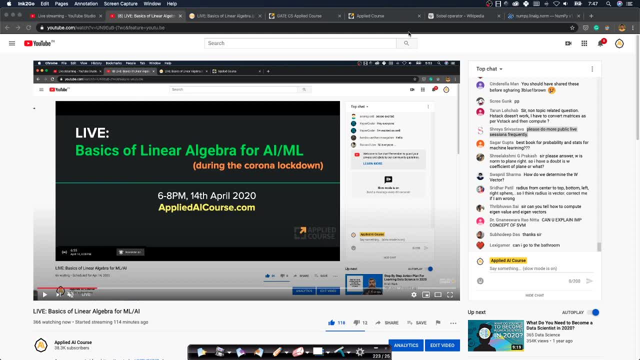 much right. So that's how we decide whether a live session should be public or private. Cool. Somebody says: what is a good book for? probability and stats? Oh, there's a very nice book. Again, there are multiple good textbooks for it, One of the best textbooks that I know of. 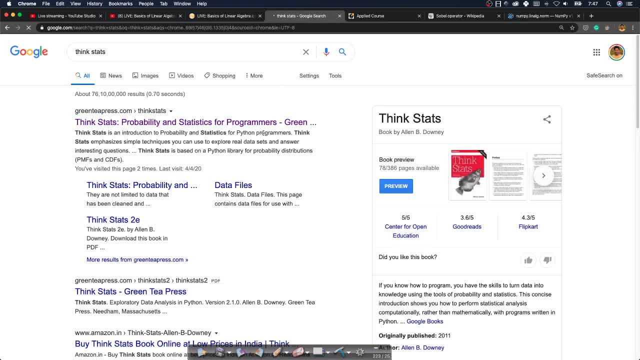 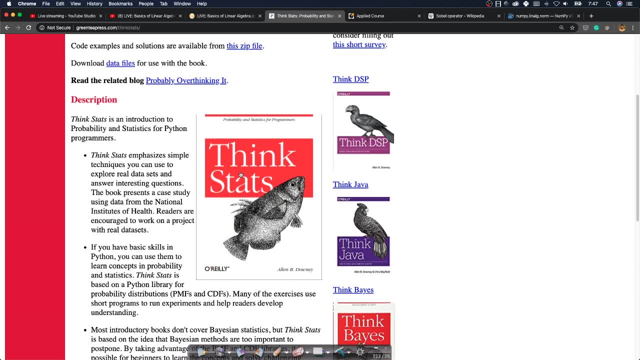 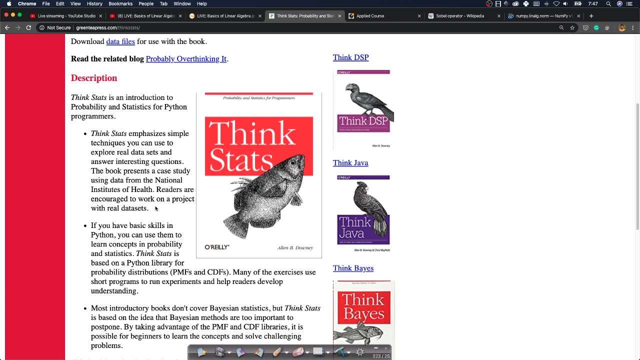 is ThinkStats from an applicative perspective. I like this book a lot because I think this book is also publicly available. Yes, you can. It's available to download in PDF. This is slightly less expensive, but it's a good book. ThinkStats is a very good book because they try to teach the 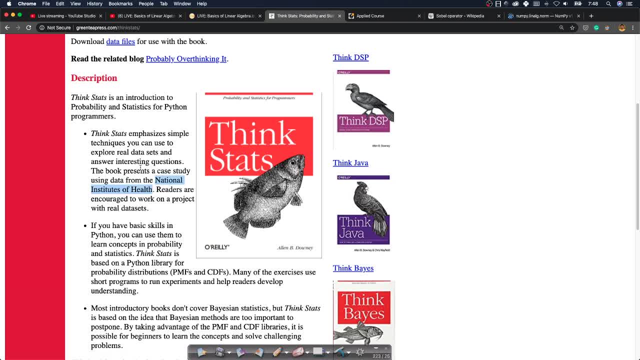 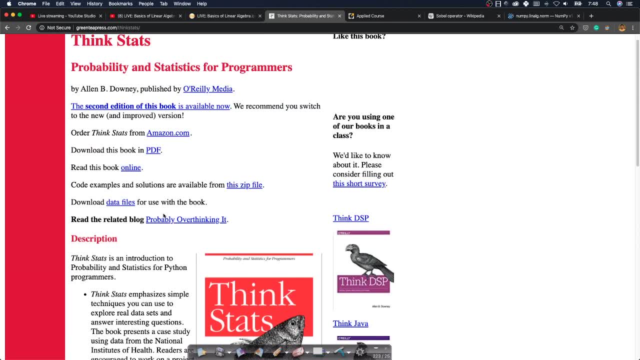 concepts by using a real world data set. So they take data for data set from National Institute of Health. They take an actual data set and they try to introduce concepts from the practical perspective. It's one of the best books from a practical standpoint. There are a lot of good. 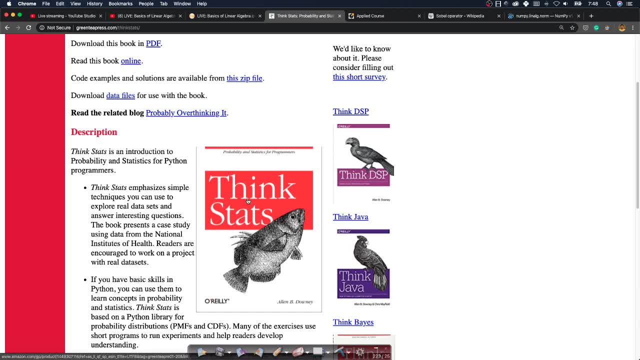 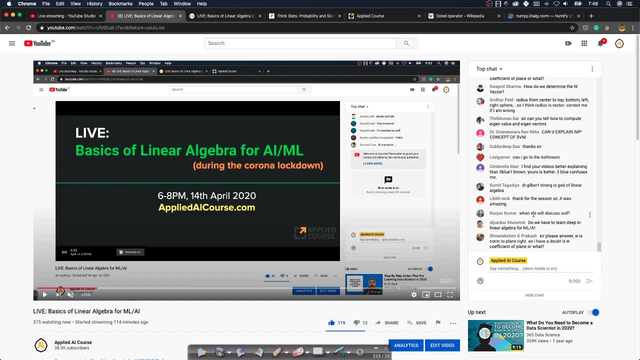 theory books, but for a, for a machine learning, you have to know how to apply things. So ThinkStats is one of my favorite books. So when will we discuss SVD? We'll discuss it when we do live sessions on recommender sessions. 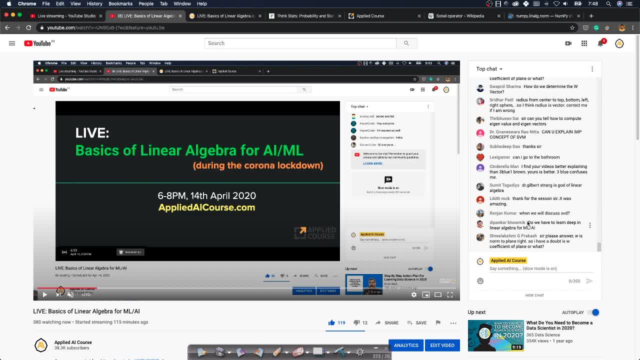 Do you have, do you have to learn deep, deep in linear algebra? for machine learning, AI Again, what is depth? That's my question, right? So what do you define as depth? I've listed all the concepts here, right? I've listed most of the concepts, if not all the concepts. So, for machine 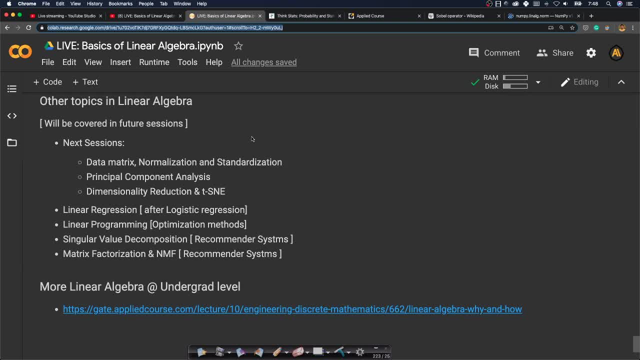 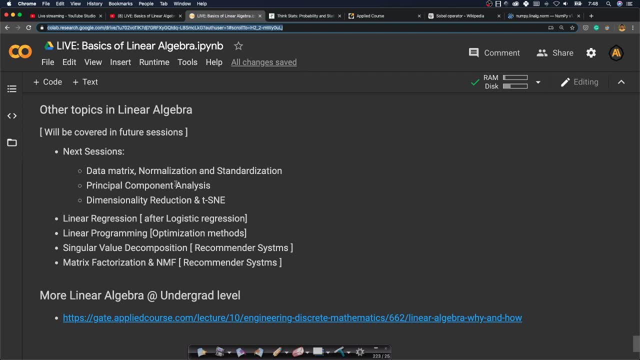 learning at various points. you need various concepts. The concepts that I just discussed right now are the foundations, but you need to know a lot of other concepts. These are all the concepts that you need to know if you really want to become a good machine learning engineer. 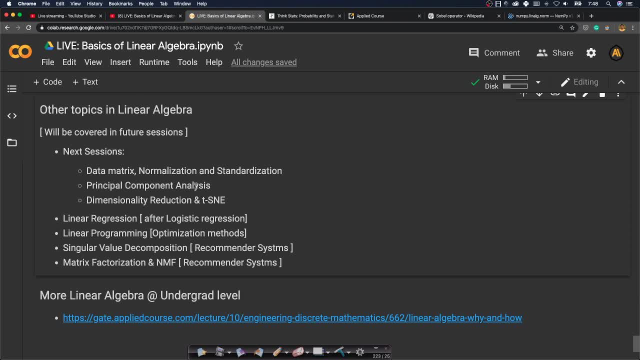 So the first concept is linear algebra. Again, this is not all that is there in linear algebra. There are many other concepts in linear algebra, But these are certainly what you need to know for machine learning. You can think of it as a good set of concepts, Cool. How do we determine the W? 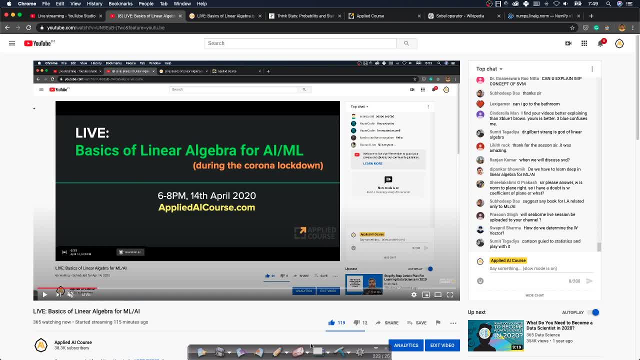 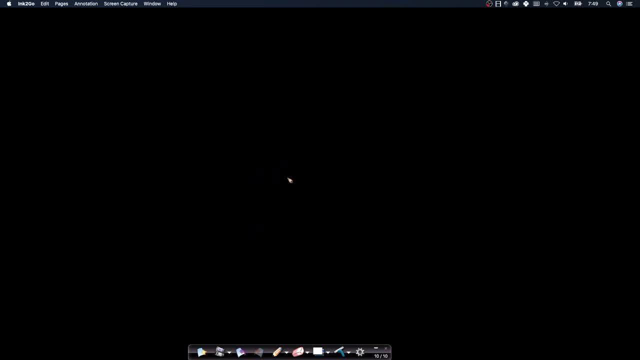 vector. Oh, so you're saying okay, so that, Okay, good point, So we determine so, Okay, so let me. let me try to answer that question briefly. So in linear regression or logistic regression or SVM, we try to find a hyperplane that separates positive points of the matrix alpha to positive points of the vector alpha적. 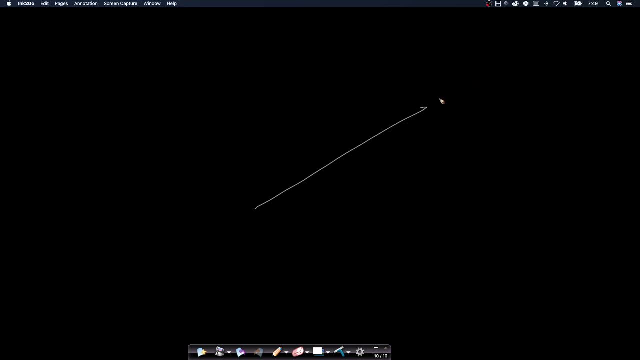 points from negative points. again, those of you who understand it can understand it perfectly, but we try to find this hyperplane. if you have a hyperplane, hyperplane basically has two, two parameters right, w and b. so this is my w and i have a b corresponding to it. we try to find this. 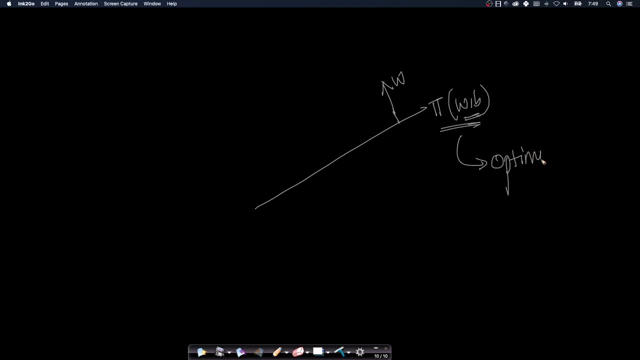 hyperplane by solving a mathematical optimization problem. look at it. we have done a few live sessions earlier, right, where we talked about maxima and minima. right again, these are concepts that you may have learned in your undergraduate level computer science. sorry that you may have learned. 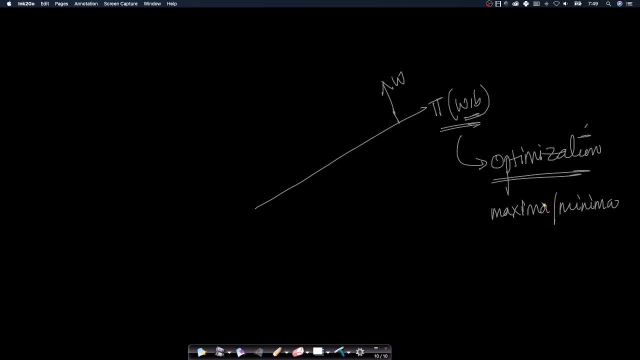 in 11th and 12th class mathematics, not even undergraduate level computer science, right. so optimization is basically a simple extension to concepts of maxima and minima that you learn in your 11th and 12th class. if you recall, we have actually discussed this in the previous live. 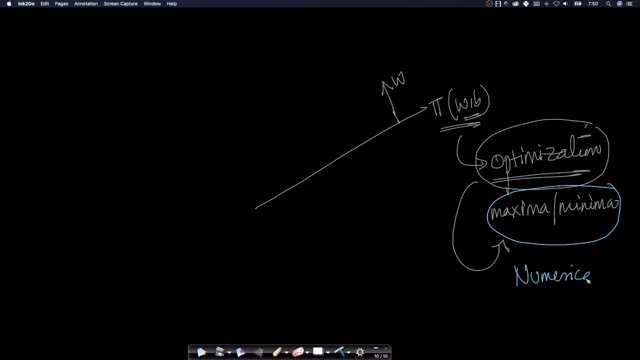 sessions in our numerical. again, all of them are available on youtube. it's called numerical programming. okay, so we have done two sessions numerical programming, one and two. so we've actually solved some problems. using maxima minima, the same concepts are used, but it, but certainly at a next level when you want to find w right. so that's how it's actually. 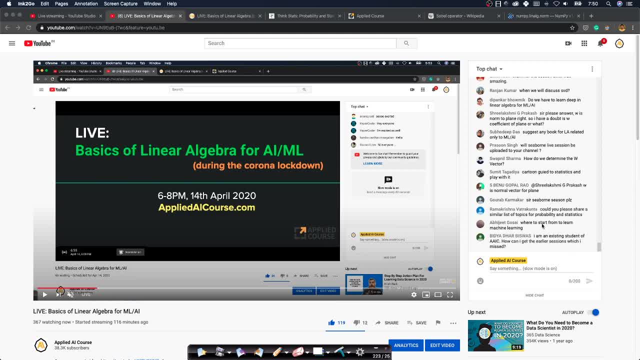 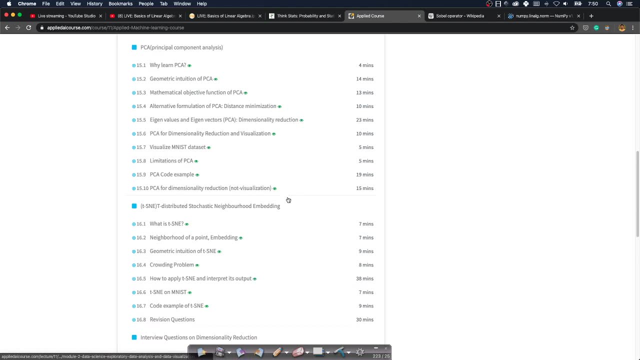 solved in the real world. so so could you please share similar list of topics for probability and stats? again, if you want a good list of topics, uh, the the textbook is certainly a good starting point. again, if you want a list of topics, you can always go to our website. 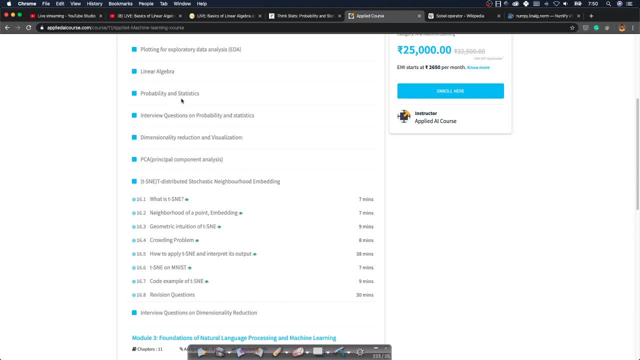 you can go to our website and you can go to our website, and you can go to our website and you can find the list of topics that we think are very relevant. right, so you can just go to probability and stats. these are all the concepts that we think are very important for somebody who is picking up. 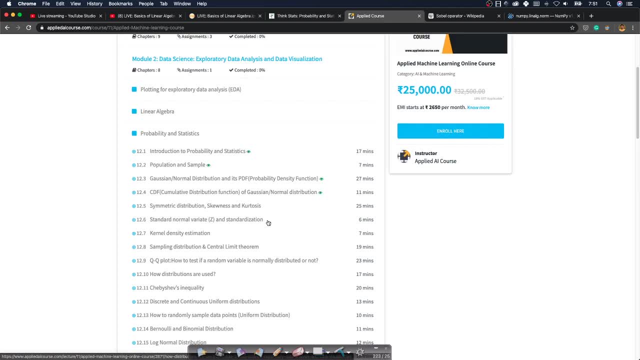 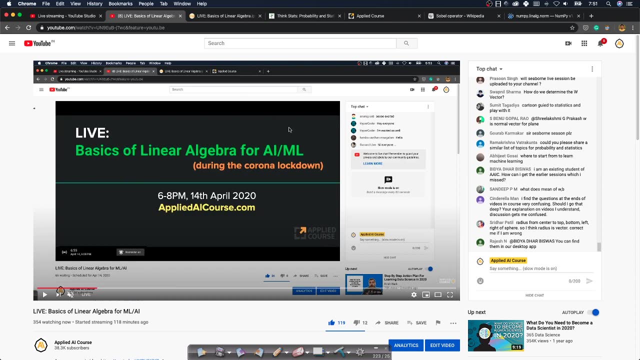 machine learning and deep learning. this is a good. again, this is just a subset of topics. you can always go here. you'll find a list of topics. topics is easy again, but please remember that no topics list is static. things change right, so you have to evolve with it again. it's all almost impossible. 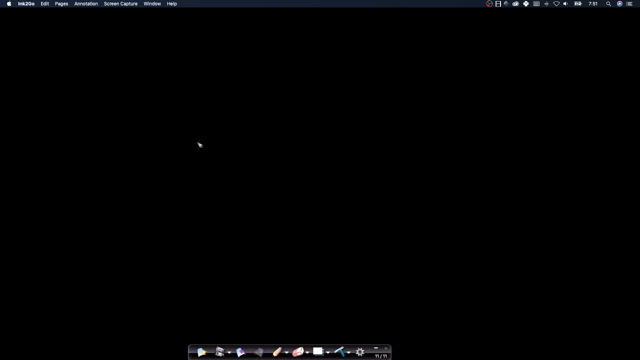 to do depth first, as i've just mentioned a while ago. please don't learn depth first. please learn breadth first. learn little bit of linear algebra- that you need. learn little bit of programming, little bit of data structures and algorithms that you need. little bit of probability and stats that you need. little bit of optimization that you need. 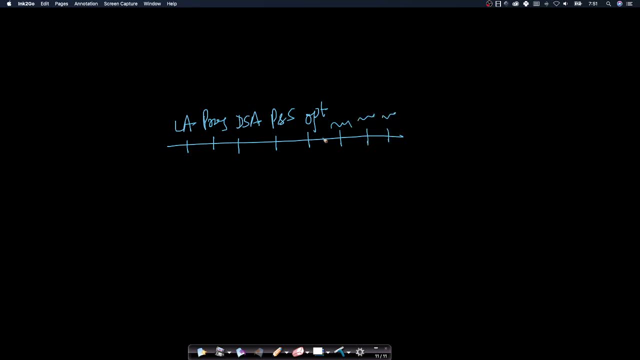 little bit of machine learning techniques, little bit of clustering techniques, little bit of deep learning techniques first. well, after you learn all these basics, then you can say: okay, i want to go deep into linear algebra, or i want to go deep into programming, or i want to go deep. 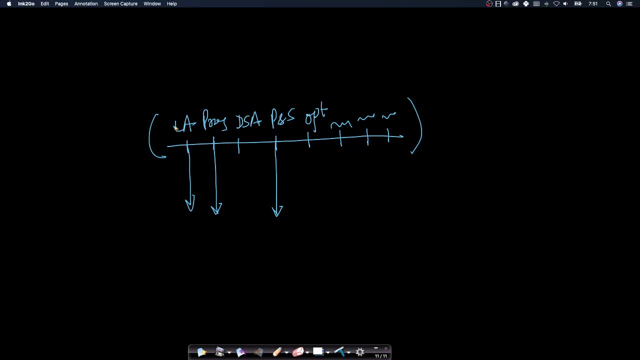 into probability and stats. this is what we recommend, because we want to go deep into probability and stats, because when you learn the breadth of concepts, you can start transitioning to machine learning and data science careers. there is no limit to how much you can learn. as i told you like, i've been reading research papers for the last 12 to 13 years. 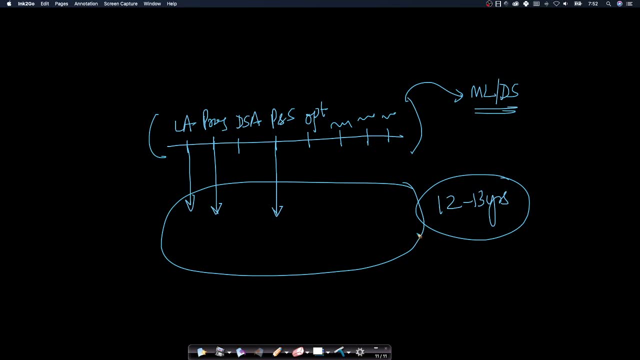 and there is no end to it. it's almost impossible to keep track of all the advances. even let's take a very simple area right: probability and stats. there is so much of great innovation that's happening in probability and statistics that it's impossible for any single person to keep. 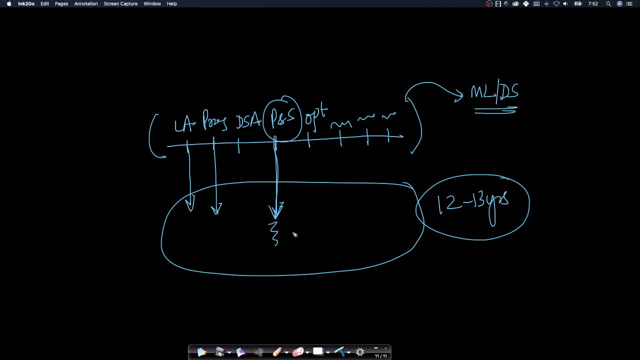 track of everything right, but i try to do my best to go deeper into each of these things a little bit topic whenever i get some time. okay, first breadth is important, then depth. if you try, if you do depth first, you will never. you could. you might become an expert in linear algebra or you might become 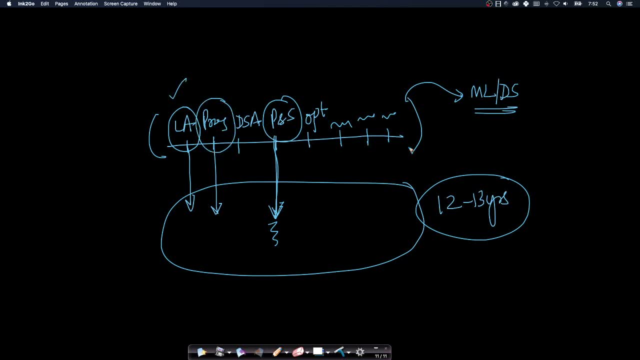 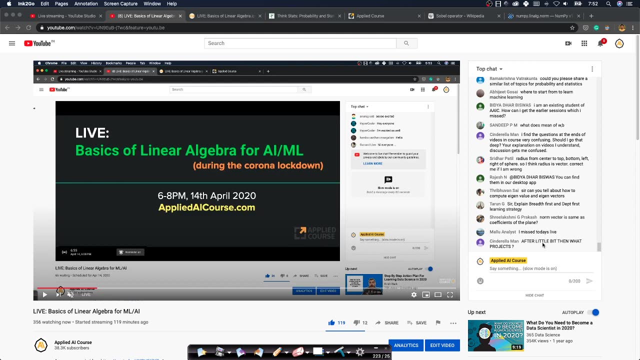 an expert in programming, but you'll never become, you'll never have the breadth of expertise to become a data science or machine learning guy. uh, okay, uh. so somebody says how to compute eigen values and eigen vectors. again, it's simply a simple function in numpy. again, that is something. 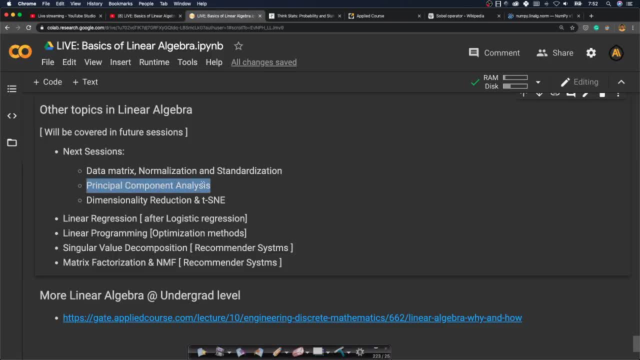 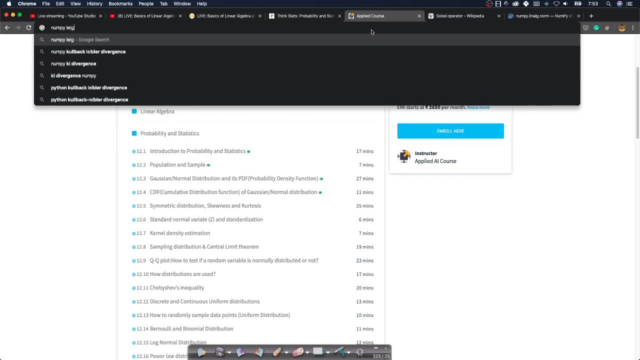 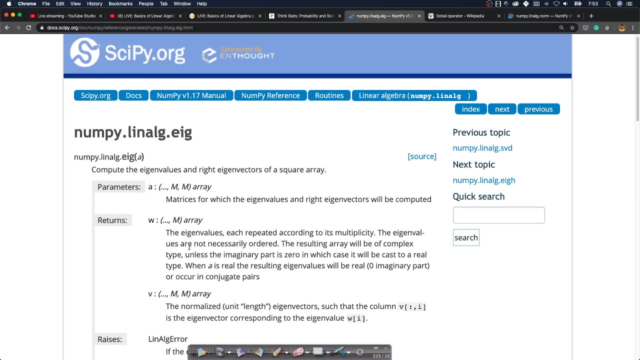 that we thought we'll discuss when we learn principal component analysis, because it requires eigen values and eigen eigen vectors. again, if you want to know that, right, it's actually just numpy uh, eigen values, just google search, okay. so in numpy linear algebra there is something called eig. read up the documentation, okay. what does it want? eig a? a is basically matrices for 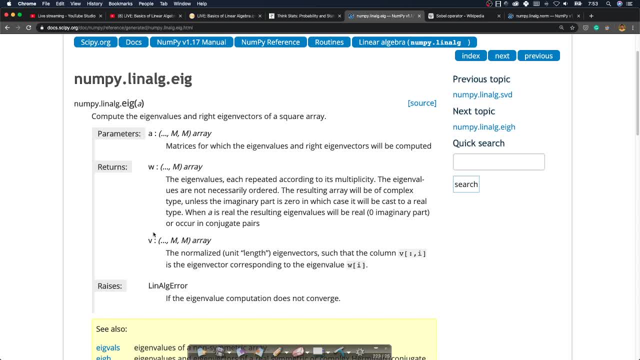 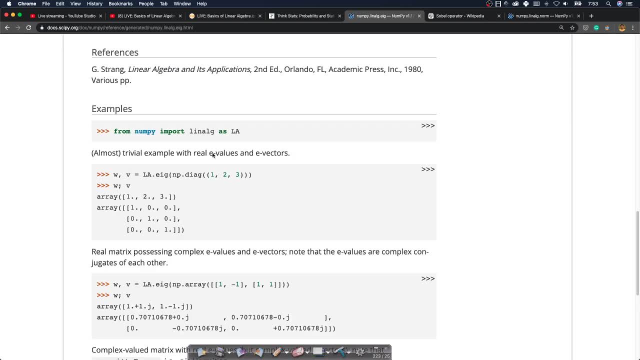 which eigen values and eigen vectors will be computed. what does it return you? it returns w and v. okay, it returns eigen values. it returns normalized eigen vectors. that's it. there is sample, there is sample code here. like it's it, it took like: even if you don't, 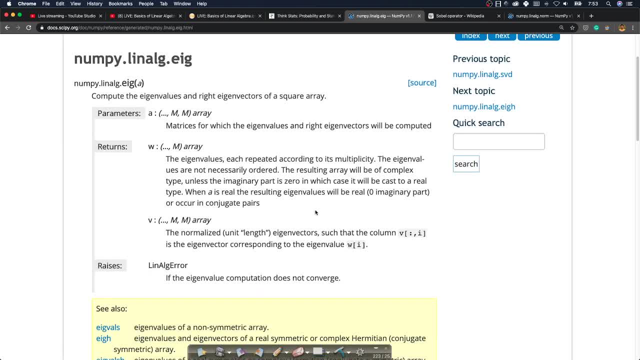 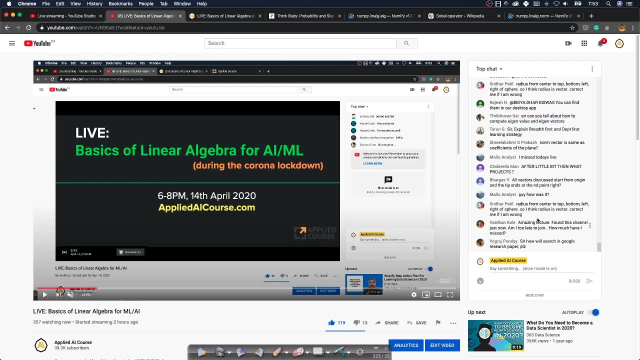 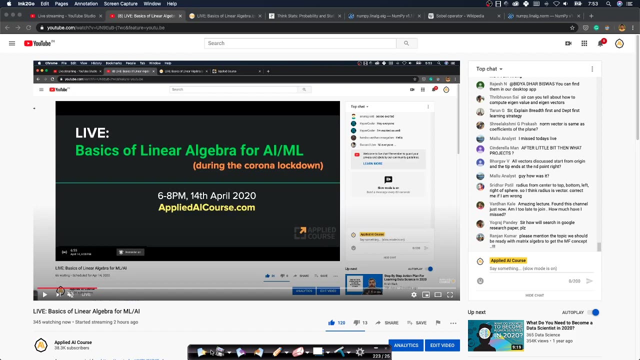 remember it, it takes 30 seconds to figure it out right, so it's actually fairly easy. so somebody's saying radius should be a vector. why should it be a vector? i thought it should be a scalar right? so i also got confused with that when i was writing the notes. so imagine: 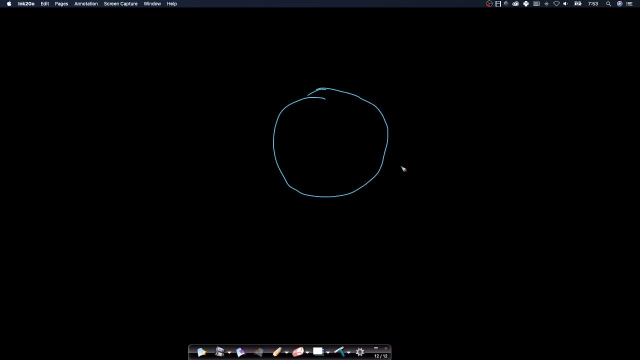 if this is my, so if this is my sphere, okay, think of a sphere, right, sphere. okay. again, i couldn't draw a sphere here. sphere on x-axis, on y-axis and also on the z-axis. the radius is the same, right, because if i change? so let's, let's take a circle, right, let's take a simple circle. 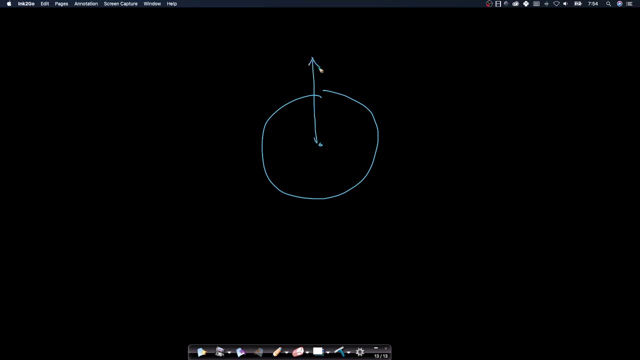 the circle. right circle is 2d, right, right, this is my x-axis and let's say this is my y-axis. let's just say, let's just say: right, so my radius, oh okay, so my radius on the x-axis is the same as the radius 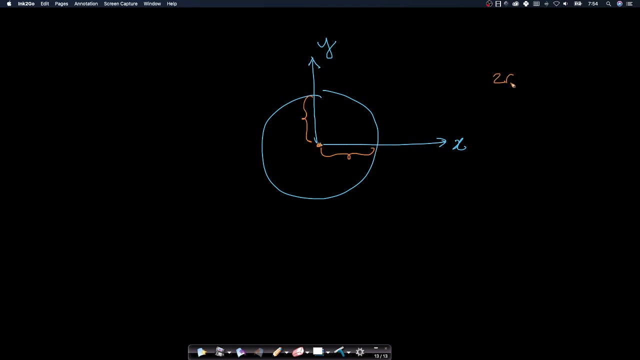 on the y-axis there are no two different radius. so in 2d space i have only one radius. now, if there are two different radii, right. if this is different from this, what do i get? what i get is not a circle. what i get is an ellipse. think about it, right? so imagine? okay, let me change the diagram here. 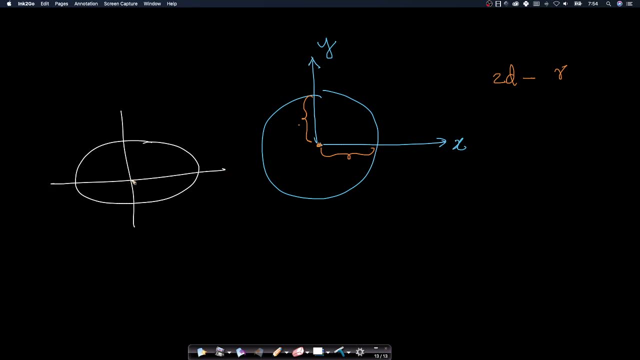 imagine, if i have this right, if this is different from this, what i get here is actually an ellipse and not a sphere. so for a sphere, the radius should be the same. actually, i think i messed up, because i was also thinking of hyperspheres in my head- hyperspheres. 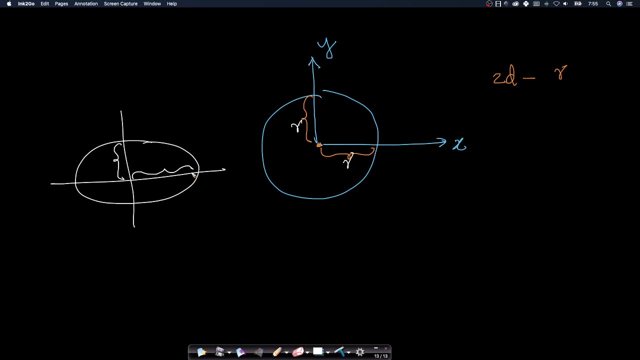 have a different way of encoding it and we don't use hyperspheres much in machine learning. that's why i did not cover it. uh, sorry, hyper ellipses. sorry, these are hyper ellipses, not spheres. all right, even, uh even, hyperspheres, the very few times used, i mean. i mean i, i don't use them regularly to. 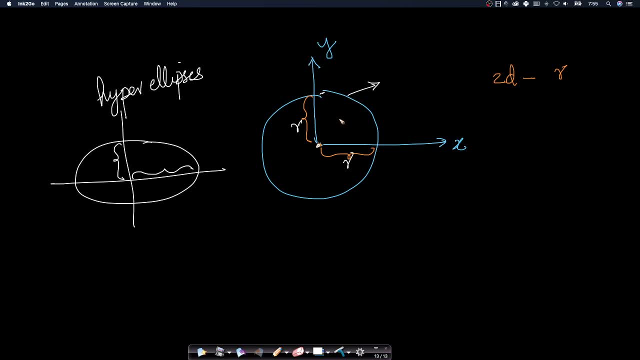 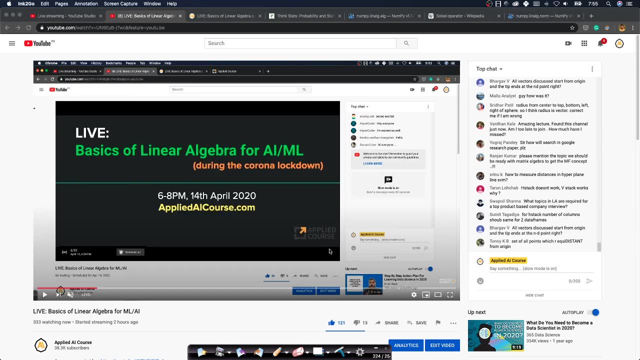 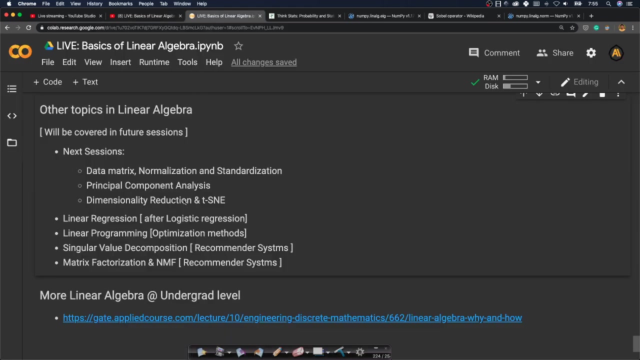 i don't use techniques which use hyperspheres regularly, but there are one or two odd data mining techniques which use it right. that's why i thought i'll cover it again. what topics are required? as i just mentioned, all these topics are required, for sure, for top product based companies, no doubt hands down. 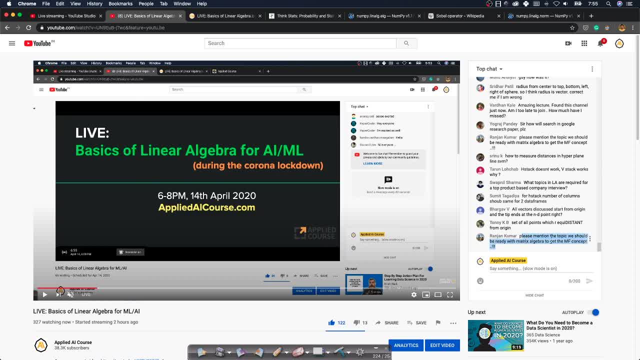 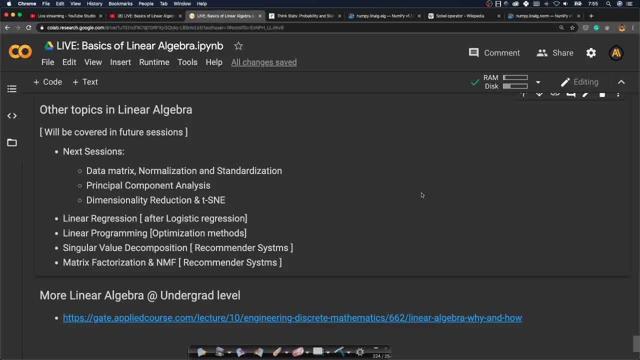 so please mention the topic which you should be ready with me. so let's start with the topic of matrix algebra to get matrix factorization concept again. don't worry about it, matrix factorization is just about matrix, matrix multiplications. if you know how to multiply two matrices, you have the basic knowledge for matrix factorization. 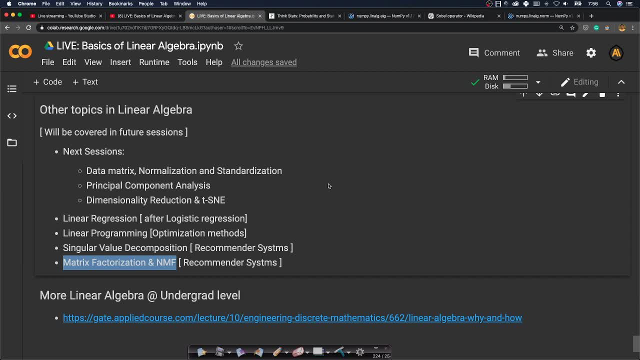 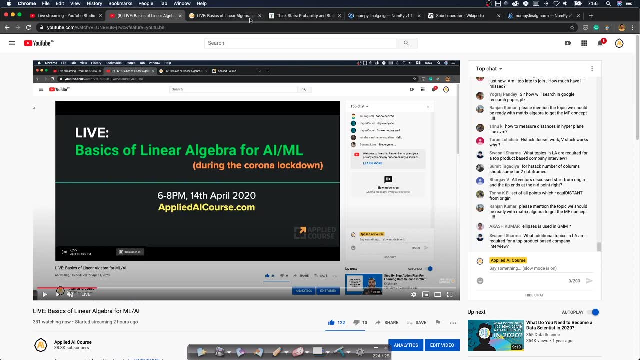 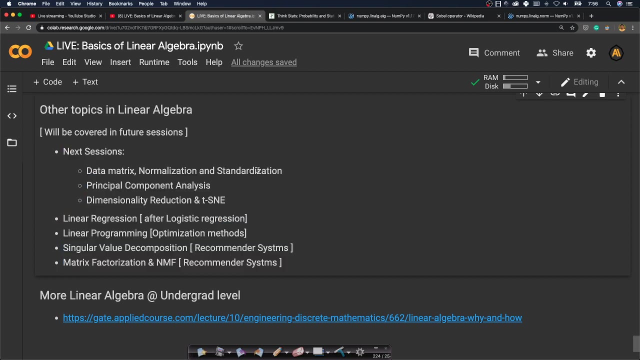 right again, matrix factorization and nmf are solved using optimization techniques. cool, i think, swapnil, i just mentioned this right. i think this is a good starting point. again, most of the questions that i remember from the interviews are mostly revolve around these. of course, there are real world problems asked to you. 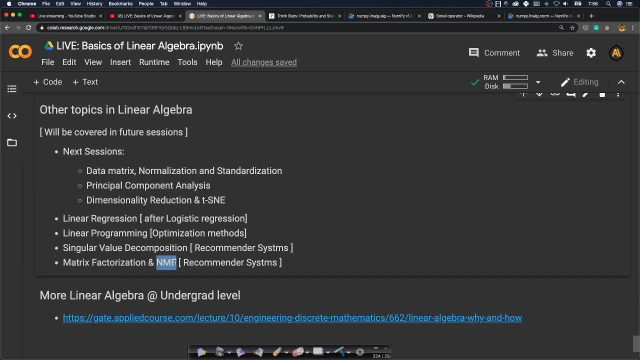 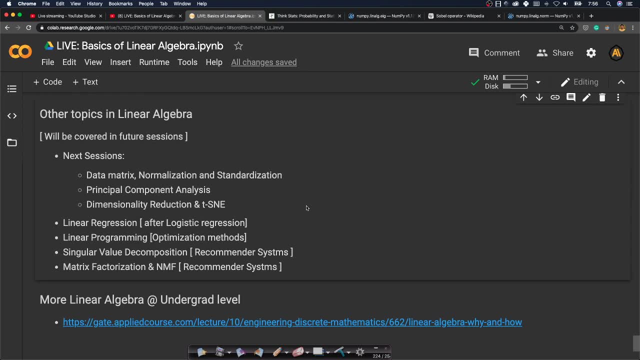 and people ask you: okay, how do you solve? how do you do? how do you do so? and so, how do you do matrix factorization when the data has this problem right? or how do you do uh, how do you do? let's assume, for example, take linear regression, right. linear regression can be, you know, understood from. 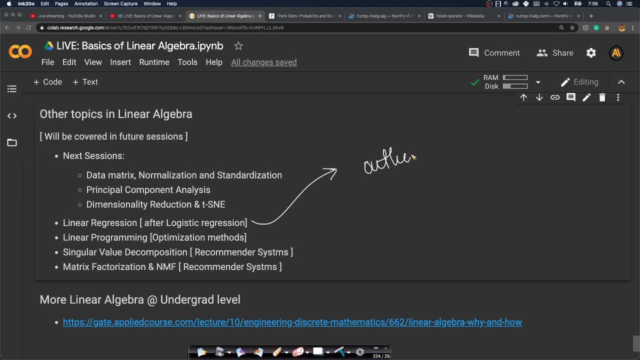 a linear algebraic perspective. what if your data has outliers? what happens to your linear regression based model? right? or how does singular value decomposition or pca behave? if there are, if there is noise in your data? how does it work? right? these are actual questions that i have asked in interviews. right, if you take non-negative matrix factorization, what happens to? 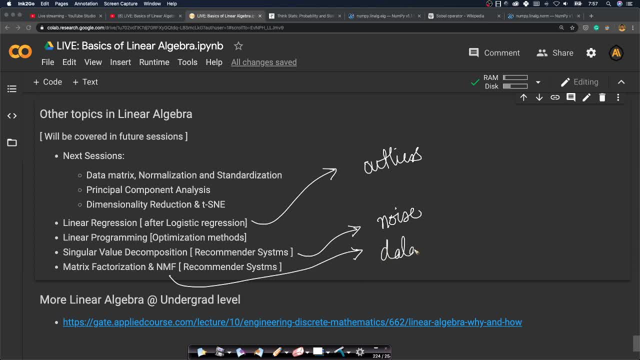 non-negative. how do you do non-negative matrix factorization when the data is very large? again, people may not ask you just the mathematics. people ask you again to answer some of these questions. for example, what happens to outliers? to answer this question, you have to know the. 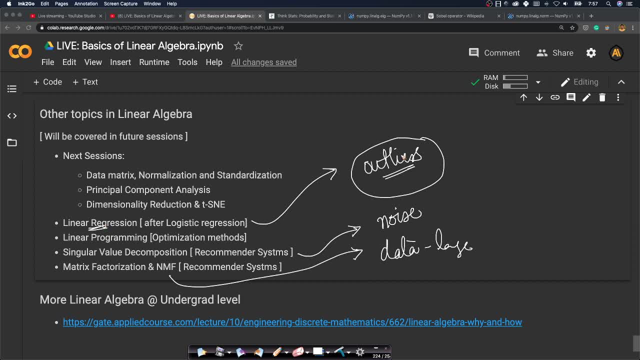 mathematics and you have to be able to apply the mathematics in the context of their outliers. right, how does nmf work if? if there is a large amount of data, to understand this you have to know the nmf mathematics internally. so a lot of questions are not like, okay, explain me the optimization. 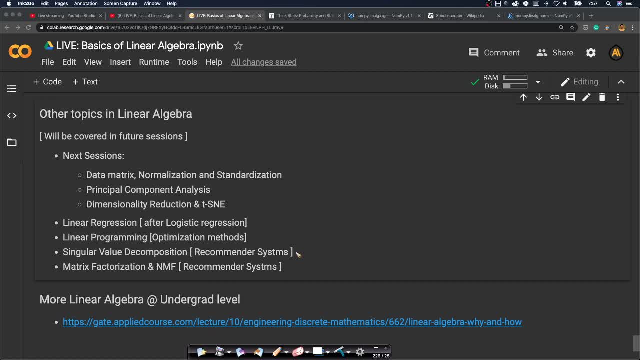 problem for nmf. that's a joke, right? or the more the more real product based company questions are okay in nmf. why do we have regularization again? regularization is another concept which we learn in optimization, which which is also sometimes covered in the in the linear algebra courses, right? so again, lot of things that are there in machine learning. 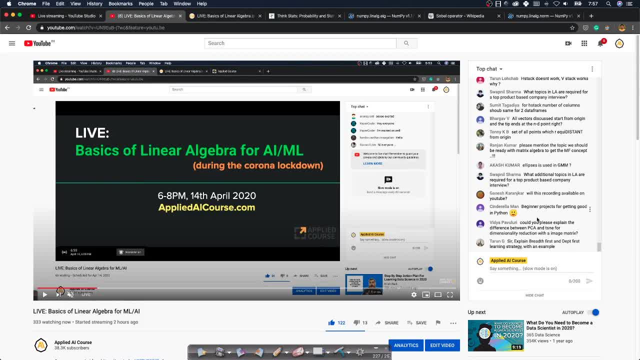 can be seen from a linear algebraic lens. uh, oh, this cinderella man. i know this guy okay. so you're asking about beginner projects to become good in python, right? so that's very simple. i've mentioned this multiple times, right, pick up. i mean just, instead of doing full projects, write code. i think i mentioned this in the previous sessions. 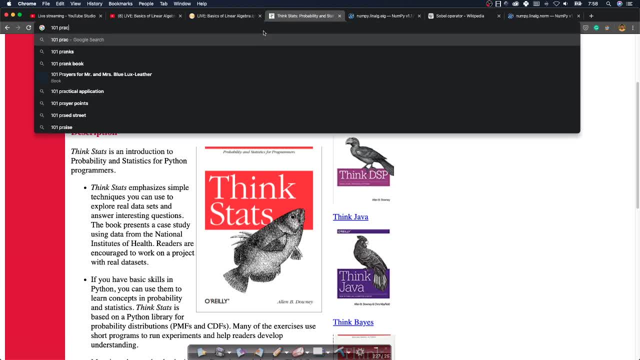 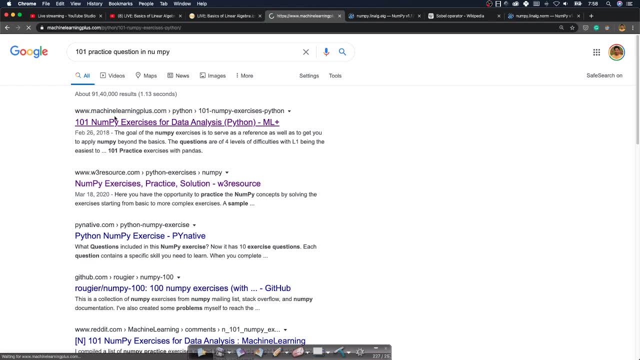 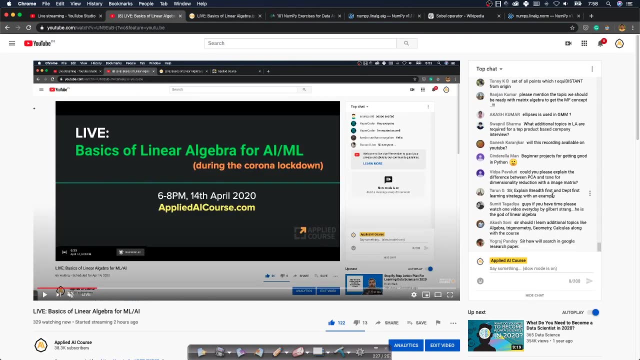 also right. there are these 101 practice sessions, 101 practice questions in numpy, most Hessian fc dependent phases one to three. i think i mentioned this. okay, i mean just google search. practice questions in numpy, practice questions in pandas. instead of doing full-fledged projects, try to get the breadth of experience first, then you can do projects. 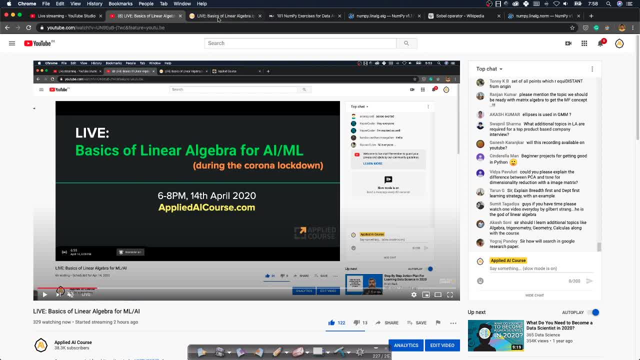 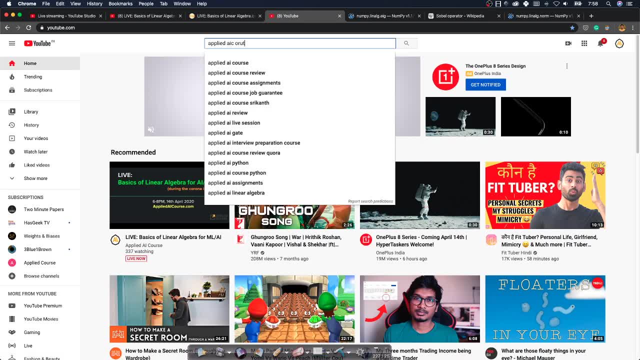 right, because the projects that you can do with basic python are fairly limited. okay, there is one live session that we have done that could help you if you want to do projects right, so let me show you. uh, let me just go. i'm just thinking. applied a course web api. 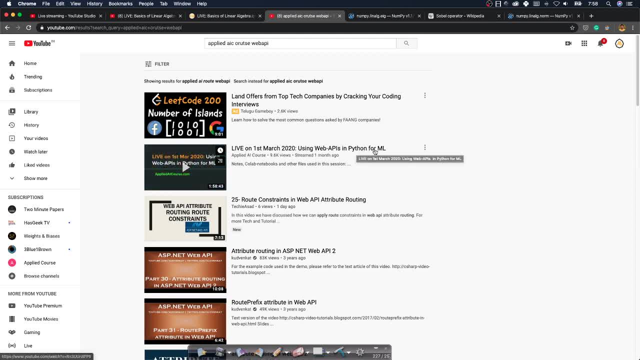 okay, so that we have done. using web apis in python for machine learning. again, you can use a lot of web apis and build some simple machine learning solutions. so this live session- again, this is publicly available on youtube. you can go check it out again. you can use web apis from google azure. 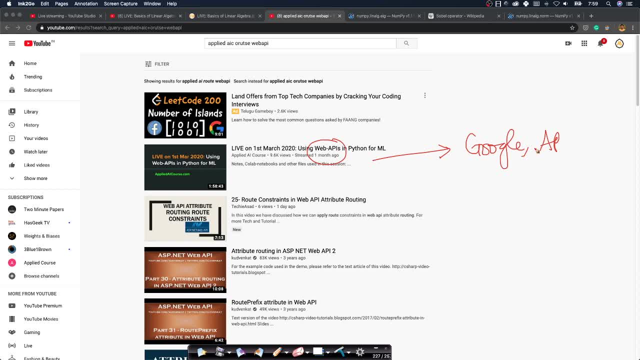 all these guys and again, all you need is basic. so google azure right. they give you a lot of nice machine learning functionality with just a api call. so if you want to become better at python also, you should practice problems, without doubt. but if you want to do a simple project, you can. 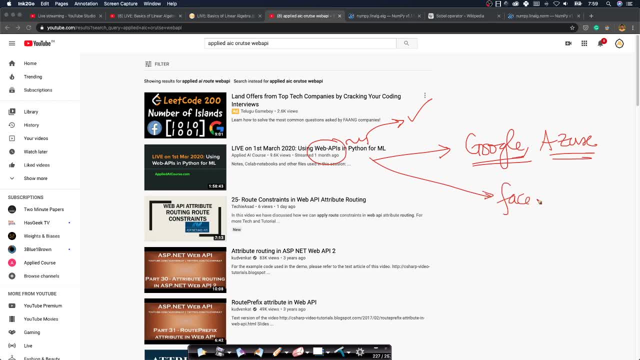 use this web apis and build a simple thing. you can build a simple face recognition system, right. you can do a simple speech to text or do a simple chat bot. again, we have a live session on how to build a chat bot also. i think it's also on youtube. we've done it more than a year ago. 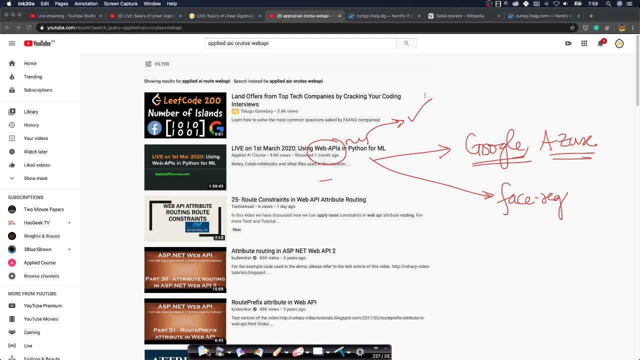 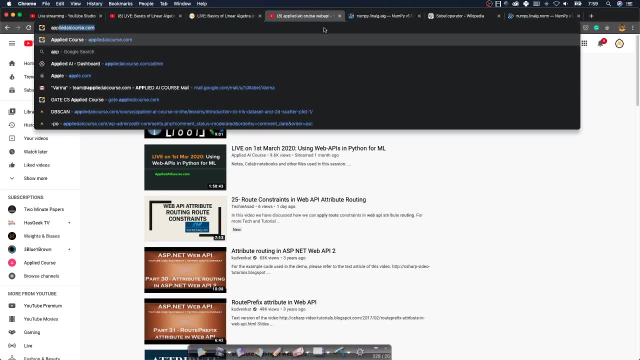 right. so there are some of these live sessions that are publicly available that you can check it out again. if you want to check out all of our live sessions in one place, we have put it in one place. we just did that recently because it's hard to maintain everything. so if you just go to live sessions, link here, so all of 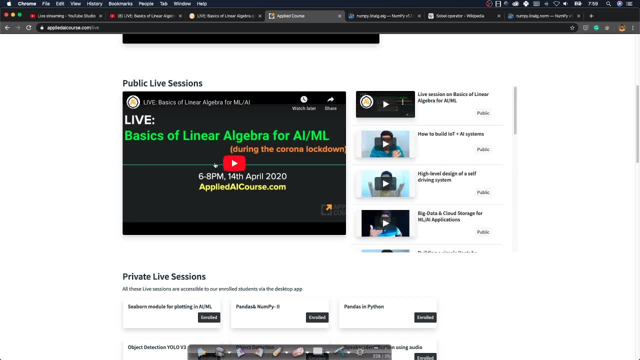 our public live sessions. there are all these public live sessions. all of our public live sessions are accessible here. right, so you can just go here. so how to build this high level design, right so? web apis: how to build a simple youtube recommendation using basic mathematics. the live sessions that we have done recently: right, there are some live sessions earlier. 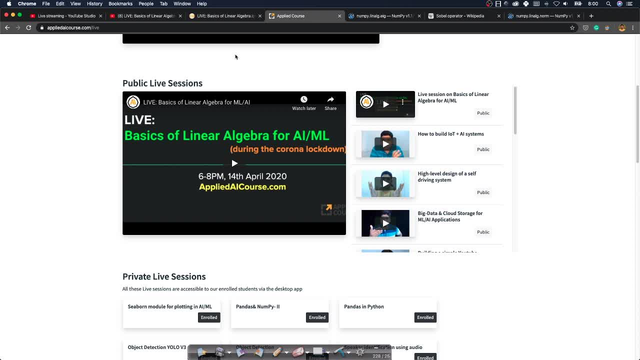 so my suggestion here is there are a bunch of live sessions that are publicly available for you to do, live sessions on how to build a chat bot. so if you want to build a chat bot from which you can build a simple project if you choose to uh, or how to search for a research, 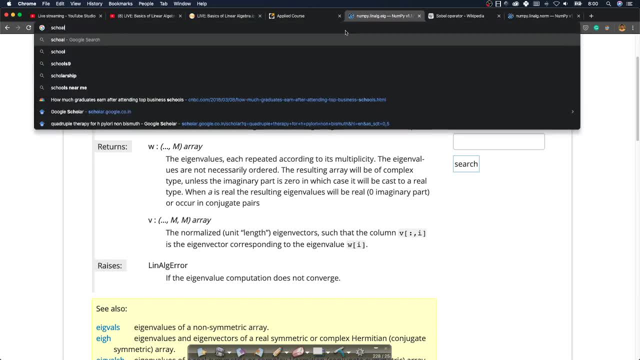 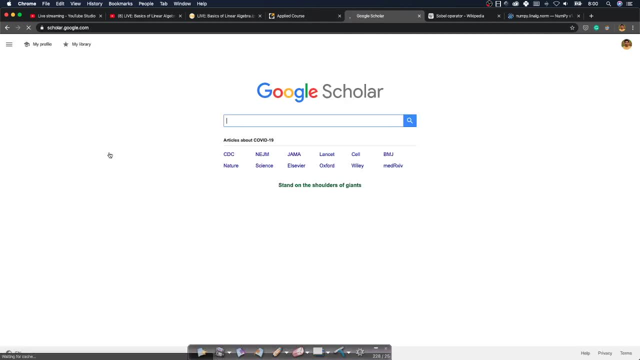 paper. that's a very good question, so the way i do it is this. so i think many people don't know this- go to scholargooglecom, scholargooglecom. google scholar is the best tool that i know of for research, right, so again, this only gives you research papers. for example, if i want a research, 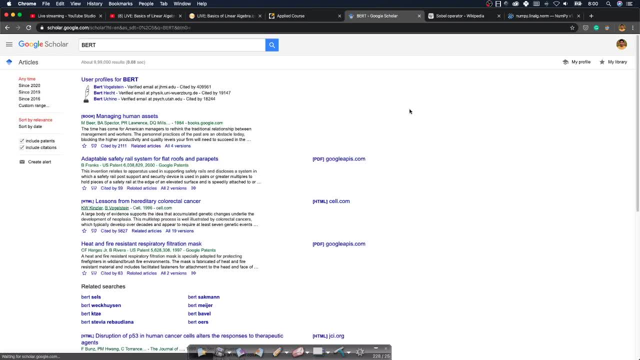 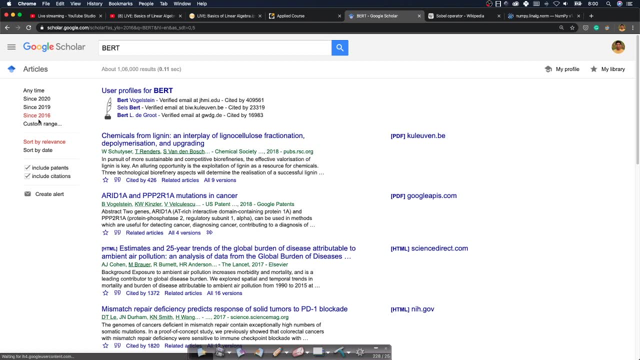 paper on bert. okay, i just search bert. okay, so i can, i can filter it, okay. so, bert, okay, it's giving me multiple papers. so if i say from 2016, it gives me all the papers again. this gives from a whole of science, not necessarily deep learning, machine learning, etc. 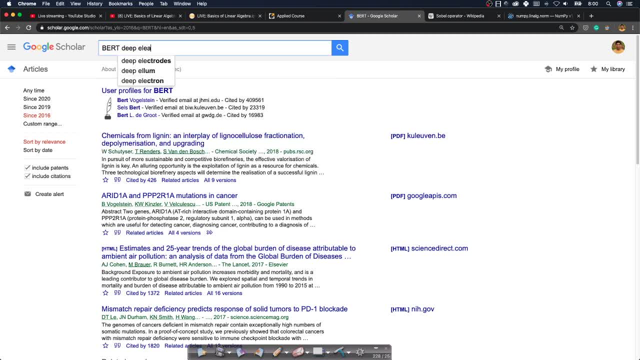 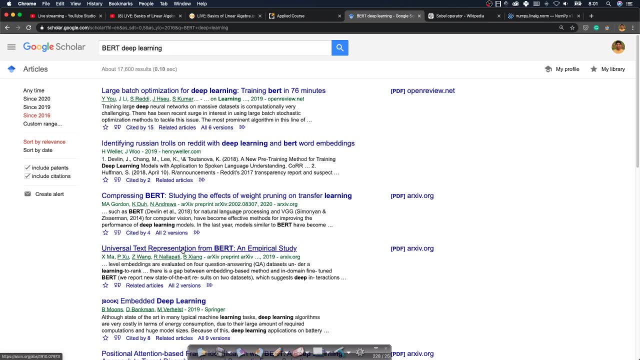 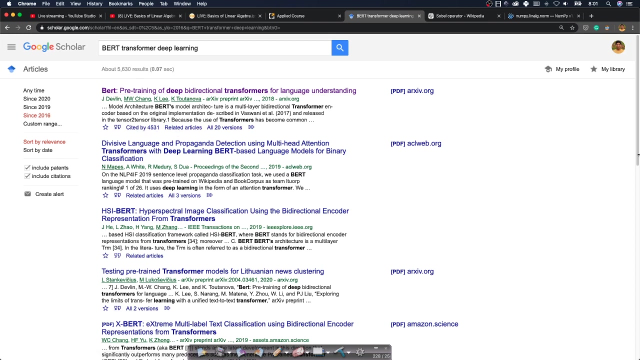 so deep learning, okay so, so this is whole of science, but deep learning from 2016? i get a bunch of papers, but why am i getting? why? large batch optimization, bert, uh, transformer- i think the keywords are messed up. okay, so, yes, this is the paper. again, whenever you are picking a paper to read, it's very important. 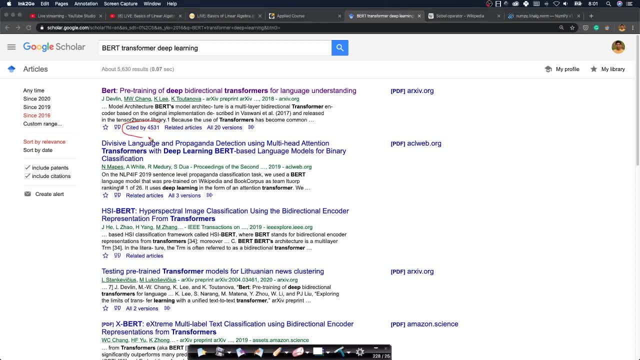 that you pick papers with lot of citations. the citations tell how important this work is. remember: this paper was published in 2018 and this already has 4531 public citations. what is a citation? i write a research paper and i refer to this research paper. i say, okay, bert, which is? 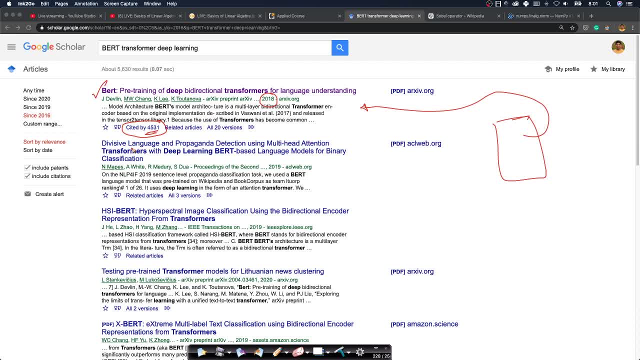 which is discussed in this paper. so if i cite this paper, i get a citation. so there are 4531 other research papers that refer to this research paper. that's how important this research paper is right. so you should always look at citations if there are not enough citations. 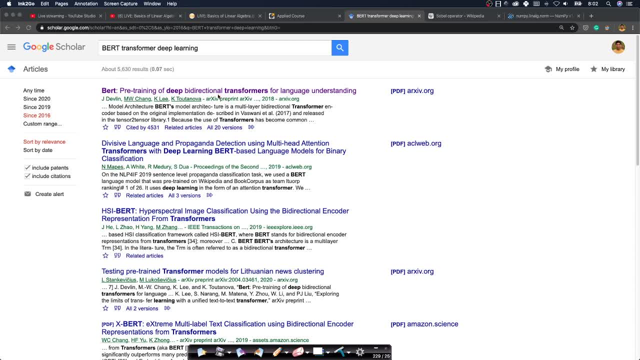 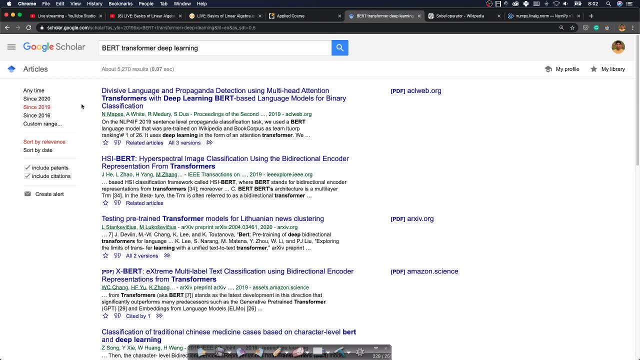 maybe it's not such an important paper. to be honest with you again, citations can also be biased. there is some problem with citations, but if i want papers from 2019, let's look it up. okay, i can also sort by date sought by relevance. there are multiple sort options, right? so my suggestion: 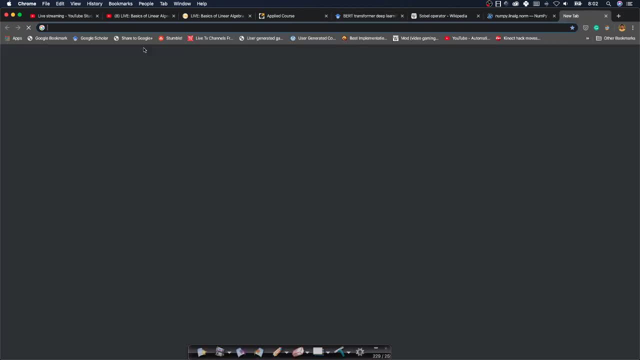 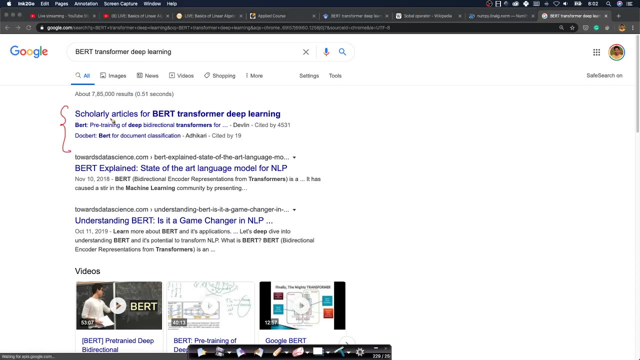 always is to use google scholar. again, you need not always use google scholar if you just go to google and search this. it also says: look at this. it also says this at the top. it says scholarly articles of birth transformer. it tells this also right. and it says, okay, this is the top paper. it. 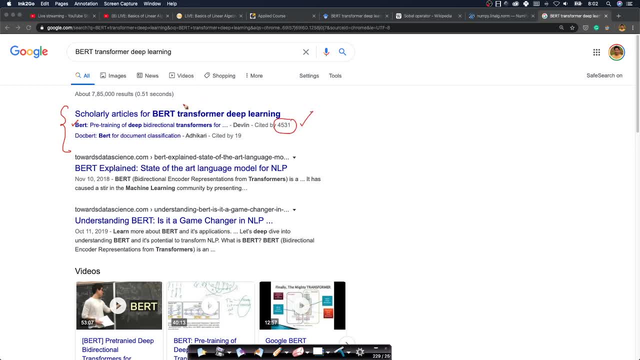 is cited by 4531. so i i what i do is i directly search on google. i get some papers here. if this has high citations, i go to google scholar and search. okay, otherwise you don't get blogs, and all that in google scholar, so right. so the second place is there are tons of nice blogs on birth. 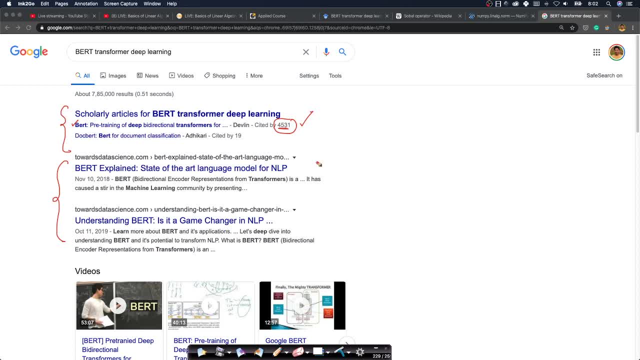 so, whenever you're reading a complex research paper, if there are other blogs which explain the research paper, i recommend that you first read these blogs, because reading a research paper is written for other researchers to understand, and if you are already not at the research level, probably it's best to read others blogs because you can easily understand this. this is written. 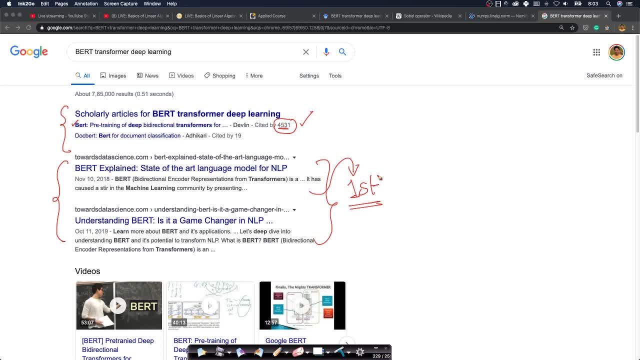 for more students, not at cutting edge researchers. you, once you understand the basics, then you can read the research paper, because research papers are actually written for researchers very often. so don't try to understand the research paper in the first go. very again, if you have spent years together doing it, you will understand it. but 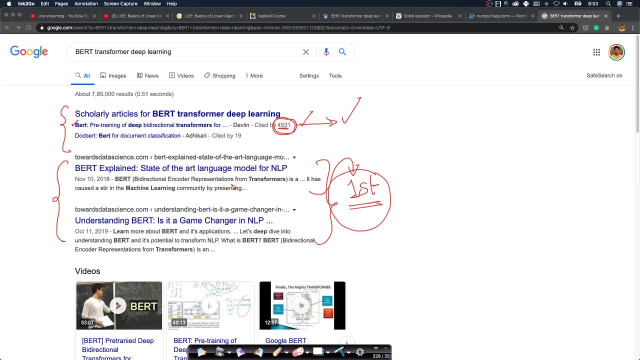 otherwise, when i was a student, reading my first research papers, i would read blogs. if somebody has written them, that's the best, that's a good starting point- and then go and read the research paper at the end. that's what i would recommend. cool okay folks. uh, sounds very good. thank you. 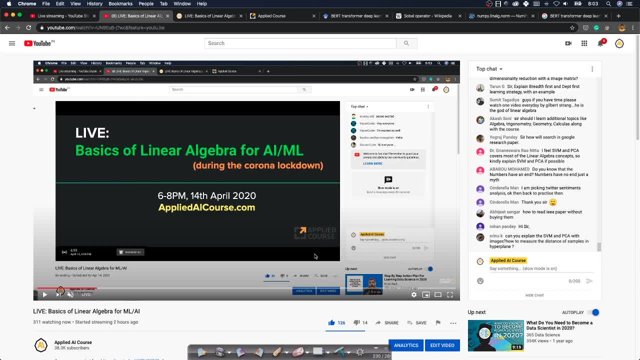 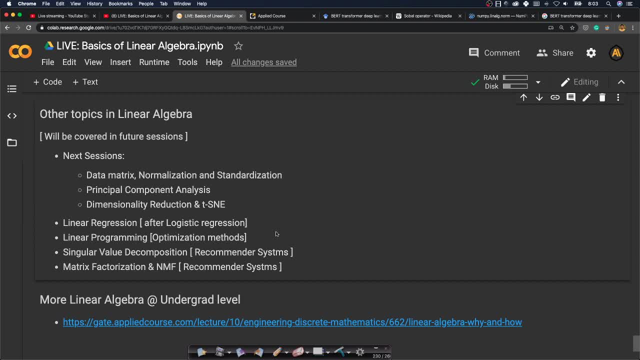 very much uh and uh. what we'll do is: uh, i'll post this, i'll post this. uh, uh, post this ipad. uh, post this collab notebook in the comment section and i'll also post it in. uh, i'll also post it in in in the 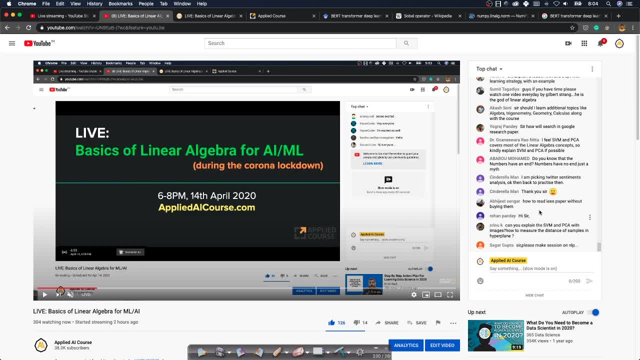 description section of the video. okay, thank you very much for joining in. uh, see you again, bye. 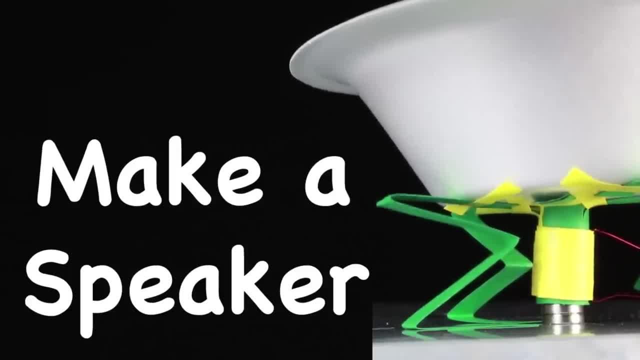 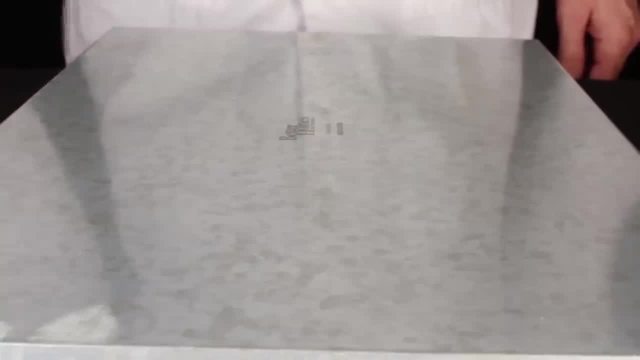 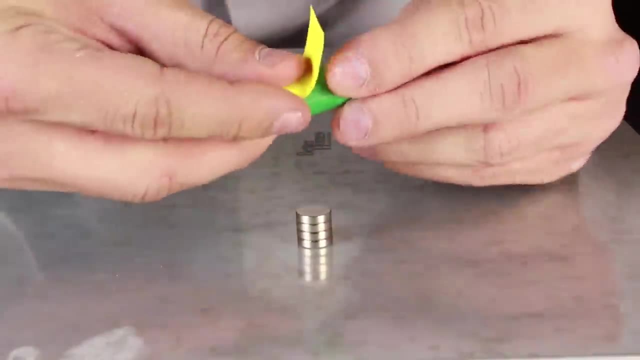 Bearded Science Guy here and today I'm going to show you how to make an electric speaker. To start with, place several neodymium magnets on a steel surface. Next, make a tube out of construction paper just larger than the neodymium magnets. After that, take one end of the tube and 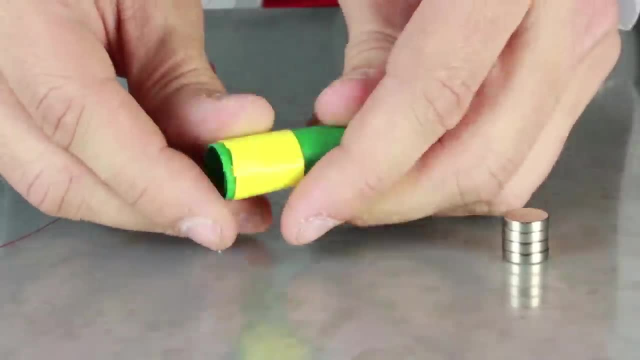 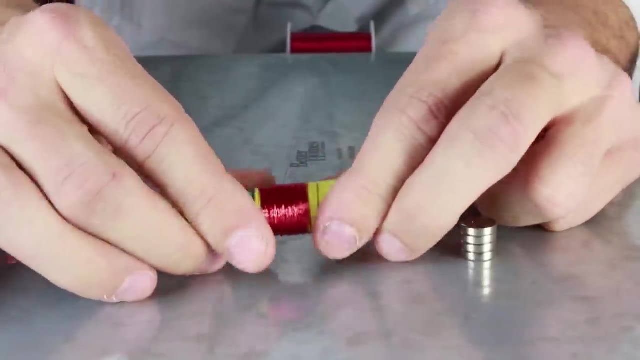 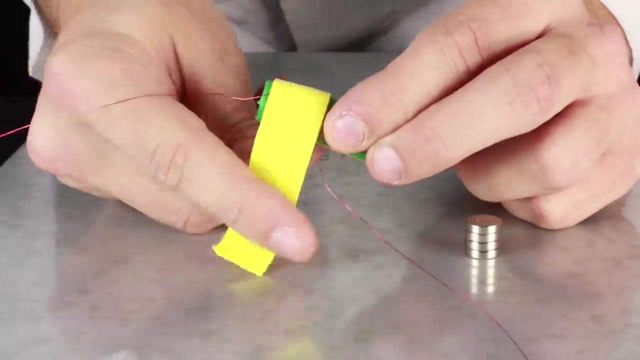 wrap it with a piece of tape with the sticky side facing outward. Take this piece of tape and wrap it with about 12 meters of 32 gauge magnet wire. Be sure to leave about a foot at either end of the magnet wire so that you can make connections. Make sure to tape this magnet wire in place so.